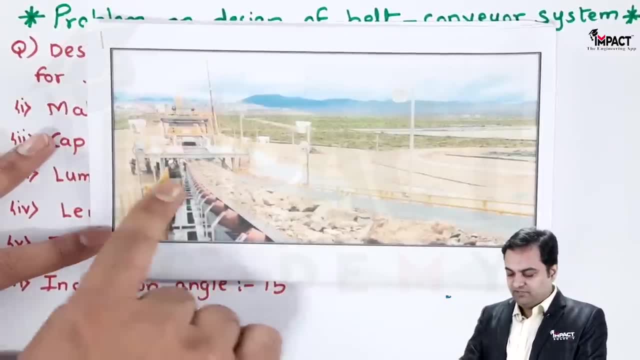 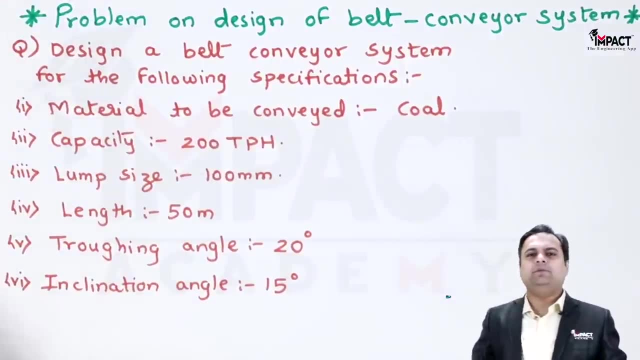 1 kilometer, we can transfer the material at a relatively longer distance. So even if the distance is 1 kilometer, we can transfer the material And, as per this diagram, we can easily see that the material is being conveyed on this belt. Next, the conveyed material: it can be coal. 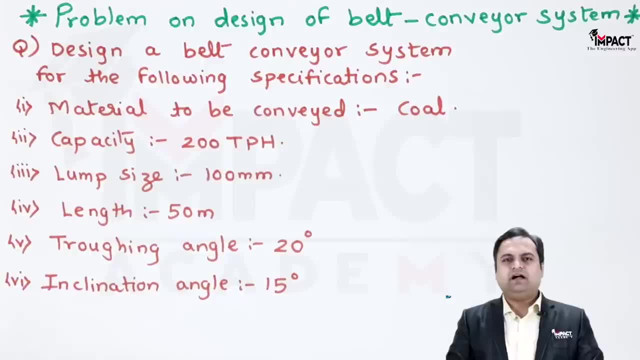 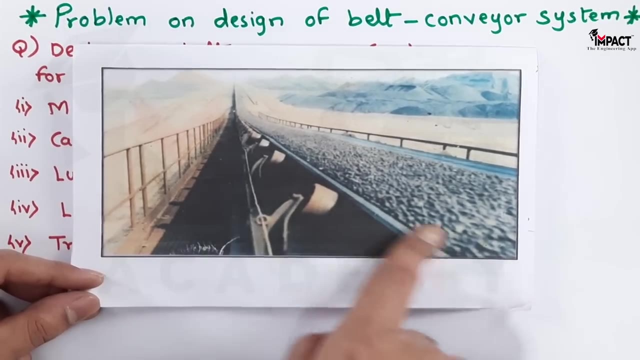 it can be clay, cement, concrete, iron ore, gold or gold ore, etc. The material can be anything which we are conveying from one place to another And, like, for example, in this diagram, we can see that the material being conveyed- it is coal And 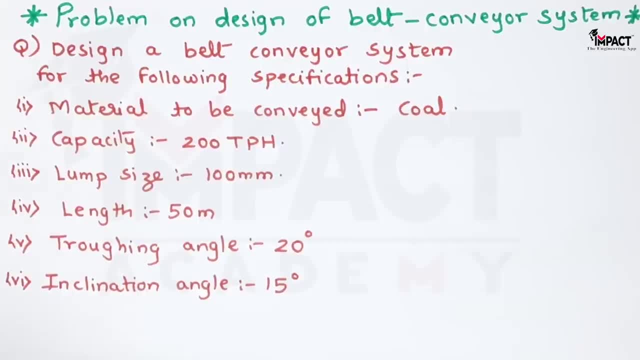 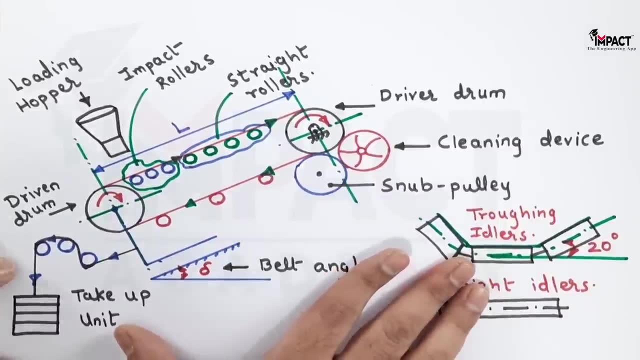 also the belt conveyor system can be the conveyor system made out of the wattage bandwidth And in this diagram some of the material given to the belt conveyor system. hopefully some more information on belt conveyor system will be explained on the diagram. So now we will see by the use of this diagram. at first, this drivenmwe have a driver drum. 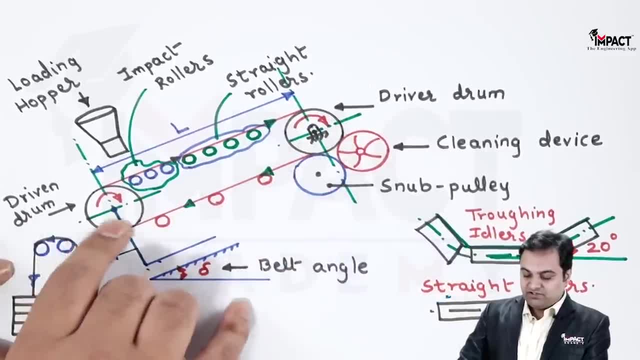 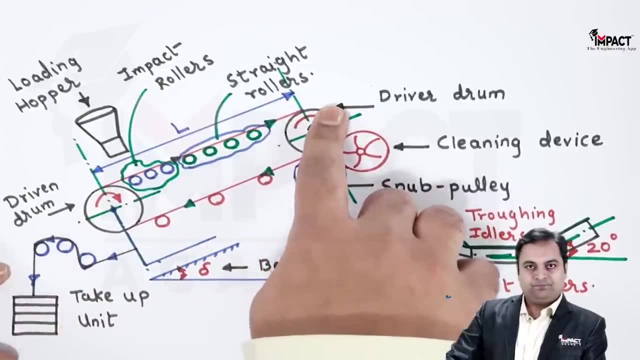 dicho driver pulley we will requiring at this time: fly a driver from left to right, you then the driver. it would take a left-��면 if the belly from right is in the clockwise direction. here is the positions, and the belt is inclined and we will see here And the 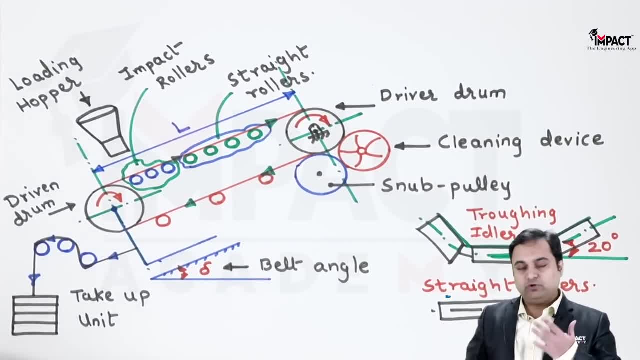 material is being conveyed to up. So that is the convention At first we have to take: or we have to hover raised its Peanut and the one less that which will beumer up side, or we have to assume that the material is being conveyed up until and unless it. 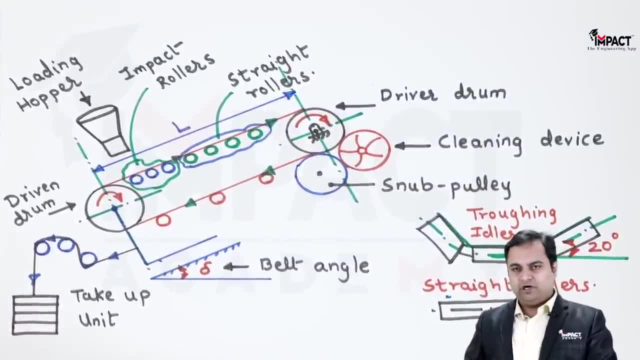 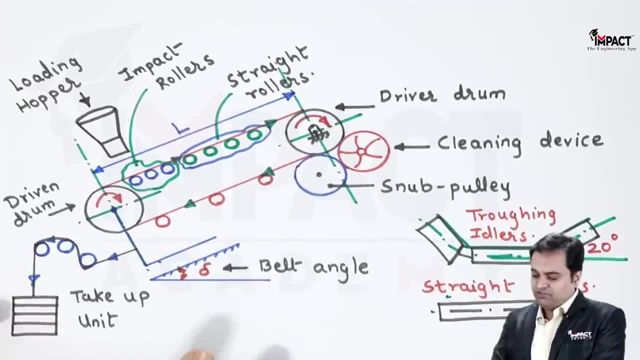 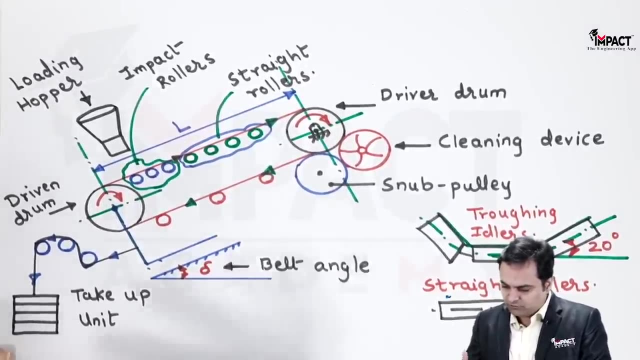 is specified in the problem that the material is conveying down, always we have to take that the material is being conveyed up. then here there are some descriptions which we have to see, or we can say some parts which we have to understand before designing the belt conveyor system. now what are those parts? 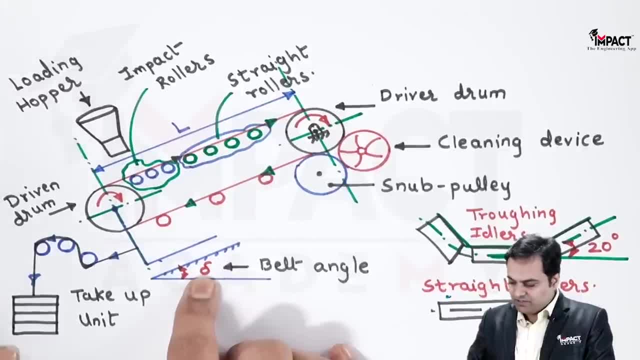 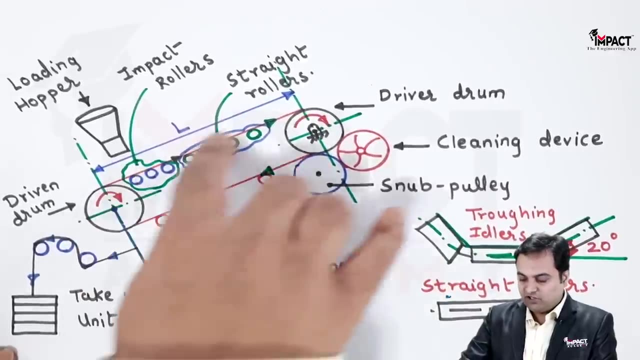 first of all I had explained this. Delta is the belt, angle means the coal is being conveyed at a certain angle, like, for example, in this problem. coal is given L. as we see, L is the center to center distance, or also we can say the distance of conveying. then here there is this loading hopper. so what happens if? 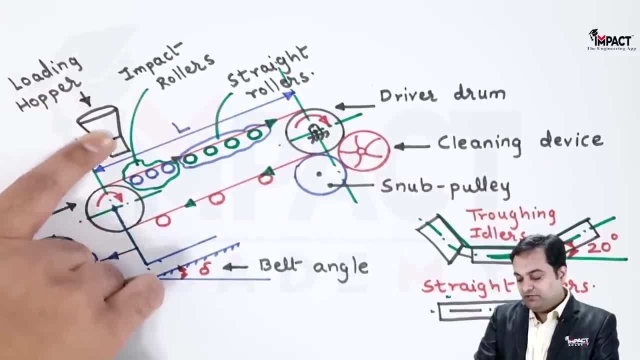 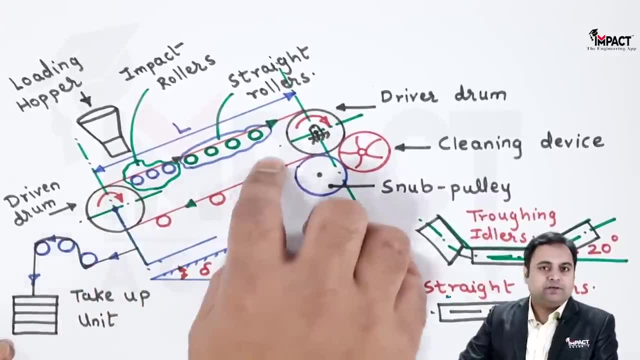 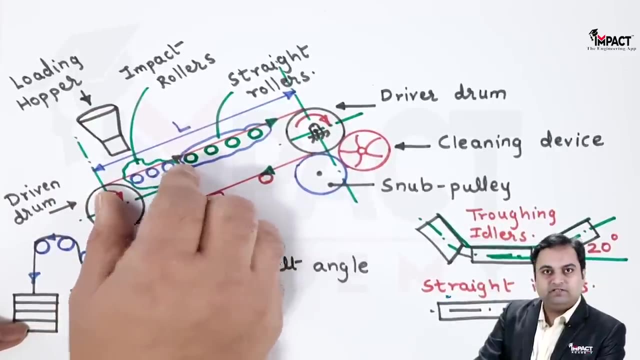 for example, the coal is falling from this loading hopper, it will fall onto the belt and in the start we have rollers under this belt. now, since the material would be falling from a certain height, we have impact rollers at the start of the belt. this impact rollers 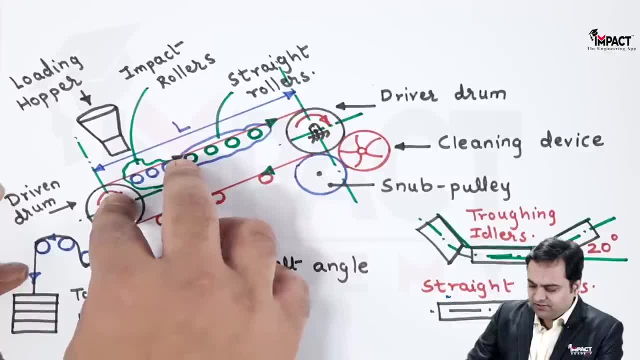 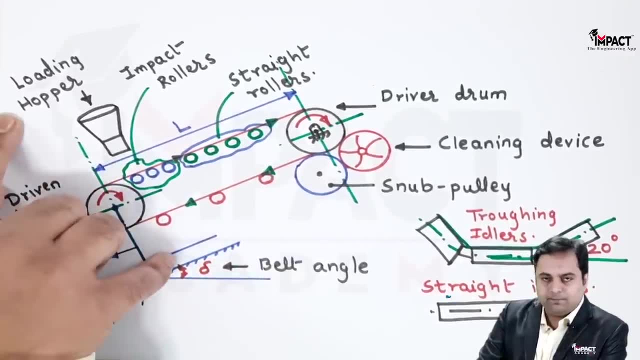 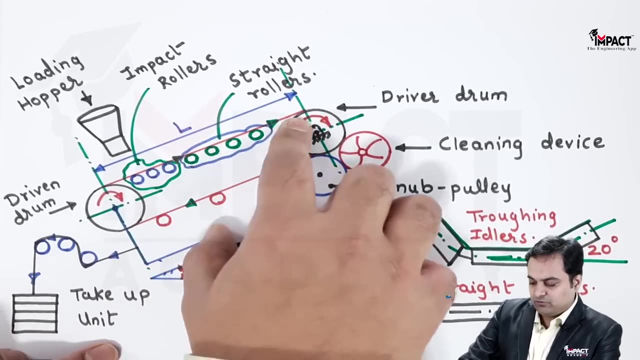 may be three or five in numbers at the start, and then this impact rollers are going to absorb the shock of the material which is falling and it will avoid the material from bouncing back. so here we have impact rollers, and further we can have straight rollers throughout, or even the impact rollers can be used. 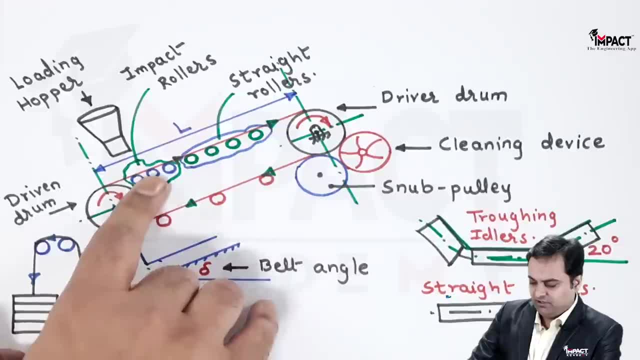 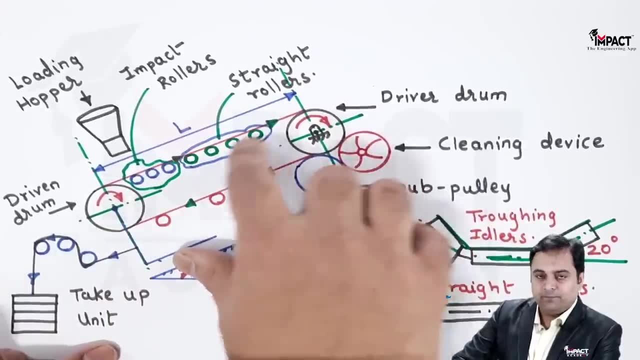 so whichever possibility is there, but at the start compulsory, we need to have the impact roller. then the material is being conveyed up at the same time. we can see the roller density is more on this top belt here that this is the top surface of the belt and here is the bottom surface at the 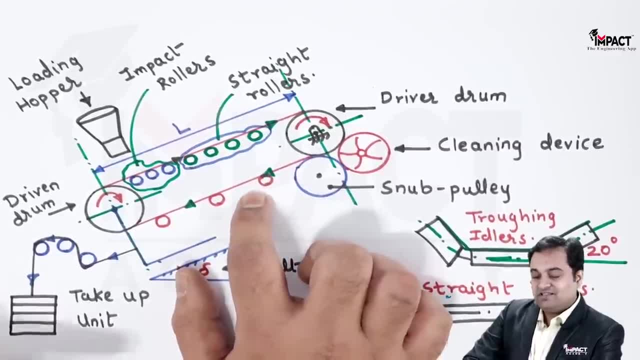 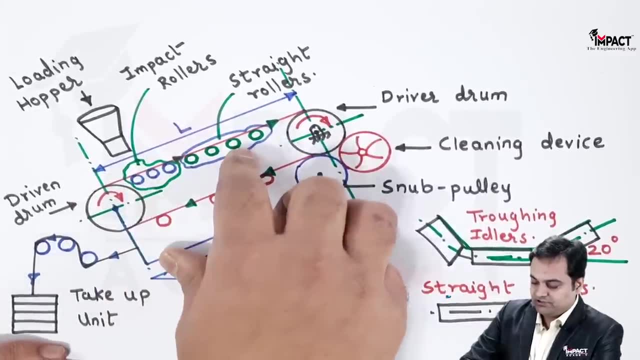 bottom we see that there are few rollers, while the reason being the material would always be there on the top side of the roller, so we top side of the belt, so we need to have more rollers on the top side compared to the bottom side, and here at the bottom the spacing is also more then on this. 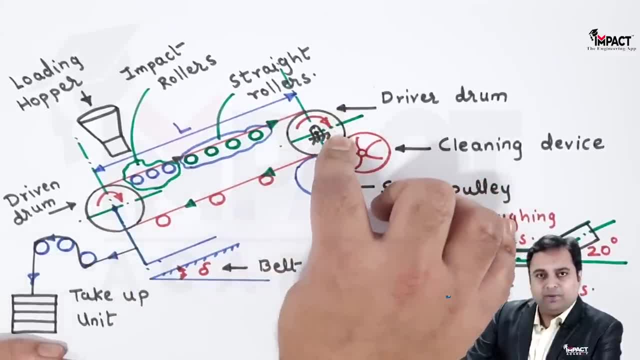 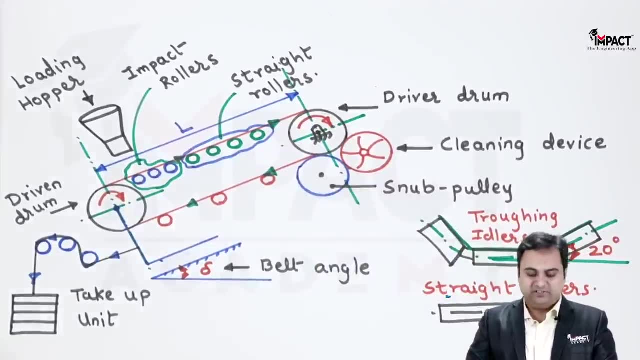 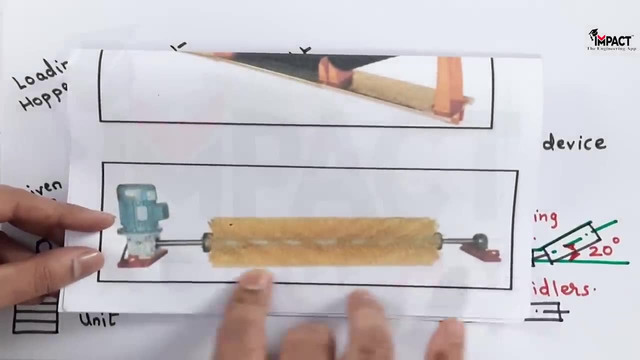 driver drum, since the material conveying material would be passing. so we need to have a cleaning device. this cleaning device can be a brush, it can be a scraper. that depends on the material which we are conveying. so here is the diagram. we can have such kind of cleaning brush attached to the pulley. 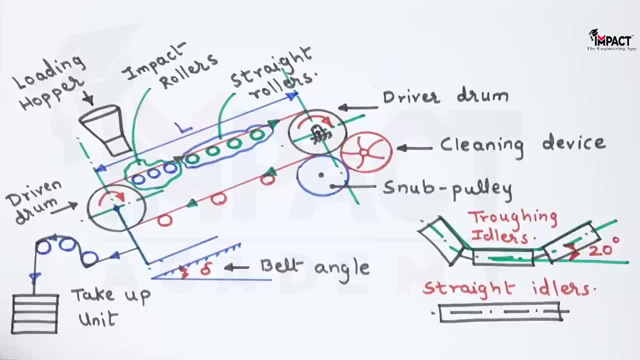 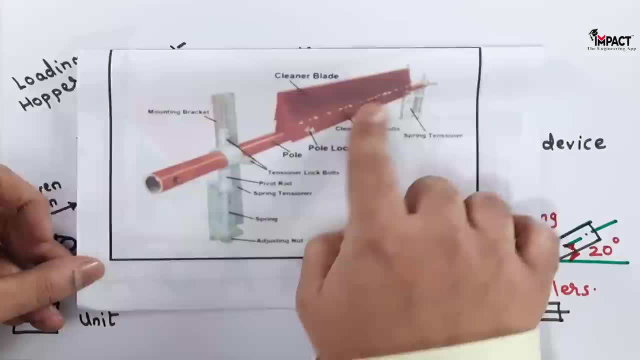 so that whatever material is being deposited, it gets clean from the pulley and at the same time, we can also have the scraper plates, like the one which is showed here. we can have this- this cleaner it is cleaner blade, or the scraper plate, we can say which is. 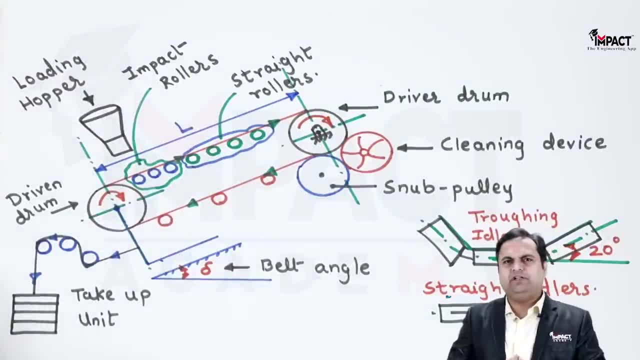 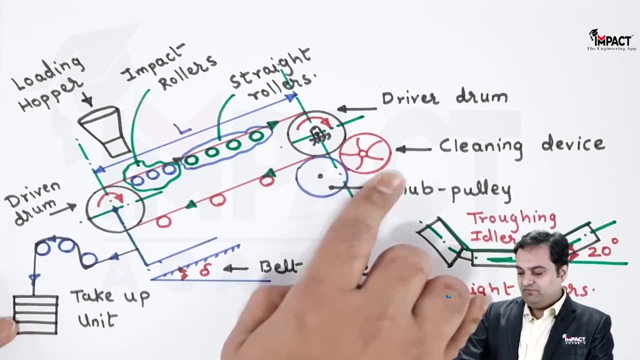 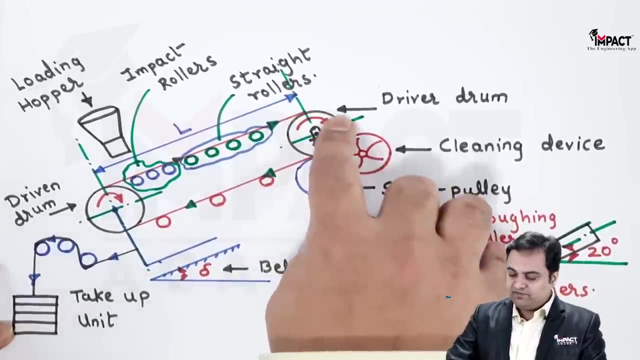 going to scrape the material, if the material to be transported is, for example, it is mud or gravel. in that case, to avoid sticking onto this driver drum, we are having the cleaning device which would clean the material. then we have snub pulley, see. snub pulley is used to increase the angle of lap of the belt. 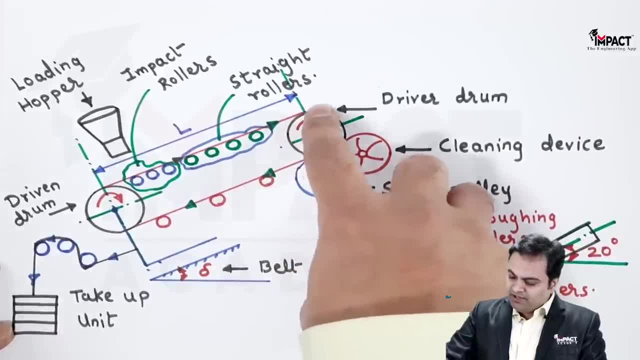 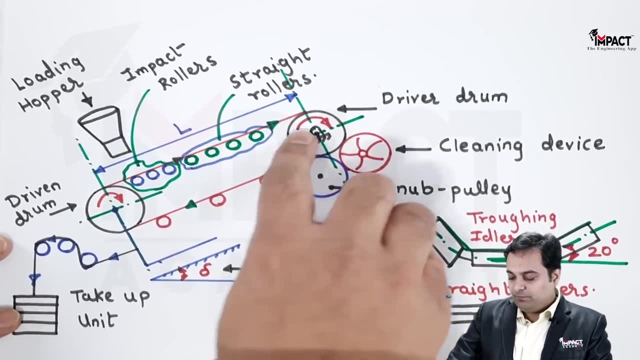 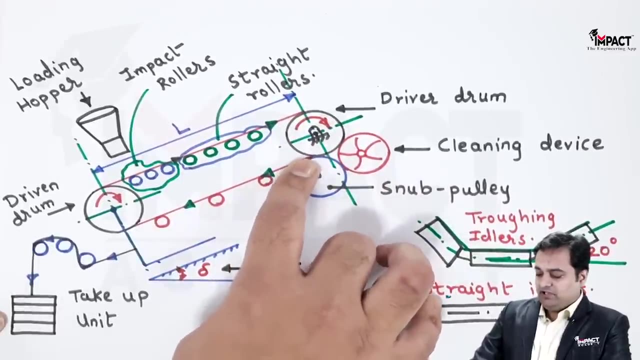 because the belt would should be in contact with the driver drum or in order to avoid the slipping of the belt, we have the snub pulley, which would be increasing the angle of lap. so by using snub pulley, the angle of lap increases and we can avoid the slipping condition at the same time, here on the driven. 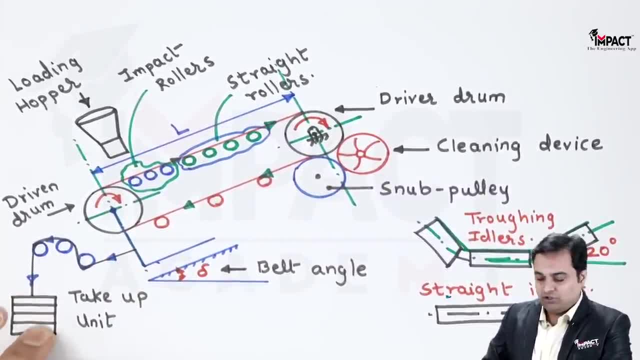 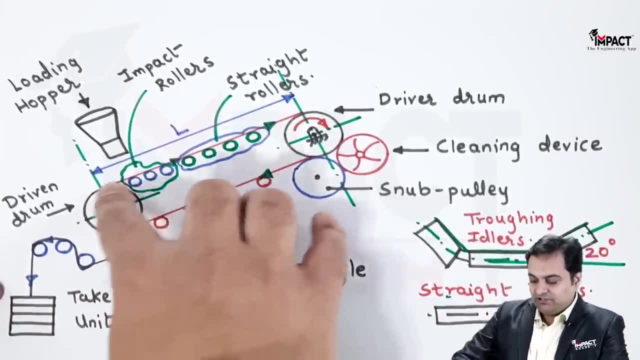 drum side. we have a take-up unit on which the weights are attached. we have a take-up unit on which the weights are attached. so by providing these weights, a constant tension is maintained over the belt and the material is being transported without the belt being sagging or becoming loose. so the tensioning unit is used. 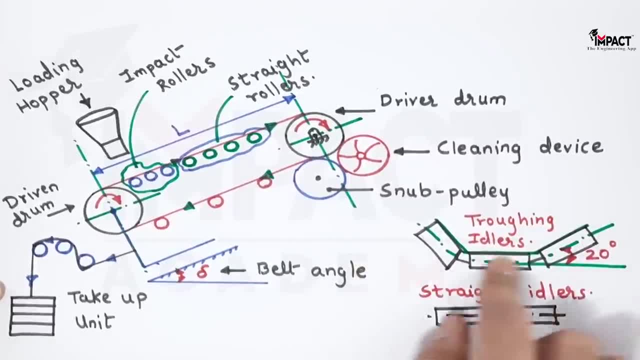 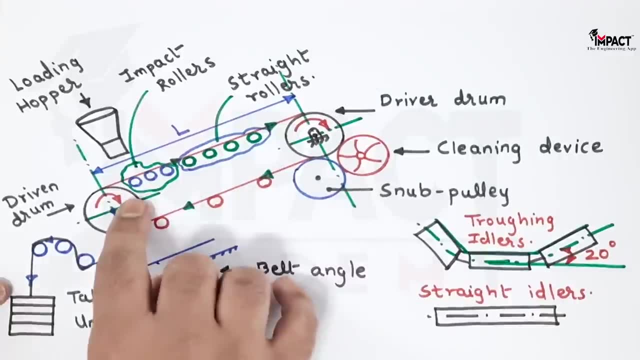 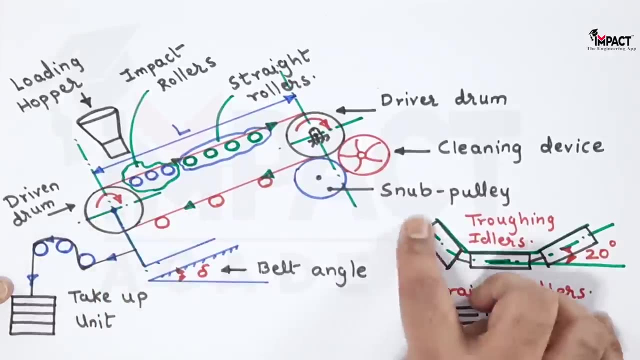 then, after that, here is the diagram in which the truffing idlers, or we can also say as truffing rollers, which are the impact rollers, they are inclined as we see here, or we can say the rollers which are used on the top side. they are in this shape, inclined at an angle of 20 degree. 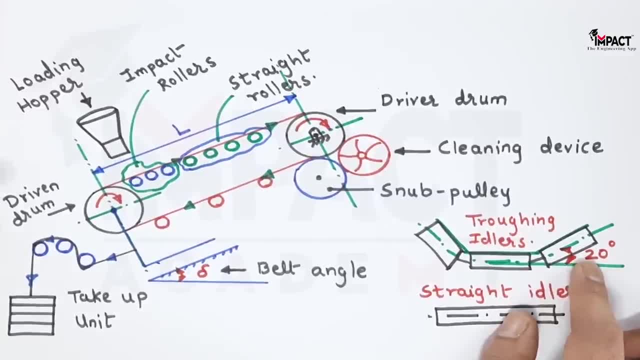 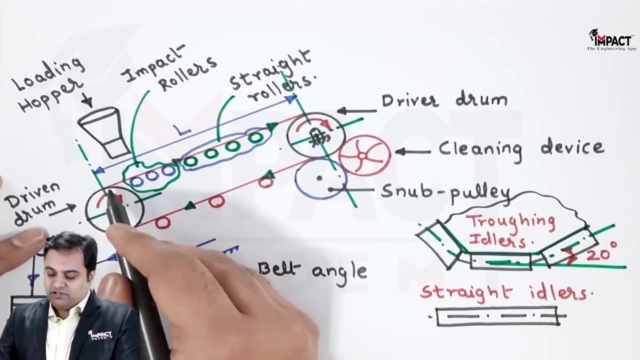 and this is the standard angle, remember next. so the shape of the truffing roller, idler or roller is such that we can keep the material over it, because if the belt is straight and the rollers are also straight throughout, then what will happen is the material may fall while conveying. 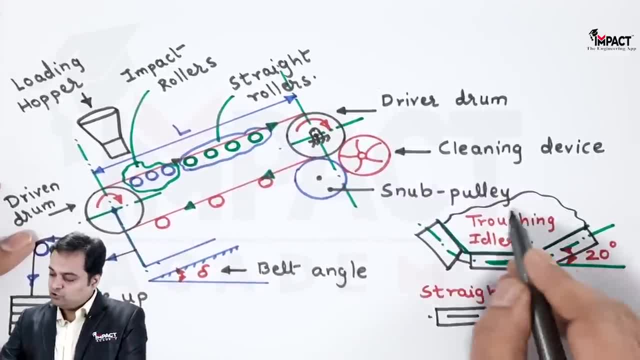 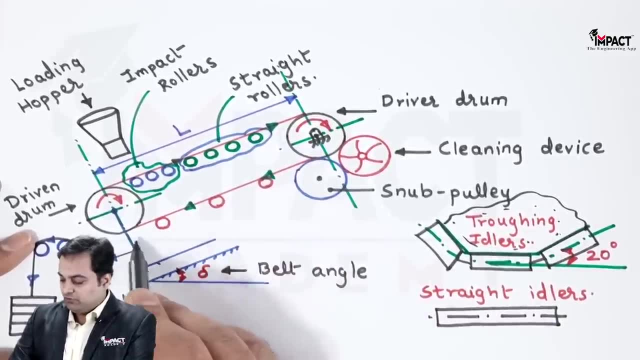 it. So we are having this bucket kind of shape here so that it can hold the conveying material. so that is a truffing idler and straight idlers which are there on the bottom run of the belt or the bottom rollers. we can say these are straight in cross section because they are not in contact. 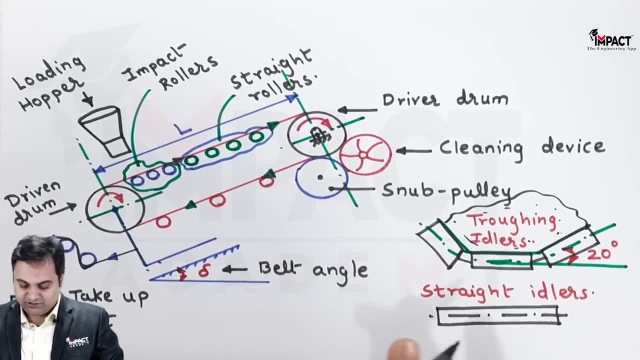 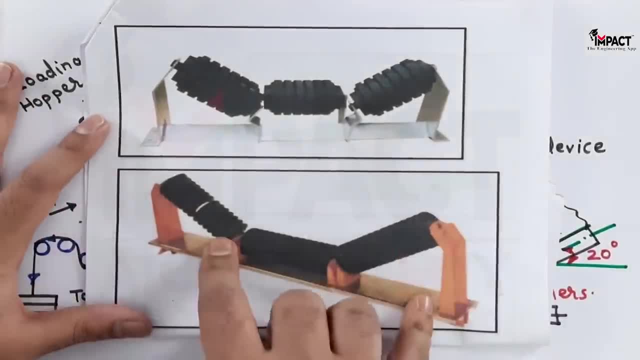 with the material being conveyed. so, in short, that was the description regarding the belt conveyor system. the next part is here. I am giving the diagram. see. this is: this is the way in which the truffing idlers, or truffing rollers, are conveying the material. 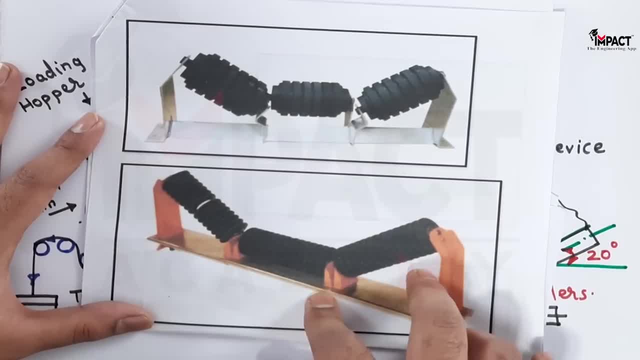 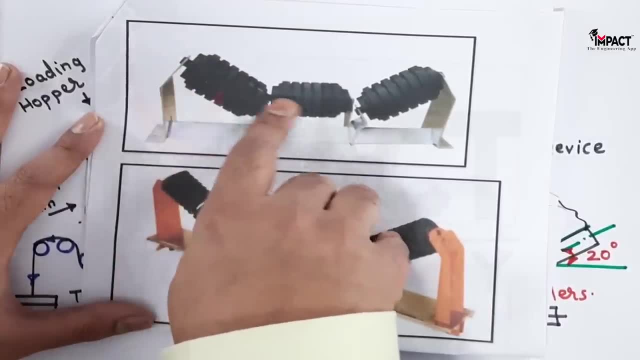 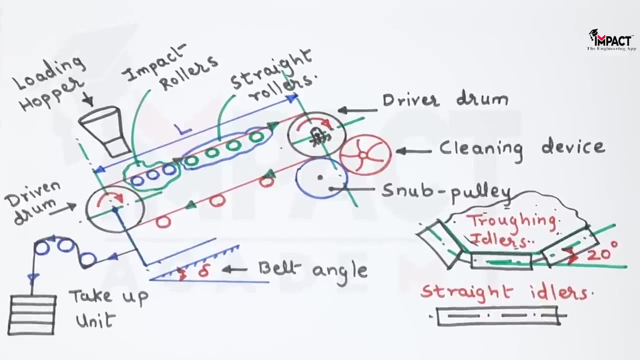 look like, as we can see here, over which the belt would be there and the conveying materials kept, also these Idlers. they consist of metallic tube or rollers, over which here we have these rollers mounted which are going to absorb the shock, and then, after assembling, it would look. 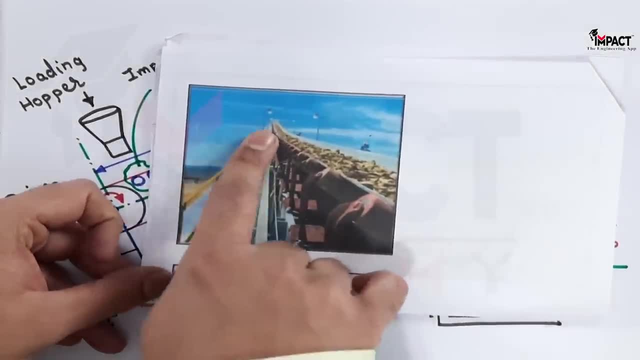 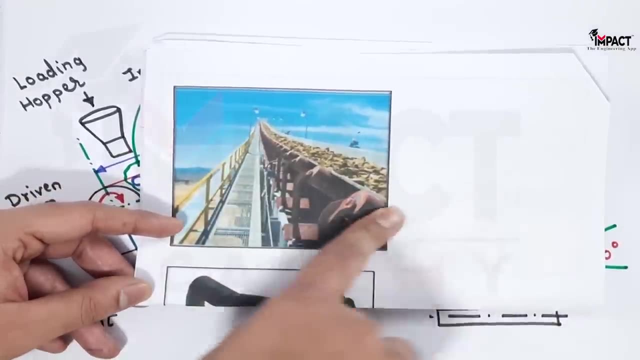 something like this, as we can see in this diagram: here there is a belt conveyor system and these are the idlers- or we can say the truffing idlers- in the belt, and the conveying material is being carried to the главное combiner. 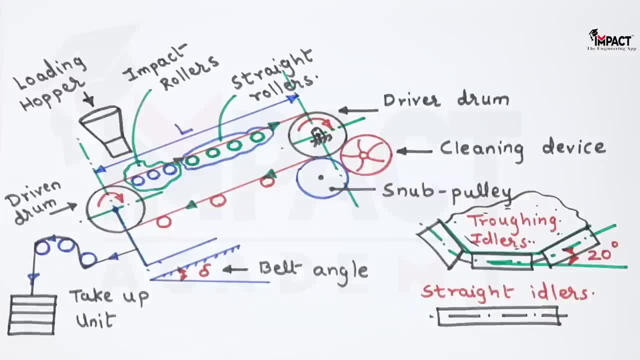 it. so that is the description. now, once we have understood, or we have got the knowledge of the belt conveyor system, the first thing which we want in the design is we need to know how many steps are there. i'll make this problem, or this design, as simple as possible. first by noting how 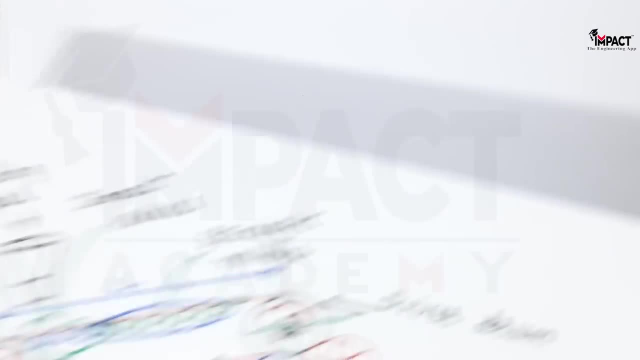 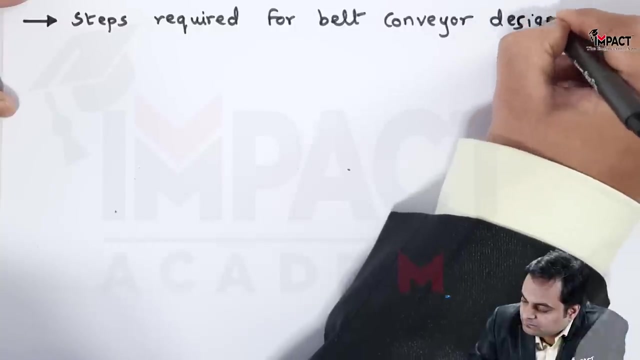 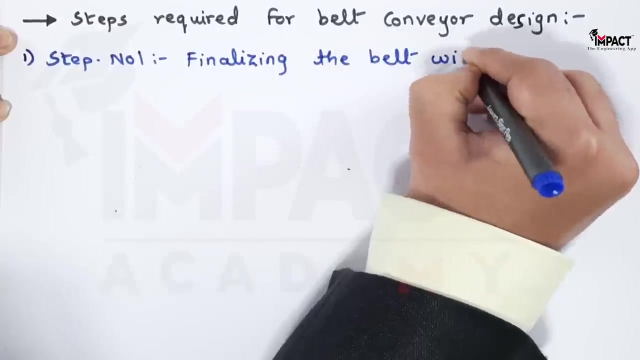 many steps are to be used and what we are going to do in each of the steps. so let's get started with it. so these are the steps which are required. so the first step is in. the first step, we are going to decide or we are going to finalize. 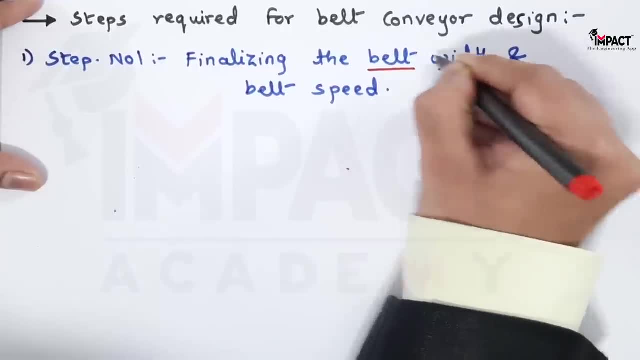 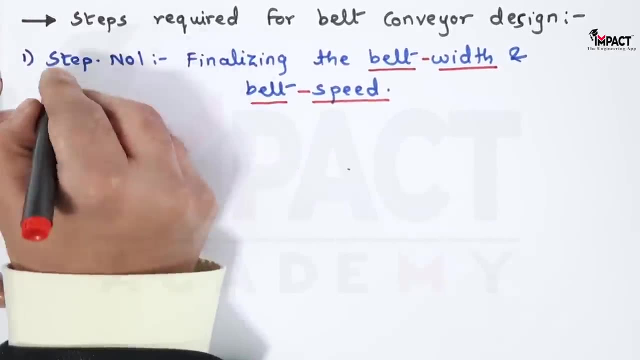 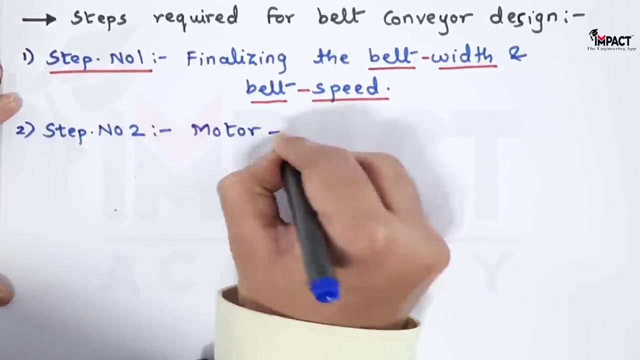 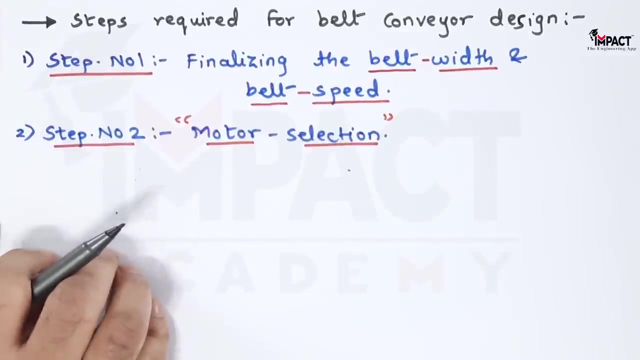 how much should be the width of the belt. so we are going to decide how much should be the width of the belt and what should be the speed, or we can say the linear velocity, of the belt. so this is step number one. next step, number second, is motor selection, where we are going to determine how much should be the power and the rpm of the 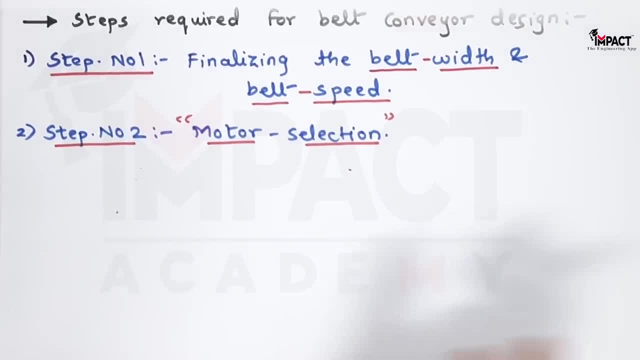 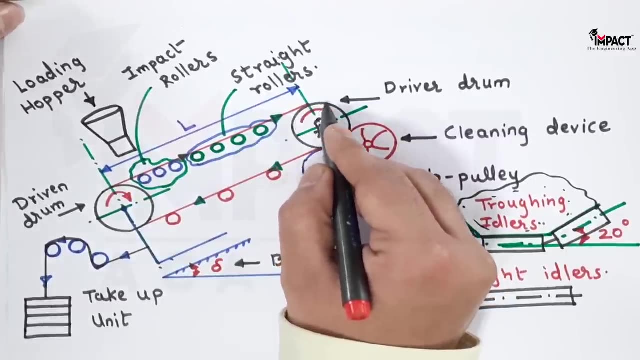 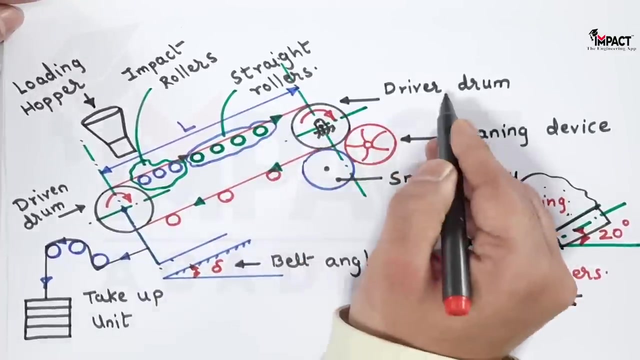 motor which is going to drive or which is connected to the driver drum. because here we need to give power only to the driver drum or the driver pulley, and that drum would be driving the driven drum with the help of this belt. so we need to give power to this driver drum. so we 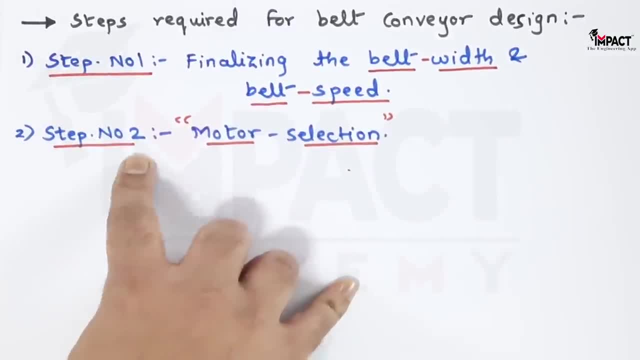 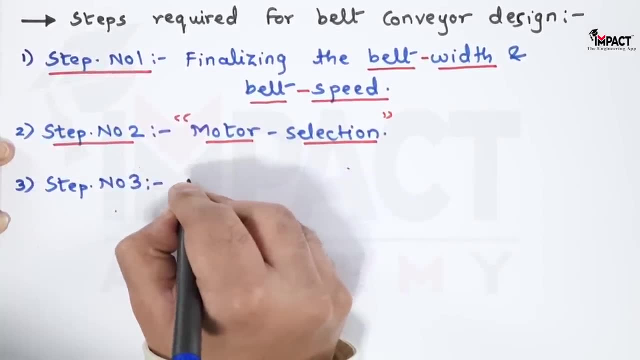 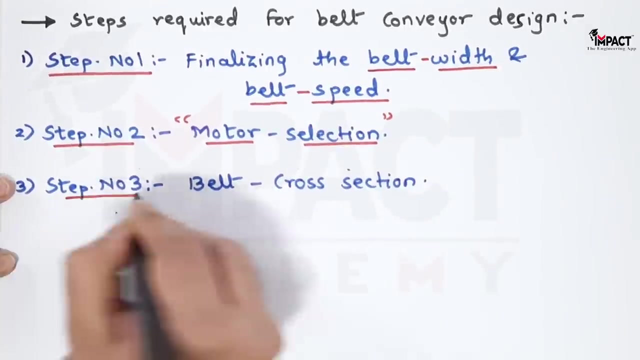 have to find the power of the motor in step number two and the rpm as well. next step number three is deciding the belt cross section. so we have to design or find the belt cross section. so we have to design or find the belt cross section, that is, finding the dimensions of the belt. next step number four: 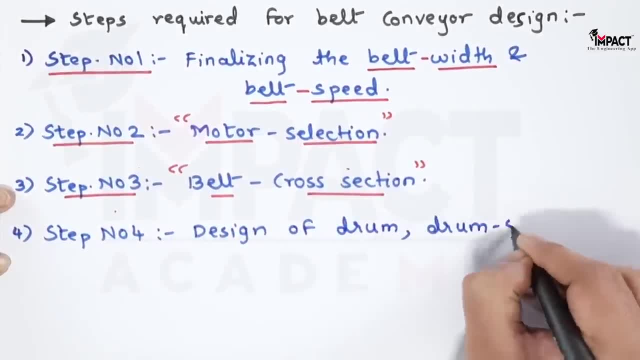 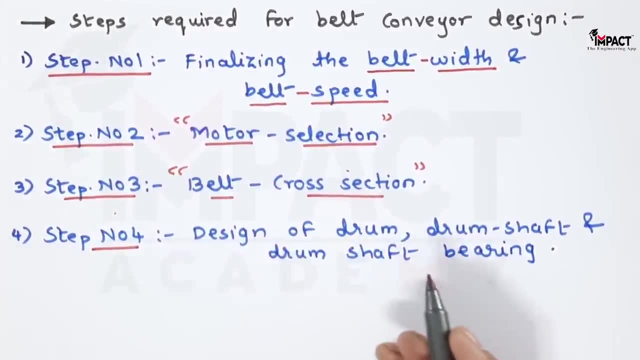 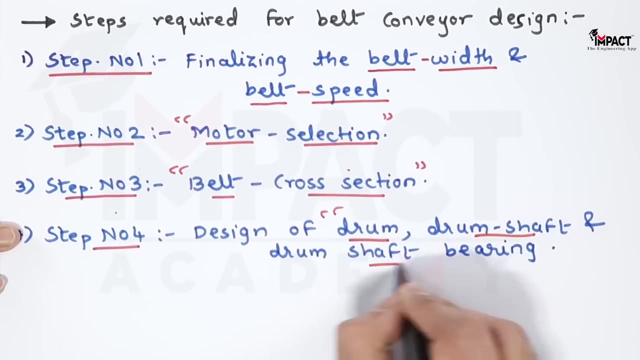 that is, finding the dimensions of the belt. next, step number four: here we are going to decide the diameter of the drum, that is, the driver and driven drum, the drum shaft and the drum shaft bearing. so that is step number four. after step number four, there is step number five, in which we 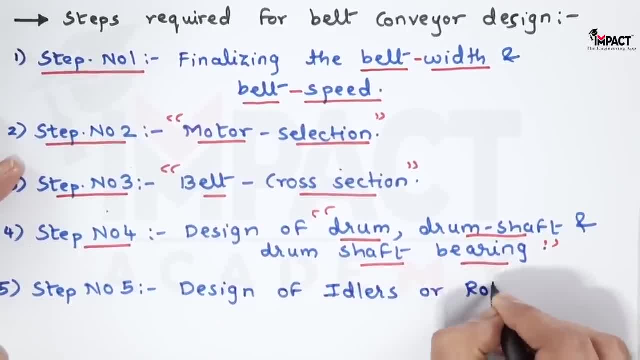 are going to design idlers, also called as roller. so, in short, Wine axe, rode, start from rate into freestyle. guts are a vise to ride around the bike which this lure is going to give a very wide angle. So, in short, these are the five steps which we have to remember in the belt conveyor design. 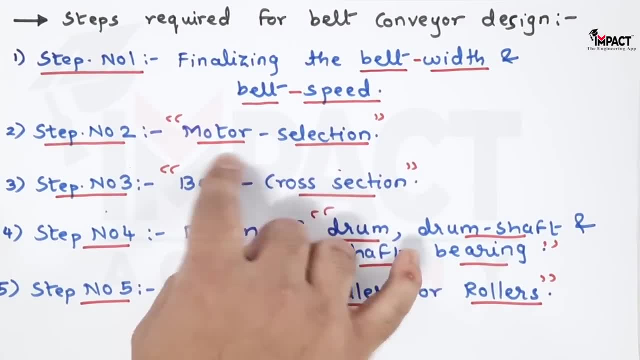 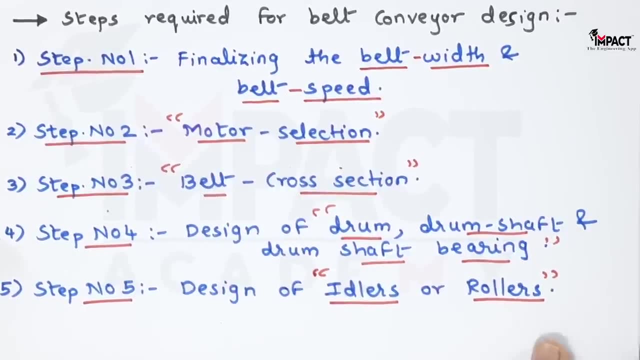 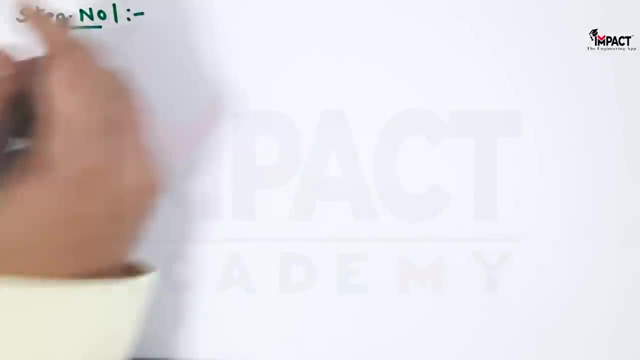 system, starting with the belt width and belt speed. second step: motor selection, then belt cross section, then the design of drum, drum shaft and drum shaft bearing. finally, design of idlers or rollers. So once we have understood what are the steps, let's get started with step number one. 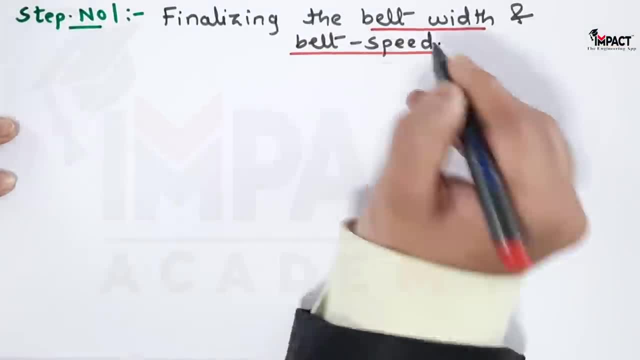 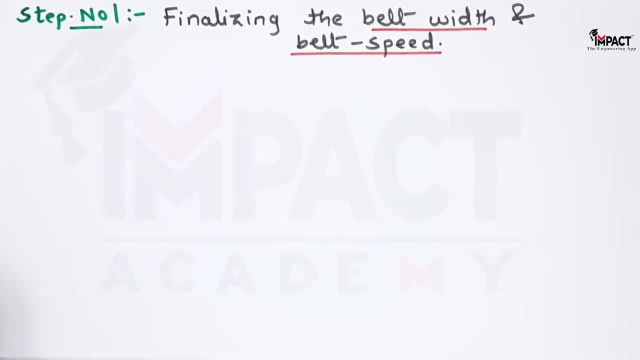 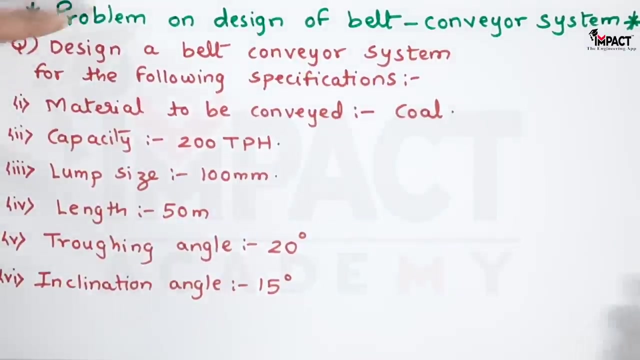 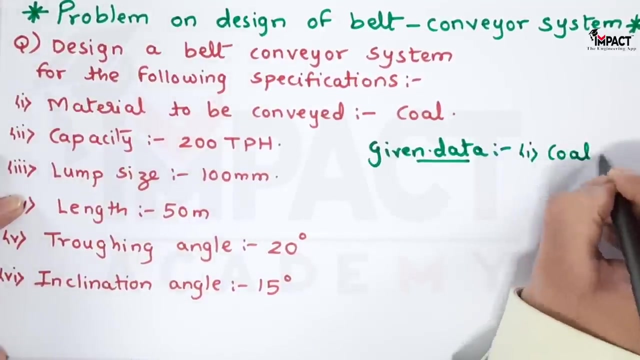 So here we have to finalize: how much is the width of the belt and the belt speed. for that we have to read the question And in this question, if I want to write it in the form of the data, it becomes: the material to be conveyed is coal. 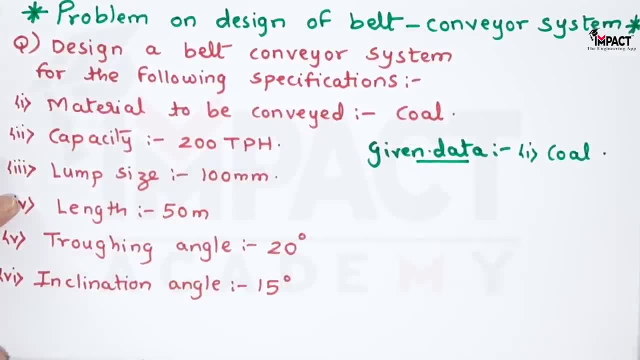 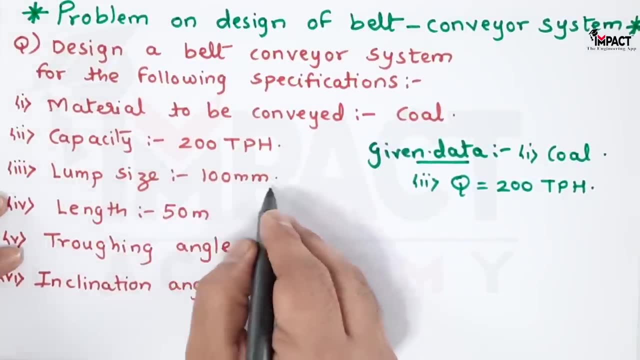 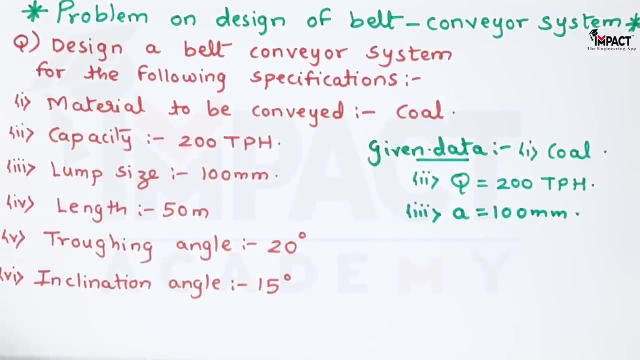 Next, the capacity is 200 tons per hour, 100 as capital Q, Then the lump size is 100 mm given. Now, whenever in the problem the lump size is given, lump size means the size of the coal, because here we are going to convey the coal. 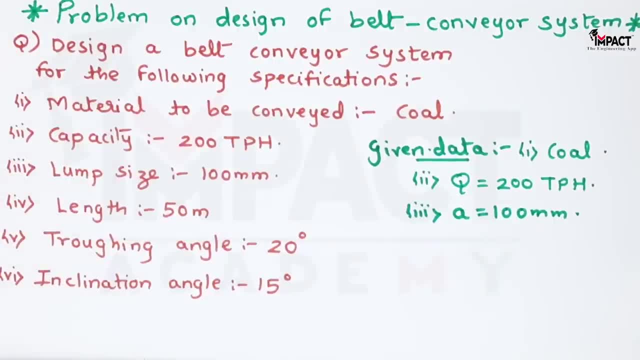 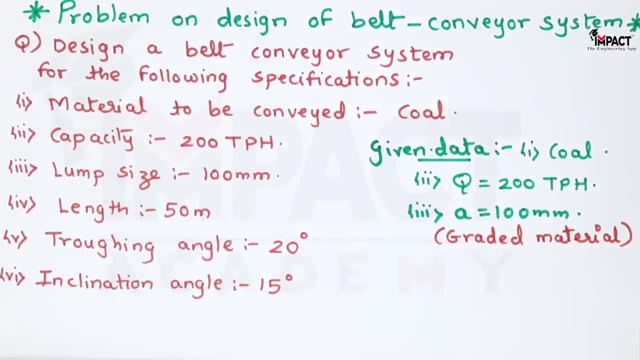 So the size of the coal is given to us. So that means whenever size is given, it means it is graded material. it is called as graded, It means The coal sizes are fixed. they are of 100 mm having equal size which are being transferred. 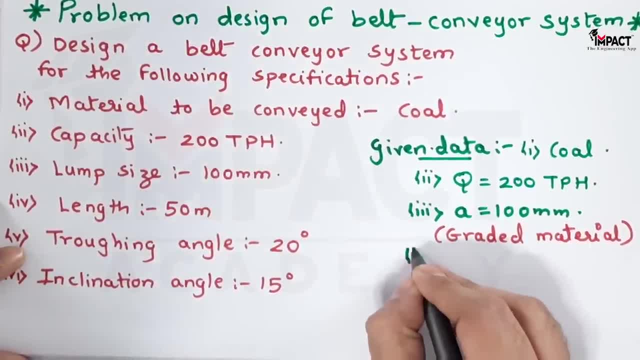 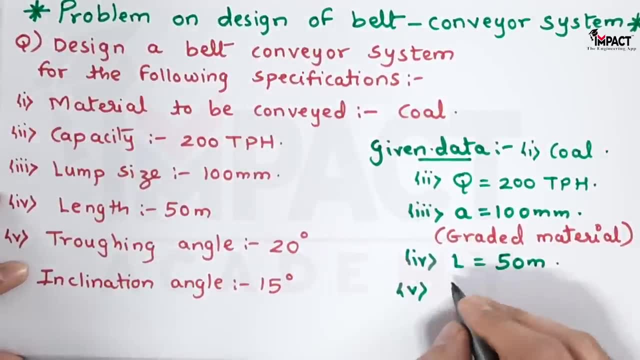 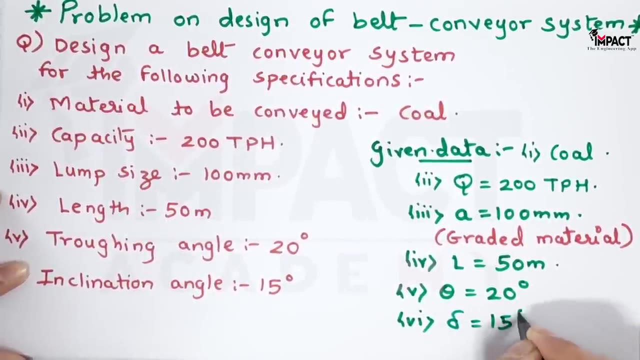 Then the length of conveying is 50 meter. The troughing angle is given as 20 degree. so troughing angle, I am denoting it as theta, and the inclination angle, delta, is 15 degree, which we can say it is also the angle of the 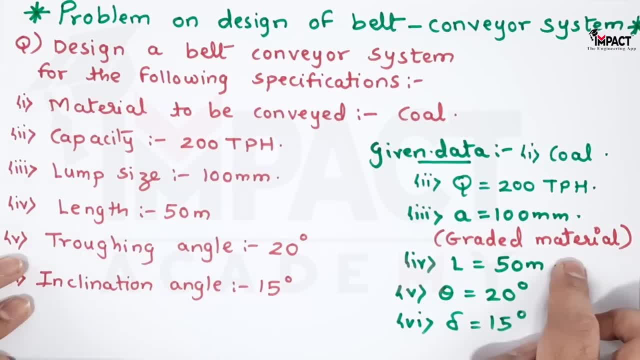 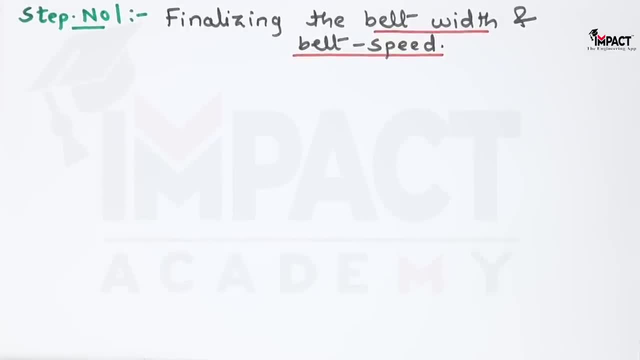 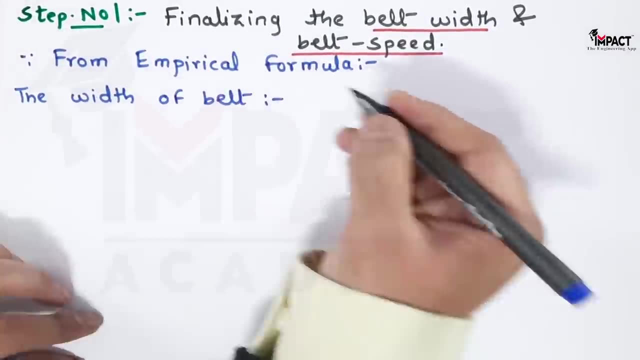 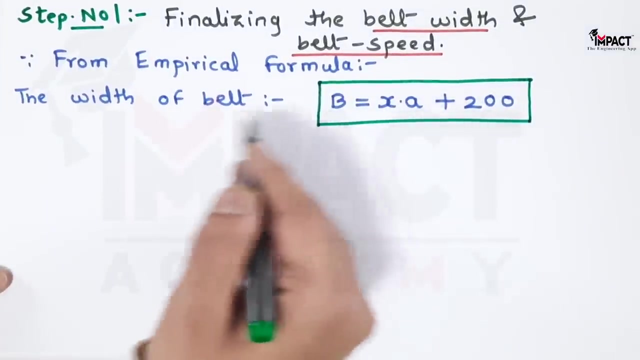 belt. Now I hope you have understood and remember that here we have graded material. So how to start the problem for the graded material? Empirically we have a formula in which the width of the belt is given by. Now, here this is the formula by which we can calculate the width of the belt, which is: 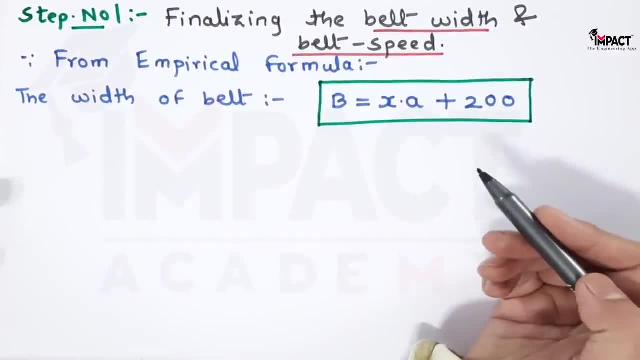 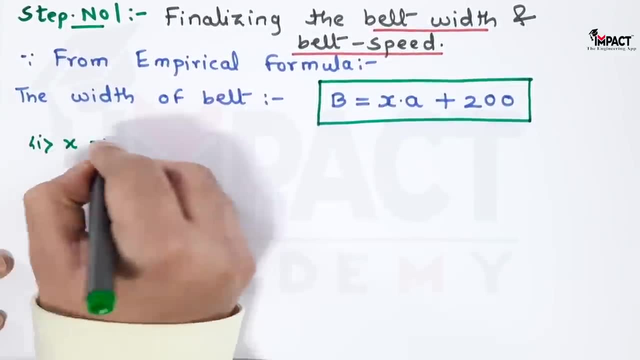 B is equal to X into A plus 200.. This formula is the formula for the weight of the belt. So this is the formula for the weight of the belt. It is there empirically. we have to remember the formula and here X value is: it is 3.5. 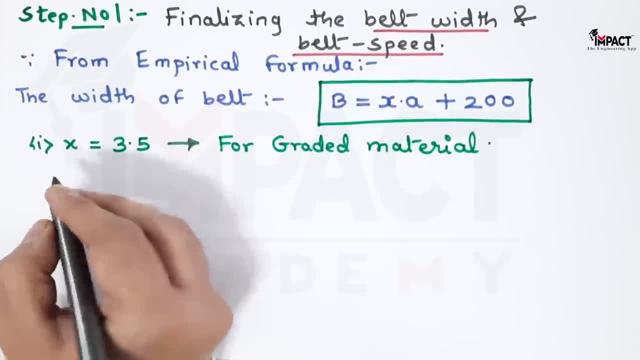 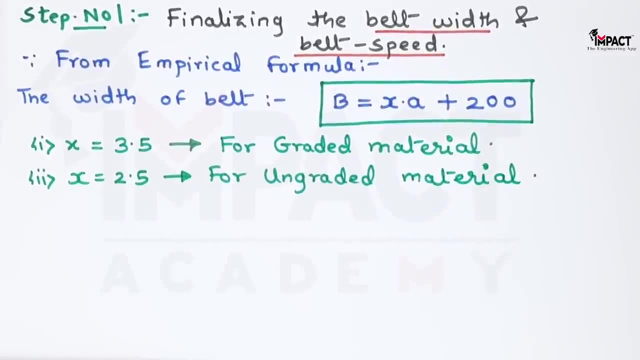 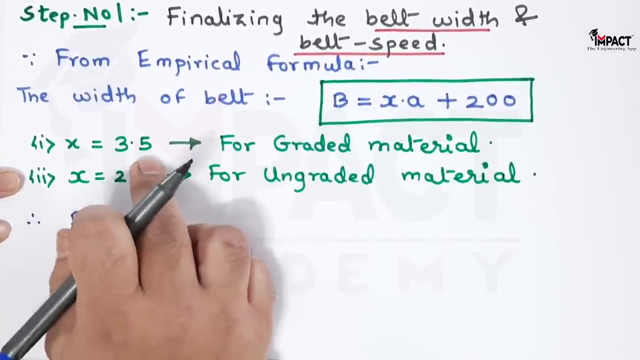 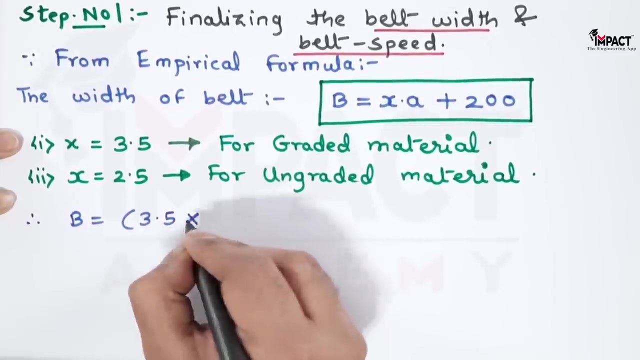 for graded material and it is 2.5 for ungraded material. Now I am putting the values. so therefore B is equal to X, since it is graded material. because the size of lump is given, It is 3.5. X value into the size of lump is 100 mm. 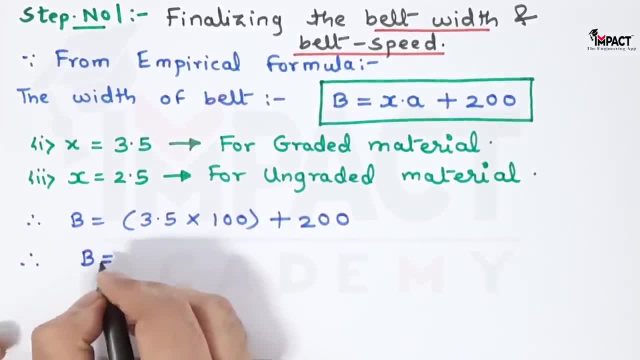 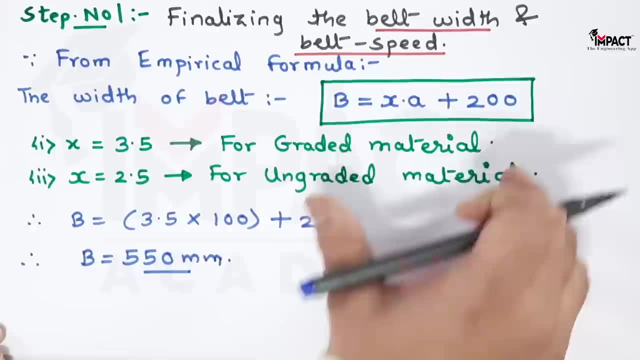 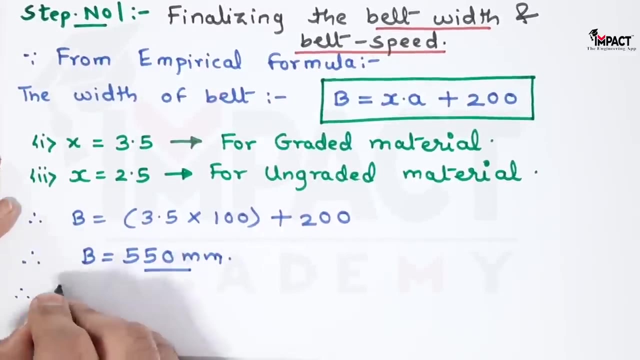 So, therefore, the width of the belt comes out to be 550 mm. Now, once I have calculated the width by using this empirical formula, Now I have to select the standard width of belt from PSG, So, therefore, So from PSG, So from PSG. 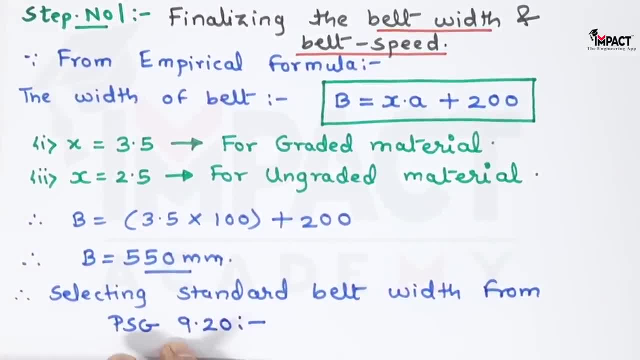 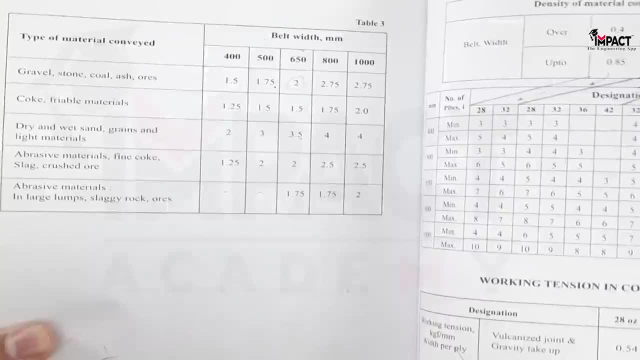 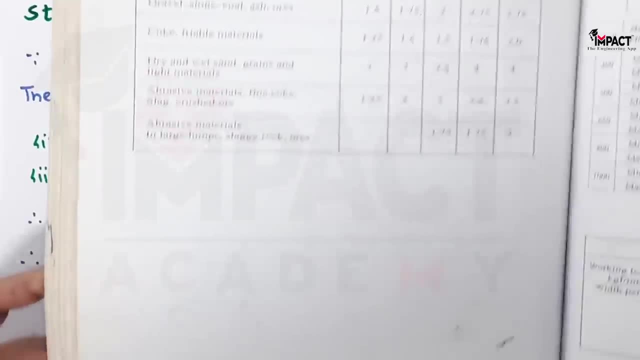 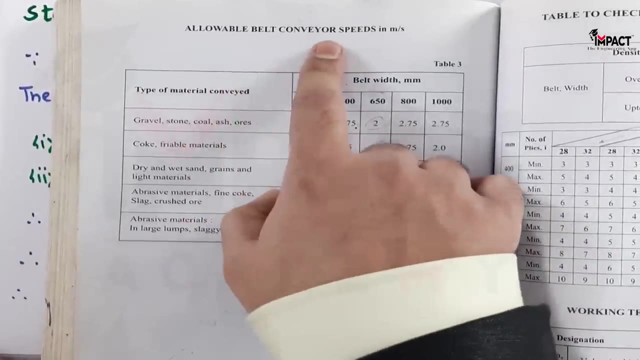 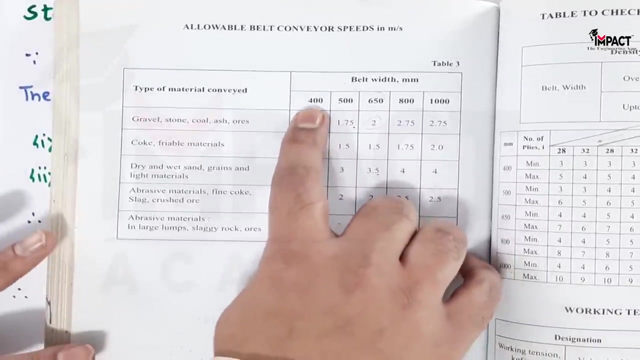 On this page, number 9.20, as we can see here on page 9.20.. So allowable belt conveyor speed. so we have the velocities as well as the belt width width. Now the belt width is starting from 400 mm, then it is 500, 650, 800 and 1000 mm. 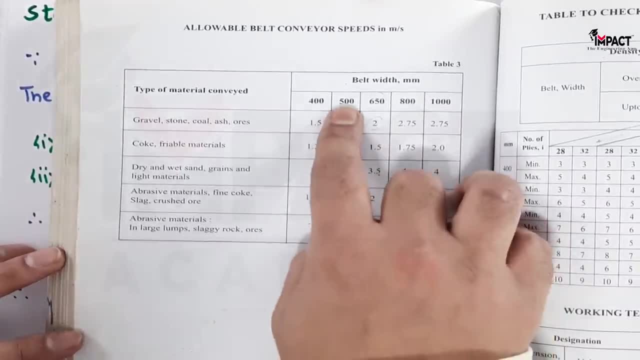 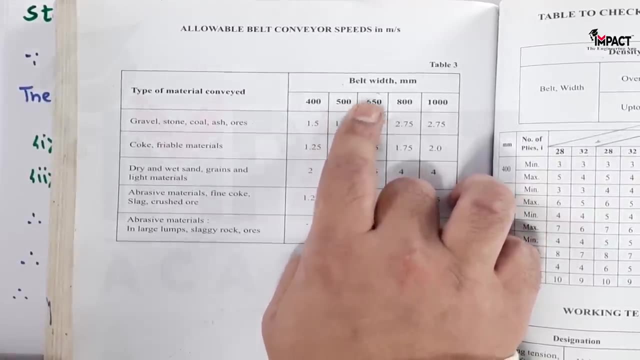 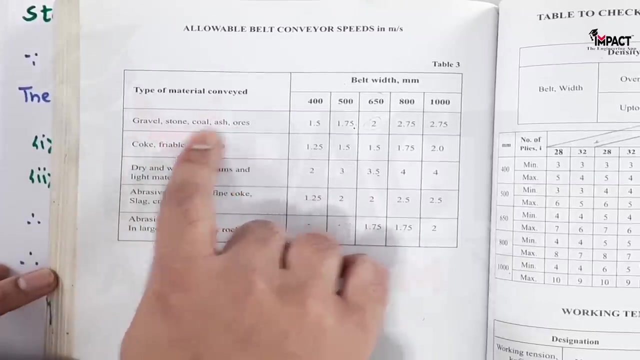 The answer which we have from the empirical formula is 550.. So select the next higher value. So after 500 we have 650. So our value is in between that. So I am going to select 650 mm as the width of the belt and at the same time here the material are given which has to be conveyed. 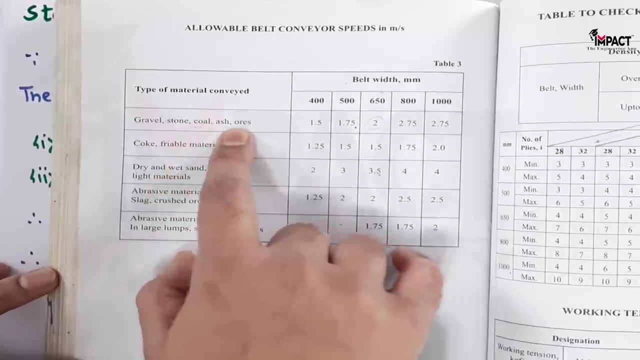 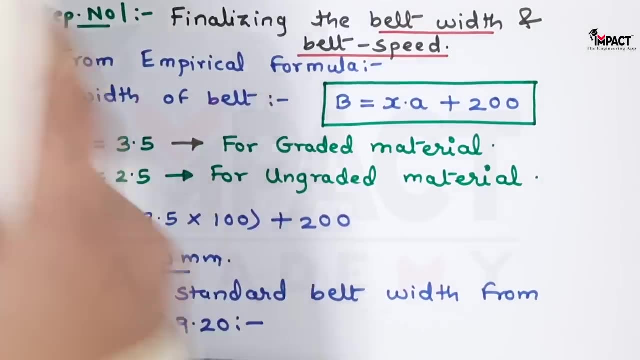 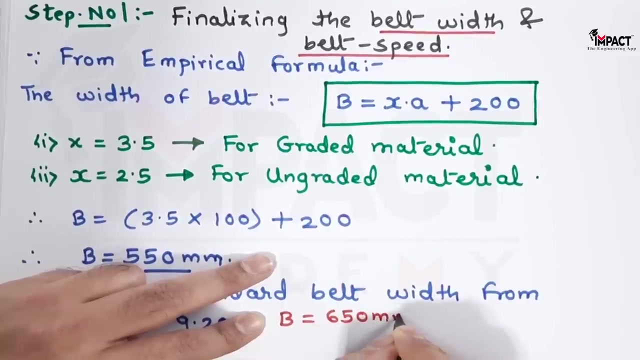 So the material is coal for us and therefore 650 mm would be the width and 2 meter per second would be the velocity. So from this reference, I get the standard width of belt as 650 mm. Also, it is 0.65 meter and the velocity of the belt is 2 meter per second. 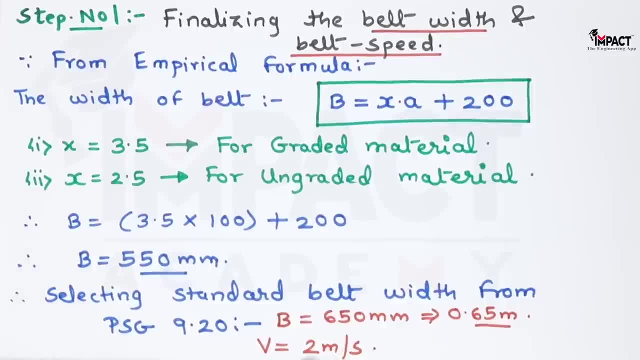 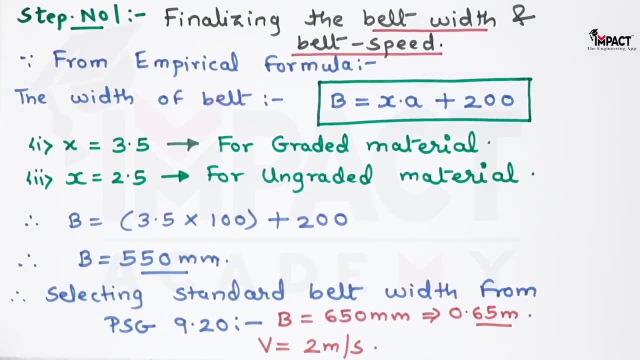 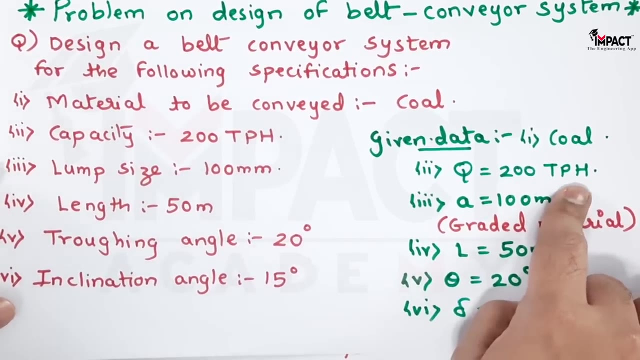 Now, once I have selected the standard width of the belt and velocity, here I am going to check if this belt can transfer the required quantity of coal, which is 200 tons per hour. So we have to check if the belt selected can carry this quantity or not. So for that the reference is: 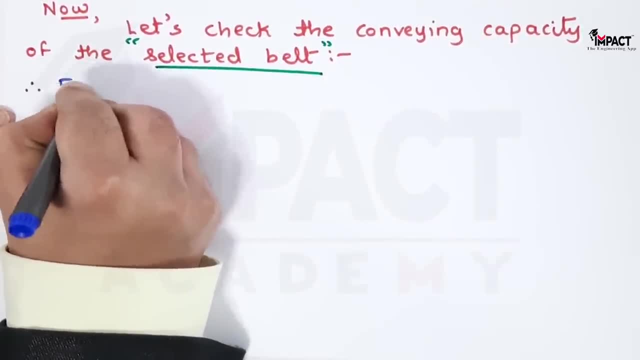 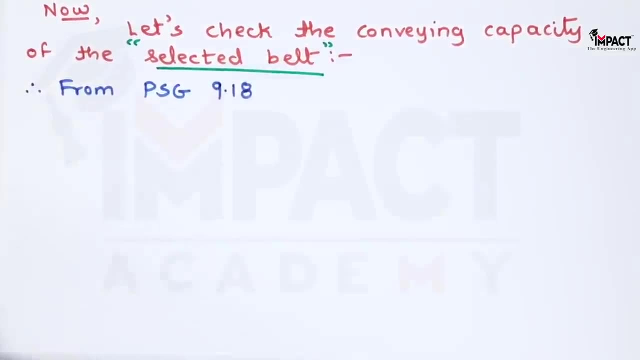 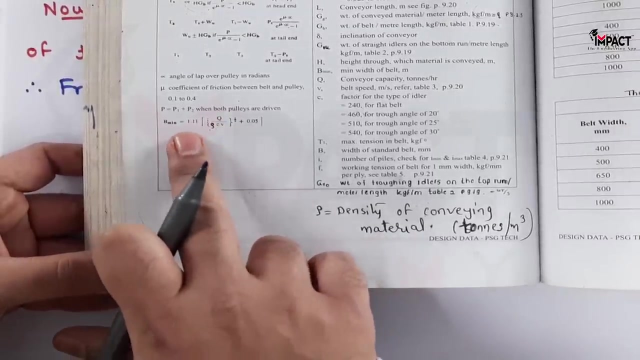 0.65 meter. So therefore, from PSG design data book, page number 9.18, it has the formula. Here we have the reference PSG 9.18 and in that we have to use this formula of B minimum, because what is B minimum? 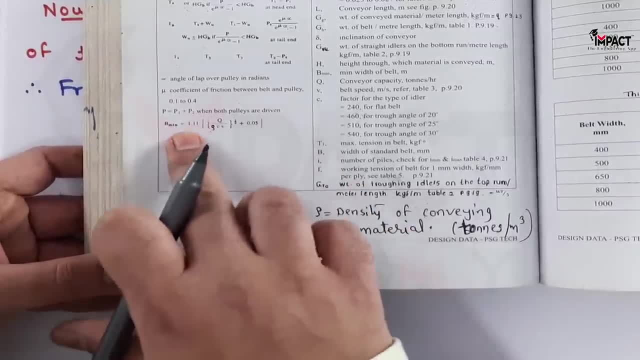 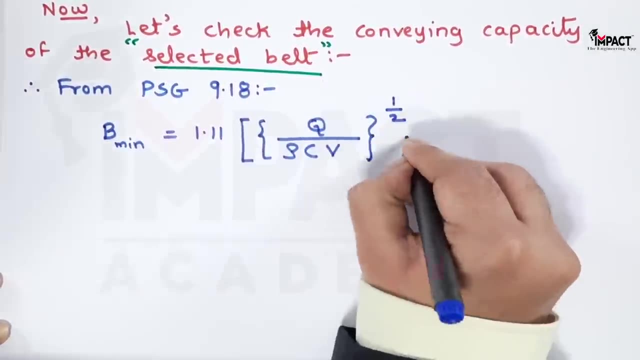 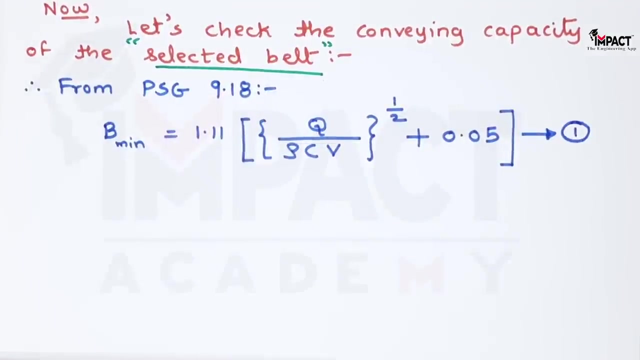 It is the minimum width of the belt. So we have to use this formula. I write it over here And in this cafe. we have to use this formula. We have to use this formula as equation 1.. And in this formula B, minimum is the width of the belt. 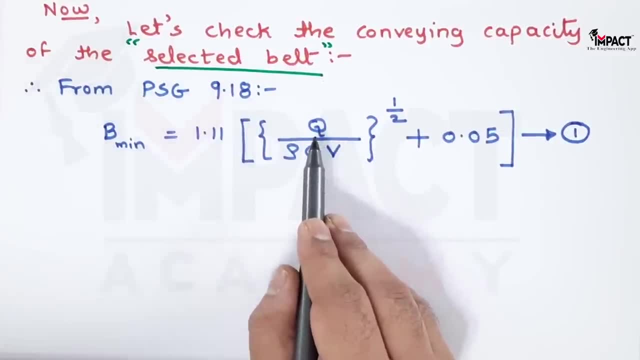 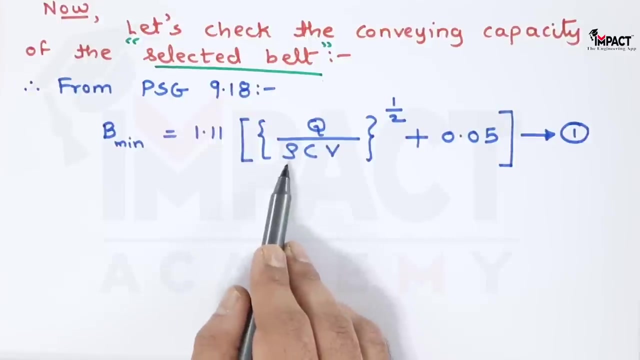 It has to be taken in terms of meter. Q would be the carrying capacity, or we can say the capacity of the belt conveyor. Then rho is the density, So R is a density incorporating weight, So R is the density of the conveying material. remember, this row is for the conveying material, so in this case it is. 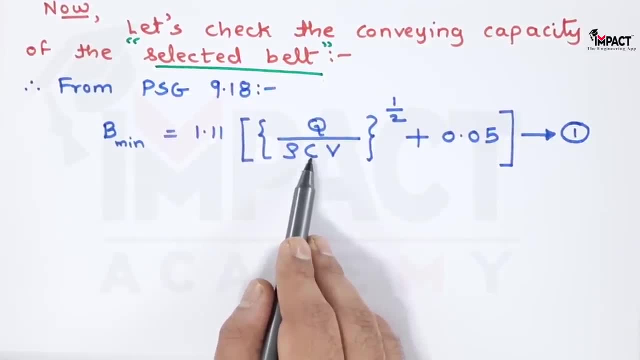 cold. so we have to know the value of density, then c. it is called as the factor for the type of idler, and here in this case we have the troughing idler angle is given as 20 degree and v is the velocity of the belt. so one by one i am going to find the values, starting with the density. so therefore, 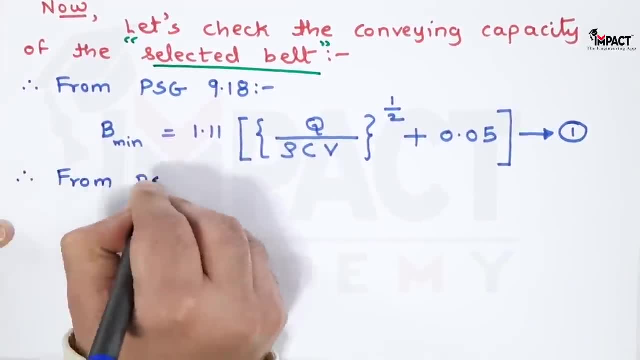 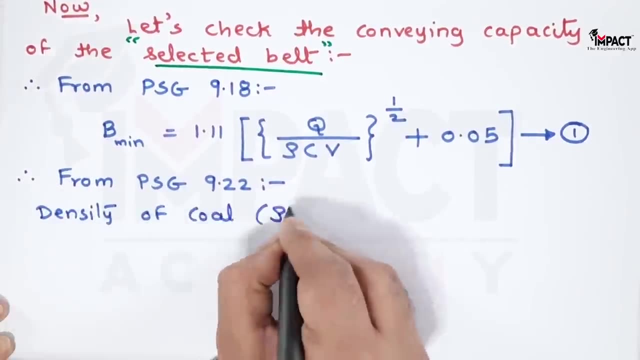 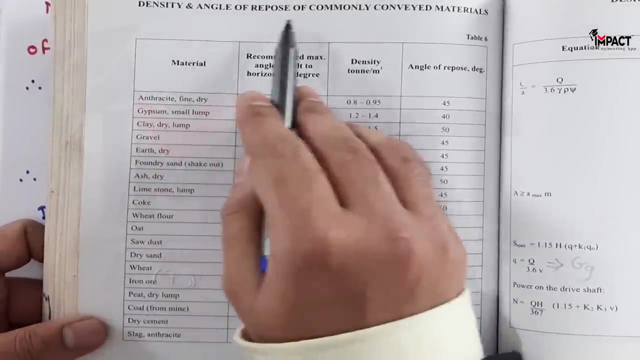 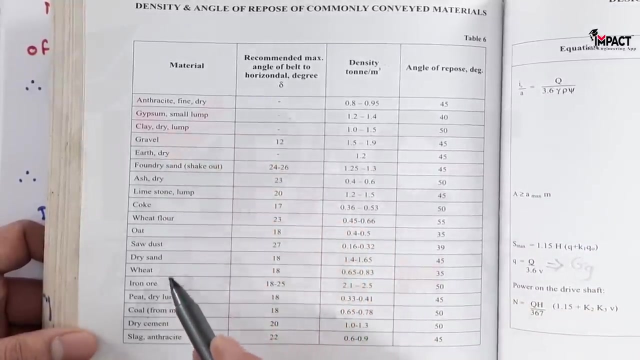 again using the reference from psg, so from psg 9.22, the density of coal. i'll write down. so here on page number 9.22, at the top we have density and angle of repose of commonly conveyed materials and here in the first column we have the materials. so we can see these different materials. 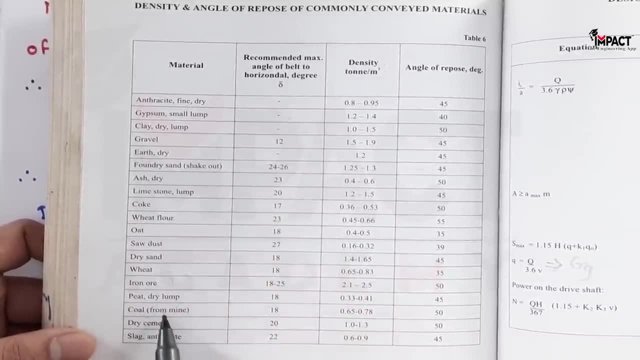 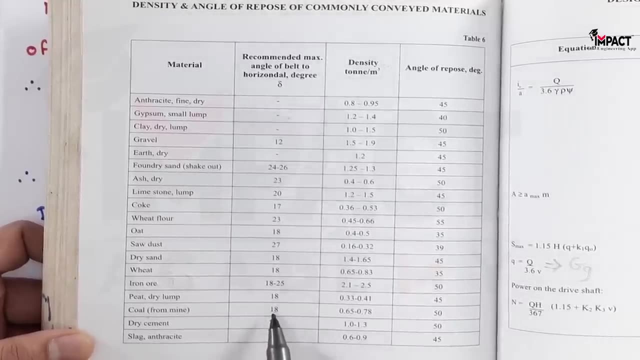 and for us the materials are: material is coal, as we can see here, the material is coal and for coal this 18 is the angle of the belt, if it is not given in the problem. but here in this case the angle is given as 20, so we have to take that angle, and if this angle is not given, we can directly take it. 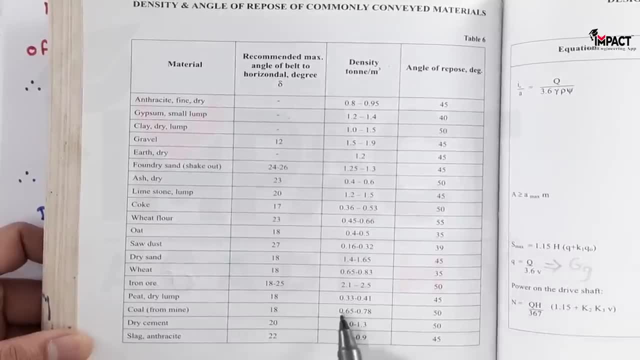 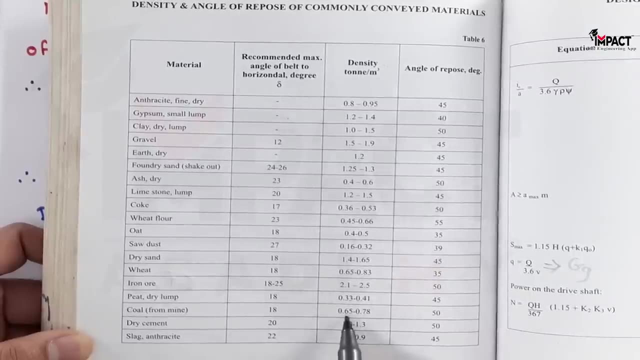 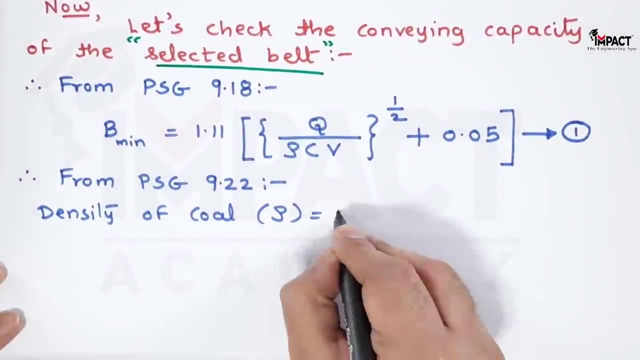 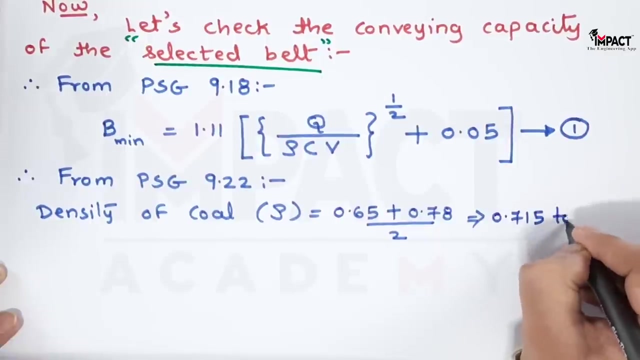 from PSG 9.22. as we can see here, and this is the density. the unit is ton per meter cube. so the density value of coal is it is between 0.65 to 0.78, so we can take the average value. so therefore density would become average of the two values, which is 0.715 ton per meter. 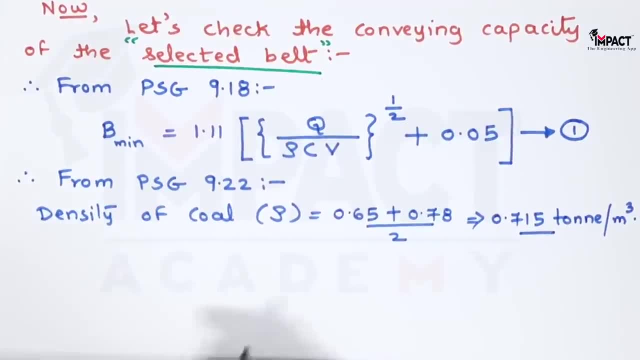 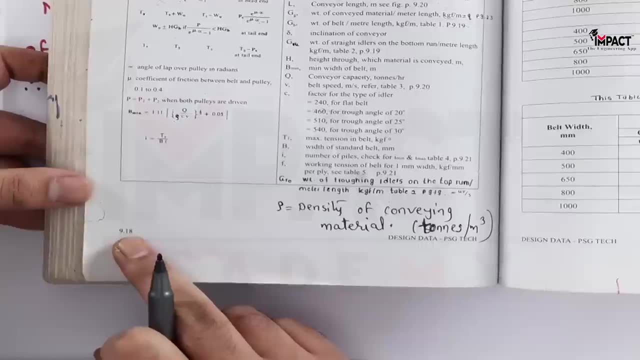 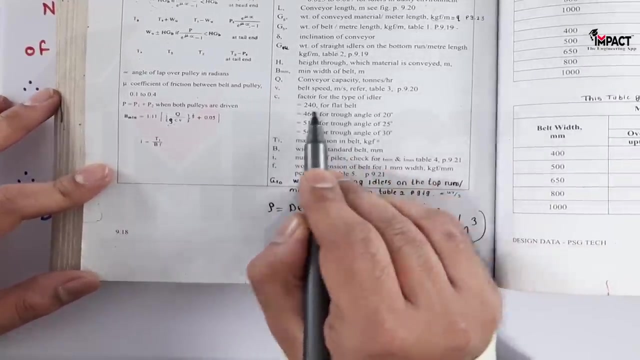 cube. so that's the density of the conveyed material. next, the value of C. now, C is there on page number 9.12. 18 of the PSG book, and here is C. it is the factor for the type of idler, and the value is 240 for flat belt. since we don't have flat belt here, we have a trapping angle of 20 degree. 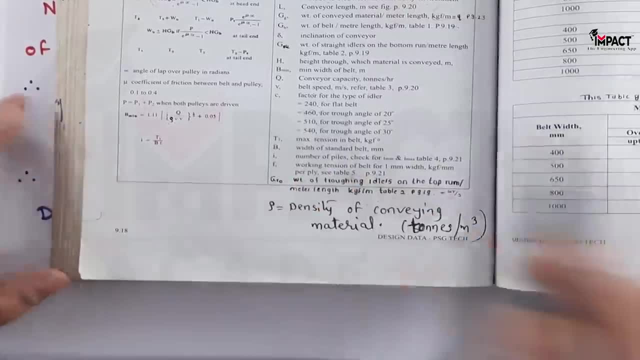 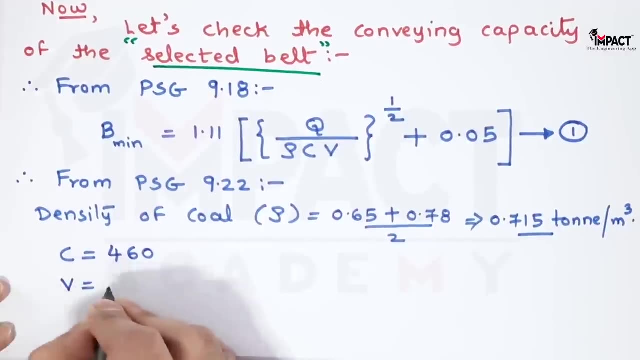 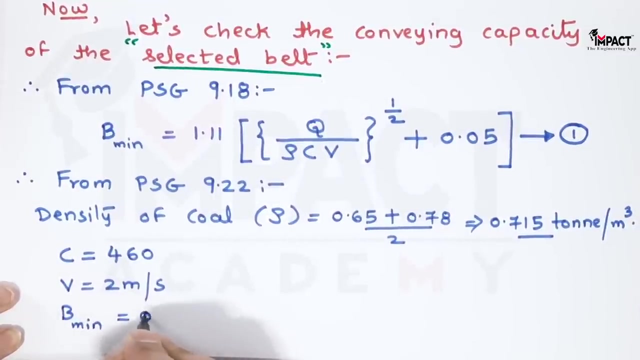 so for that the C value is 460, so I am taking the value as 460. then the velocity of the belt is already known to us: it is 2 meter per second, and then the minimum width of the belt is 0.65 meter. so therefore, putting all values in equation first, hence we have the minimum. 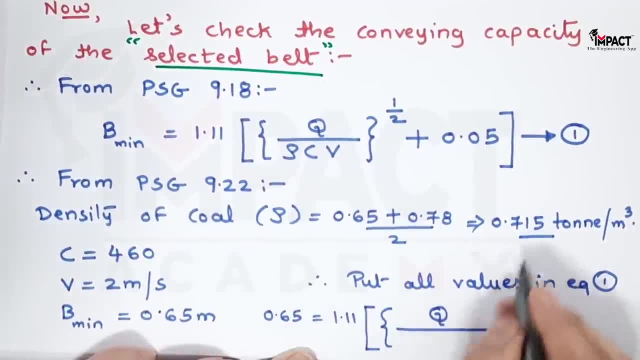 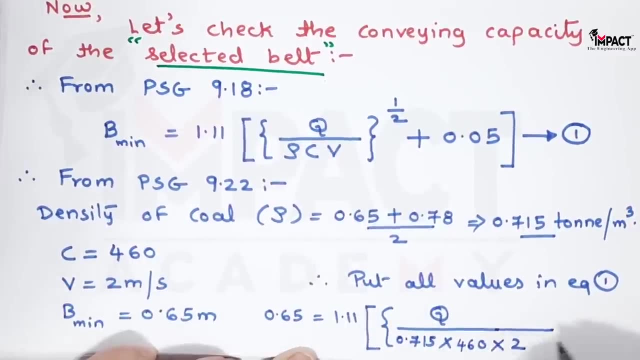 Q is what we have to calculate density. rho is 0.715, C is 460, V is 2 meter per second. raise to half, it means that is square root plus 0.05.. So we have to calculate the density of the belt. 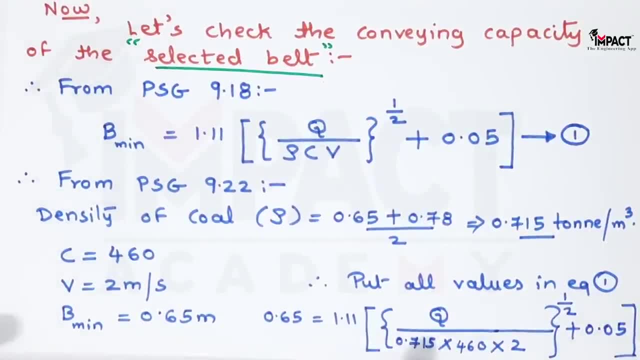 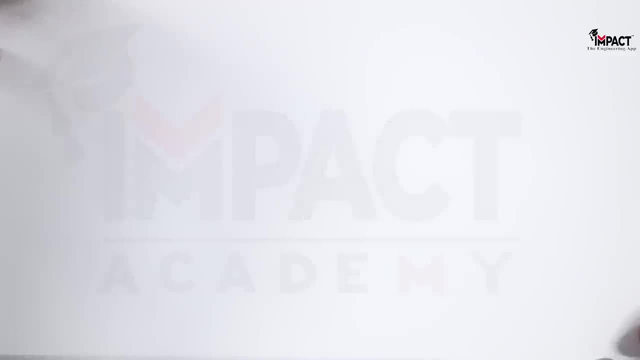 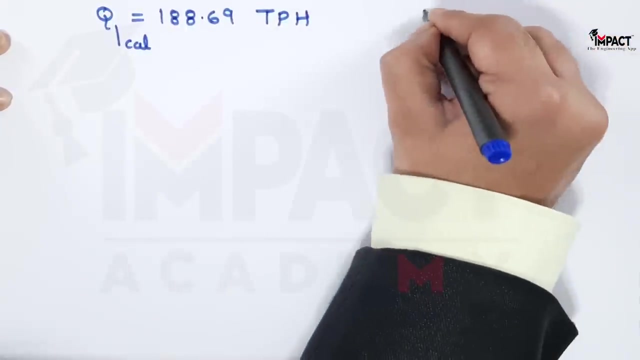 So we have to calculate the density of the belt. So from this I can get the value of Q, which is the carrying capacity of the belt in terms of tons per hour, and the answer this: 188.69 tons per hour. Now this value is the calculated value of Q and the required is required value is 200. 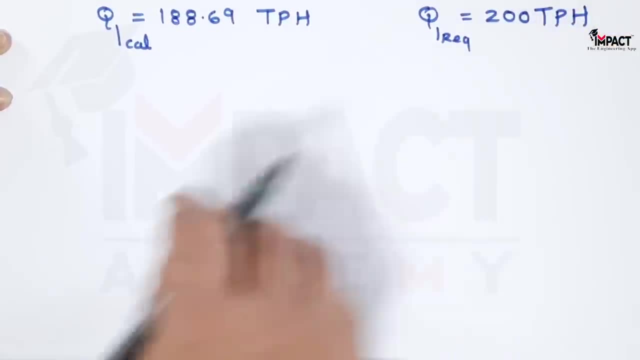 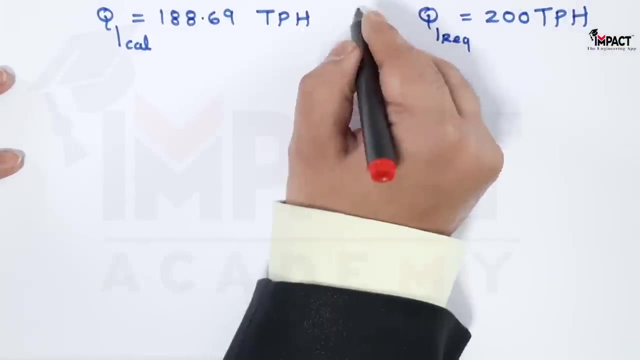 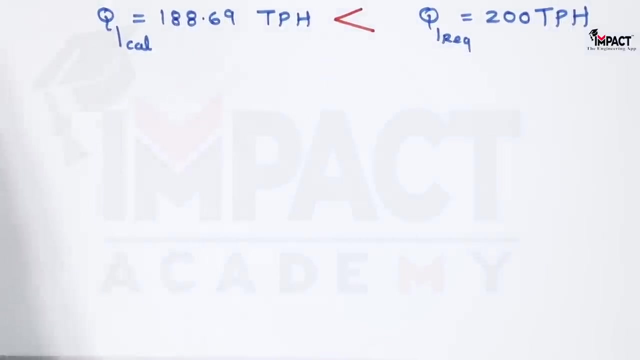 tons per hour, as per the data given. So we can clearly see that the calculated value is less than the capacity to be transferred. So it means, therefore, the selection of belt fails. So now, selection fails. It means the belt which we have selected having with 650 mm and velocity 2 meter per second. 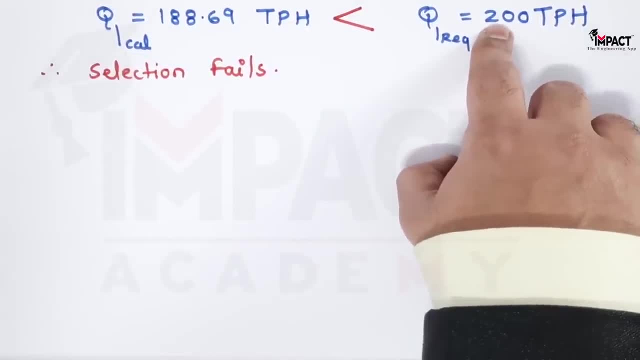 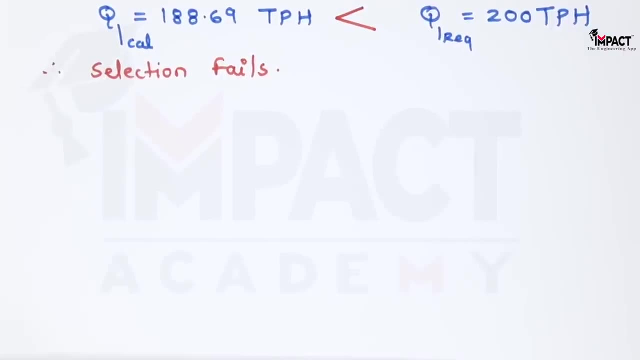 is not able to convey the required quantity, that is, 200 tons per hour, as we can see here. So the selection is failing. Now, once the selection fails, we have to go on, means the problem would not stop here. We have to go for the next criteria, and that is. 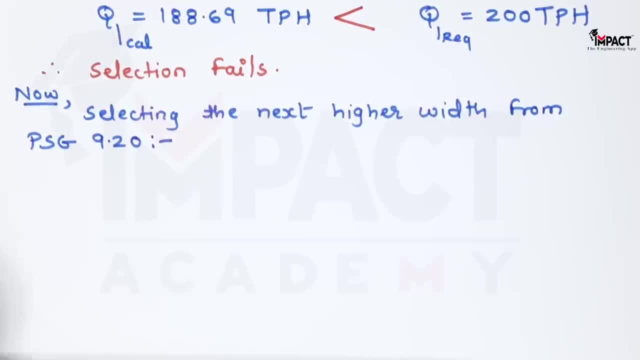 So we have to select the next higher width, like previously it was 650, so we have to increase the width. And again going back to PLC, PSG 9.20, from where we had selected the width on PSG 9.20 instead of 650, now the next higher. 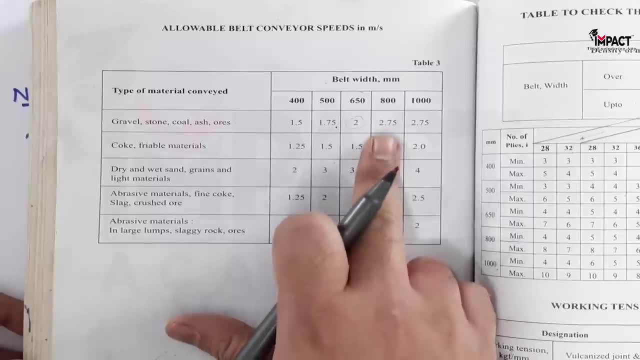 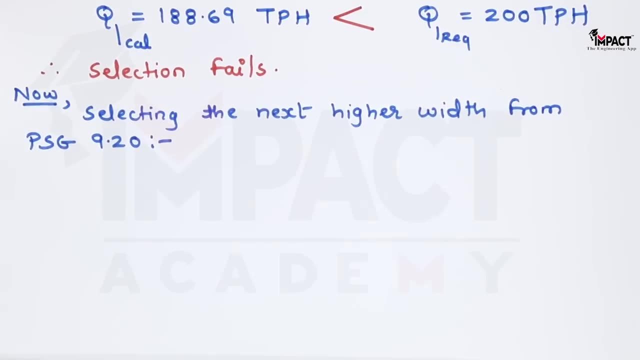 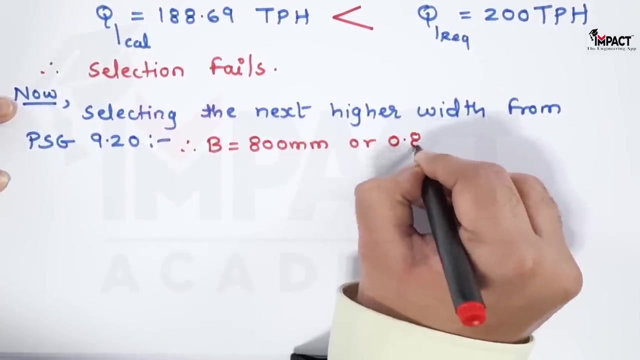 value is 800.. So I am going to select 800 mm as the width, and so the velocity will also change: from 2 it will be 2.75 Newton per meter per second. So therefore now the next new width would be 800 mm or 0.8 meter, and the new value of 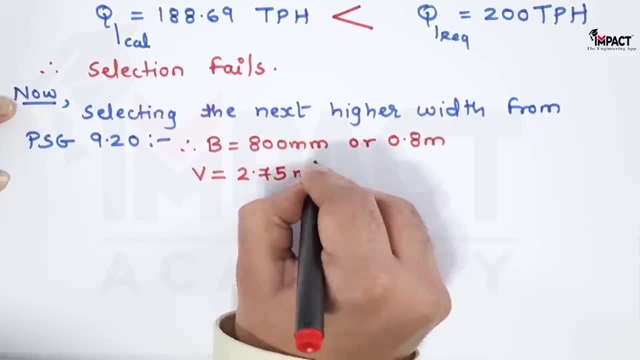 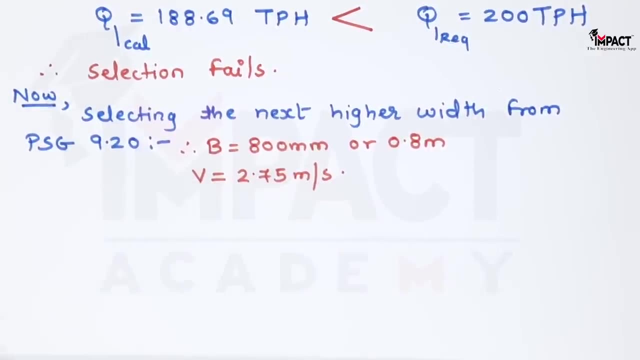 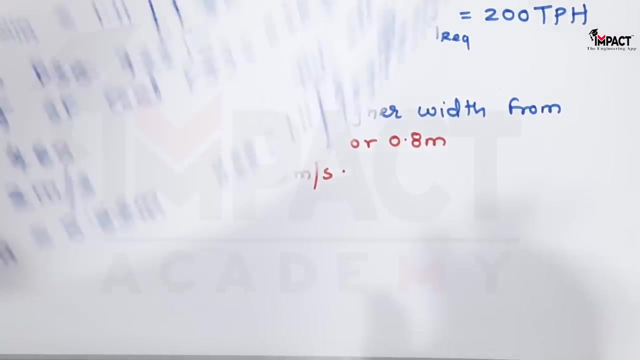 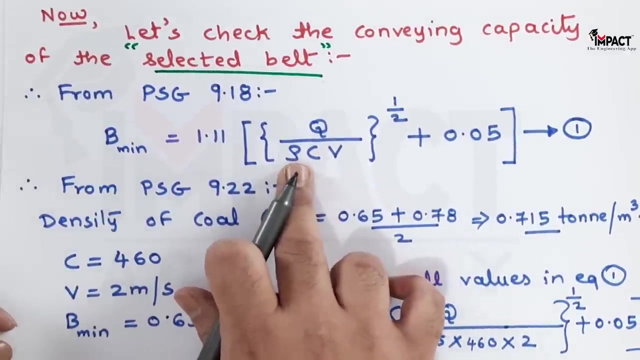 velocity will be 2.75 meter per second. Then again, for these two values, we have to check the carrying capacity of the belt. So, again using the same formula, like in equation 1.. The width would change, C value density will remain as it is and the velocity is going. 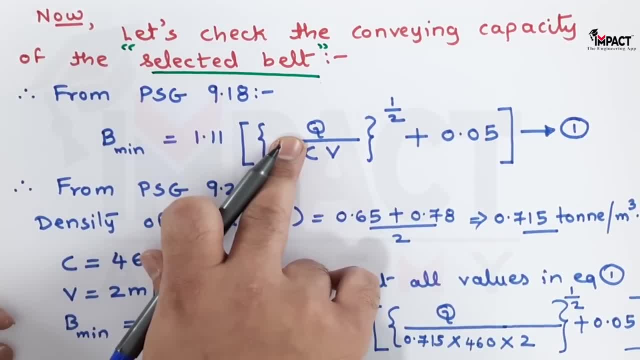 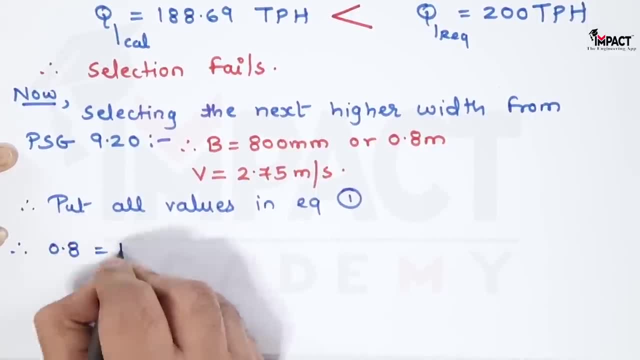 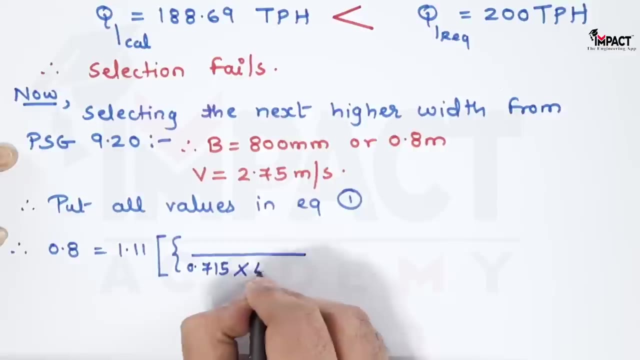 to change. So I am putting all the values in equation 1 to get the new value of Q. So therefore, where B minimum is 0.8 meter, density is 0.715 ton per meter. cube C value is 460 and now the velocity has changed, it is 2.75. in the numerator we have Q raise to 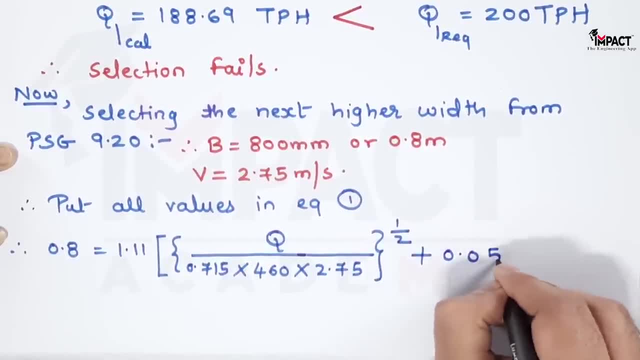 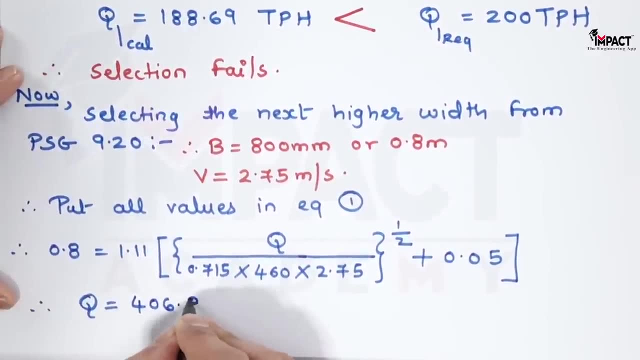 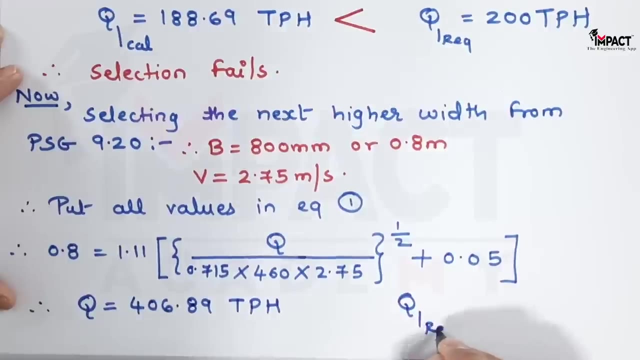 power, half plus 0.05.. So therefore, on Q, 0.75.. From calculating, the Q value will come out to be: it is 406.89 tons per hour, and again the required value is 200 tons per hour. So now, when I compare, I can say that this calculated value is way much greater, almost. 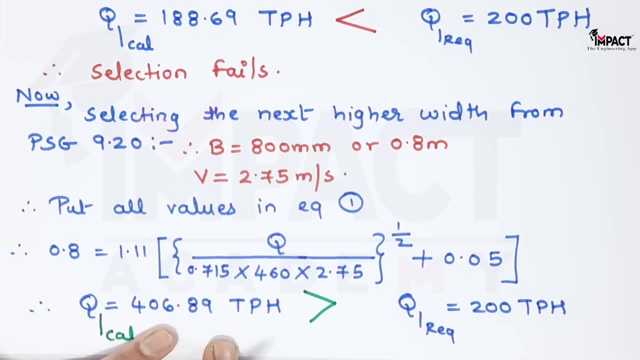 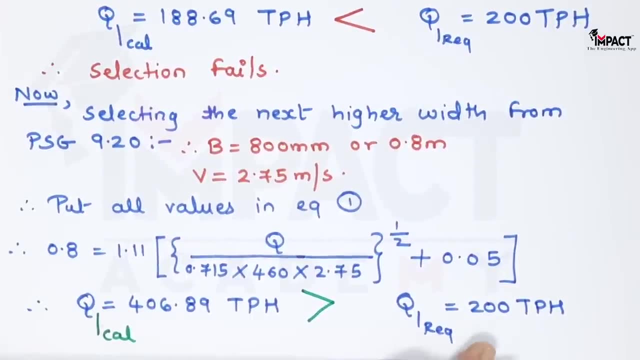 the difference is double. So The belt which has been selected now, having the width of 800 mm and the velocity of 2.75 meter per second, can transfer almost double the amount which is required. So the condition has been met. but we have to check. the velocity of this belt means if 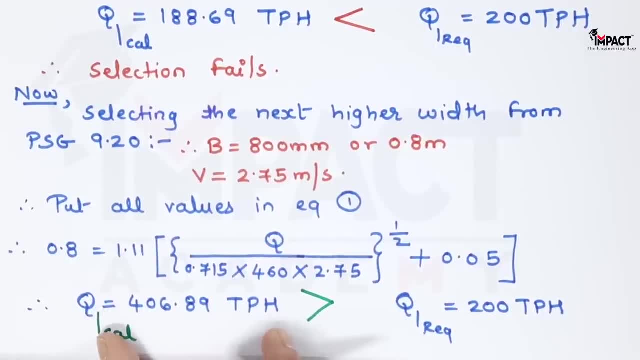 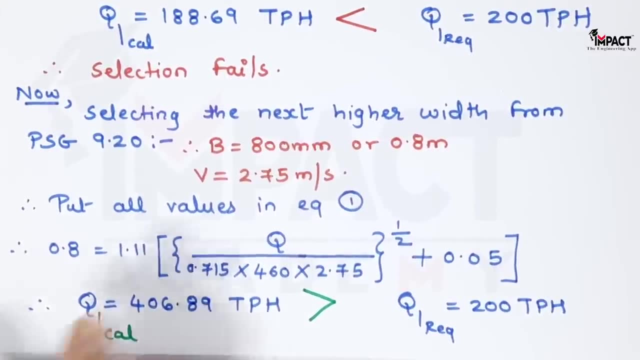 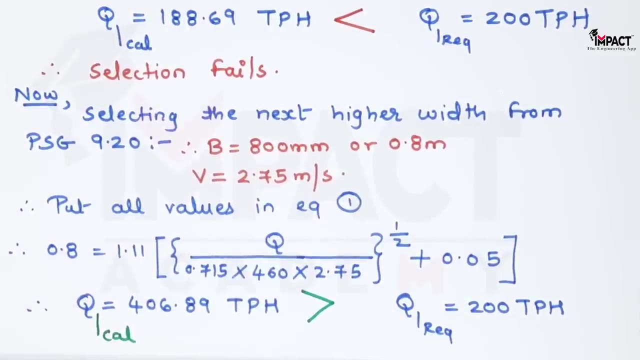 it is carrying this much amount of material, then the velocity should also be in a particular range, means the velocity should not be exceeding the value of 2.75 meter per second. then what will happen? instead of conveying the material, the material would be flying away, or we can. 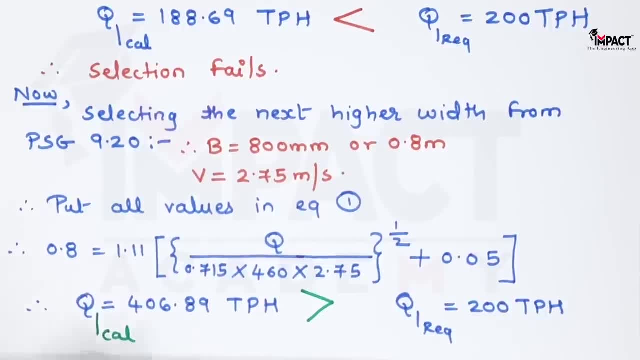 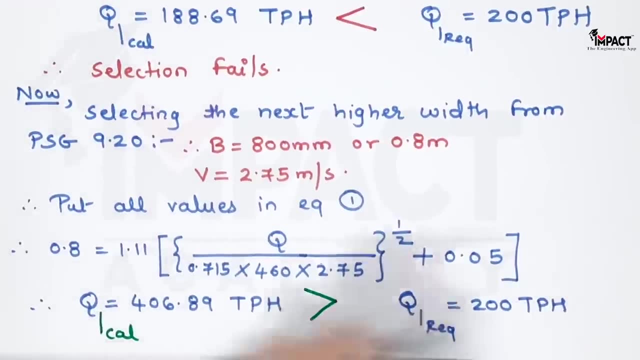 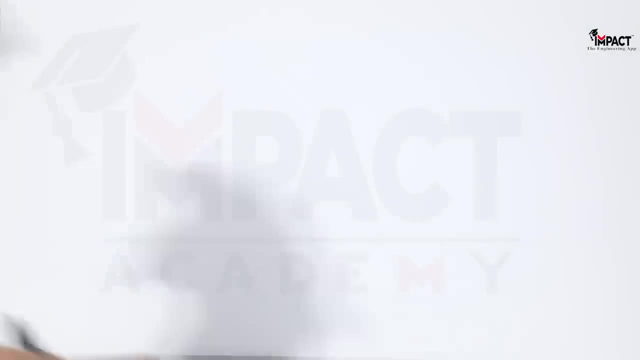 say the material would fly away from the conveyor belt at a very high velocity. so we have to check that and for that also I am using the same equation and therefore keeping the quantity as 200 tons per hour. so checking the velocity, because the material which would be falling 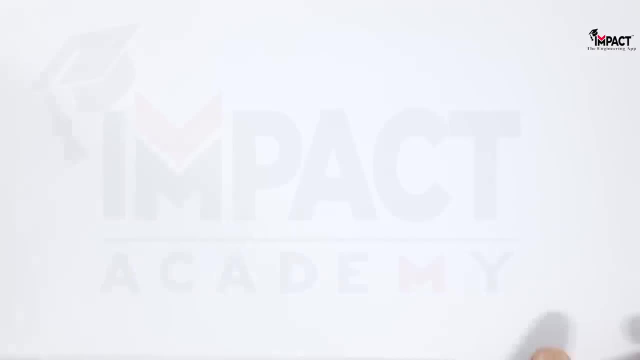 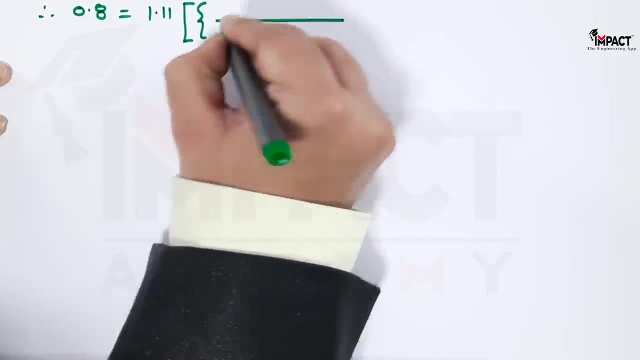 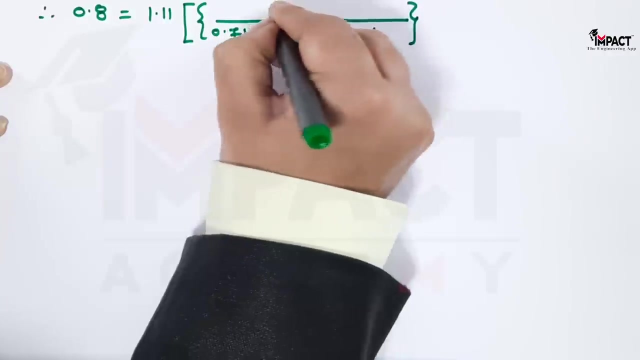 on this conveyor belt system won't be greater than 200 tons per hour, So per hour as per the requirement. So therefore, the belt width is same. density, C value, velocity is what we have to find out- and Q value is 200 tons per hour, because that is. 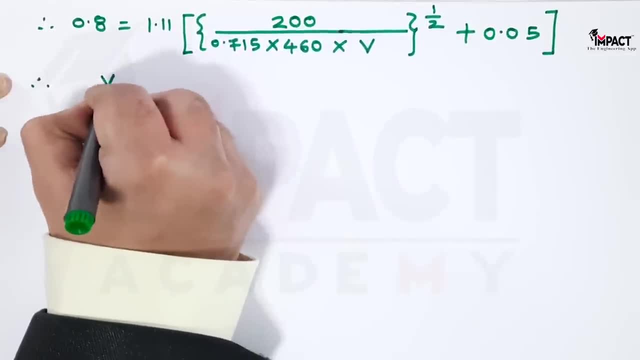 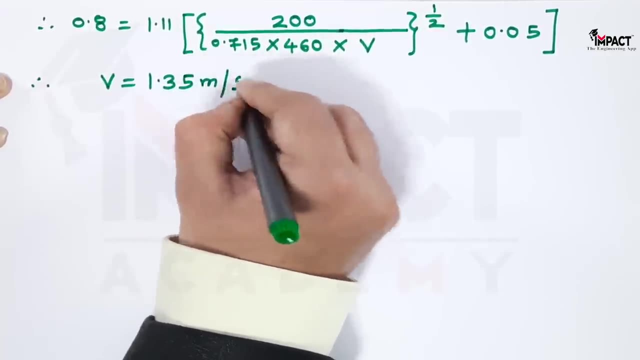 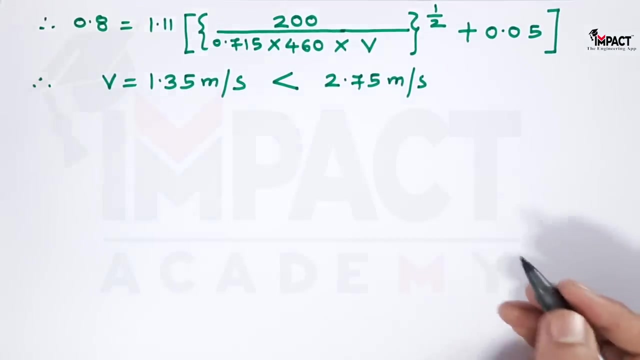 required. So therefore, on calculating this, the velocity comes out to be 1.35 meter per second, And since this value is much less than the design value, which is 2.75 meter per second, it means now this belt can easily convey the required quantity of coal, which 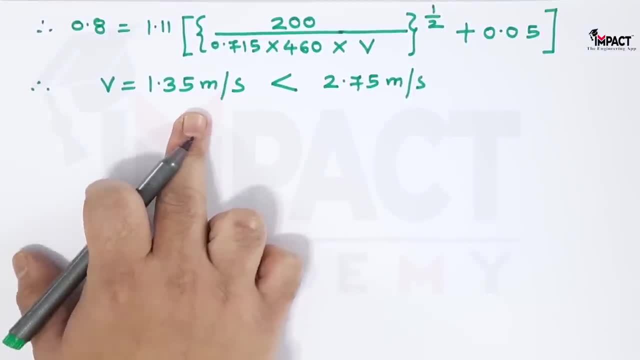 is 200 tons per hour at a velocity of 1.35 meter per second, which is less than the velocity which we have designed. If this value of velocity would have been greater than 2.75,, then again the belt would have been failing. So we have to go for the next higher. 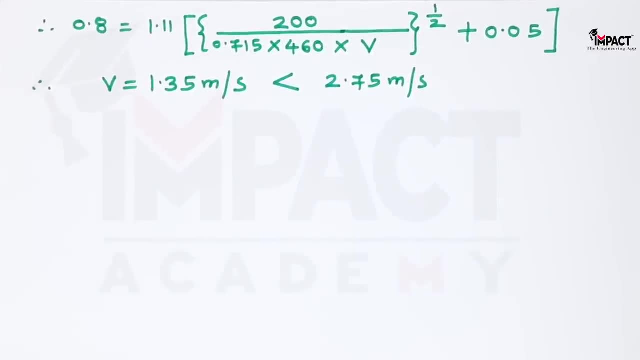 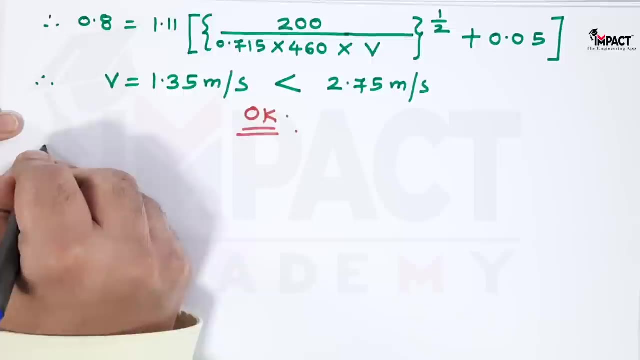 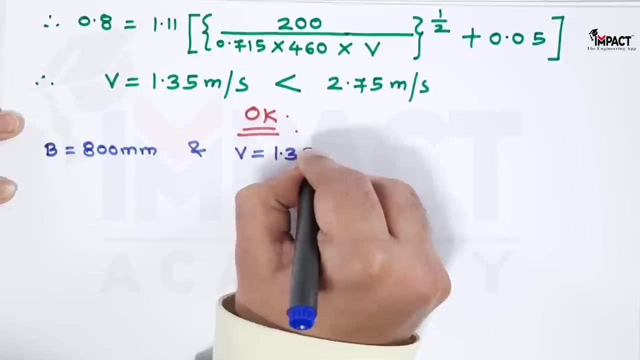 So now, in this case the selection is okay And therefore the final width and velocity would be belt width as 800 mm and the velocity of the belt is 1.35 meter per second. Now, if suppose the lump size is not given, here I am writing an important hint. So 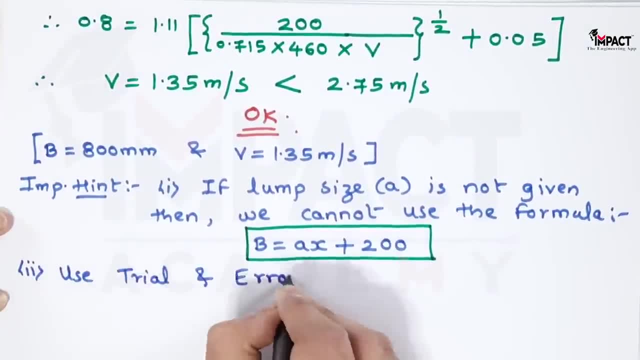 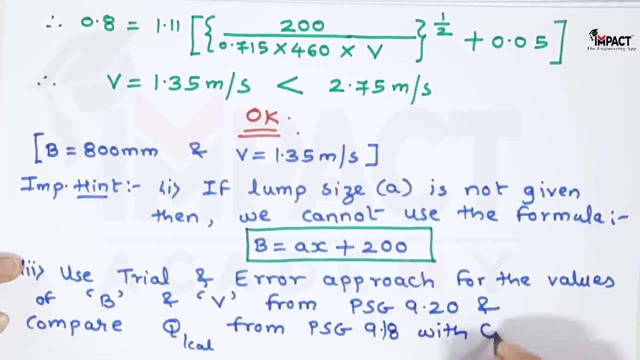 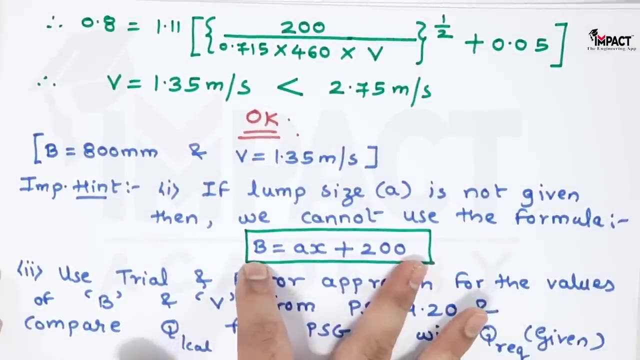 here I have written an important hint- that if the lump size A is not given, then we directly cannot use this formula of width. In that case we have to use the trial and error method, In that from PSG- 9.20, we have to select the value of width and the velocity and then 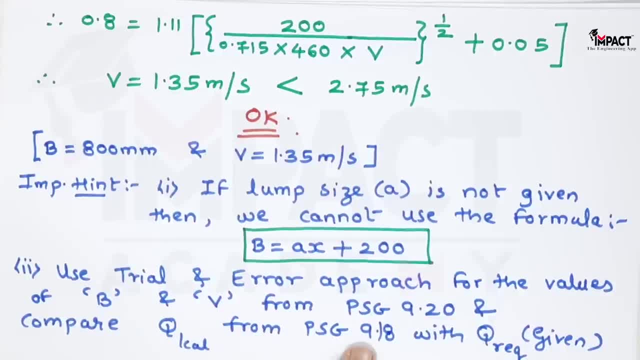 by applying the values it can be calculated. So the value of this value is basically 0, we have to basically calculate the value of the length and the velocity. So the value, again using the formula from PSG 9.18, we have to find out the amount of material being conveyed. 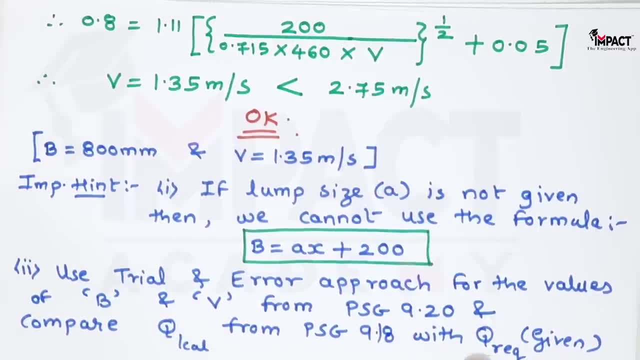 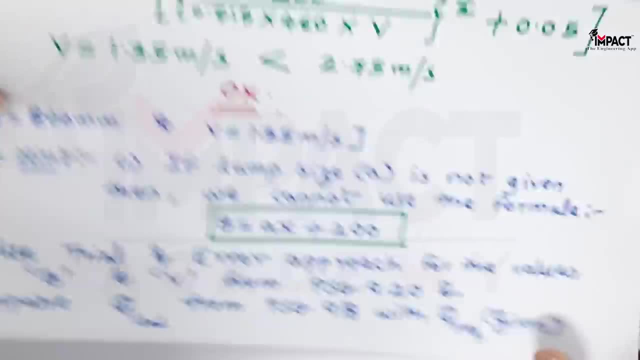 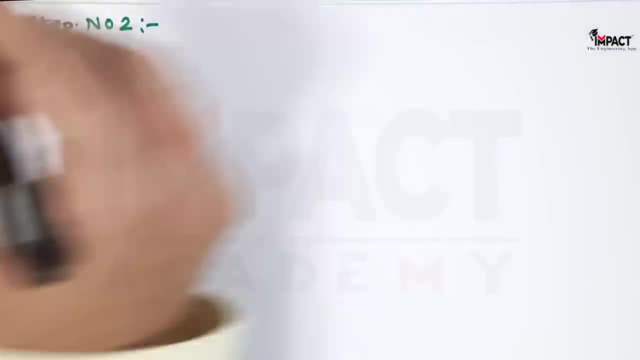 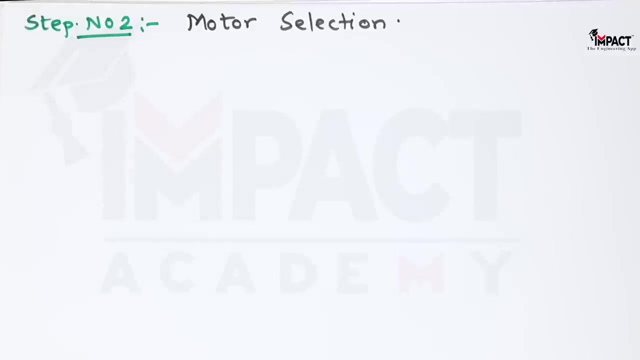 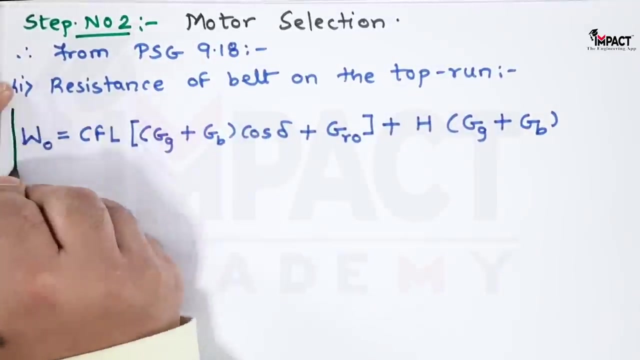 that is, that will be Q calculated, and we have to compare it with the Q required which is given in the data. so that is the method which we have to use now. step number one is completed. next is step number second, which is the motor selection. now for motor selection. first we have to reach on PSG 9.18 again. so therefore, 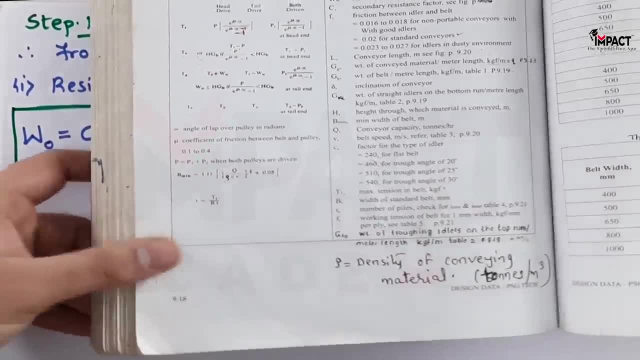 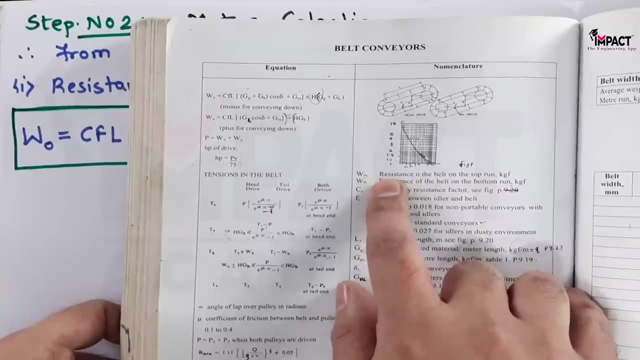 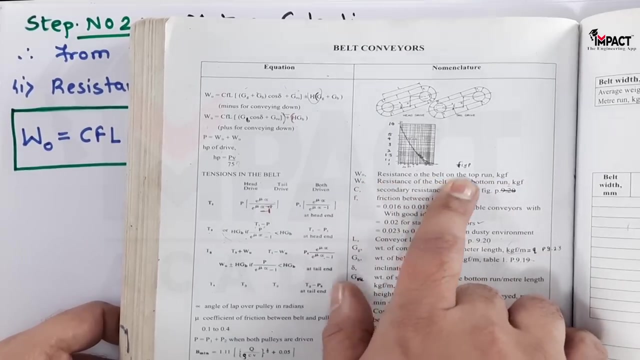 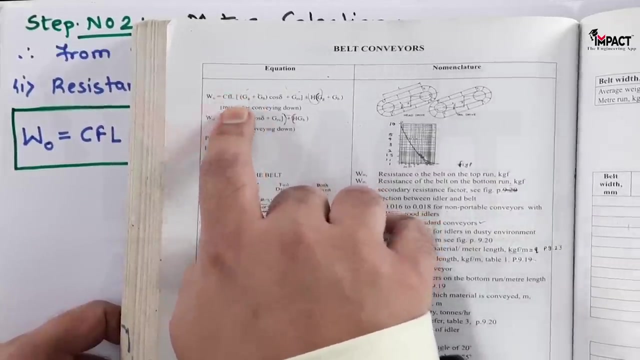 so, on PSG, 9.18, at the top we have the first formula, which is WO. now what is this? WO is given over here? it is the resistance on the of the belt, on the top run. the unit is KGF, so that is the force which is acting on the top of the belt. the formula is EFL, G suffix into bracket. 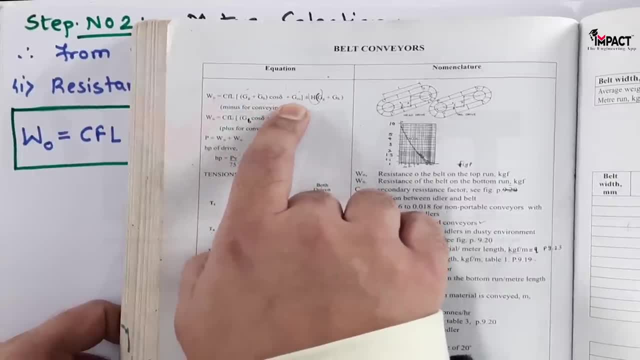 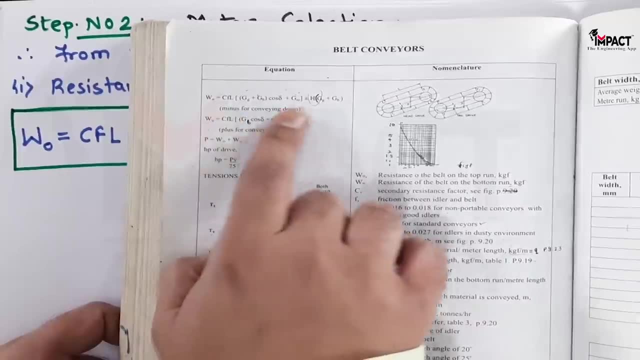 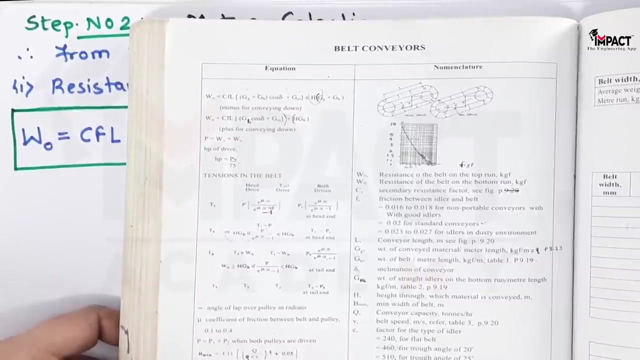 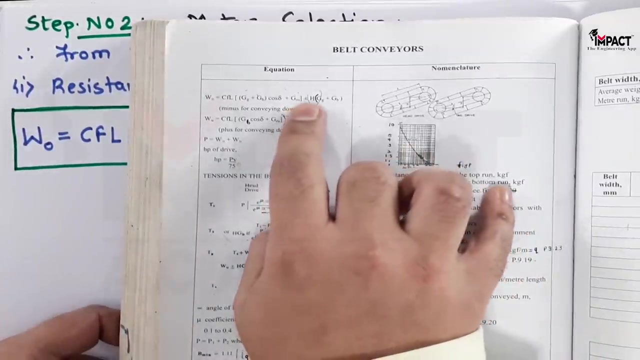 G suffix G plus G suffix B, cos, delta plus GRO, plus or minus. now this plus or minus will depend upon the conveying direction we have to take negative, that is minus for conveying down. in this case, in this problem, nothing is mentioned. whenever nothing is given, we have to always take the direction as conveying up. so if it is conveying, 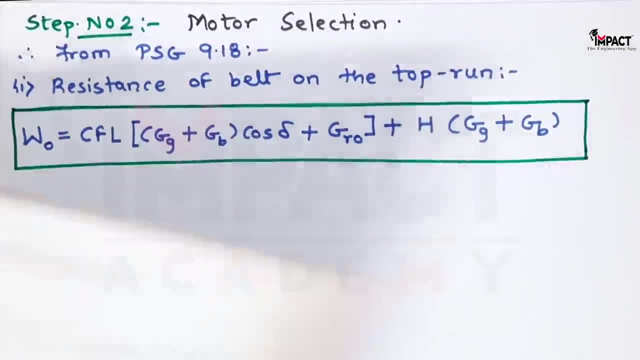 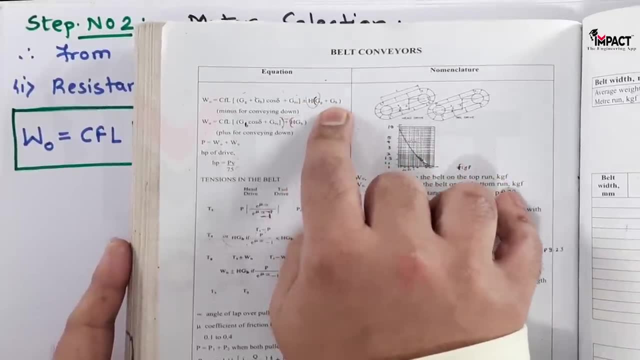 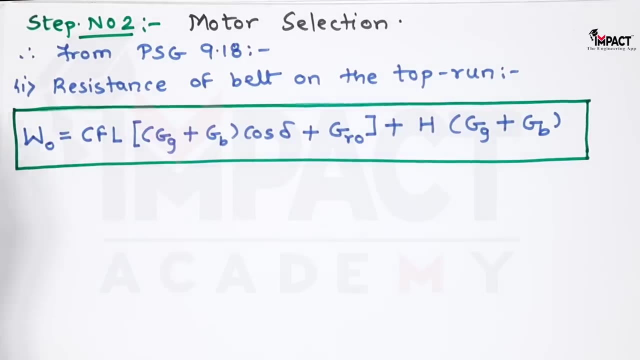 up. we have to take the positive sign in the formula. so here I have written the positive sign. then it is H into G suffix G, and then it is G suffix B. So let's start by calculating each of the values. first of all the value of C, now this: 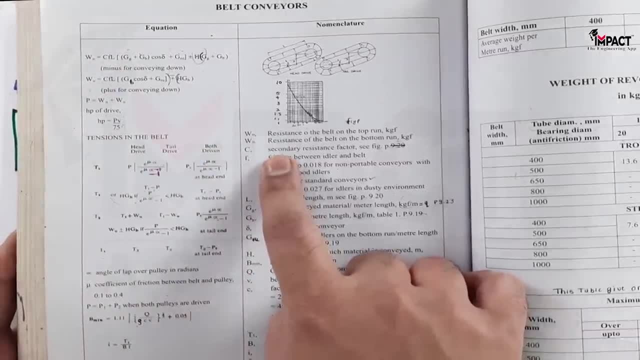 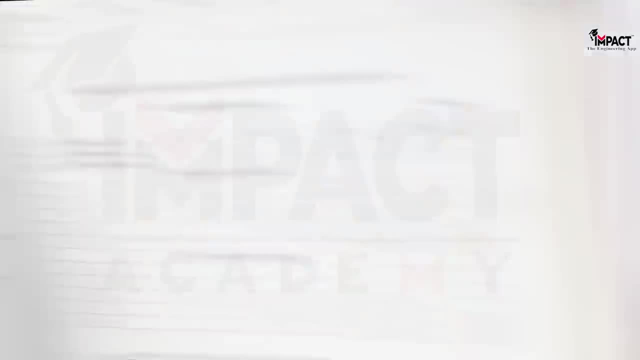 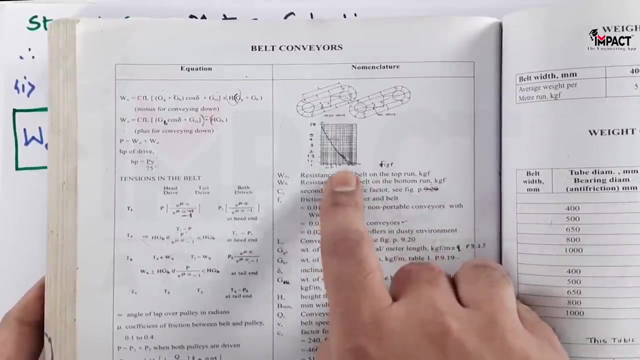 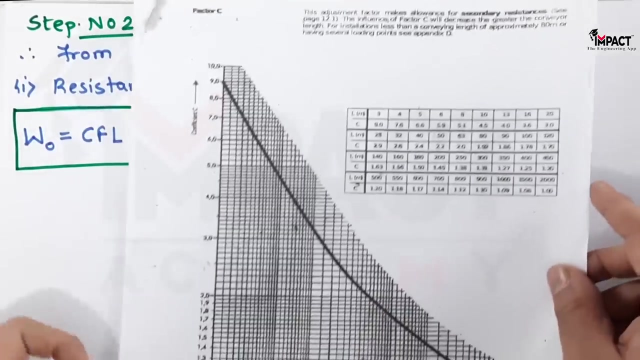 capital. C is given over. here it is the secondary resistance factor. and how to get that secondary resistance factor? for that, here there is a graph on this: PSG 9.18,. now from this graph we can get the value of C, and I have it on the enlarged scale. so I will explain it here. 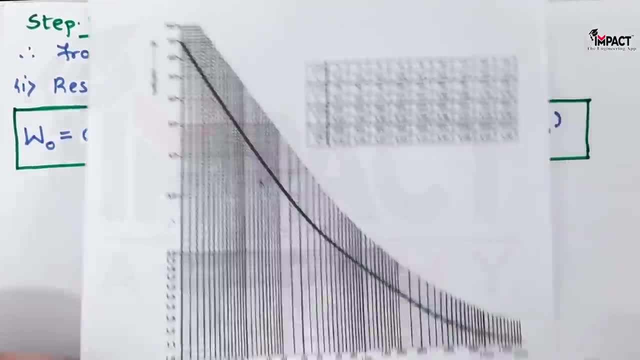 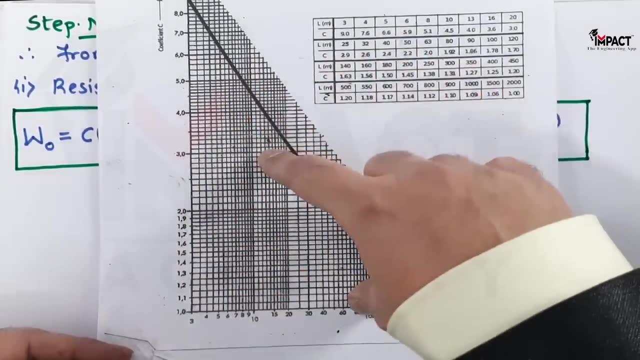 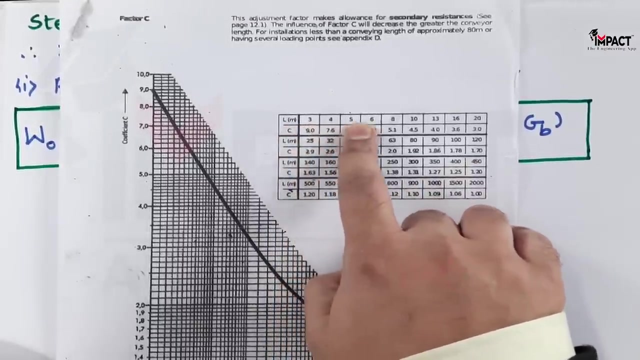 on this graph we have the coefficient C versus the length of the belt, which is the conveying length, and whatever the data is there on this graph is being tabulated over here. so in this table the length of the belt are given starting from 3 meter and in our case the 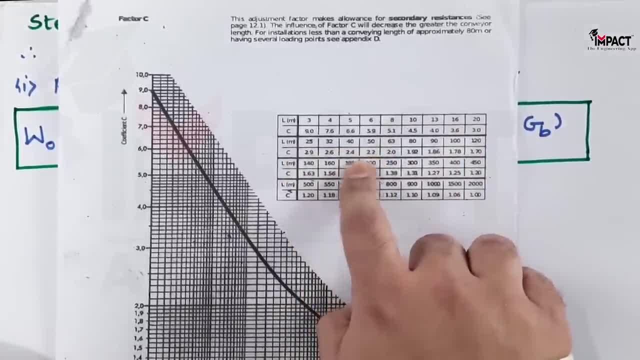 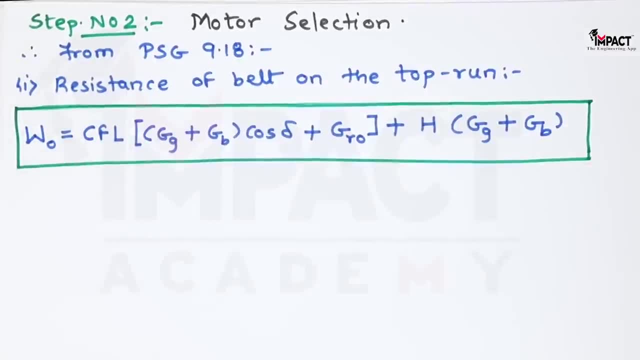 length is 50. So for 50 meter length here the C value is 2.2, as we can see here for 50 meter length. so C value is 2.2 and I am keeping it as the second equation. C is 2.2, then next is the. 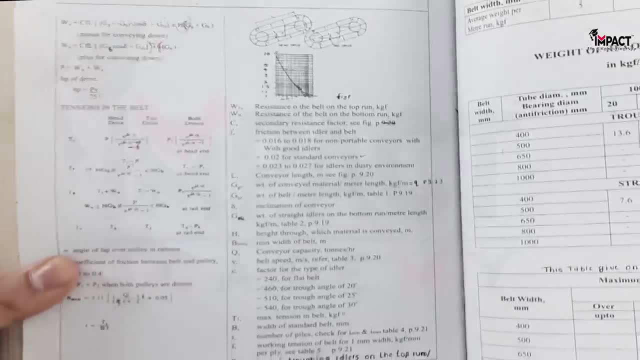 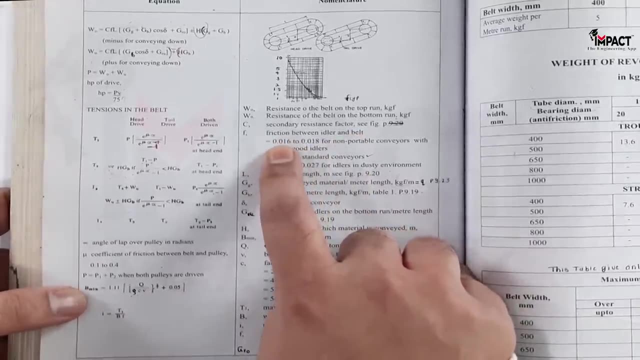 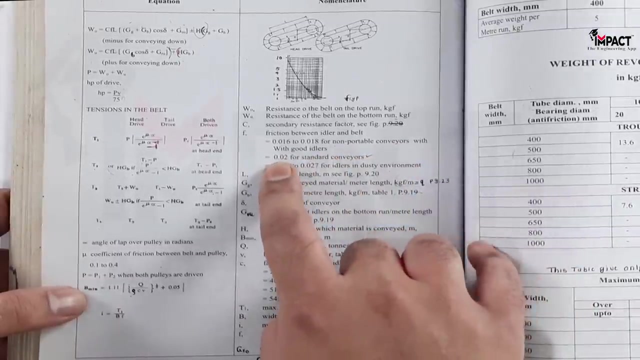 value of F. now, F is the friction between the idler and the belt, so that values are 0.01.. It is for non-portable conveyors with good idlers and the value is 0.02 for standard conveyors. 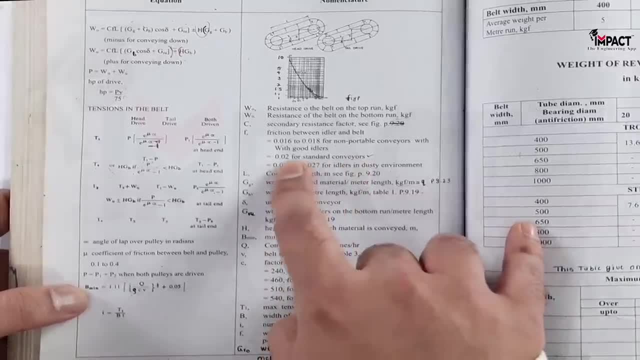 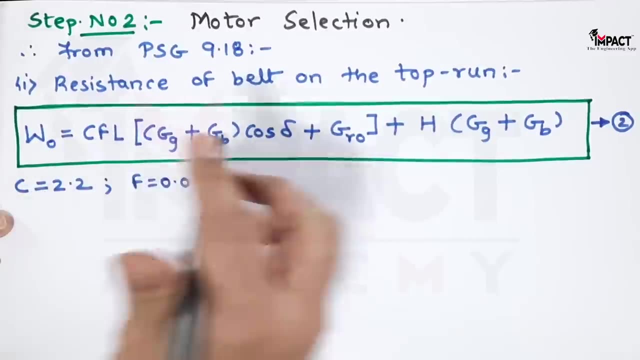 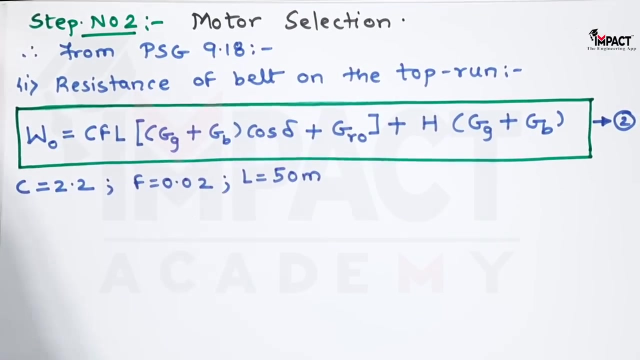 So we have to select the value, always for the standard conveyors, and it is 0.02, so that is the small f value. next, L is the length of the belt, which is 50 meters. then after that, G, suffix G. now, what is that? 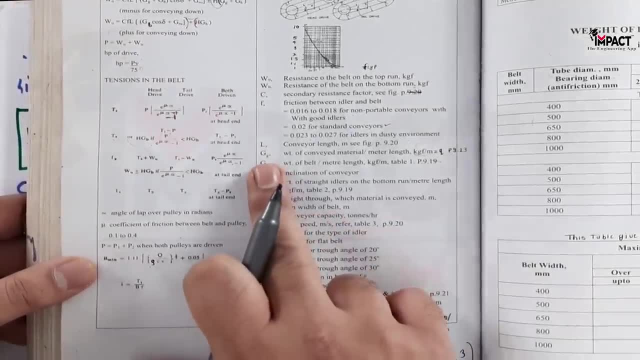 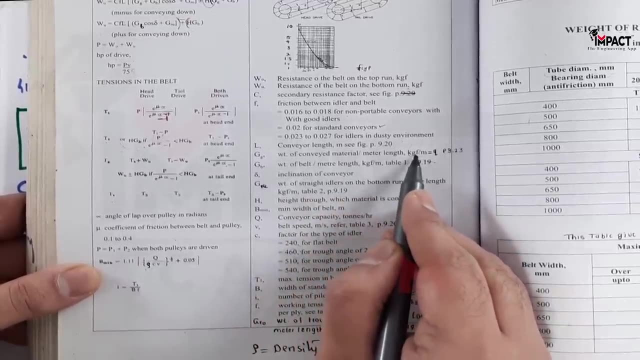 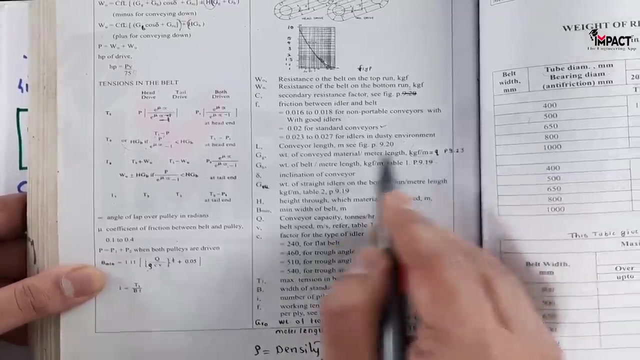 Onto this same PSG, 9.18, G, suffix G. it is specified as weight of the conveying material per meter length. the unit is kgf per meter and it is also denoted as small q. I have written here small q, so 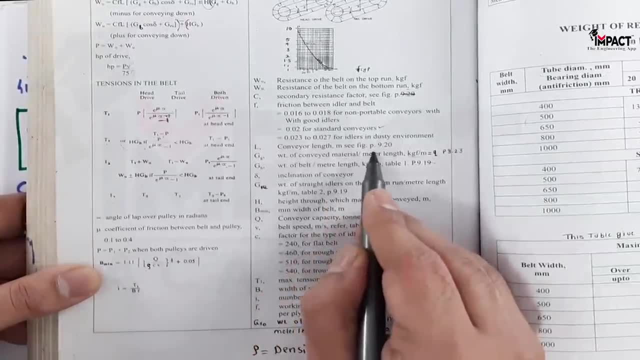 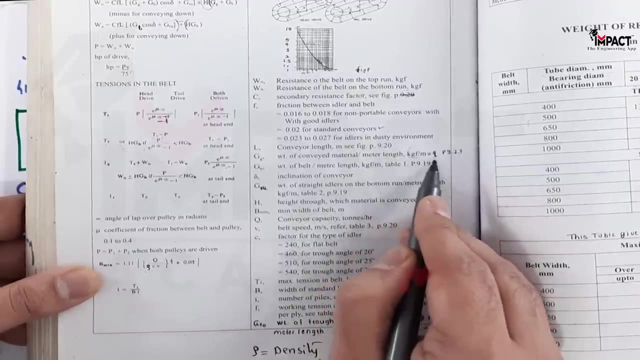 that is the weight of the conveyed material. in this case it is coal. for per meter length it means on 1 meter length of the belt, how much is the load acting of the conveyed material? so that is denoted as small q. So that is denoted as small q. 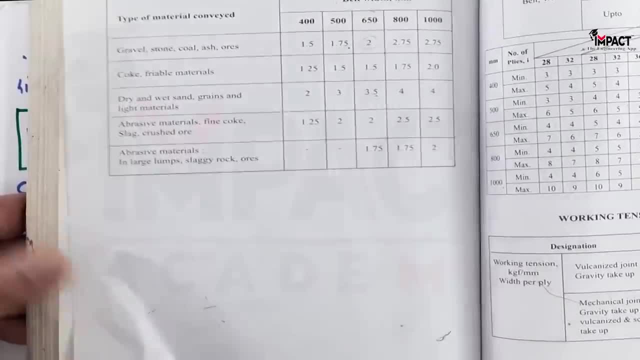 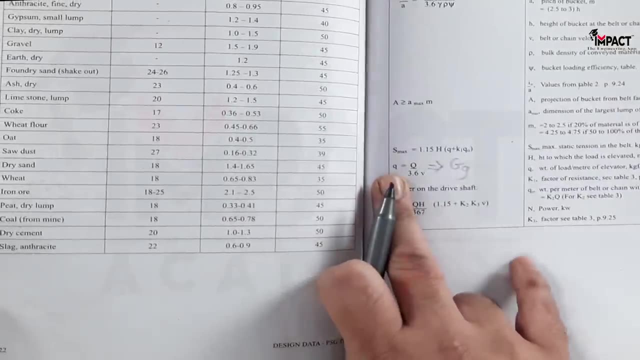 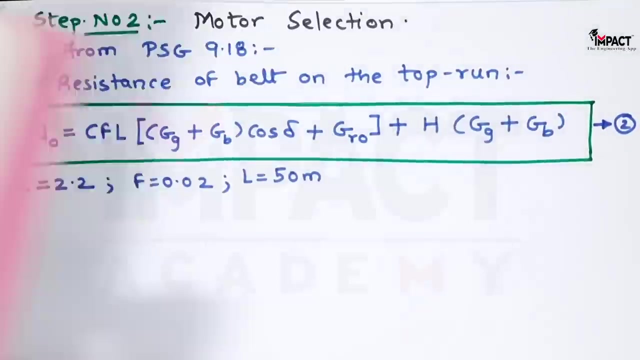 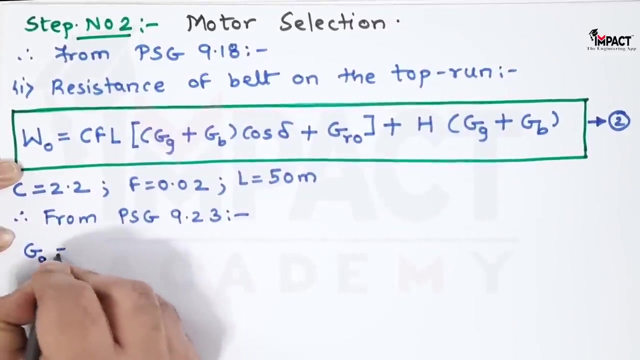 For that we have to go on PSG 9.23,. here on PSG 9.23, there is this formula of small q, which is capital Q upon 3.6 V, and that is G suffix G. So therefore, from PSG 9.23, G suffix G is equal to small q, it is capital Q upon 3.6. 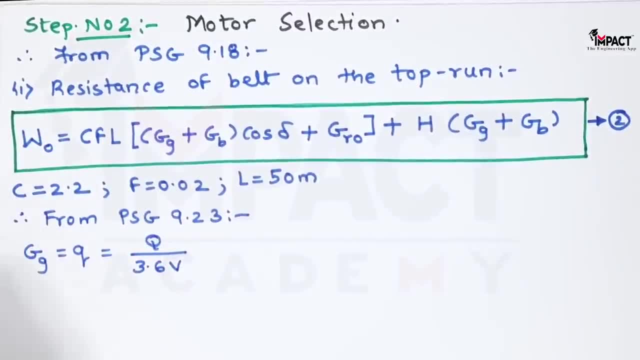 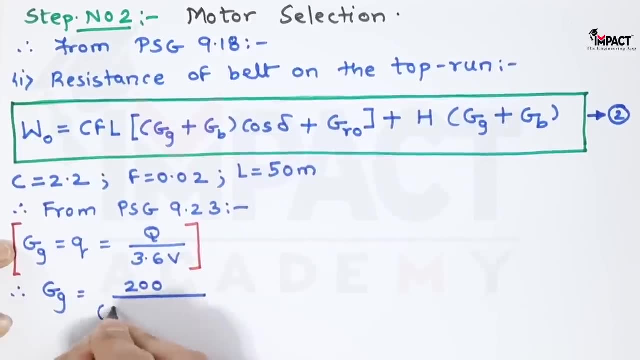 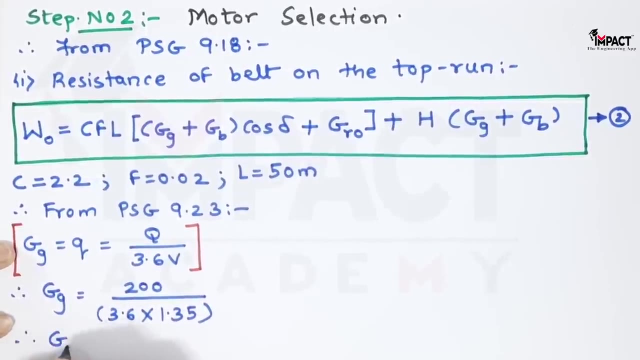 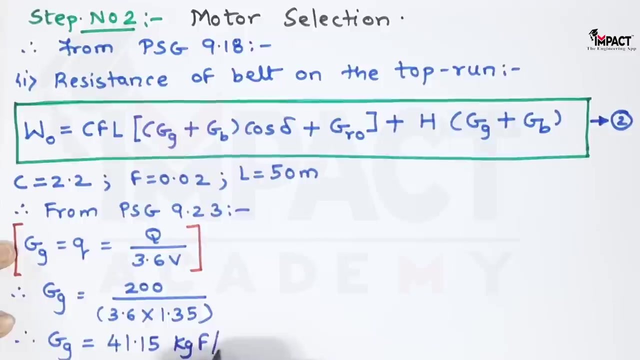 V into V, which is the velocity of the belt. Now Q is in terms of tons per hour, that is 200 tons per hour 3.6. the velocity is finalized as 1.35 meter per second. So on calculating this, the answer comes out to be 41.15.. The unit is kgf per meter, So that is the value. 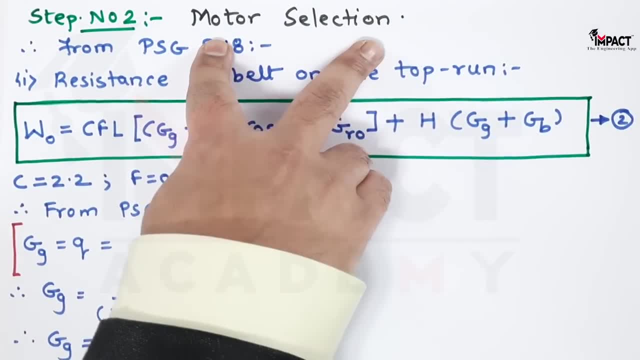 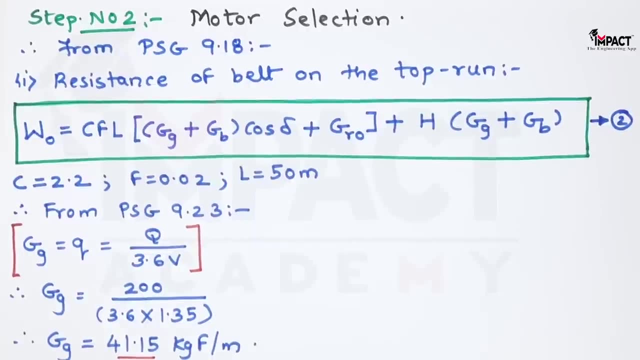 of G suffix G and remember, whatever we are doing, it is for the motor selection. It means we have to select the power as well as the RPM or the speed of the motor which would be driving the driver pulley or driver drum. Then, after G suffix G, there is G suffix B. 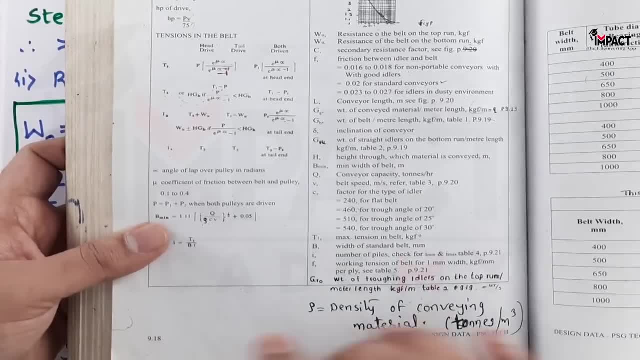 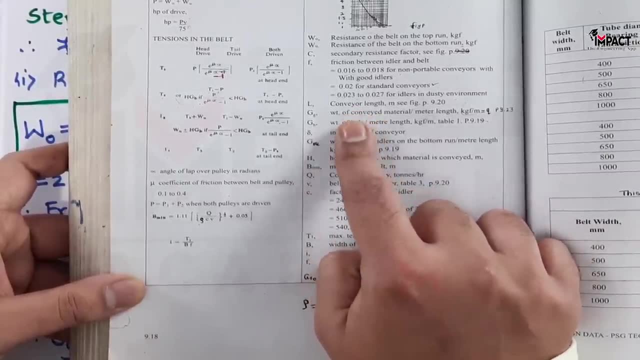 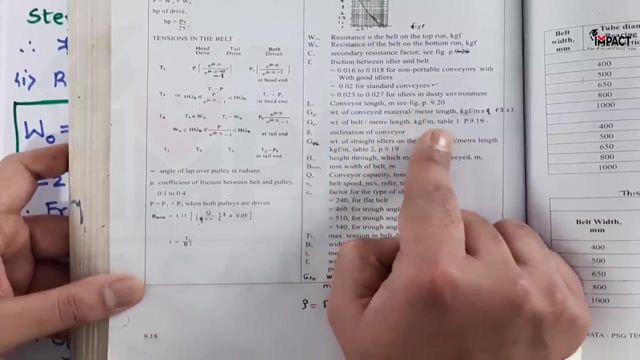 which is again on PSG 9.18, we can see G suffix B is the weight of the belt. Previously G suffix G was weight of the conveyed material. Now G suffix B is weight of the belt per meter. length. Unit is same kgf per meter and 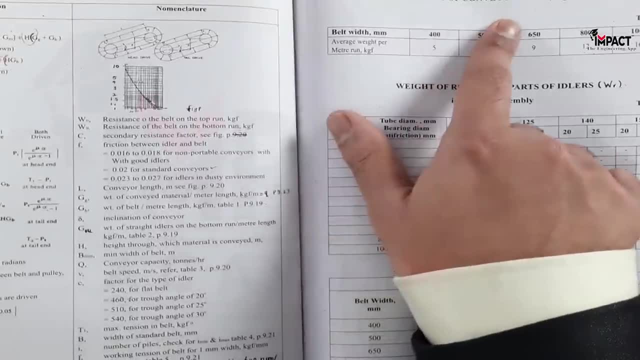 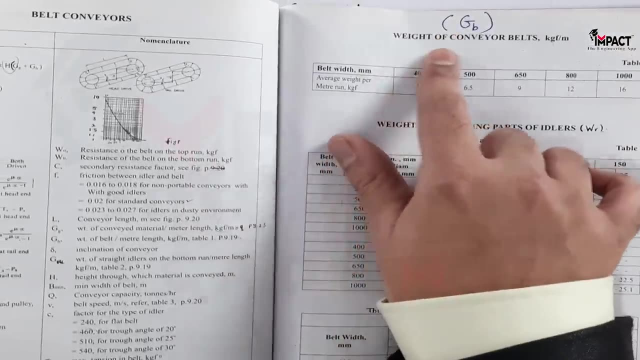 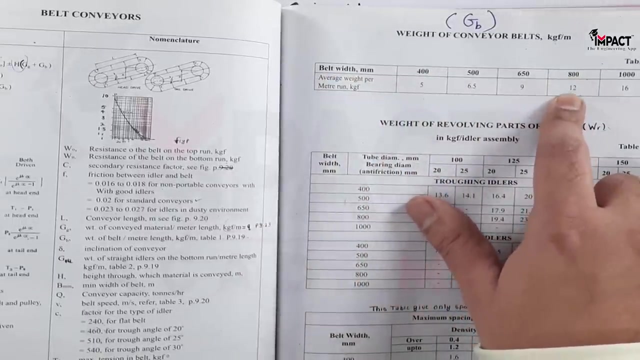 this. we can get it on the opposite page, that is, on PSG 9.19.. On PSG 9.19, G suffix B is the weight of the conveyor belt and it depends on the width of the belt. So the width selected is 800 and the value is 12 for G suffix B. So we have to take this value, 12.. Unit is: 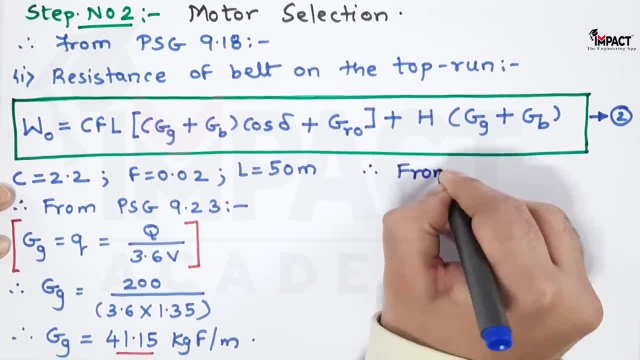 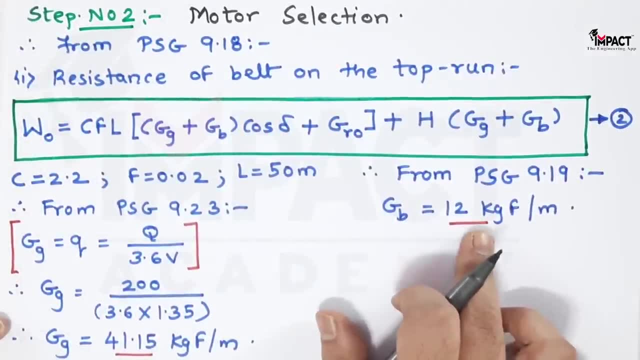 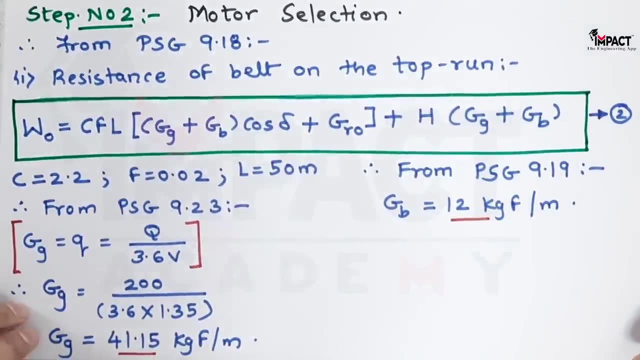 kgf per meter. So therefore it is 12 kgf per meter. So that is the weight of the belt per meter length and G suffix. G was the weight of the conveyed material on per meter length. Then after that delta, delta is the angle of the belt, given as 15 degree in the problem. So belt angle. 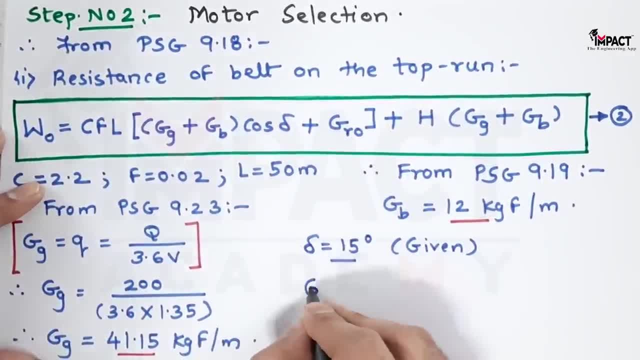 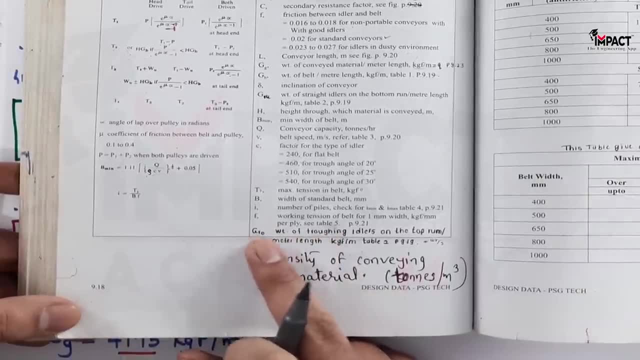 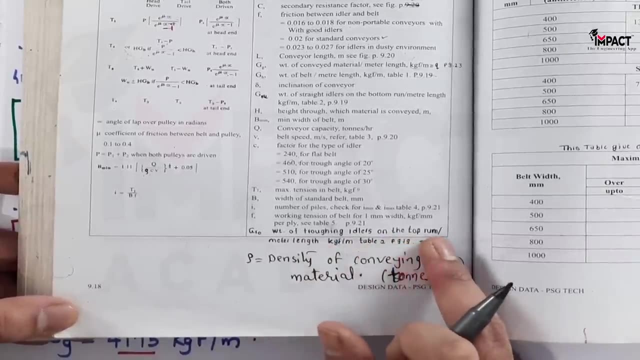 is given. Next is GRO. Now GRO is again on PSG 9.18.. Here I have written at the end: GRO is the weight of the trapping idlers on the top run, because trapping idlers are used on the top run of the belt. 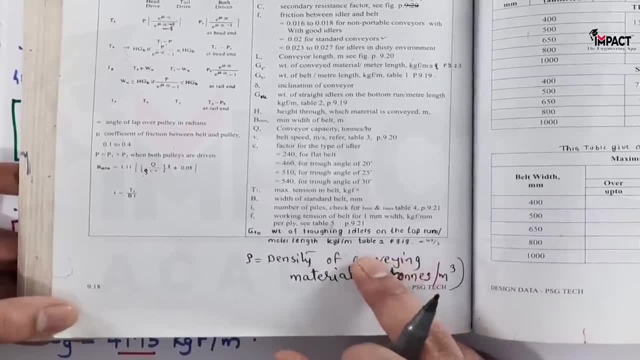 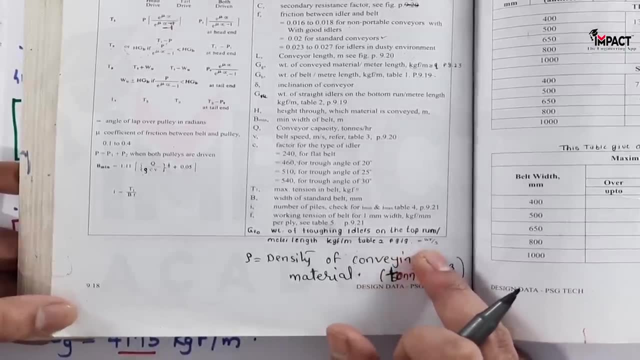 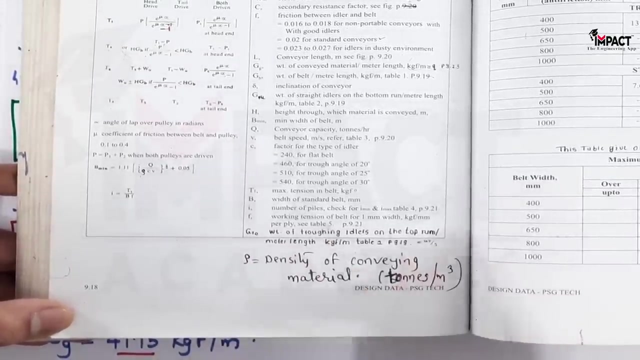 per meter length in terms of kgf per meter and it is on PSG 1.9.. The formula is WR upon S. In the older PSG this formula was not there, but I have written it. but in new PSG, in the new edition, this formula. but in new PSG we can find this formula is already given. So 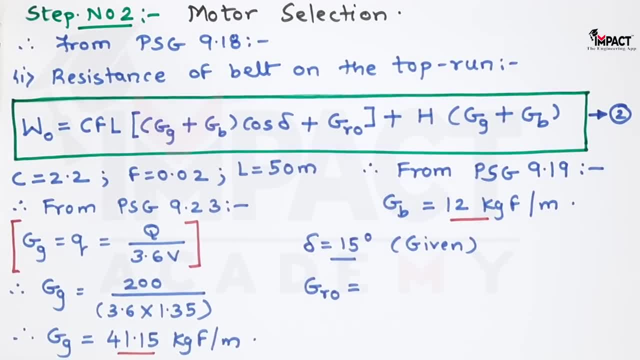 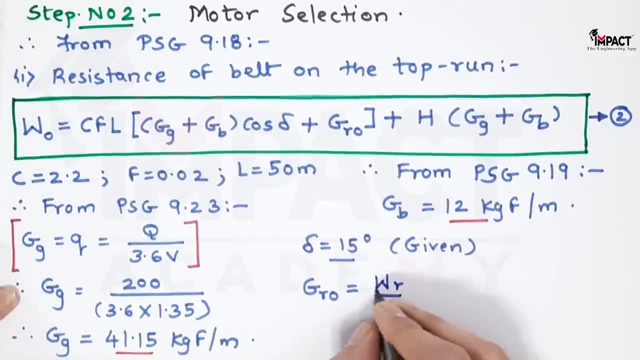 so GRO is weight of trapping idlers on the top run. So therefore, GRO is the formula: is W suffix R divided by S, which is the spacing. Next, W suffix ARE divided by S into B. Now we are seen that there is a weight of w suffix R on the top. GRO is 0.殘 of weight of the. 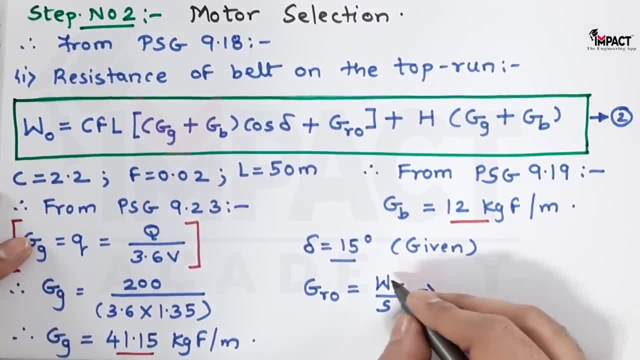 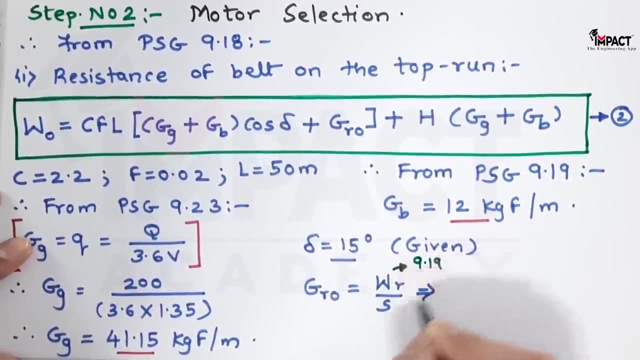 trapping idlers on the top. W suffix R divided by S over D. What is this Next? W suffix R divided by D. double suffix R divided by i. Next once, if we compare this after this: mm. weakness on these S values. they are also found in PSG 9.19 both of them and how to get the. 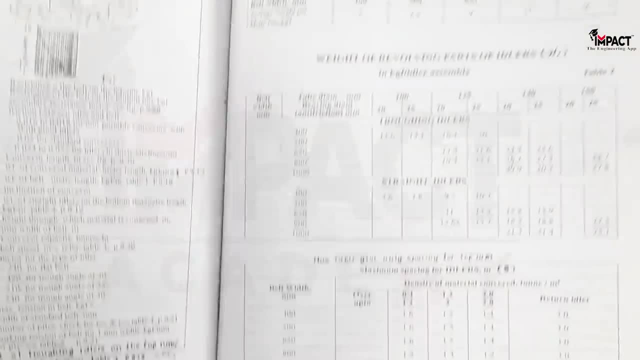 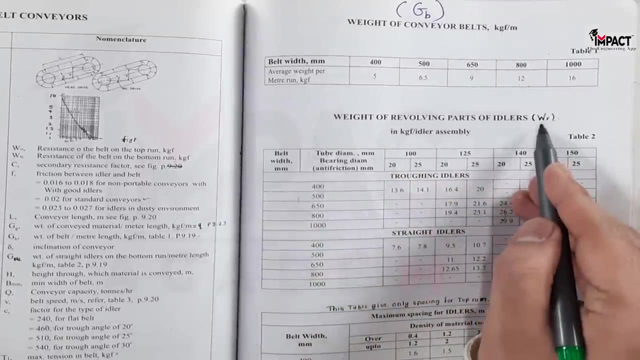 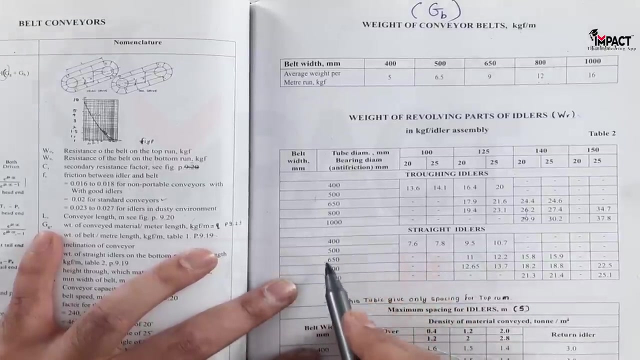 values that I'll explain. so on PSG 9.19, your weight of the revolving parts of idler W suffix R is what is required over here. on this first column we have the width of the belt. for us the width is 800, so go into this column now we can. 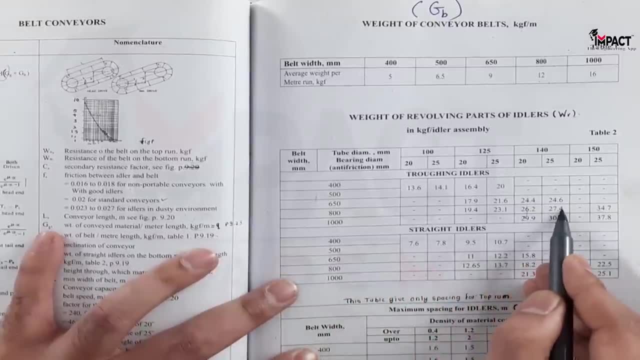 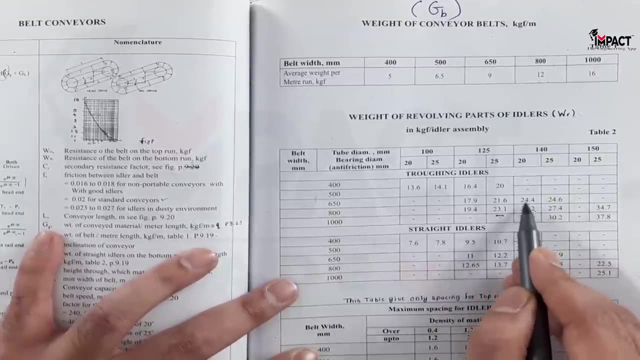 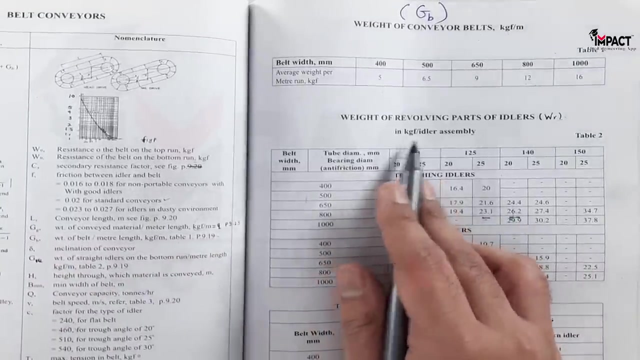 see there are 4 values. so out of these 4 values select the middle 2 values and from that select the greater value. that would give us the value of W suffix R, which is 26.2. it is the weight of the revolving parts that is weight for idler. 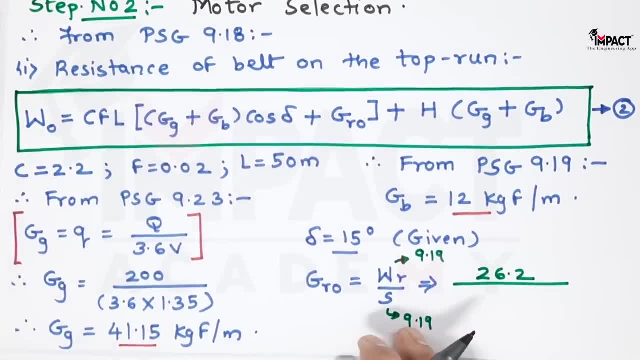 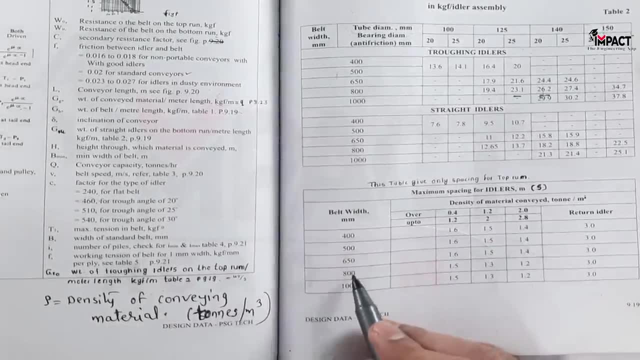 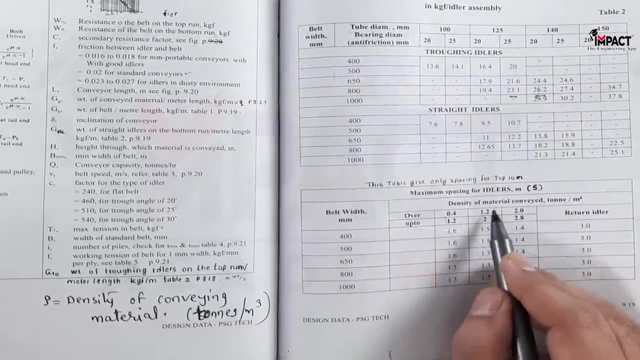 so that is 26.2. then S- see S- is the maximum spacing for the idlers on the top run. so here the width is 800 and these are the densities given. so the density of the conveyed material, that is pole for us. the density, we have already found out, it is 0.715. so 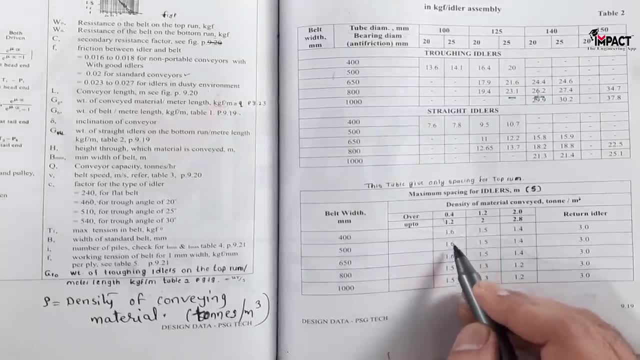 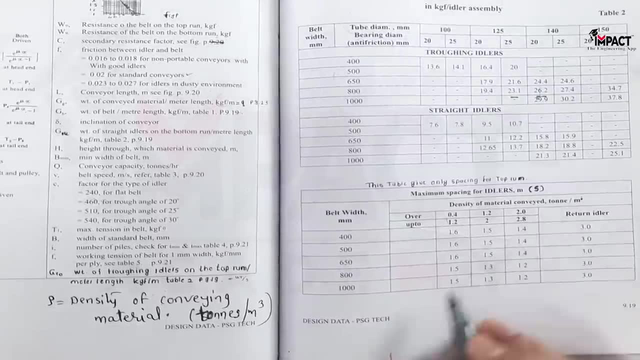 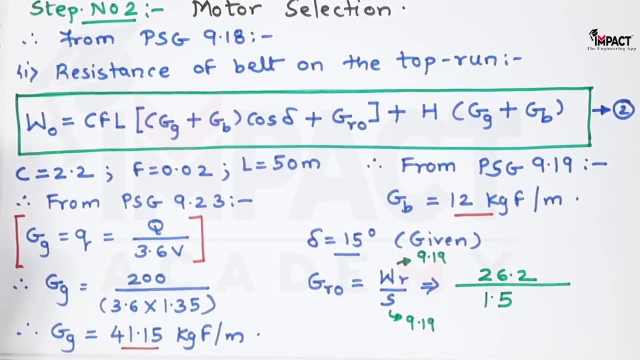 it is in the range of 0.4 to 1.2. so go into this column and at the intersection of 800, here we are getting 1.5. that is in terms of ton per meter cube. so therefore we have S value as 1.5. on calculating this, GRO comes out to be: 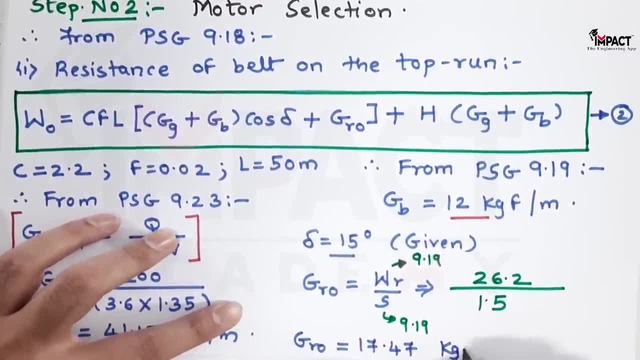 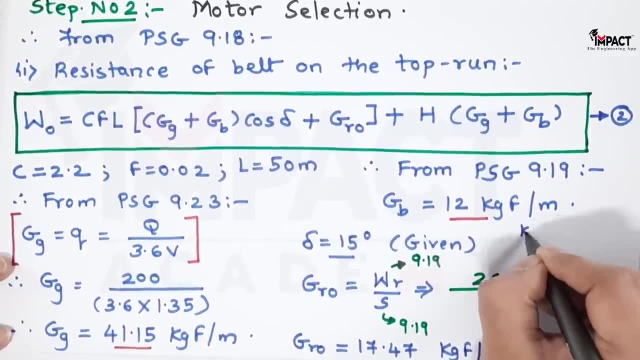 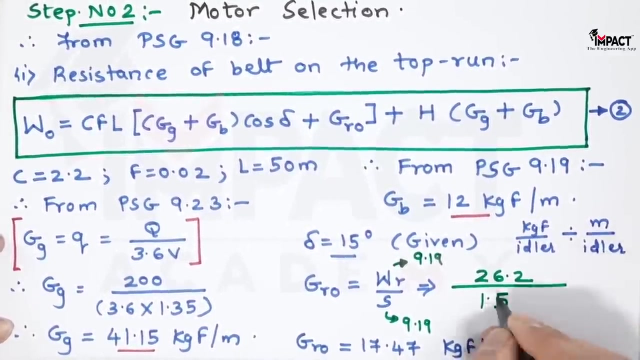 17.47. unit is kgf per meter, because WR is having a unit of kgf per idler. divided by now, S is having the unit of. it is meter per idler. that is the unit of S. so when it becomes multiplication here we are going to get reciprocal. so idler and 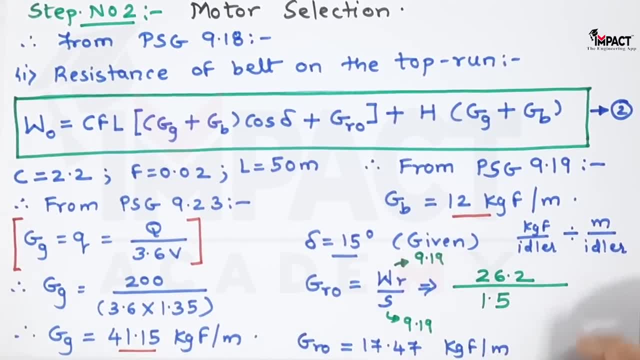 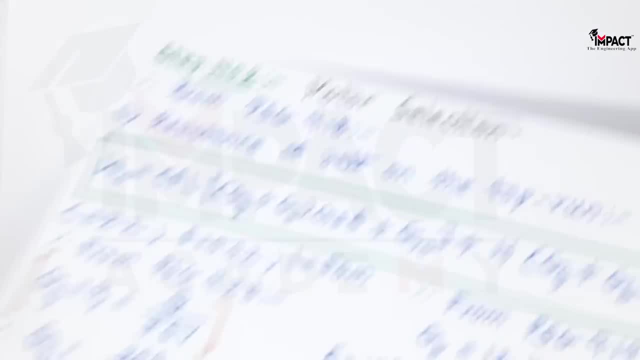 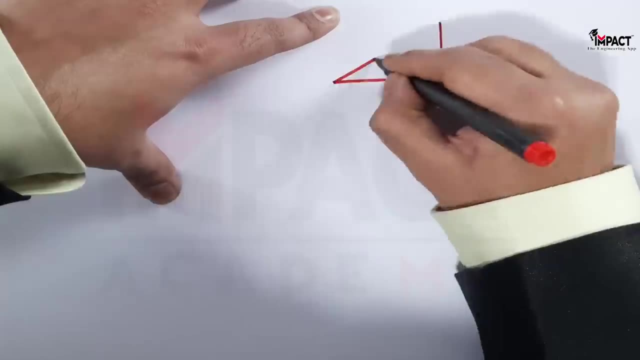 idler will get cancel, and the unit is kgf per meter. so that is GRO. next is height: see capital H is the height through which the material is conveyed. we know the length, and for that we can use a simple principle of trigonometry i. 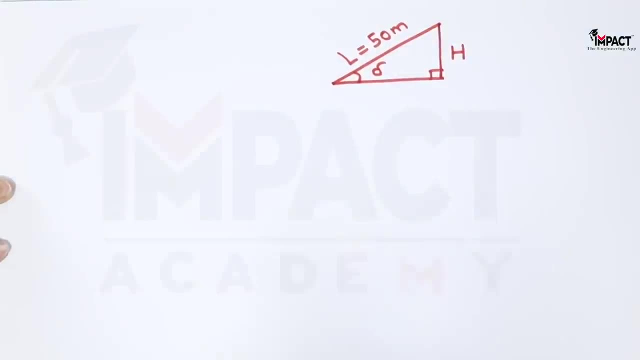 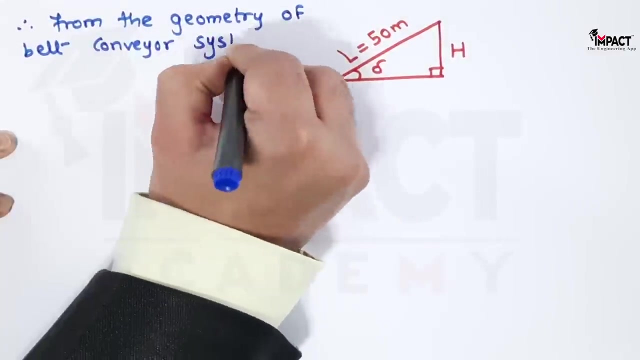 know. we know the length through which the material is being conveyed, that is 15 meter. but the height needs to be calculated, because that is the height going to be know the length, and for that we can use simple principle of trigonometry- from where up to which the material is being conveyed. So therefore, from this geometry, H is what? 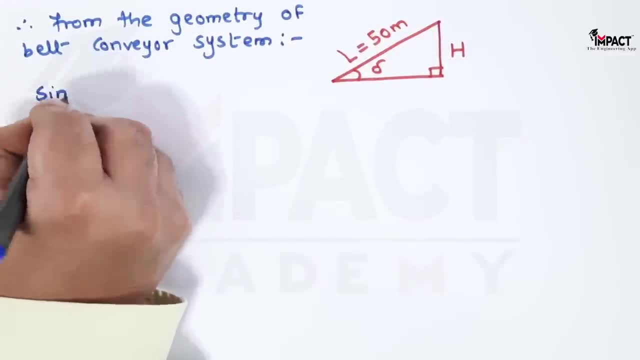 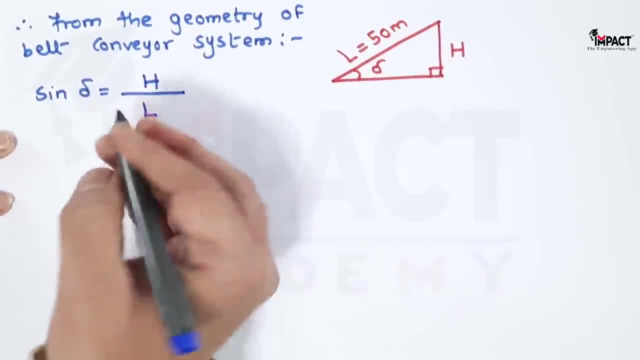 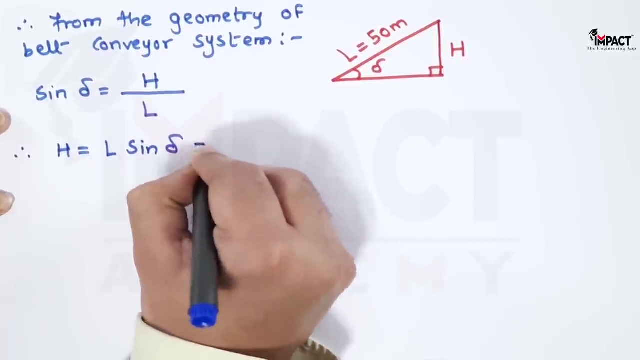 is required. So I will be using the formula of sine Sine. delta is opposite side, which is H, upon the hypotenuse side, which is L. So therefore H is equal to L sine delta. Delta is the angle of the belt, which is 15 degree, So therefore H value comes out to. 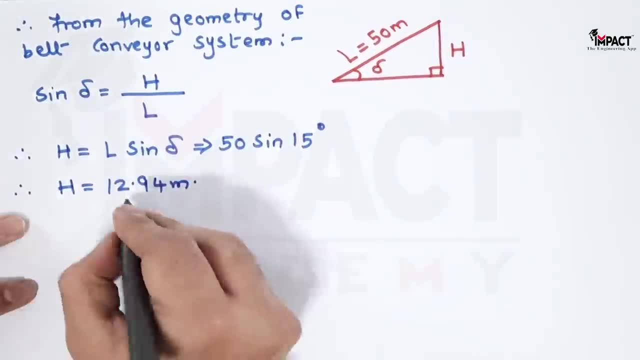 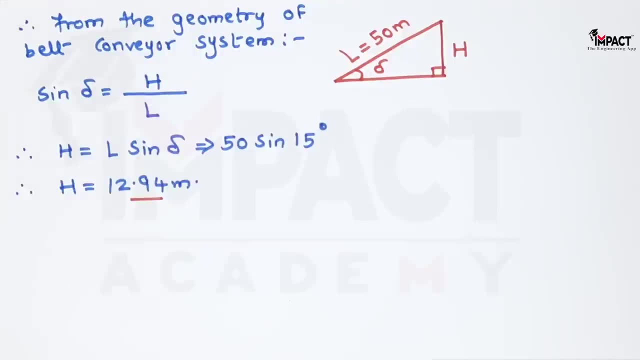 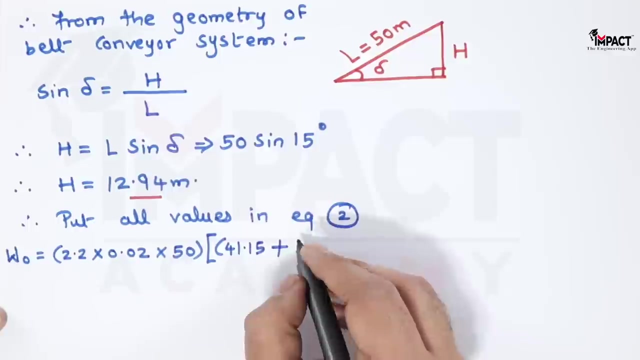 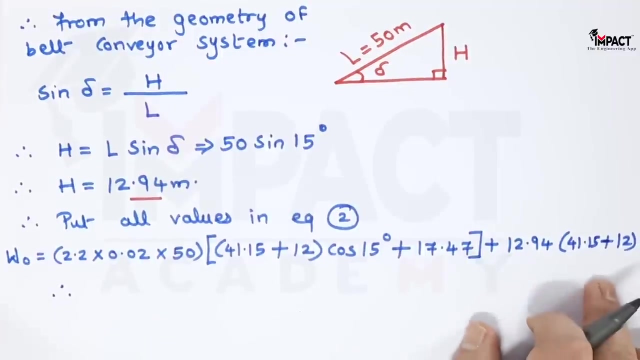 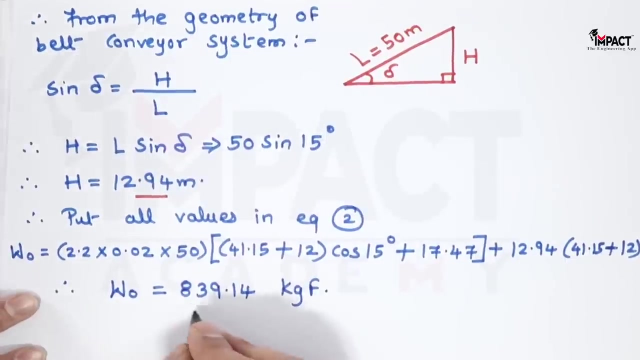 be 12.94 meter. Now, once all the values are known, I will be putting these values in equation. number second, So, therefore. So, after calculating this, the WO answer comes out to be 839.14 kgf. Now, similarly, 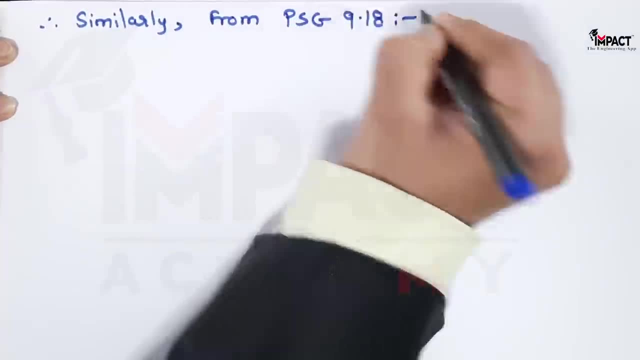 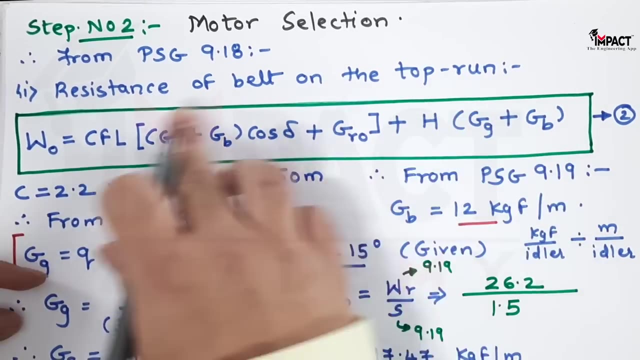 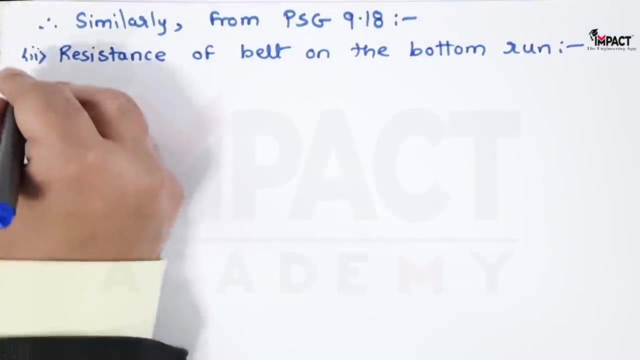 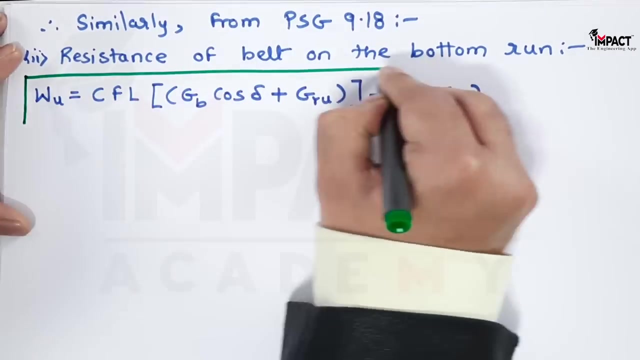 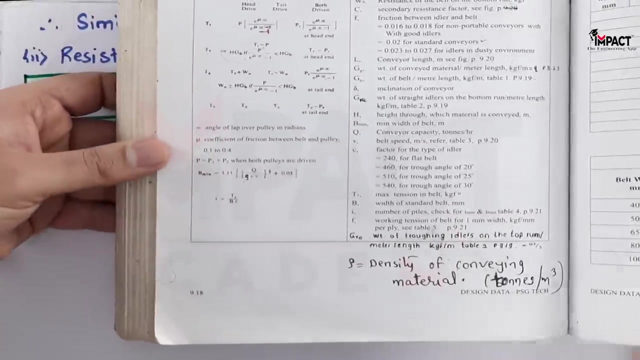 from the same page, that is, from PSG 9.18,. the way I have calculated the resistance of belt on the top run, I am going to calculate at the bottom run as well. The formula is that would be equation 3.. So from the same page, that is PSG 9.18.. Here. 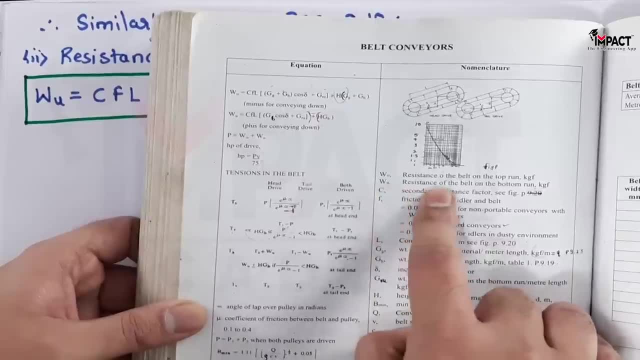 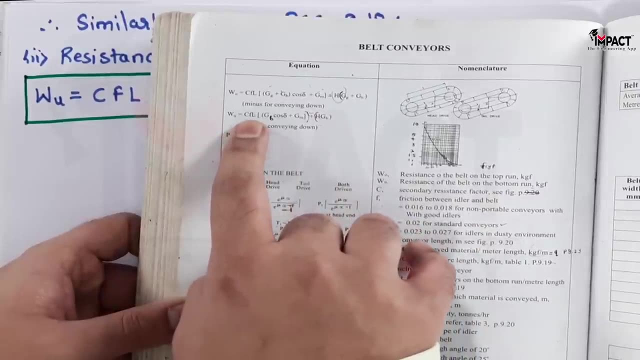 the second formula is W suffix u, and W suffix u is the resistance of the belt on the bottom run. Previously we have calculated the resistance on the top run. The formula is CFL. So we have here GF plus delta plus GRU. Now, outside the bracket we have plus or minus sign, and 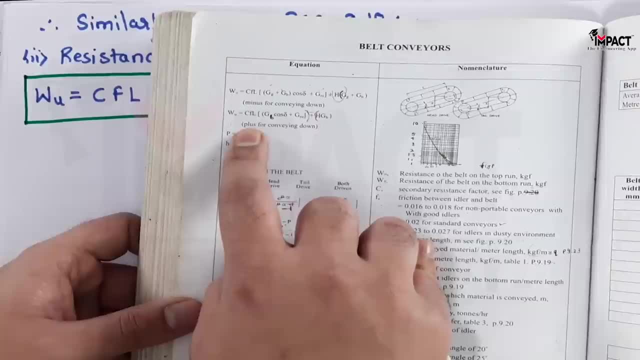 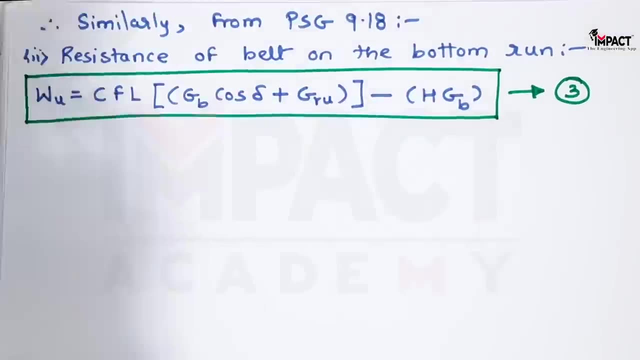 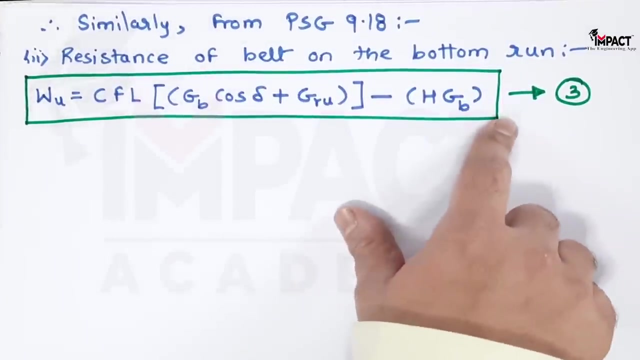 that depends on the conveying direction. Here it is given we have to take plus sign for conveying down, But since we are conveying up we have to take negative sign. So I have taken negative minus H into GV. So this is the formula Now when I look at all the values. 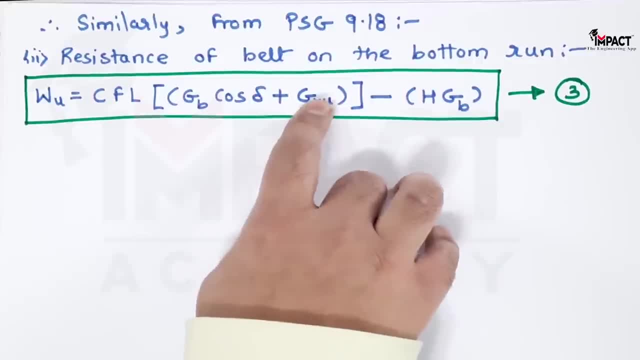 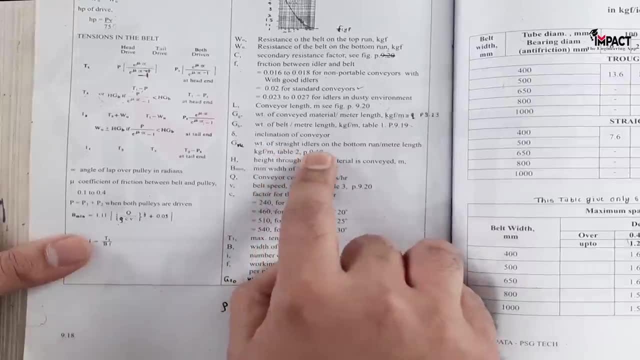 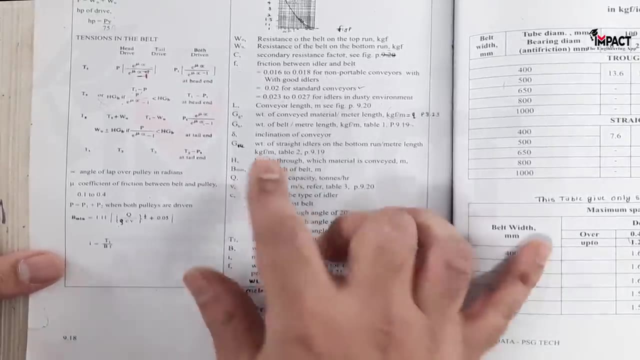 we have all the values over here except GRU, So that is what we have to calculate. Now calculate, and GRU is the weight of the straight idlers which are used on the bottom run, and in the start I had explained that why we are using the straight idlers at the bottom. 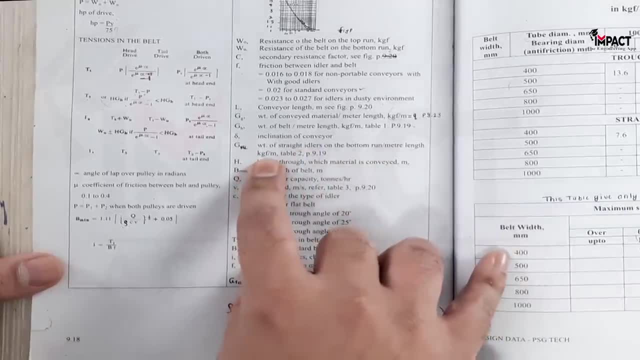 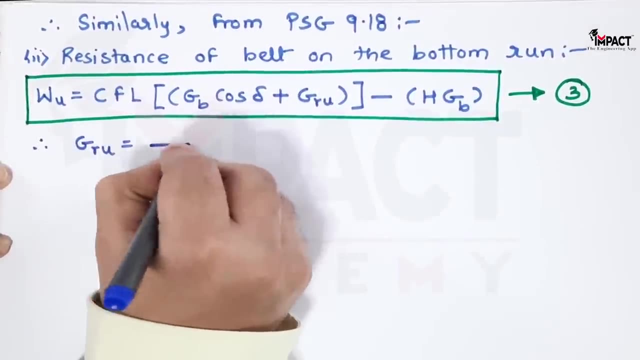 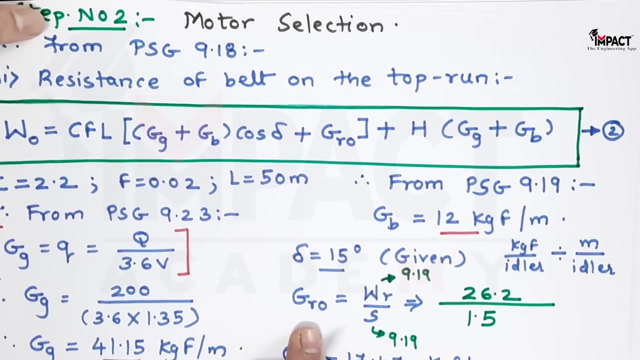 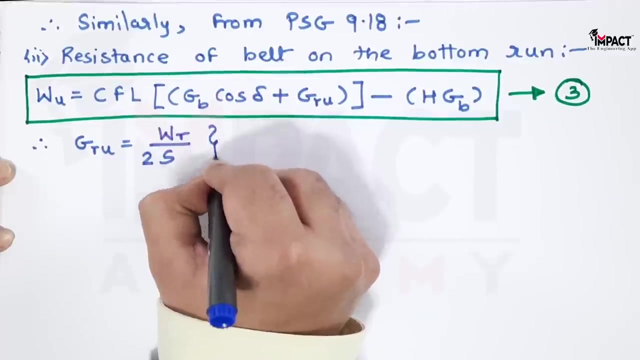 So it is the weight of the straight idlers on the bottom run. the unit is kgf per meter. So therefore GRU is taken as W suffix R upon space in a similar way, like I had used the formula for GRO, W suffix R upon S, here I am going to write 2S, and the reference is same: it is from PSG. 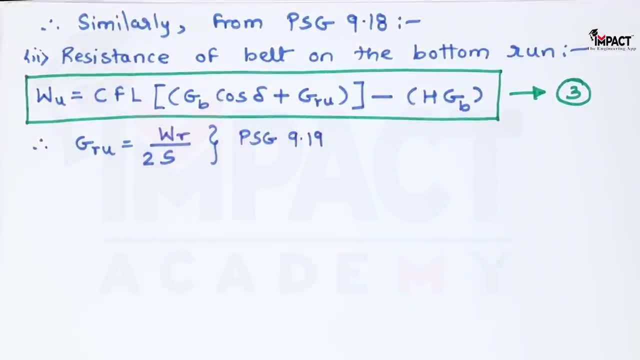 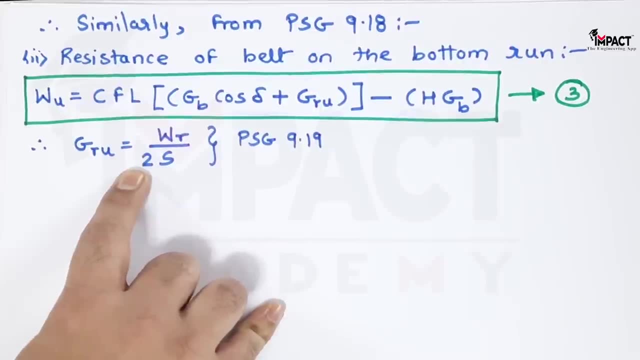 9.19.. Why I have written 2S? because in case of the bottom run rollers they are placed at a greater spacing, So the spacing is more compared to the top run rollers. So here I am writing 2S because the space is more at the bottom run. 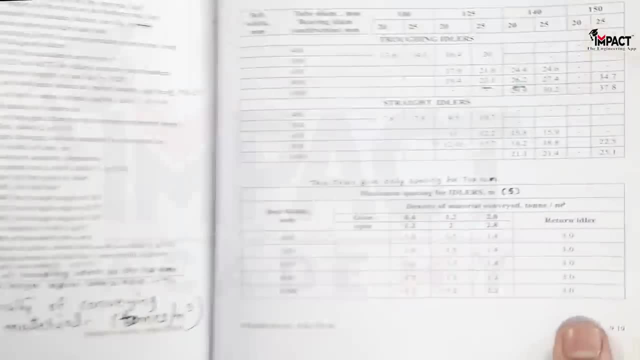 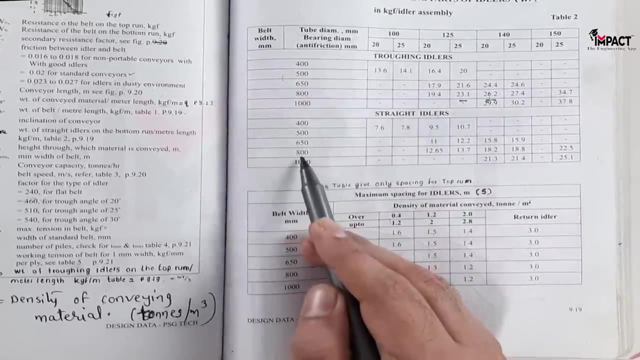 So that's why, and therefore the values are from PSG- 9.19.. We have to look for straight idlers. previously there were troughing idlers for straight idlers. take the width, which is 800 mm, and here we have again four values. 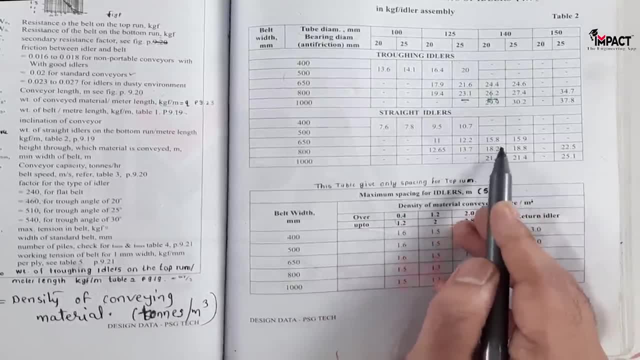 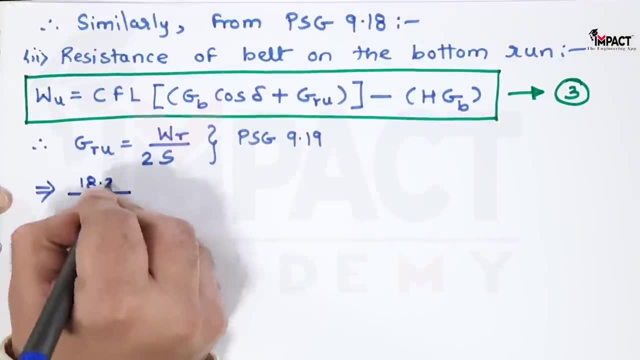 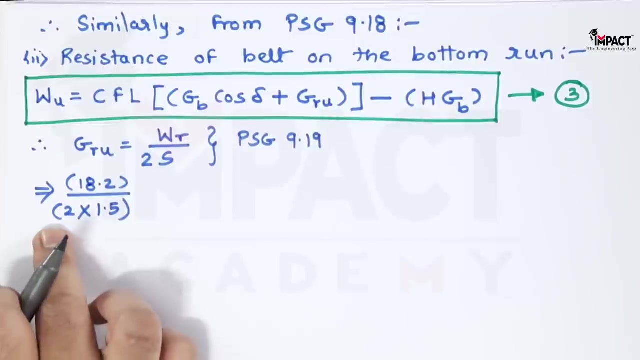 So select the middle two values and out of that take the greater value, So 80.. 18.2 is the answer, which is the WR value, and the spacing would be same, that is 1.5. S value is same, but it is double because at the bottom the idlers are located at a greater distance. 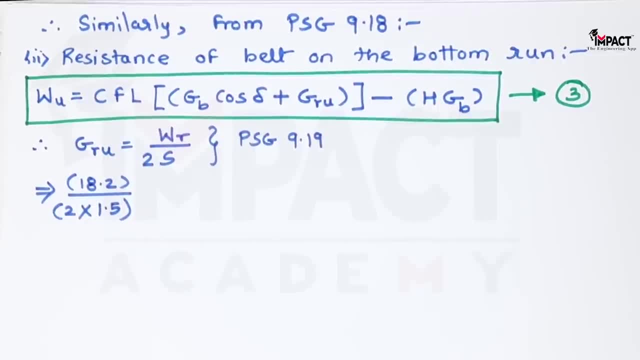 compared to the top run, because the top run is carrying the material, So the rollers are closely spaced on the top run compared to the bottom run and the answer is 6.07.. And the unit is 16.2.. Okay, Okay. 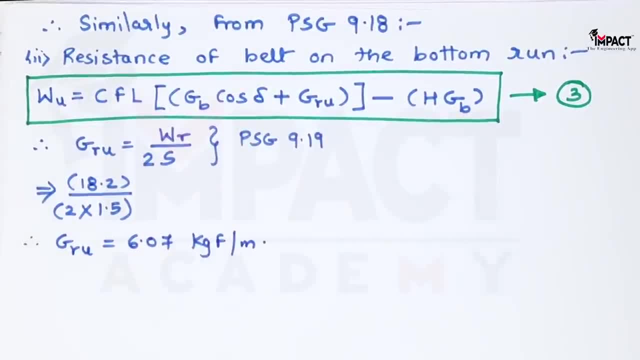 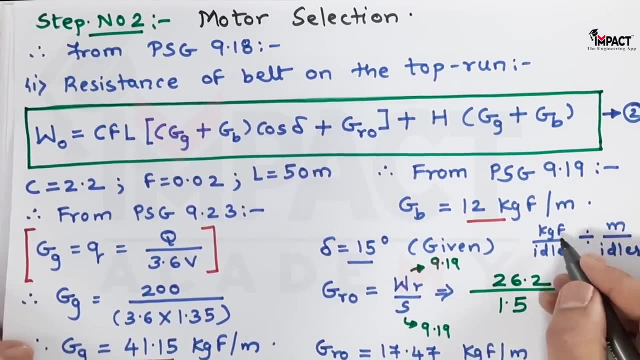 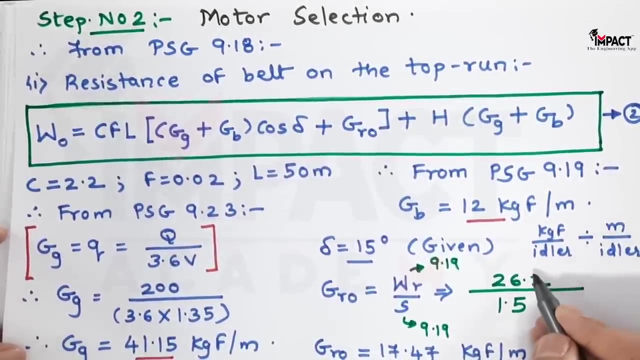 So the unit is KGF per meter and why we arrive at this unit is explained in GRO. in a similar manner, we have KGF per idler divided by meter per idler. So when we have multiplication idler goes on top idler idler will get cancelled out. 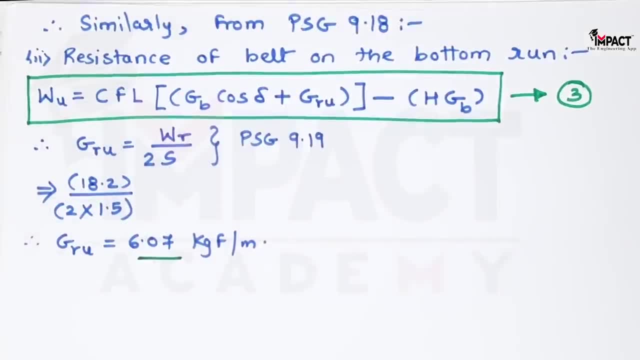 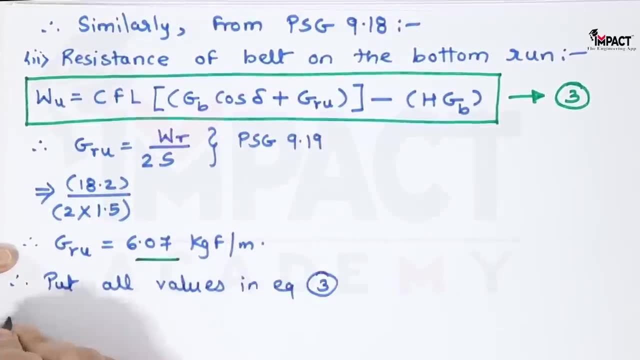 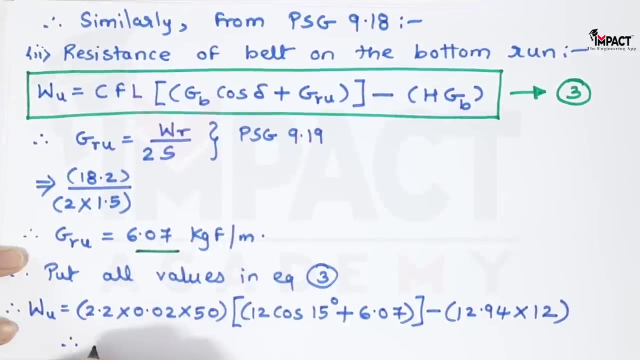 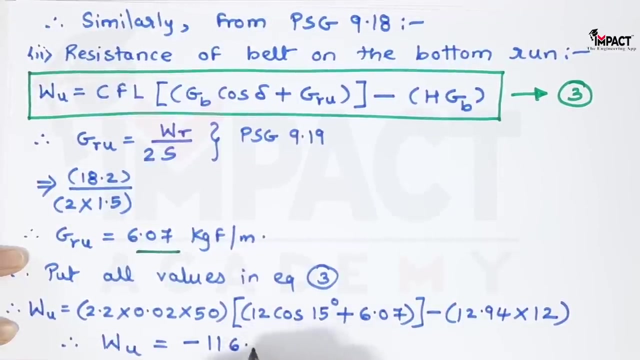 and finally, the unit would be KGF per meter. So once I have calculated GRU, I can put all values in equation 3.. So the unit is 16.2 KGF per meter. So therefore W suffix U value will come out to be minus 116.43 KGF, and this negative sign. 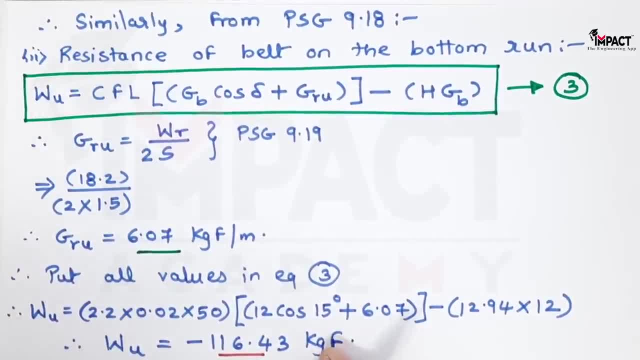 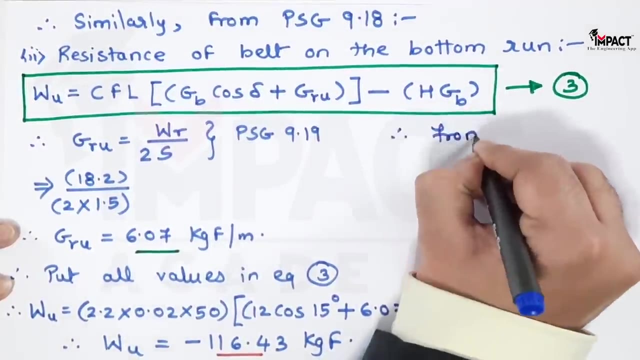 indicates we don't need to apply the force. it means the material will fall due to gravity. so that is why the force on the bottom run is negative, because the material is falling through gravity And therefore the total resistance on the belt- again from PSG, 9.18 P is equal to the 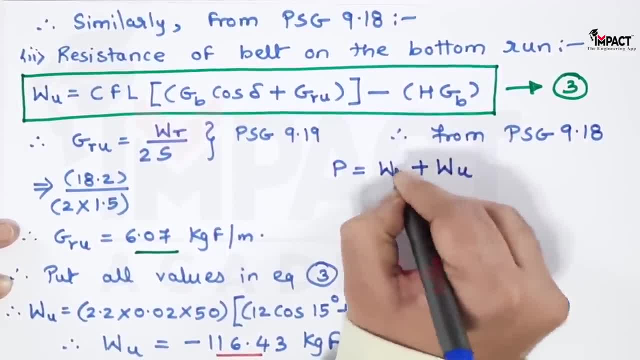 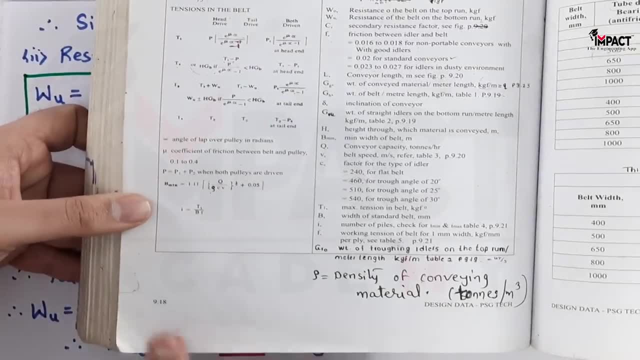 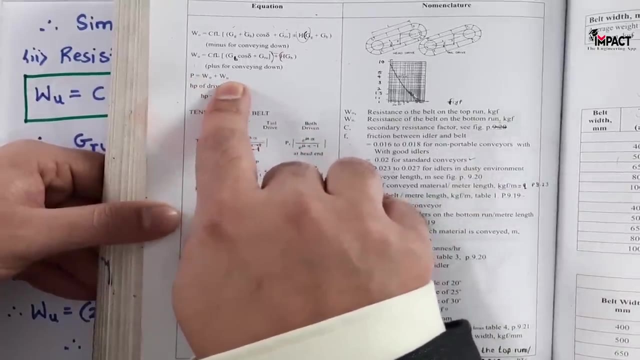 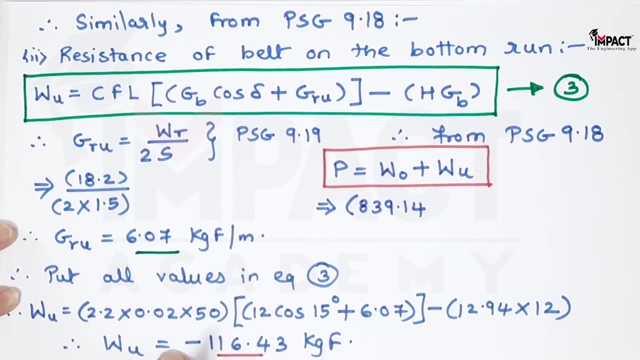 total resistance on the belt, weight on the top run plus weight or resistance on the bottom run. I will explain from where this formula comes. on PSG 9.18. here we have: P is equal to WO plus W suffix U. Okay, And therefore W suffix U is negative. 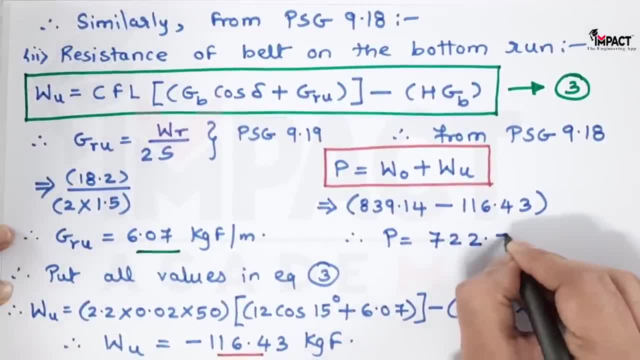 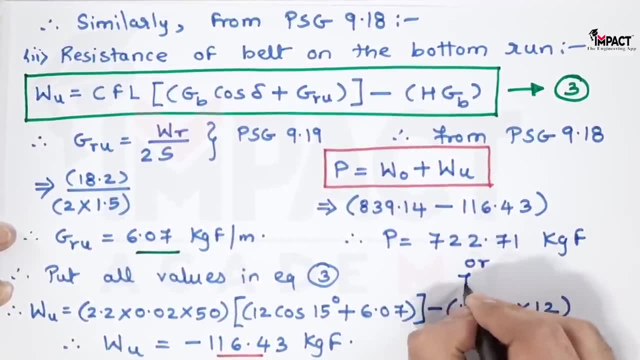 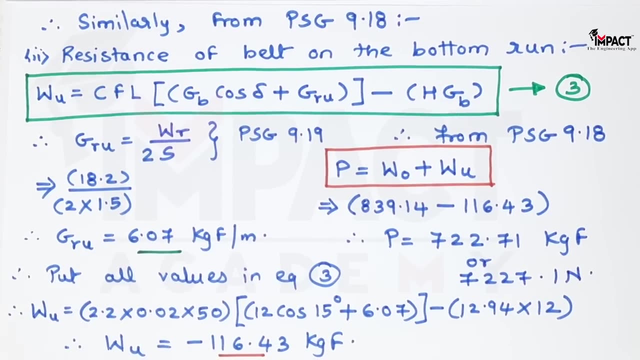 So, therefore, P value comes out to be 722.71 KGF, or when I multiply with 10, it becomes 7227.1 Newton. So that is the value of P. Okay, And remember, whatever we are doing this, it is for the motor selection part. 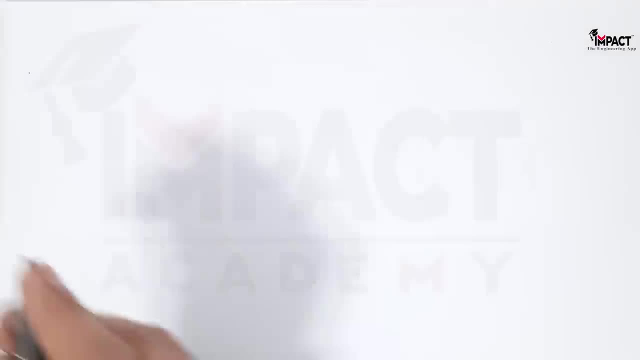 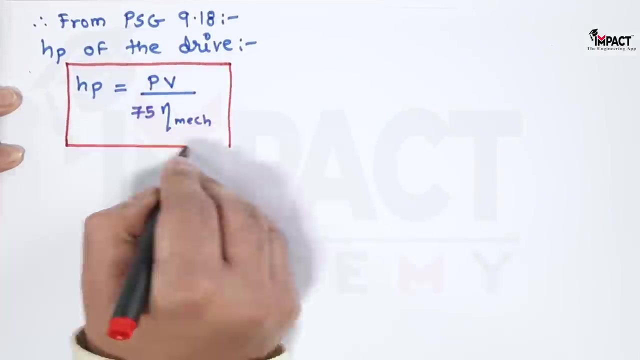 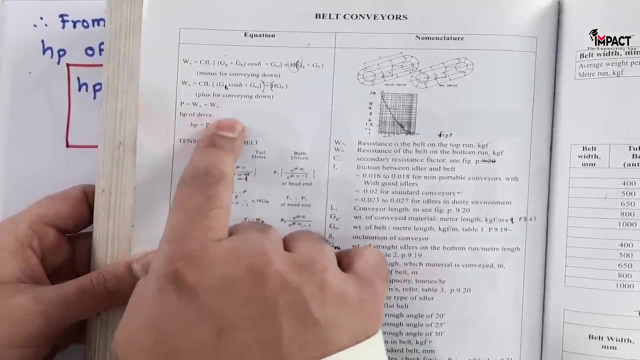 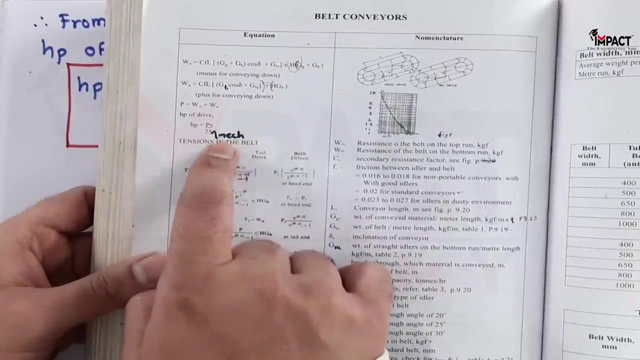 Now, once the value of P has been calculated, Now from PSG 9.18, here we have this formula: HP of drive, HP is equal to P into V upon 75. Now, Previously efficiency was not there in the, in the older PSG version. it would be there in. 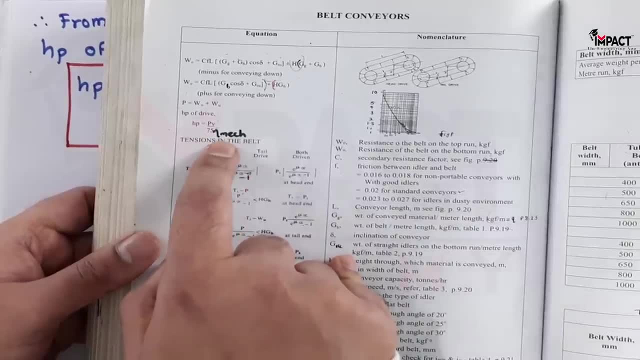 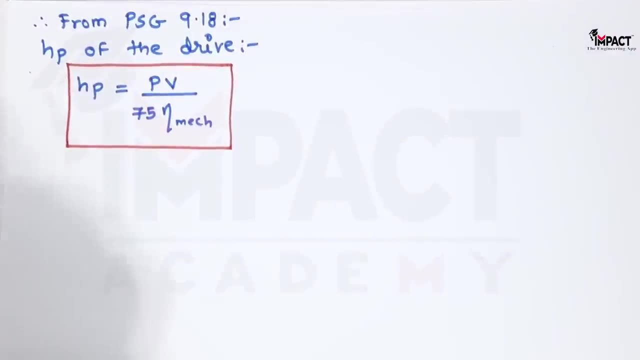 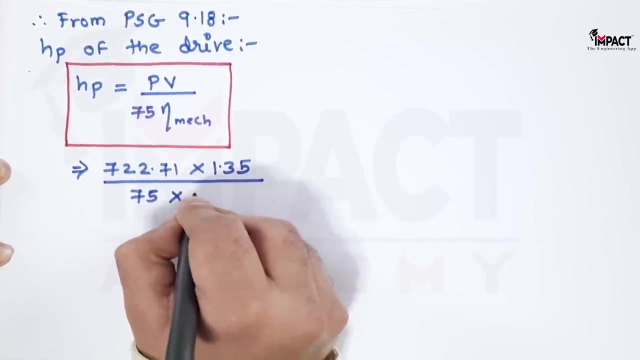 this updated version of PSG design data book. so here we have mechanical efficiency in the denominator, the formula I have written it over here. so therefore, putting the values P should be in terms of kgf velocity, in terms of meter per second mechanical efficiency: we can assume it to be 85%, so that 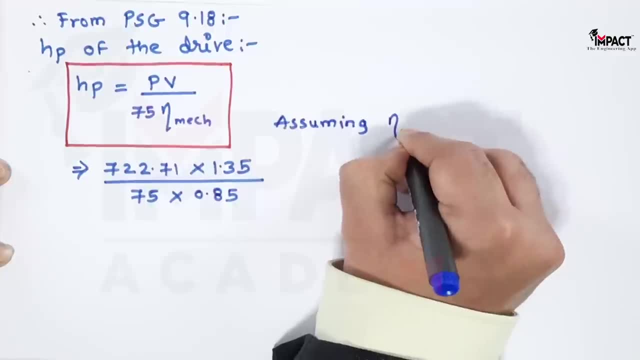 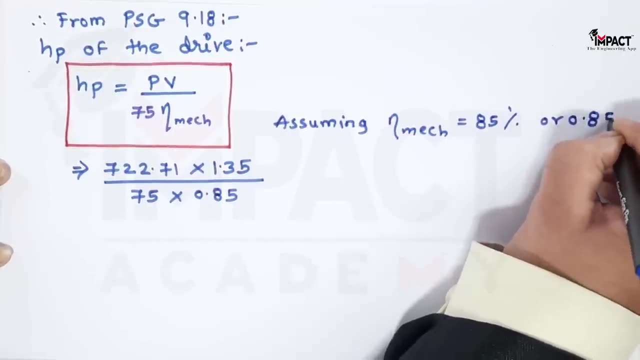 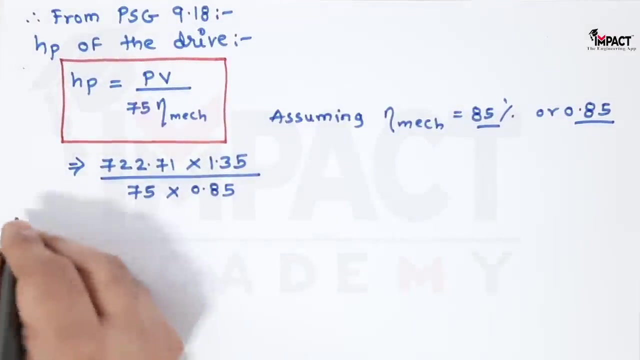 becomes 0.85. that is, assuming mechanical efficiency as 85% or 0.85, we can either assume 85% or even 90%. that is also correct. now, from this the horsepower of the motor comes out to be 15.30. 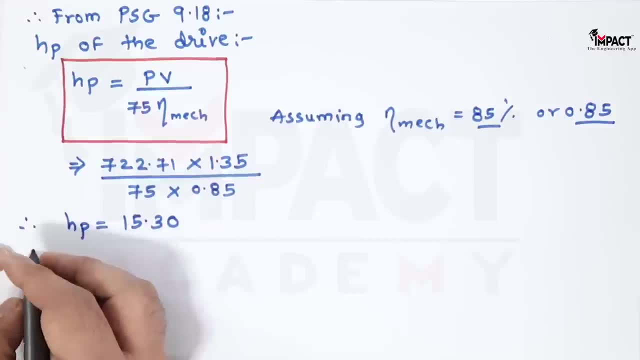 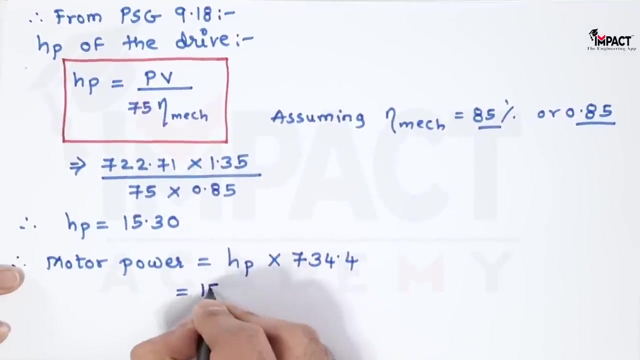 HP. next I'll convert it into watts. so therefore the motor power, because one horsepower is 734.4 watts. so therefore it is 15.30 into 734.4. so therefore the motor power comes out to be- and writing it as MP capital, it is 15.30 into 734.4. so therefore the motor power comes out to be- I'm writing it as MP capital, it is. 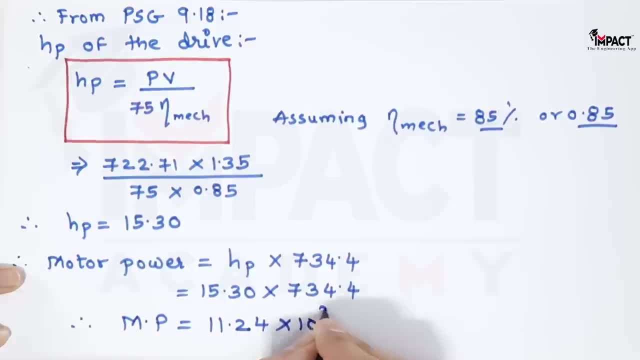 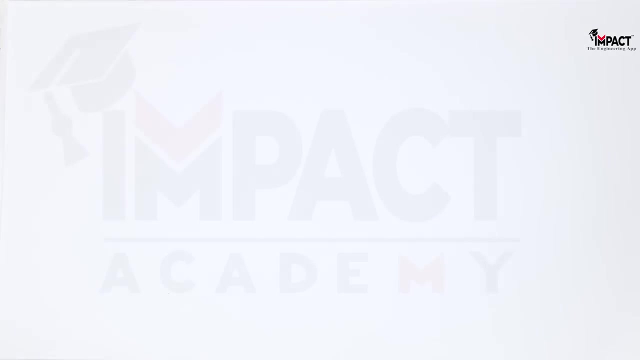 11.24 into 10, raised to 3 watts, or we can say 11.24 kilowatts. then, after getting this motor power, I have to select the standard motor power. so therefore, from PSG 5.124, we have to select the standard motor power. so here we have PSG 5.124. we have to select the standard motor power. so here we have PSG 5.124. we have to select the standard motor power. so here we have PSG. 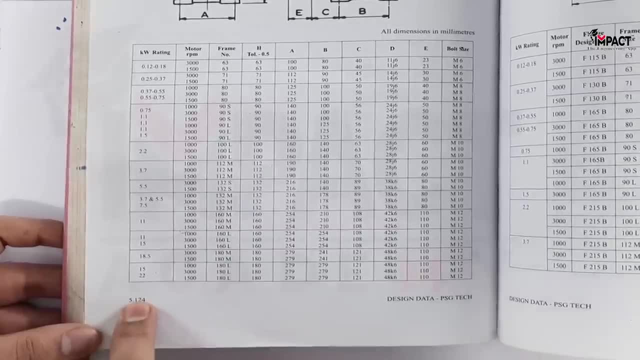 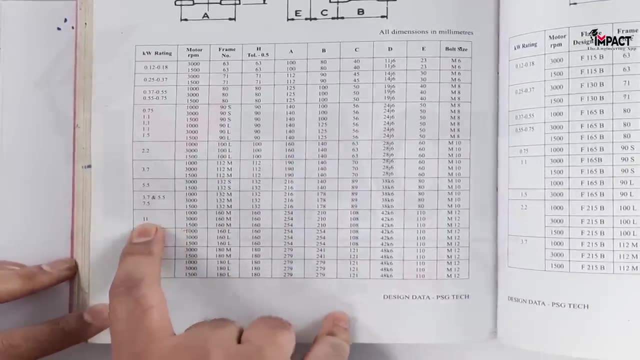 PSG 5.124, we have to select the standard motor power. so here we have PSG, page number 5.124, and in this column, the first column is having power in terms of kilowatt. now we see here we have 11 kilowatts. after that we have the power. 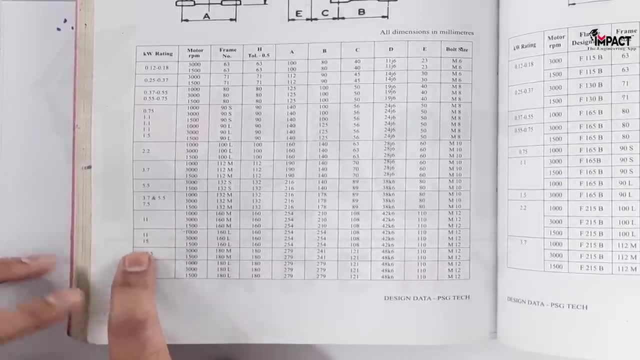 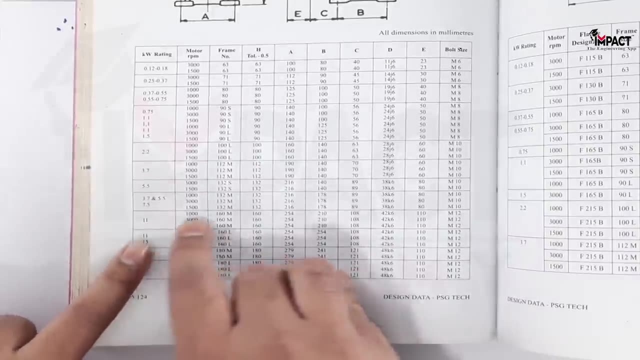 in the range of 11 to 15, as we can see here, since our answer is 11.24, so it is very much close to 11 kilowatt. so I have to select the standard power as 11 kilowatts, but it is available in three. 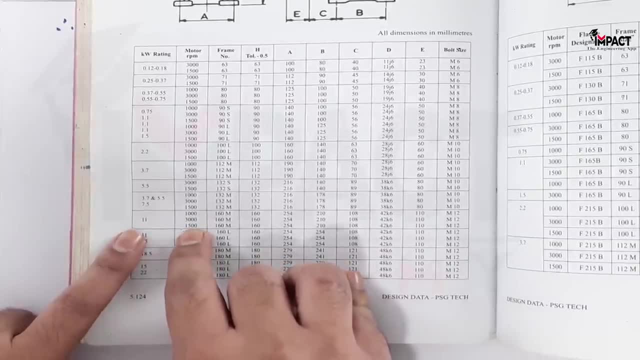 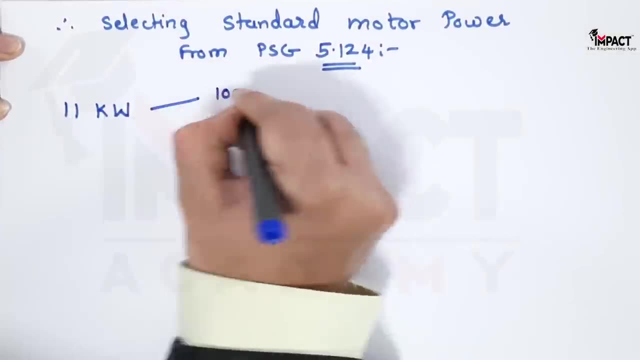 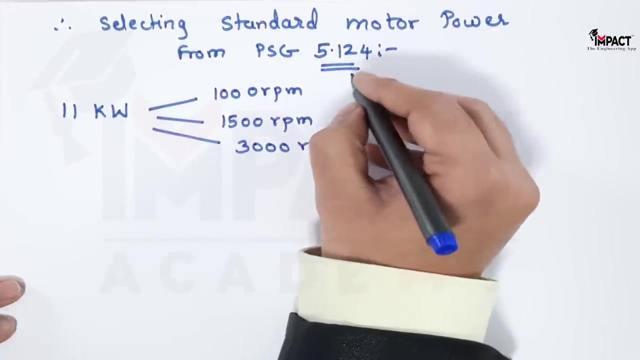 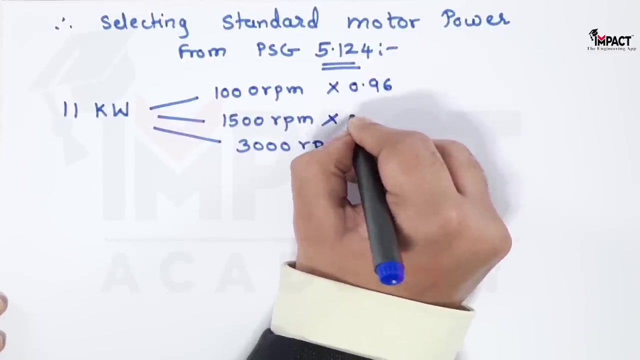 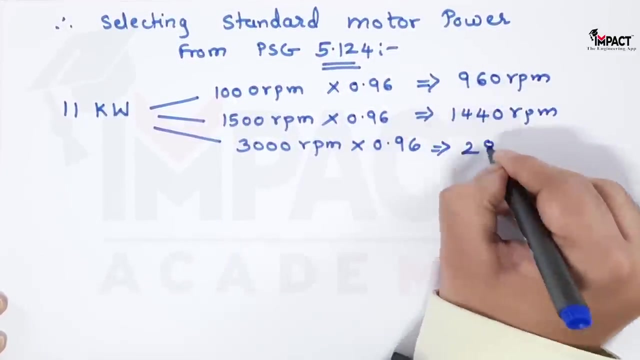 different speeds, as we see here: thousand rpm, then there is 1500 rpm and then there is 3000 rpm. so how to select that? now? these three speeds are available in that I am again multiplying with the mechanical efficiency, taking it as 96%, so 0.96, so it is 960 rpm, so three speed options are available. 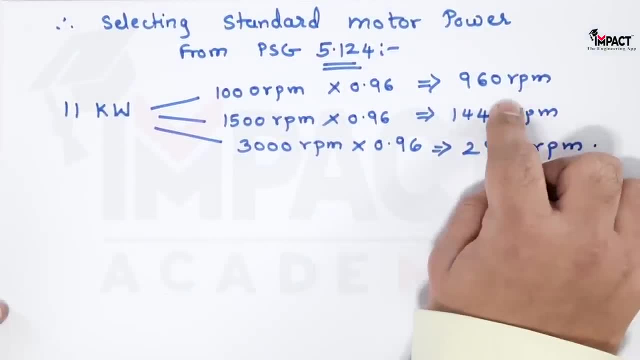 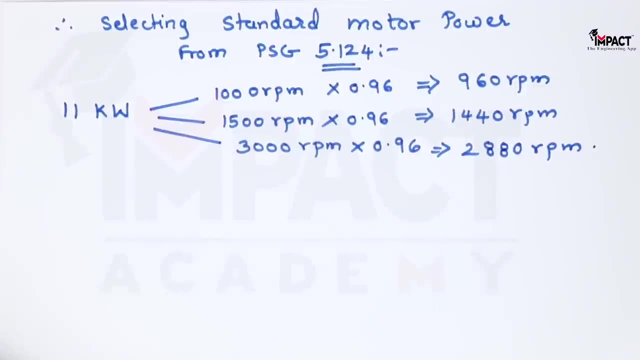 as we can see here. remember, whenever, in case of motor, if the motor is operated on a less rpm, as we can see over here, that motor becomes costly, because in that case the construction of that motor is complex. well, in order to get the speed reduction, so here this motor having rpm of 960 would 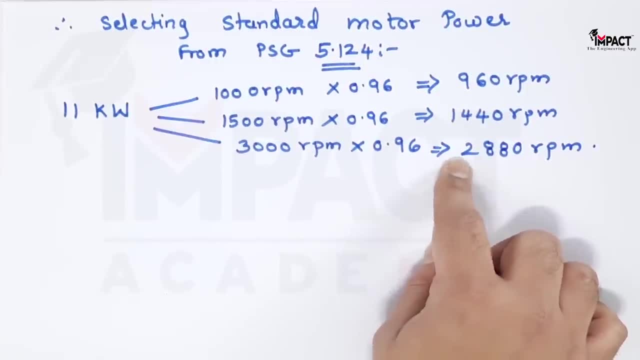 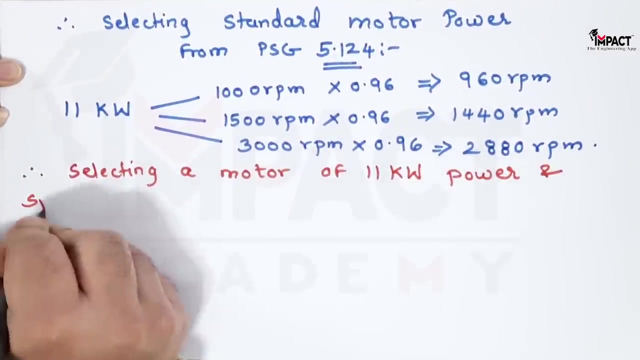 be a costly motor. then for the further option when the speed is high. in such a case the space required would be greater. so we have to have a compromise between the cost as well as the space. so therefore, so selecting that. well, if you can see the speedу, I am again multiplying over here with 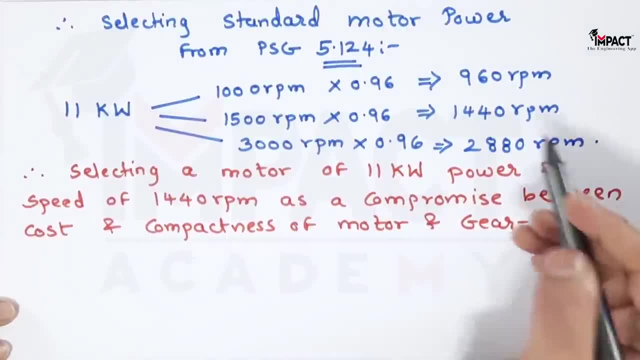 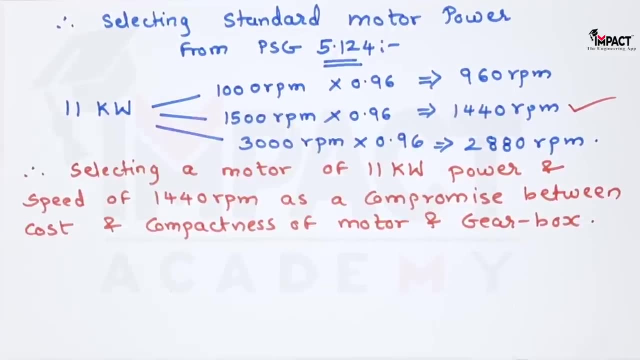 a standard motor of 11 kilohertz power and having a speed of 1440 rpm as a compromise between the cost and even the size or compactness of the gearbox and motor. because whenever these conveyor belts are used, they are used in that space and mostly coal in order to convey it would be used. 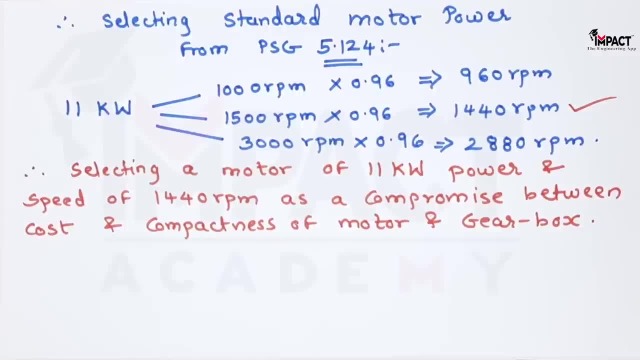 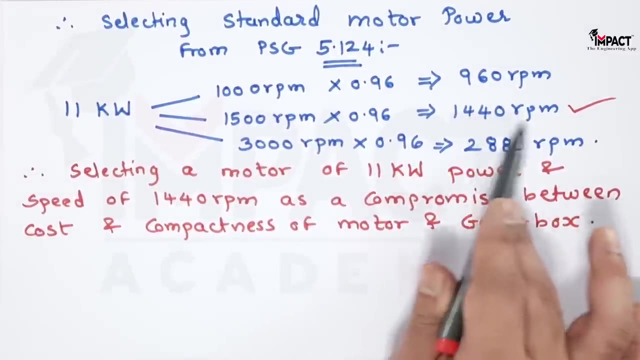 in the mining application. so there the space requirement is not a problem. at the same time, if it is operating at a really high speed, then the space required would be more, but at the same time we have to check for the belt speed as well. so in order to compromise, for that, select the 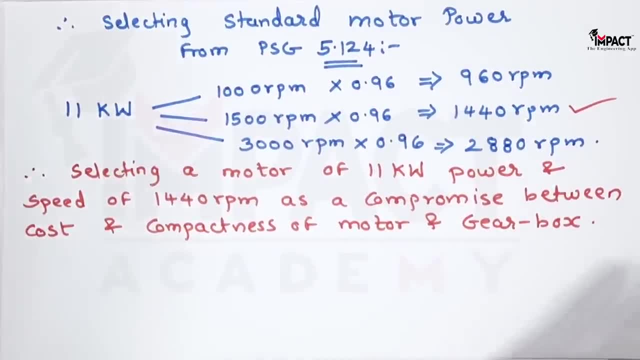 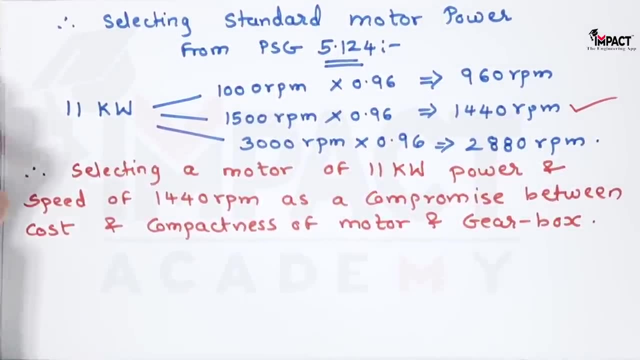 intermediate speed, which is 1440 rpm. now, that completes the step number second. so in the belt conveyor system first we had designed the belt and now the motor selection. part is over, now going for the belt cross section. so in the belt conveyor system first we had designed the belt and now the motor selection. 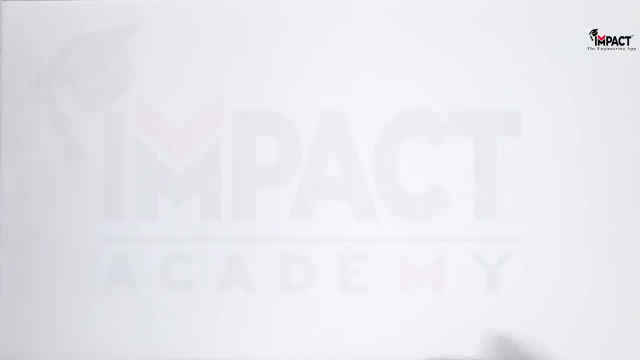 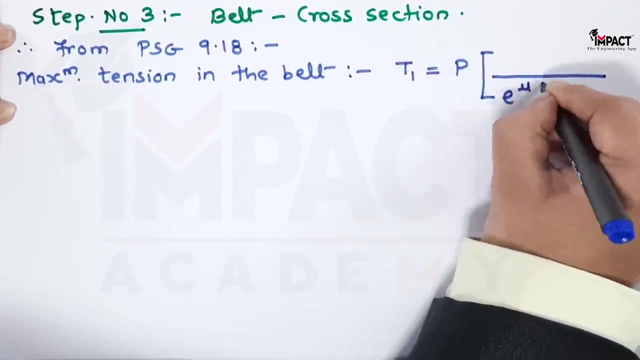 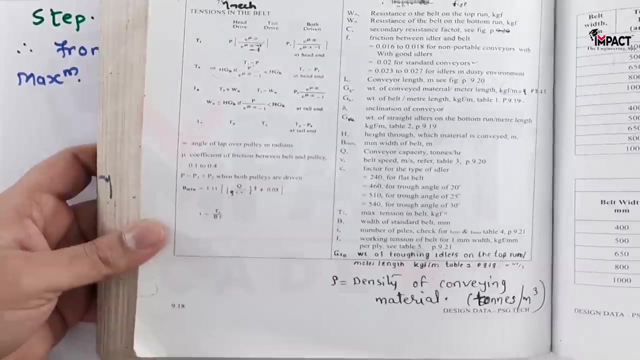 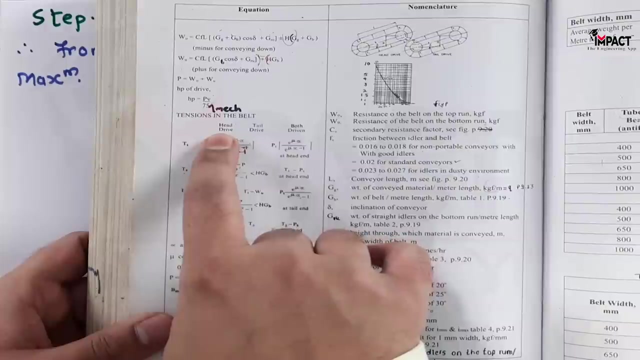 now going for the belt cross section. so the third step is. step three is deciding the belt cross section. for that, the first thing required is the maximum tension in the belt. so therefore, so from psg 9.1 head. again, here is the formula of the tensions in the belt. so we have the head drive. 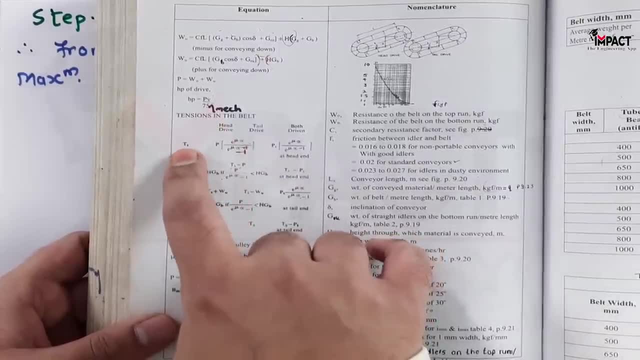 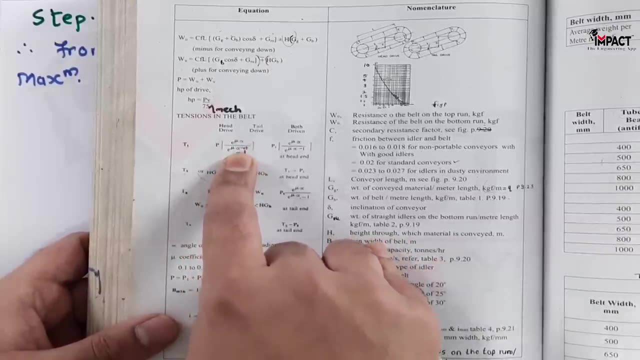 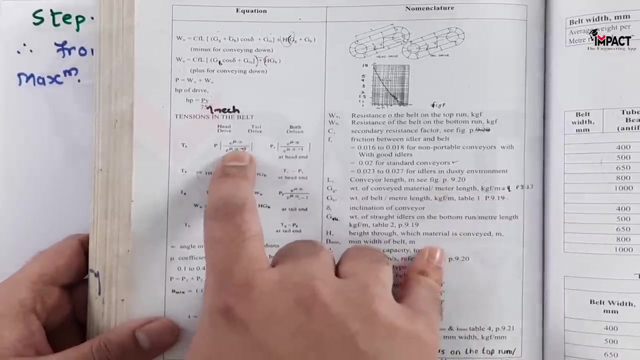 or we can say: the driving pulley for that t1 is p into into bracket, e raise to mu into alpha upon, e raise to mu alpha minus one. now, in this case, this minus one is not in the race to par, as we can see here. the formula is: 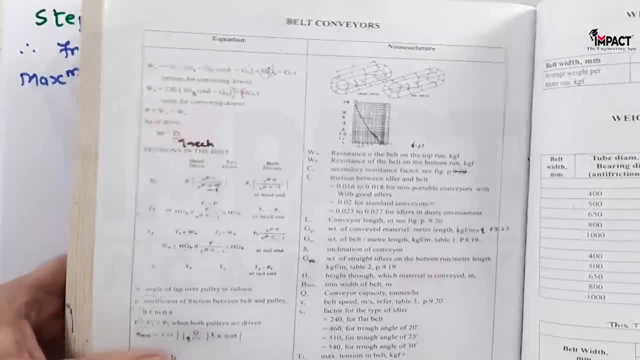 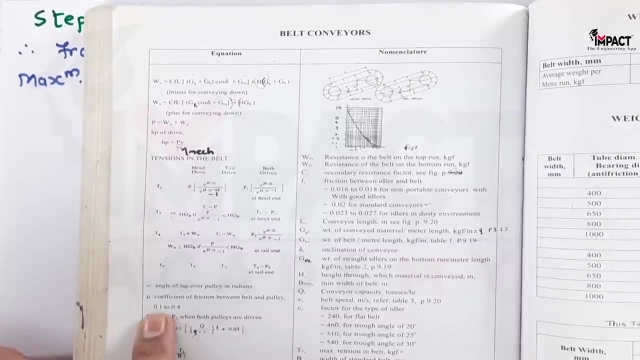 written over here, so we have to check it next. mu is the coefficient of friction. coefficient of friction between belt and pulley. the value is between 0.1 to 0.4, so it is better to take the average value, because nothing is specified about. 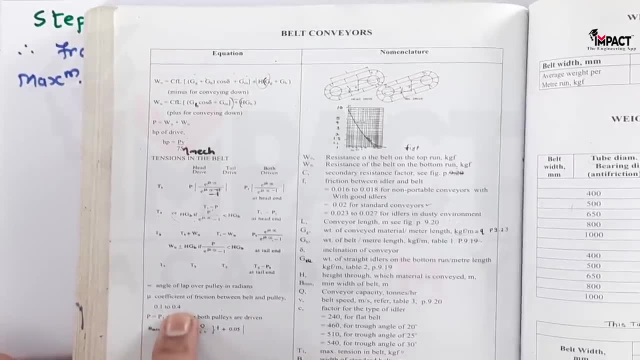 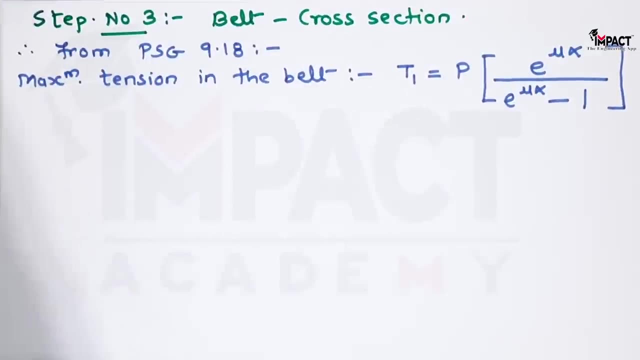 the coefficient of friction. the average of 0.1 and 0.4 would be 0.25. then alpha is also there. alpha is the angle of the snub pulley. snub pulley i had explained in the beginning. it is used for: 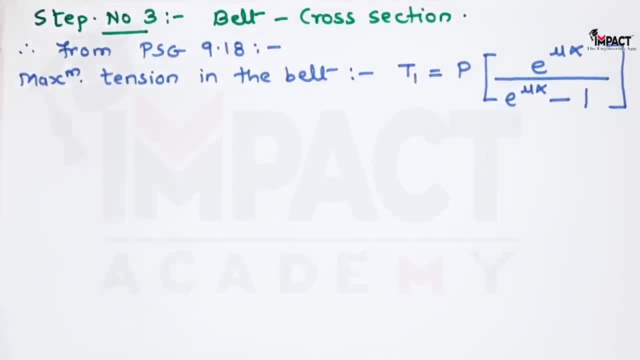 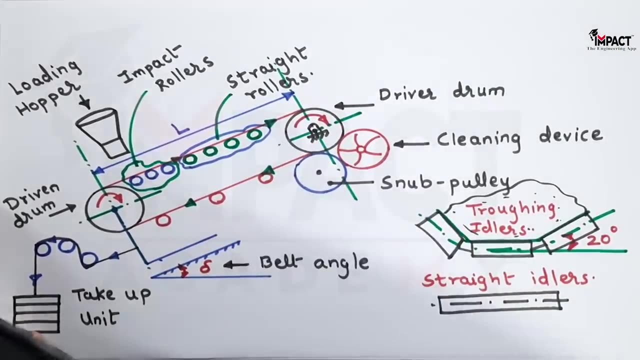 increase in the angle of the snub pulley. and then alpha is also there. alpha is the angle of the ainsi hoarding the data over here. Answer the câfahak thing. snub pulley is used to increase the angle of lap for the given belt. 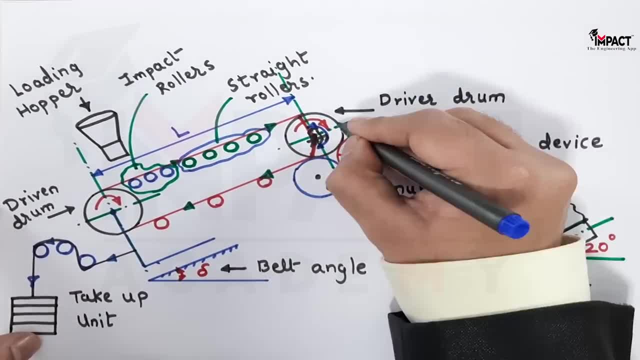 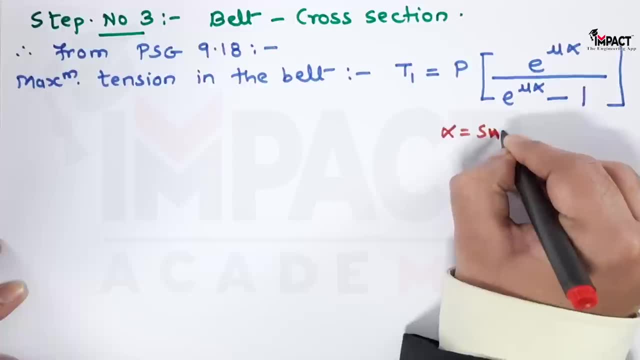 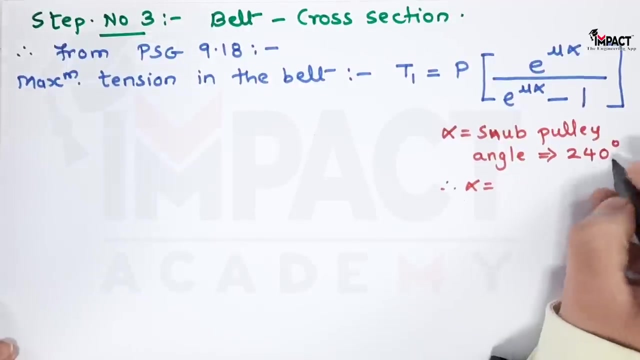 so this is the angle of lap, denoted as alpha. so here alpha is the number pulley angle, which is taken as 240 degree, the standard value. Therefore, in terms of radian multiplied by pi, divided by 180, so it comes out to be 4.19 radians. Now putting 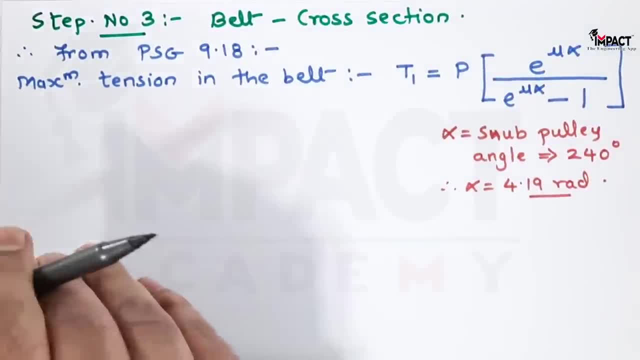 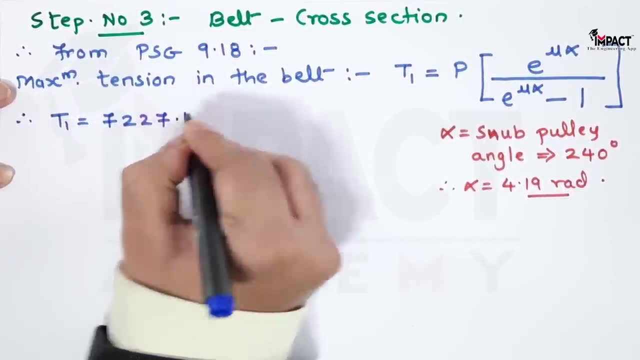 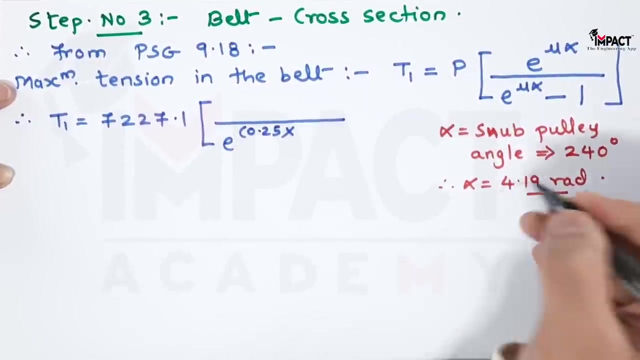 all values to get T1, P should be kept in terms of Newton. So therefore P is 7227.1. P raised to mu is 0.25.. As I have said, take the average value. Alpha is 4.19 put in terms. 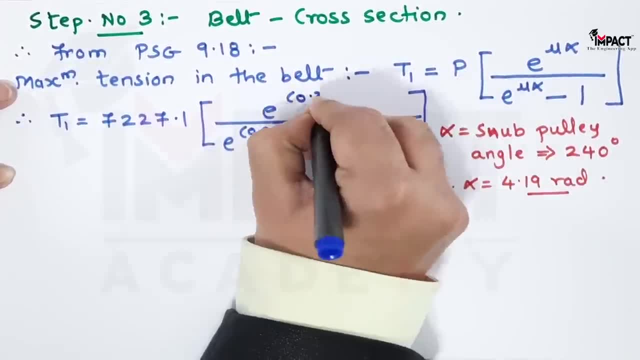 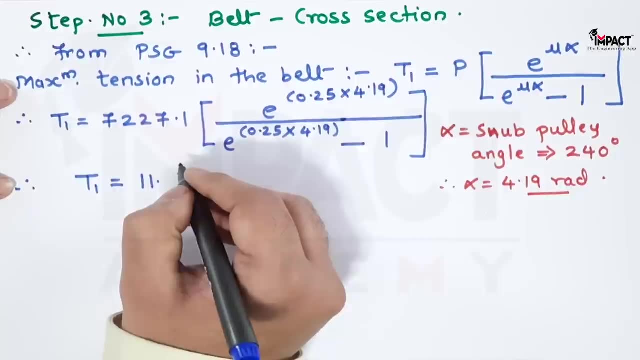 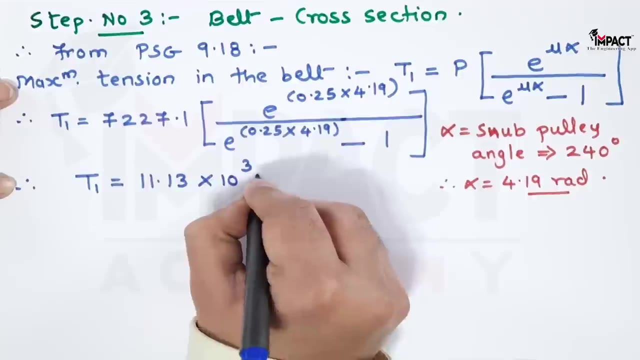 of radian minus 1.. So therefore, on calculating this, I am going to get the answer of P1, which is the maximum tension in the belt, also called as tension in tight side, 11.13 into 10, raised to 3 Newton, or it is 11.13 kilonewton. 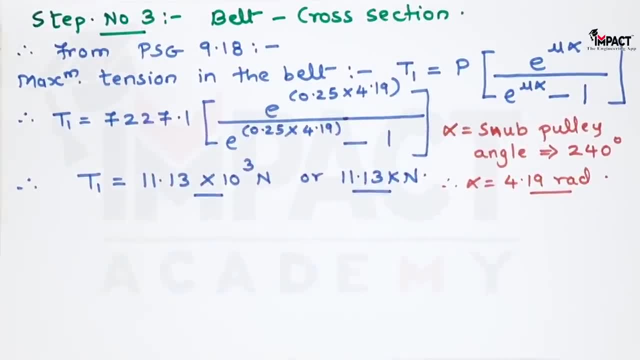 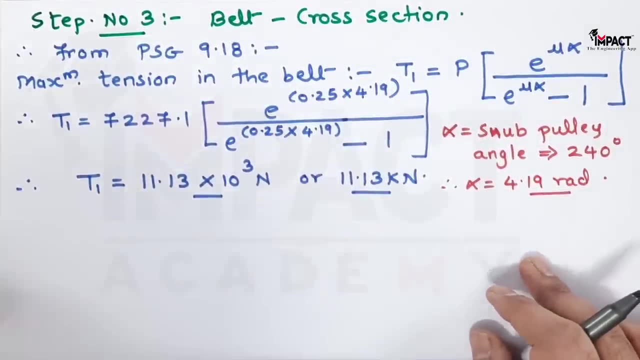 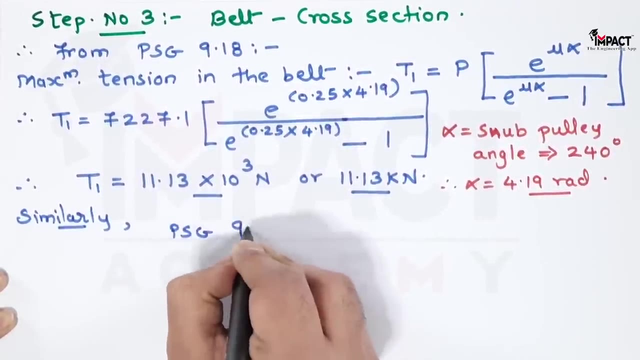 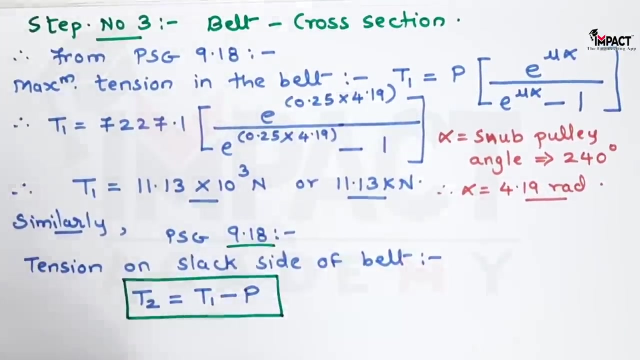 So that is the tension on the tight side. Next, similarly, I will be calculating the tension on slack side as well. It would be required in the further part of the problem. So, similarly on the same page, that is PSG 9.18.. So on PSG 9.18, here we have the formula. 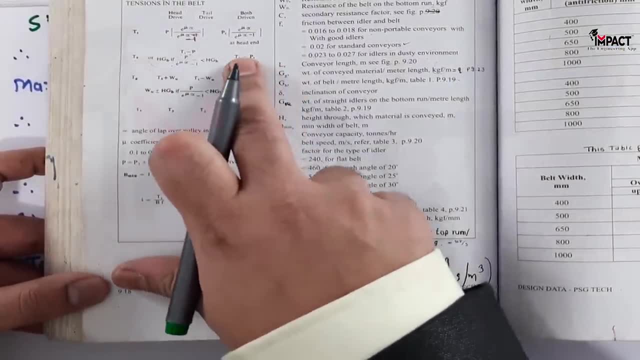 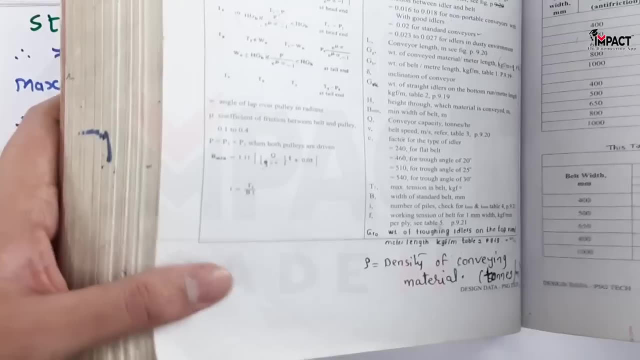 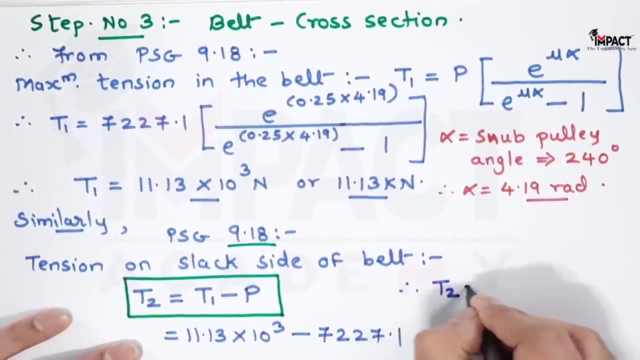 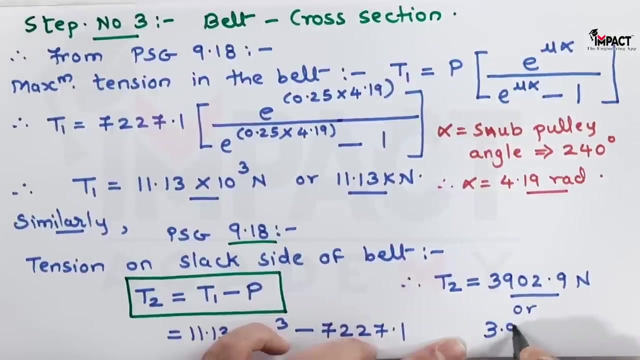 of T2.. Which is the tension on the slack side. It is P1 minus P1.. As we can see here we can write P because P1 indicates for the head drive. So therefore, putting the values, So therefore T2 value comes out to be 3902.9 Newton or 3.902 kilonewton. So T1, T2 have 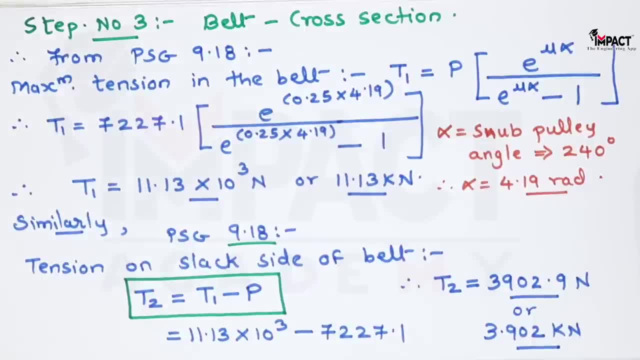 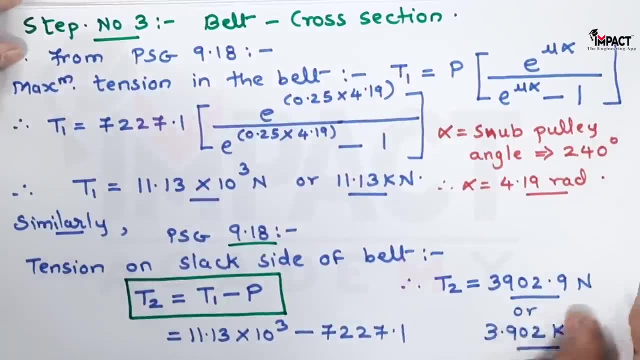 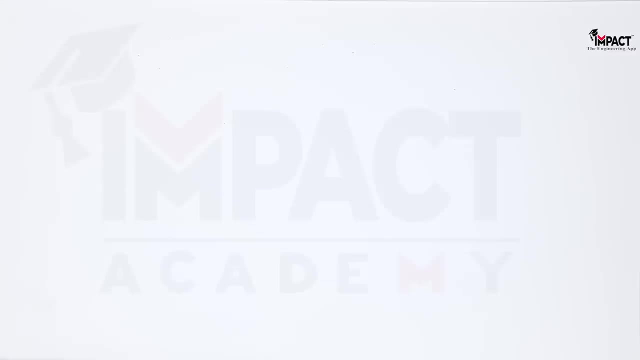 been calculated. That is, the tension on the tight side and slack side respectively. Now, since we are deciding, the belt cross section belts are made up of rubber and there is fabric duck At the same time. first we have the fabric duck In between, the rubber is impregnated. 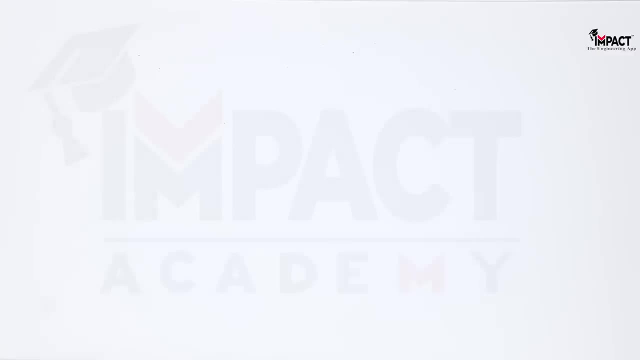 and the top layer as well as the bottom layer consists of rubber. So there are number of plies or the number of layers in case of the belt. So sometimes a couldn't have a fabricmay or a layer. In other words, if my belt is impregnated, maybe even split between the fabric. This is a doubt. You should realize that if there are two or three layers, then there are two layers, 즙 An and rubber, and in other all of them are declared to increase winners. These So, therefore, from PSG: 9.18 number of plies, or we can say the layers are denoted as I. 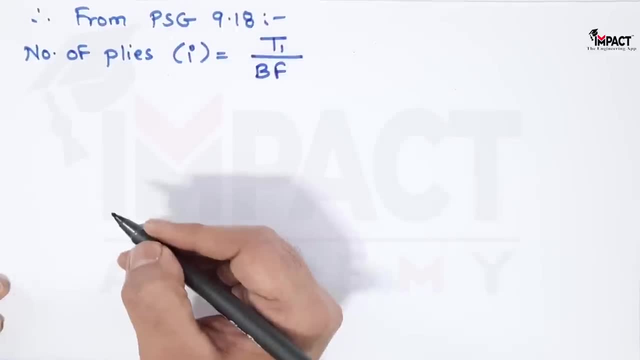 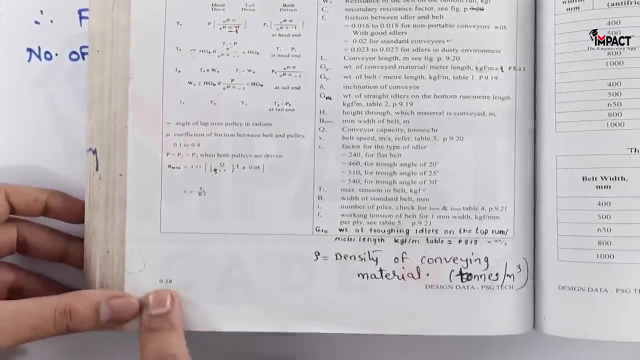 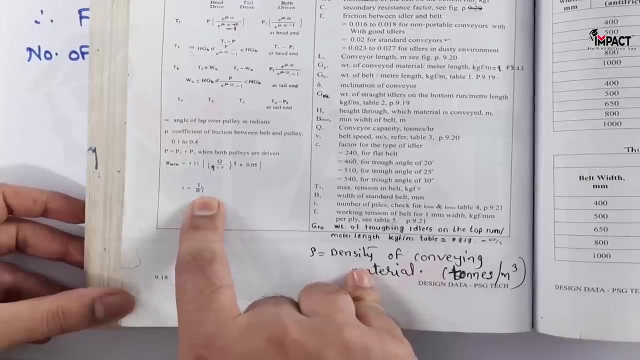 is equal to T1 upon B into F. So, going on to the same page, that is PSG 9.18, at the bottom, see the last formula, which is: I is equal to T1 divided by B into F. So this is the formula. 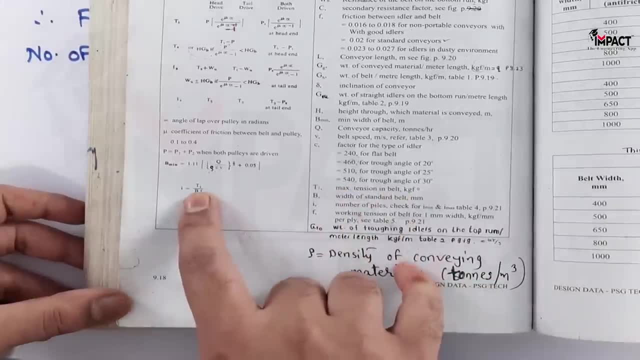 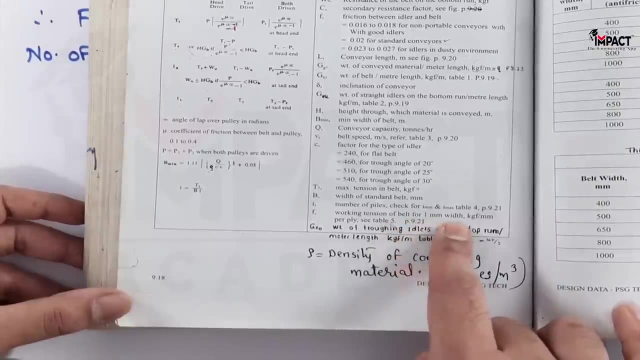 for the number of plies, where T1 is the maximum tension in the belt We have found out. B is the width it should be in terms of mm and F is the working tension of the belt for one mm width. it is in terms of kgf per mm. and how to get this small f value that I am going? 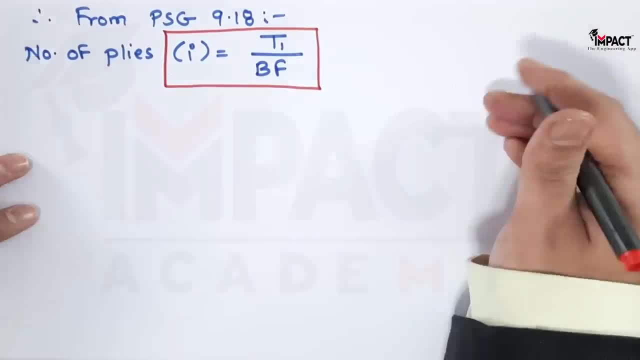 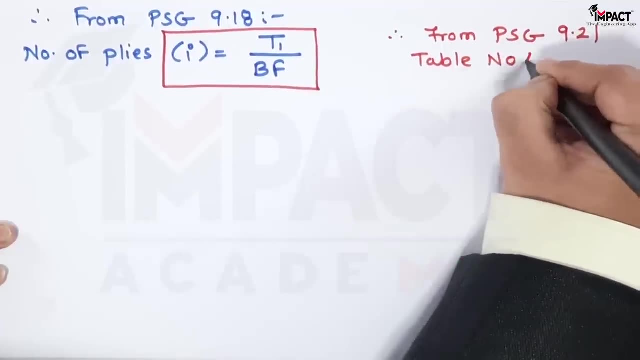 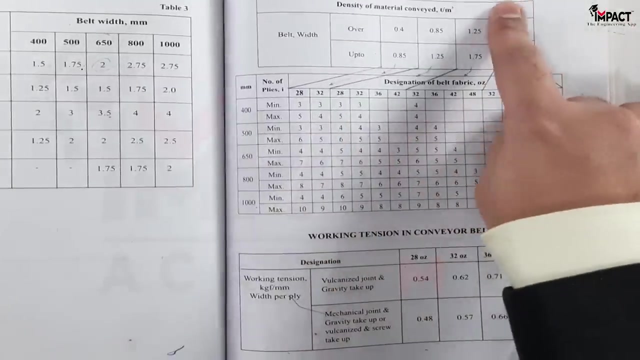 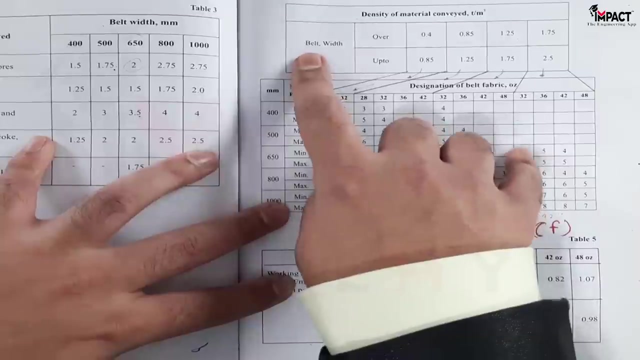 to explain it over here. So first, from PSG 9.21, table number 4 and 5. as we can see, here we have PSG 9.21, here we have table 4 and table 5.. So how to get the values: see here we have the belt width as well as belt width. 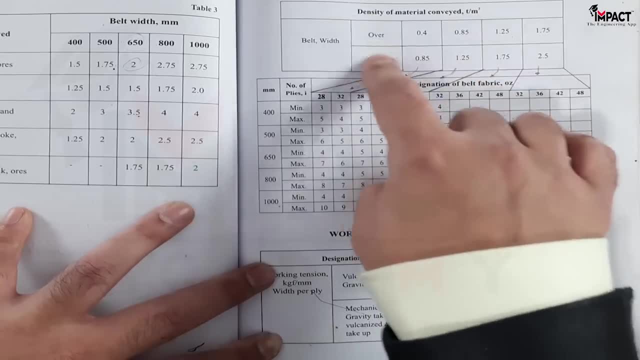 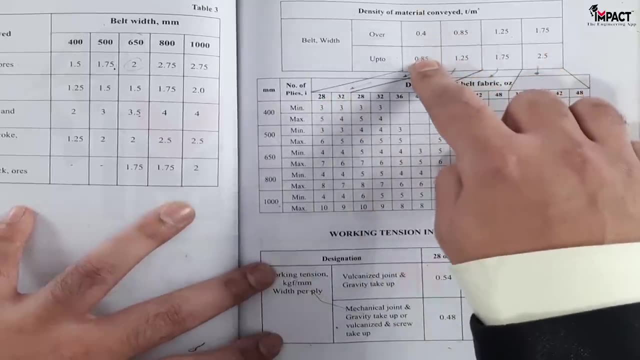 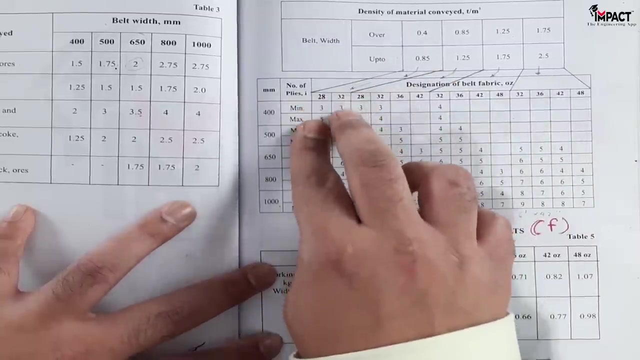 is there on this column and inside this table. here we have the density of the material being conveyed. So we have to draw the lines like, for example, there is first column, So connect the first column in this way with the two columns over here. Next the second column is connected. 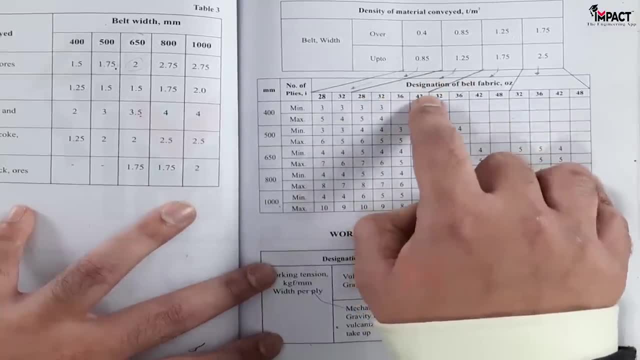 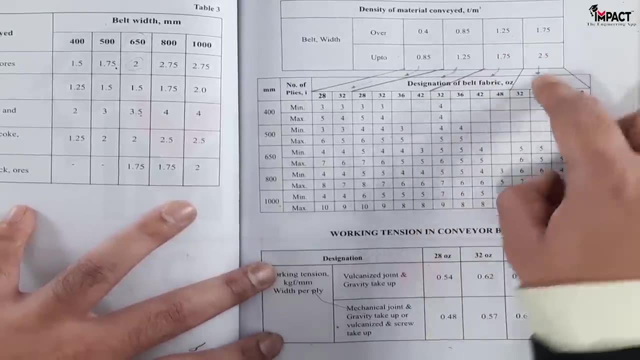 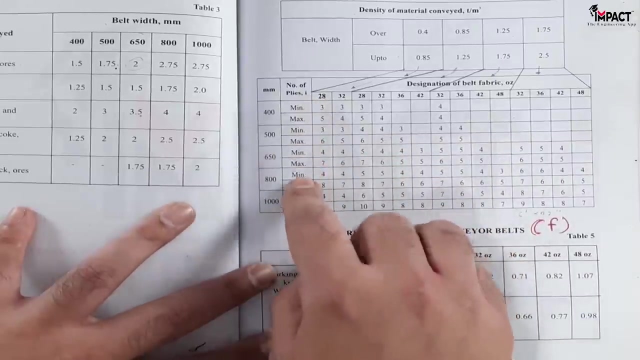 in this way up to the remaining four values. Next, the next two columns are connected with the remaining four values and finally the last one. So, with the help of pencil, you all can make these connections. Now, how to select the value? see, first of all, the width is 800 mm for us, and these are the 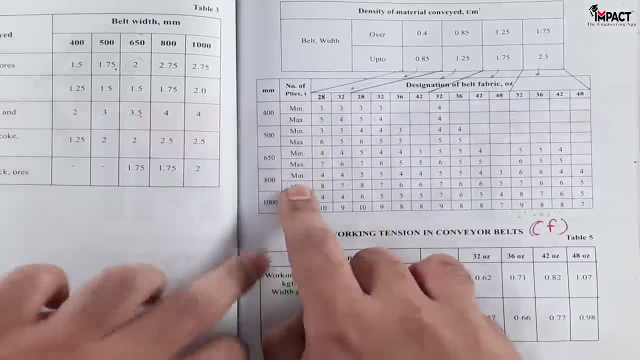 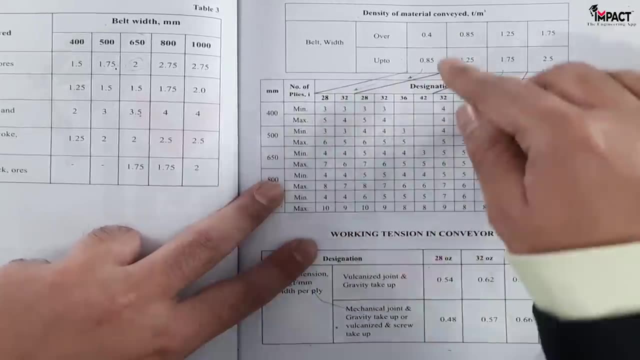 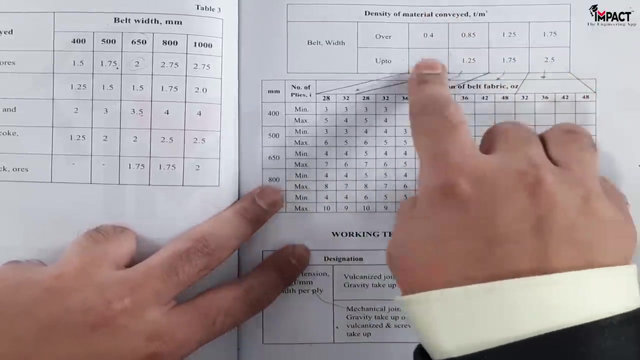 minimum number of plies. i is the minimum number of plies, so in this 800 we have to check. now the range is the density which we have. how to start this? first of all, the width has been selected. it is 800. so this is the row, now to decide which column we have to go into. 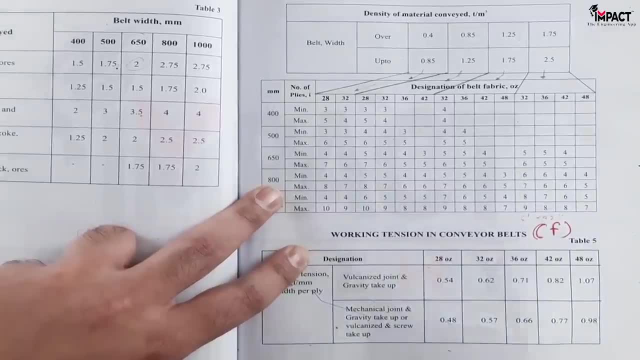 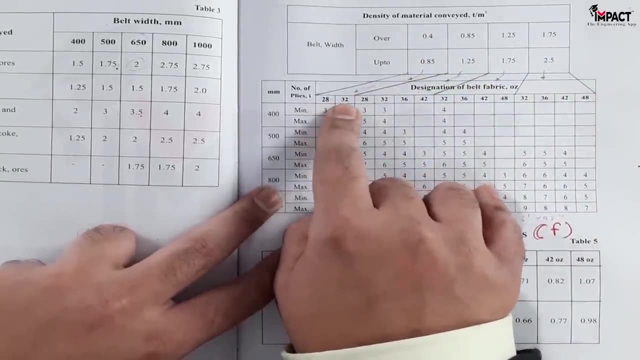 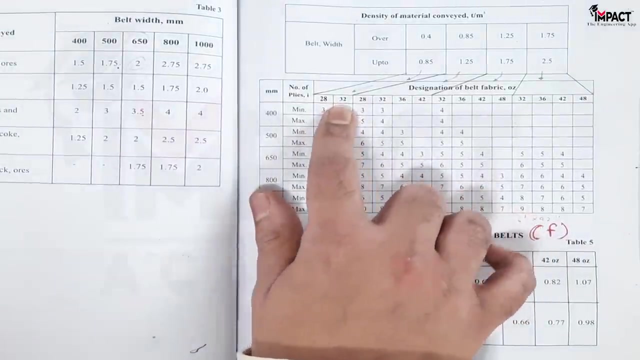 check for the density. the density of the conveyed material is 0.715 tons per meter cube. it is in this first range. so, first column. now we have two values, 28 and 32. these are called as o's, that it is the designation of the belt fabric o's value if it goes on increasing. 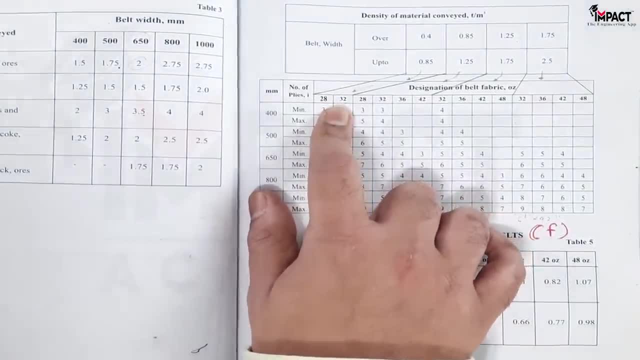 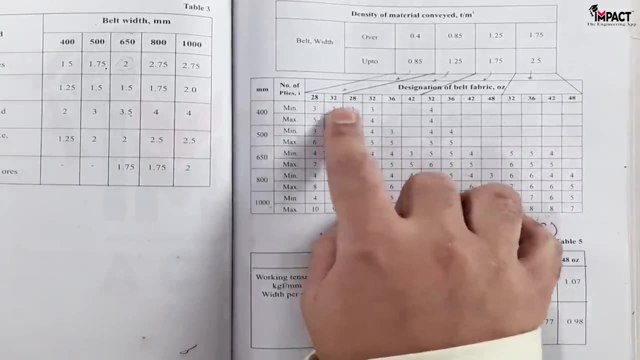 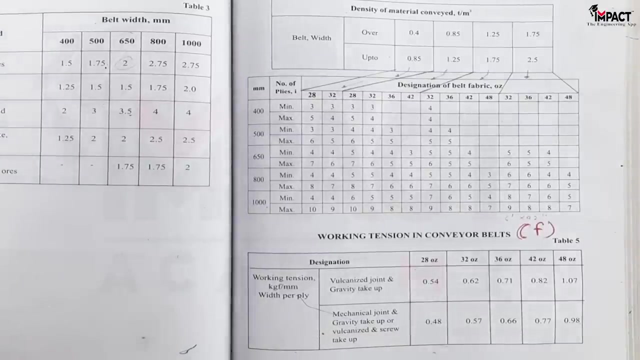 it means the weight of the belt is going on increasing. and if the weight increases, in that case the life of the belt will go on increasing. it means if the o's value is going on increasing, then the thickness of the belt will also go on increasing. and finally, if the thickness 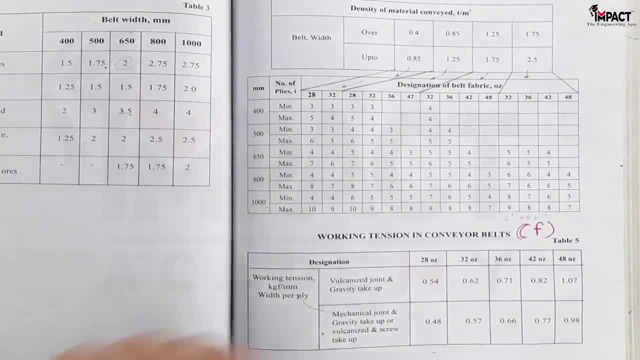 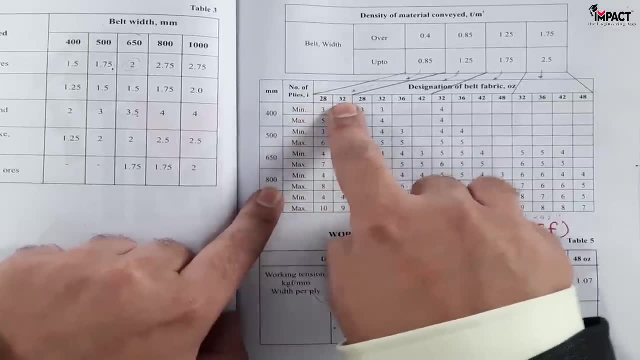 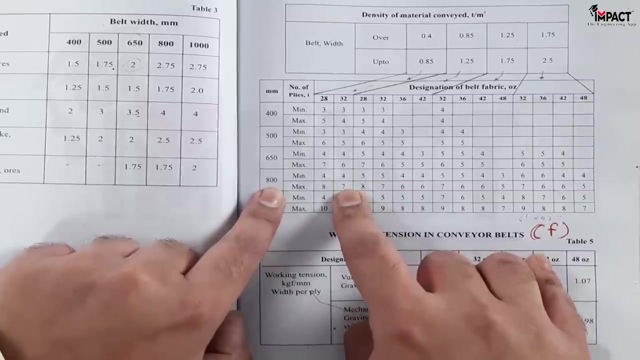 increases, then the life of the belt will go on increasing. so when we have selected 800 as the width, out of 28 and 32, we have two options: go for 32, higher value, always higher value. next, in this reach up to the value of here, we have 800 and the minimum plies are: 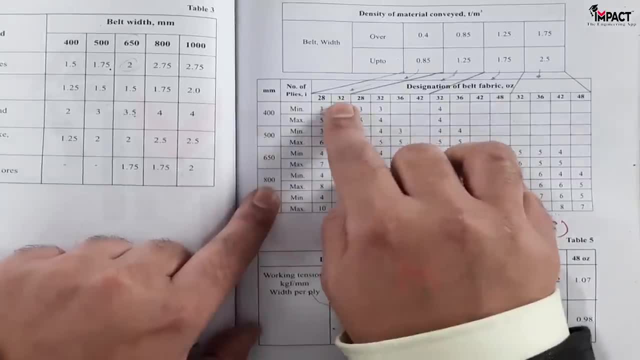 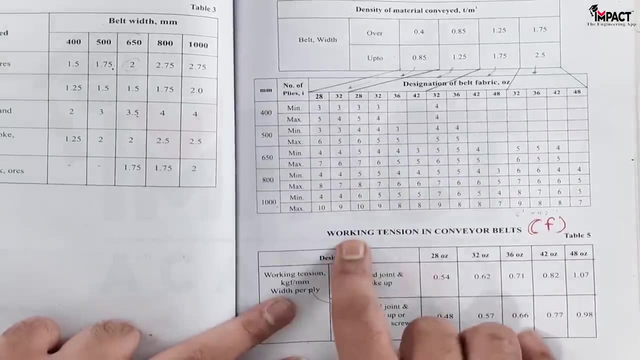 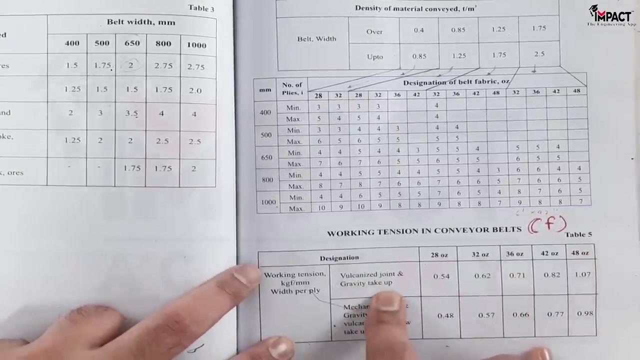 4. so first I'll explain how to get the plies and just before that we have: this value is 32 o's, so we are going for the F value, small f value. so this is the working tension in the conveyor belt. write it as small f. and for 32 o's we have vulcanized joint and gravity. take up: 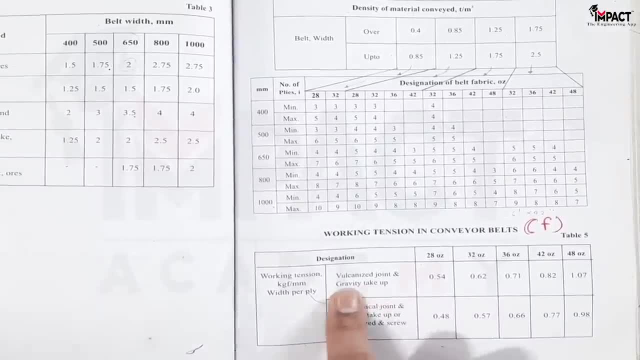 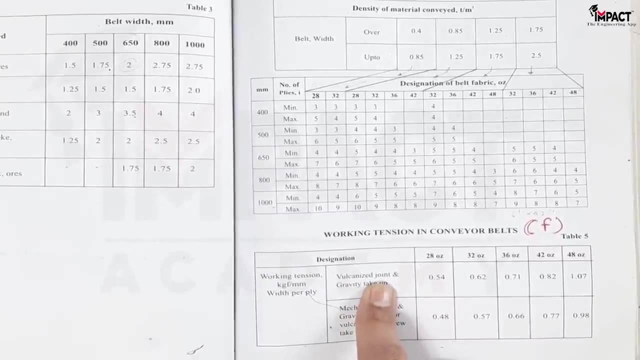 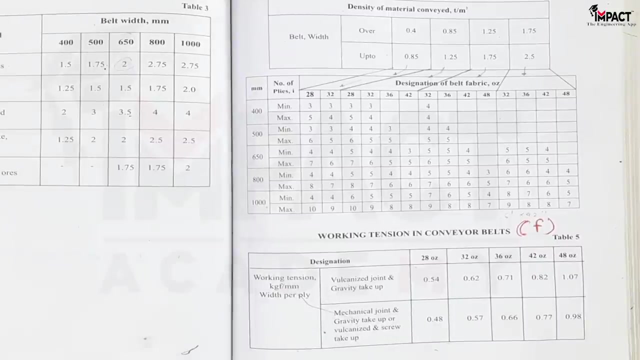 so we have to assume that here, in this case, it is a gravity take up, that is, the tensioning has been adjusted with the help of gravity take up and vulcanized joint means. the method of connecting the belt is: either we can connect it with the help of bolts, because belt won't be in a single piece. 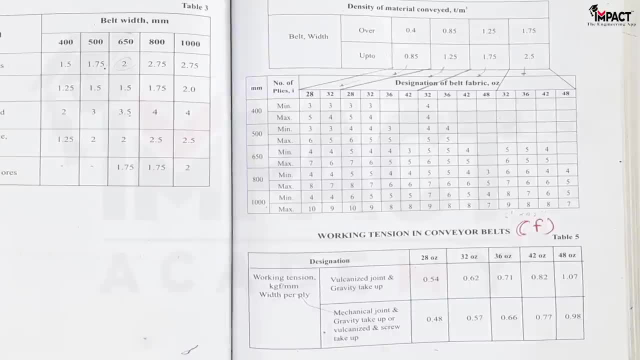 like, for example, if we have to transfer the material up to 50 meter length, as in this case, in this problem, then there won't be a 50 meter belt in a single piece. we have to use different sections or different lengths of the belt and connect them. so the connection method is either: 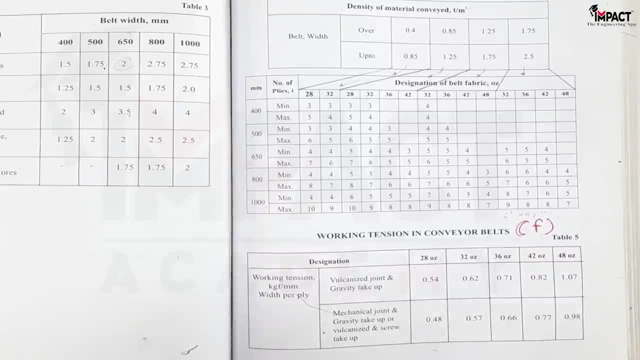 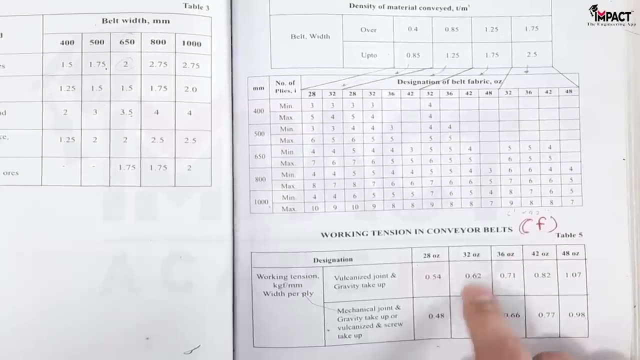 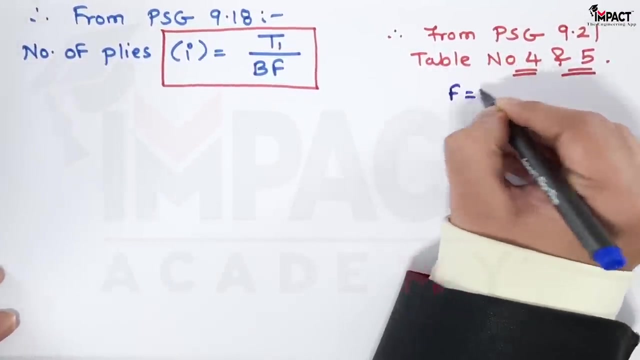 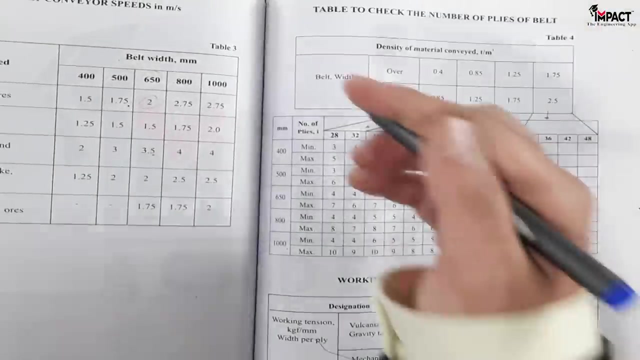 by belting or we can vulcanize the belt throughout, as mentioned here, and take the value of 32 o's. so the value is 0.62 of small f, as we can see here. so therefore, from table 4 and 5 we get small f as 0.62 again. i'll explain how to get the values. first go for the density. 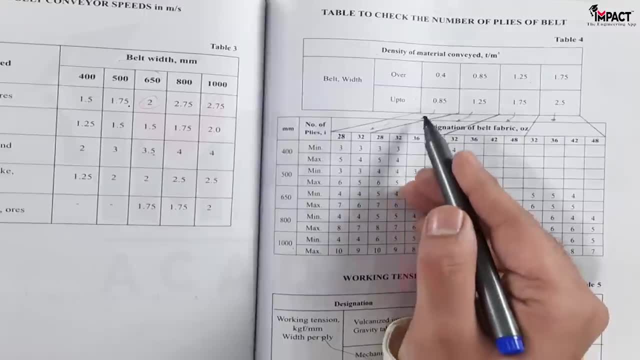 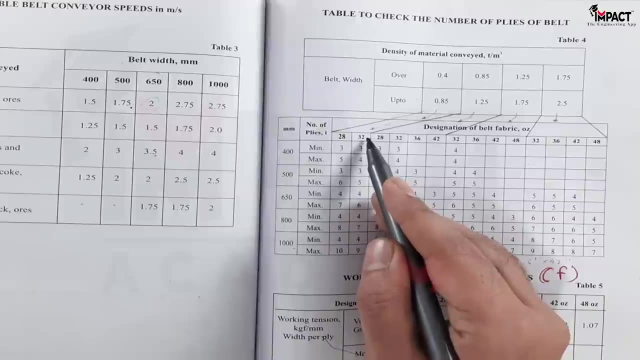 decide which column we are in and from that column here we can see the directions and out of the two o's values select the higher value and we have to reach up till here, that is 32, and then go into this table 5 for 32 o's and vulcanize joint. the value comes out to be: 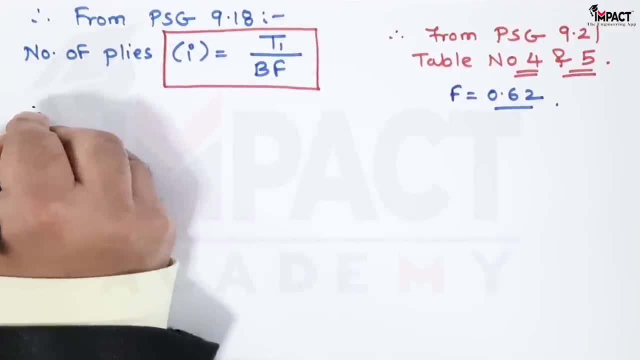 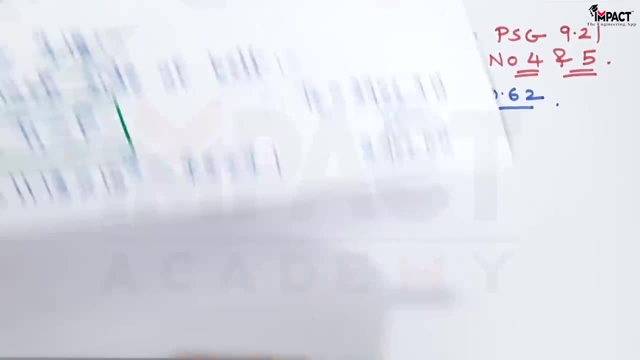 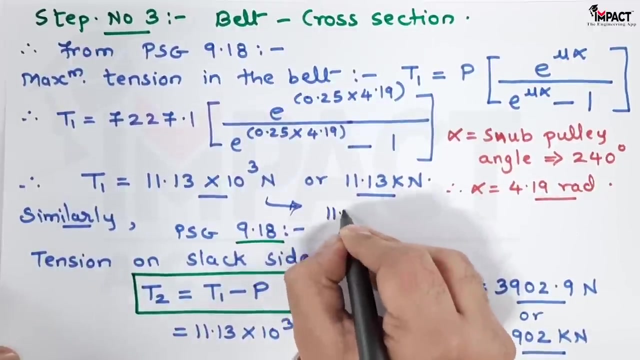 0.62. now, therefore, the number of plies would be: this: t1 should be kept in terms of kgf. in terms of newton, the value is 11.13. 10 raise to 3 newton, so that would be 11.13 into dividing by. 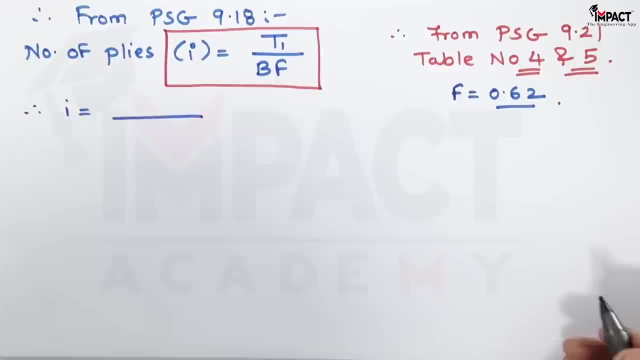 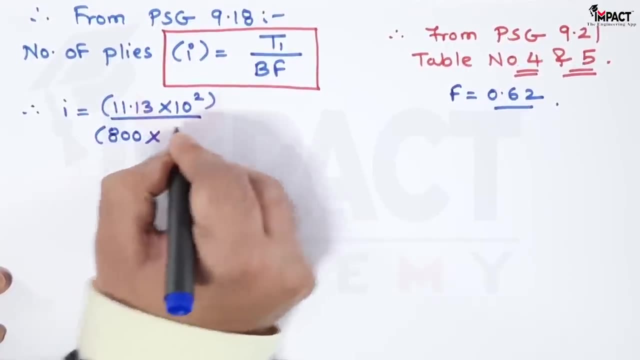 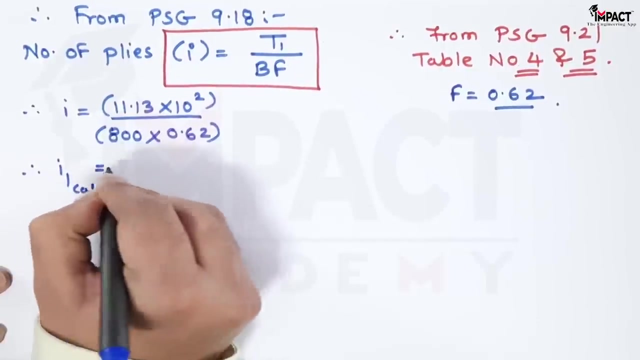 10, 10 raise to 2 kgf. then the width of the belt, capital b in terms of mm. 800, mm small f is 0.62. so therefore i calculated is 2.24. so we have to check if the number of plies are greater than or less than this calculated. 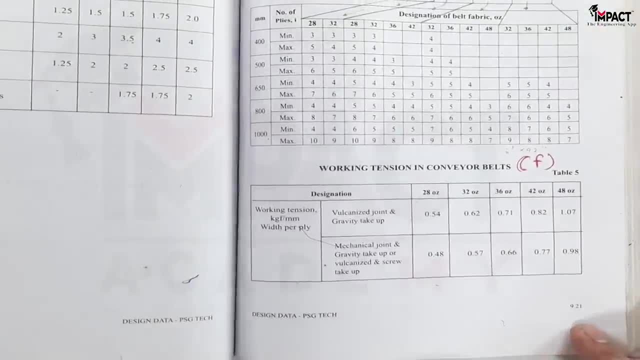 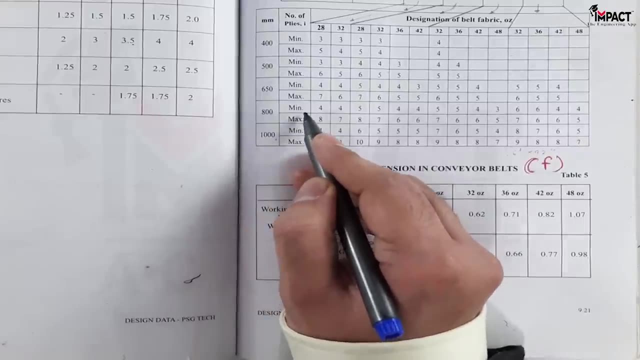 value for that, going into the same psg 9.21. and in this table here minimum number of plies are given: ้a. And hope you liked this video. give a likefte, a like and attach comment below for 800, the minimum number of p promise and the minimum number of liked and present. 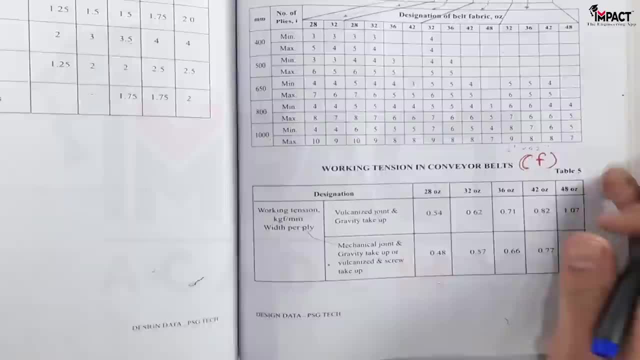 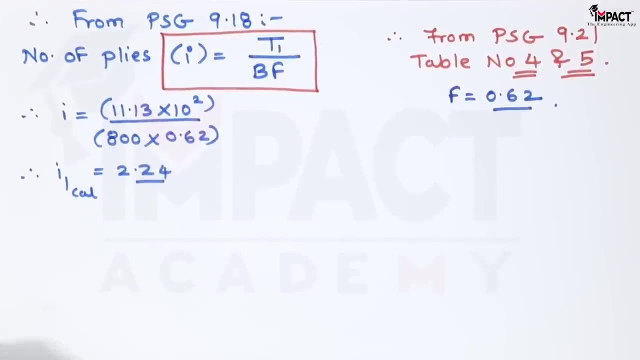 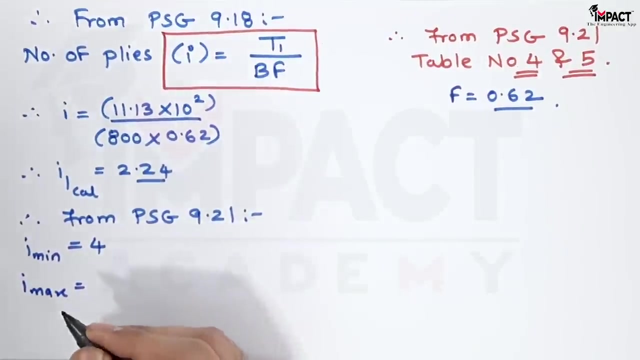 it is 4 and the calculated value is 2.24. So it means minimum number of p should be for 32 o's, Therefore from PSG 9.21. the minimum number of place are four and the maximum number of flies are also given in the tool year maximum. 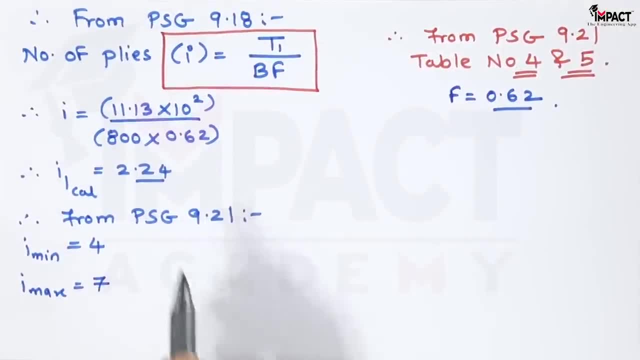 plies are 7.. Now if suppose the calculated value would have been greater than the maximum value, that is, if suppose this would have been 8, then we would have taken the maximum value as 7, but since this value is less than minimum, so we have to start with the minimum value. 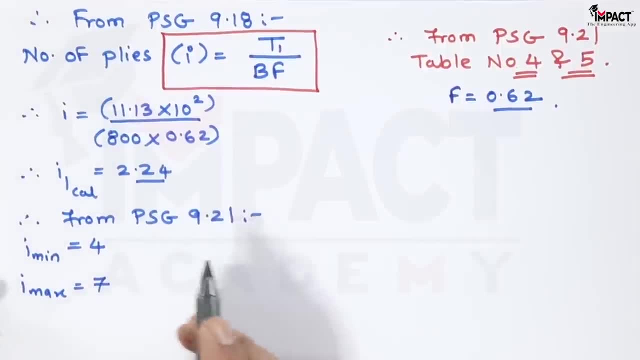 which is 4.. So now the number of plies are fixed. the number of plies: we are going to take it as 4.. Maximum is to be taken if this value exceeds the maximum value, if it is 8,, 9,, 10. 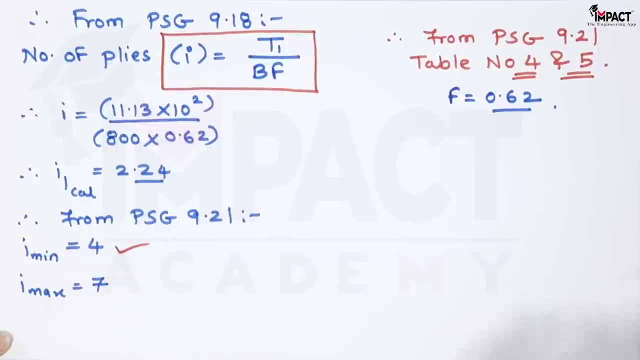 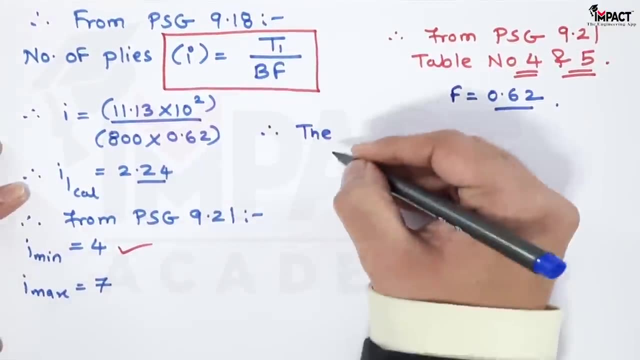 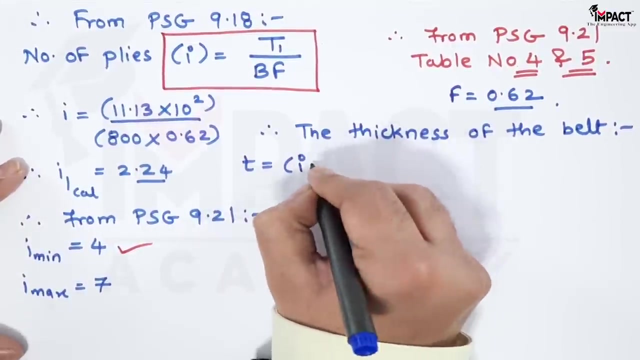 then we have to take the value as 7 as the number of plies and then do the further calculation. Now, therefore, I will write: the thickness of the belt is given by once the number of plies are decided. it is I that is the number of plies into 1 mm, which is the thickness of each ply. 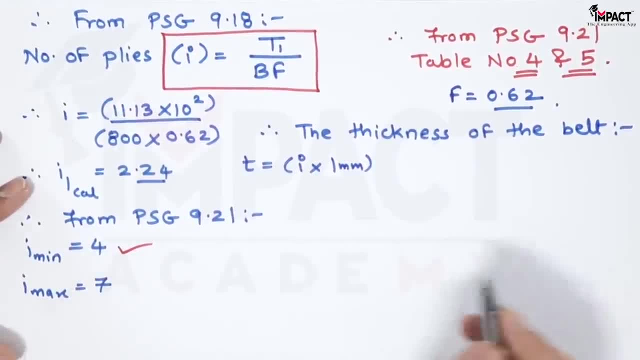 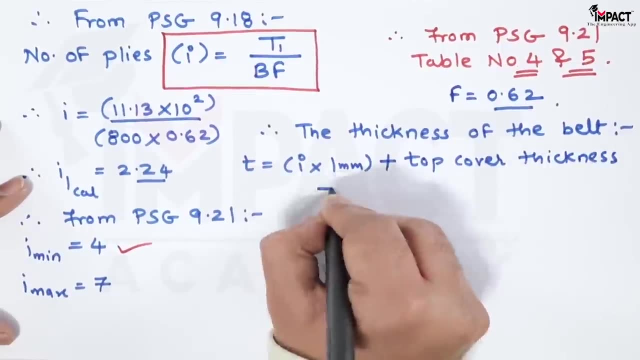 like, for example, we have 4 plies or 4 layers, so each layer would having would be having a thickness of 1 mm, which is the thickness of each ply. So this is the thickness of each ply, which is the thickness of 1 mm plus. So this is the formula to get the thickness of belt. 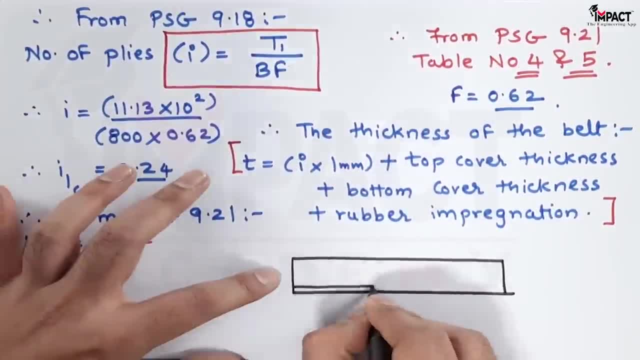 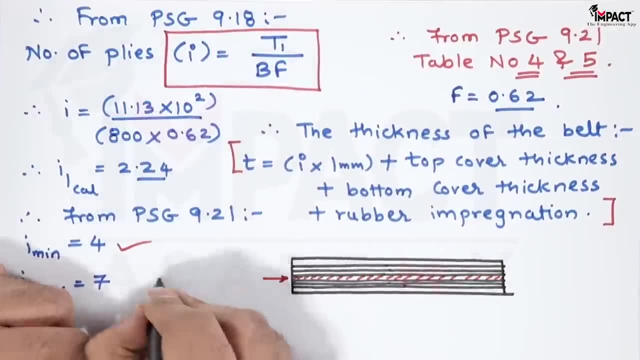 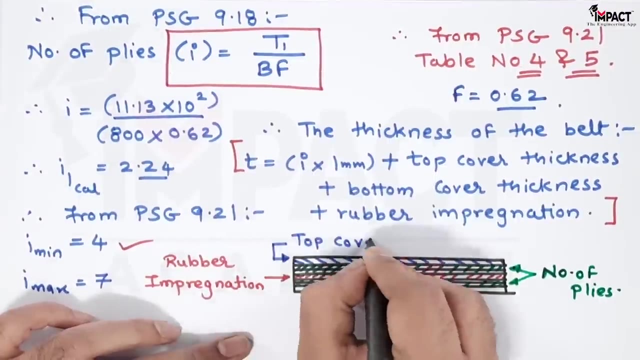 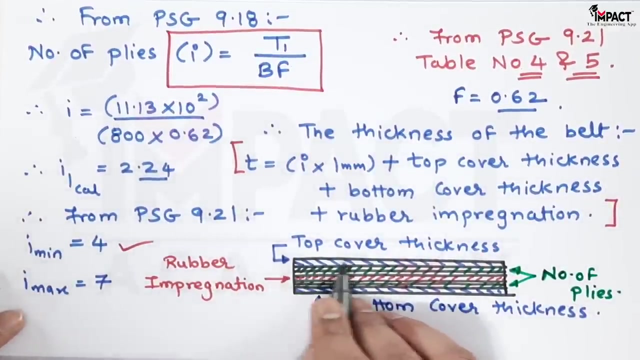 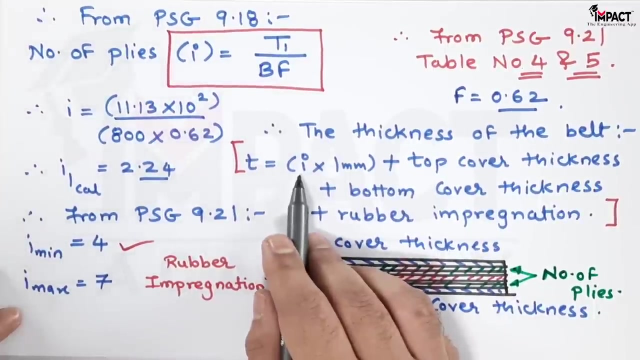 I. So this is the cross section of the bed. here we have top cover. thickness in between these green section which I have shown. these are the four plies, I having thickness of one mm each. now in the red which I have shown, that is the rubber impregnation. and then we have 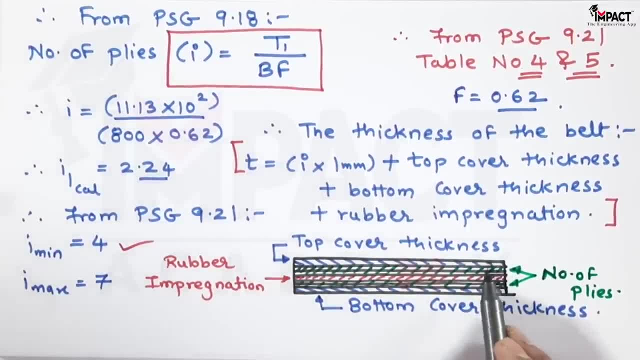 the top cover thickness and bottom cover thickness. at the top, since the material is being conveyed, we should have a greater thickness compared to the bottom cover thickness. I am writing the values, so T is equal to I is the minimum number of plies, which are four each plies. 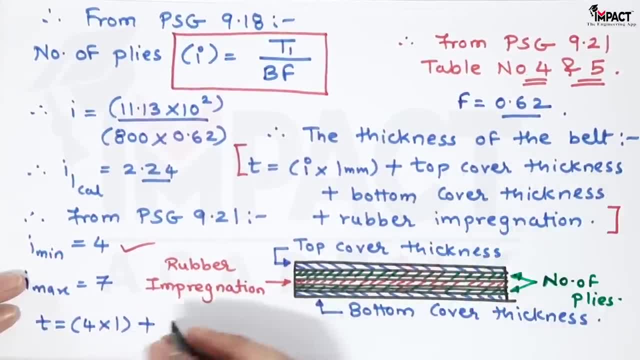 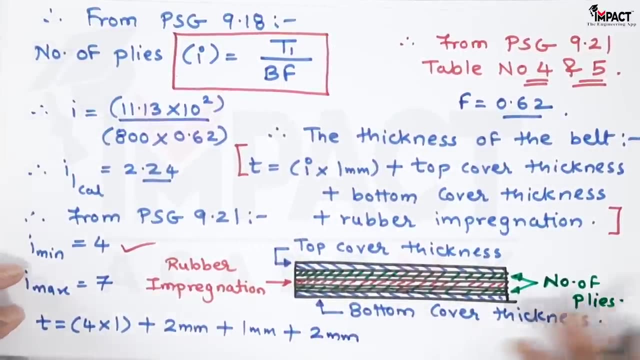 having a thickness of one mm plus top cover thickness should be taken as two mm plus bottom cover thickness should be taken as one mm and the rubber impregnation should be taken as two mm. and why the thickness is less at the bottom cover? because that is in, not in. 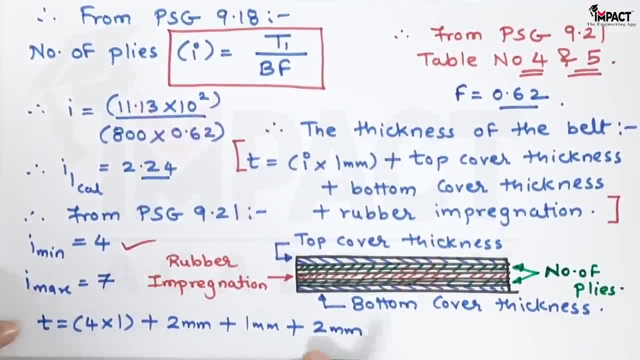 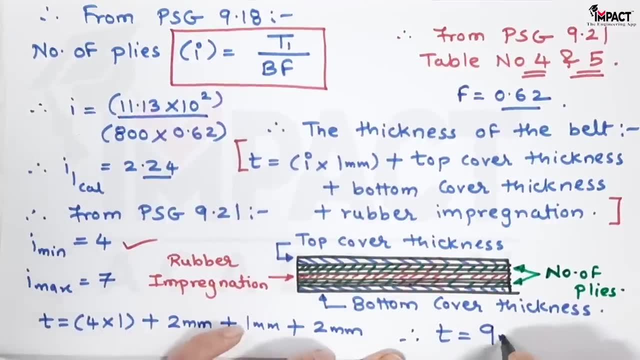 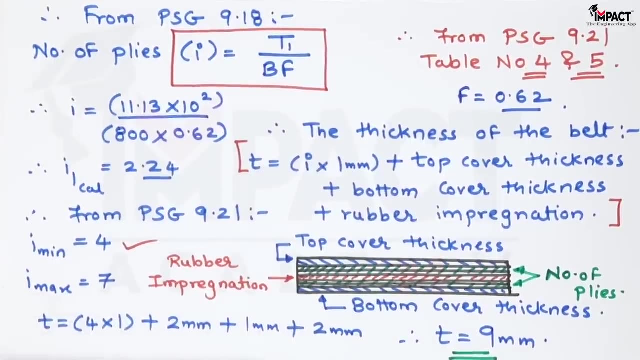 contact with the conveyed material. so that is why the thickness is less. and finally, after calculating this, T comes out to be nine mm. so in the belt cross section part, we have found the thickness of belt, and even the width is there with us, which is 800 mm. previously we have found out: 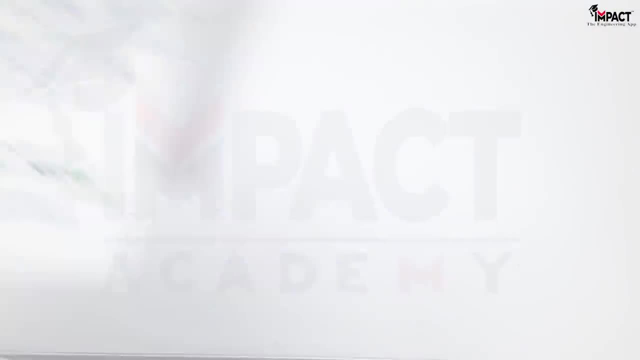 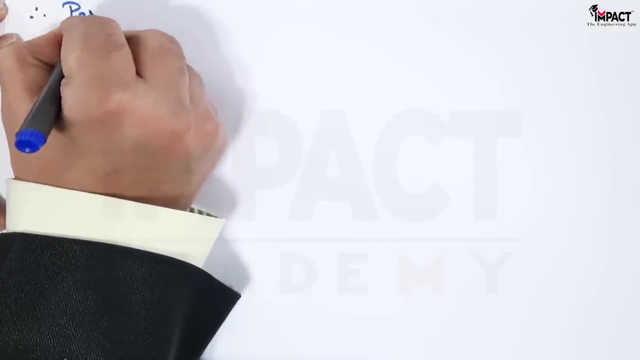 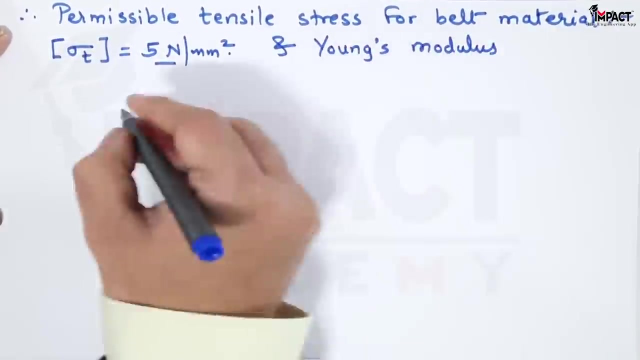 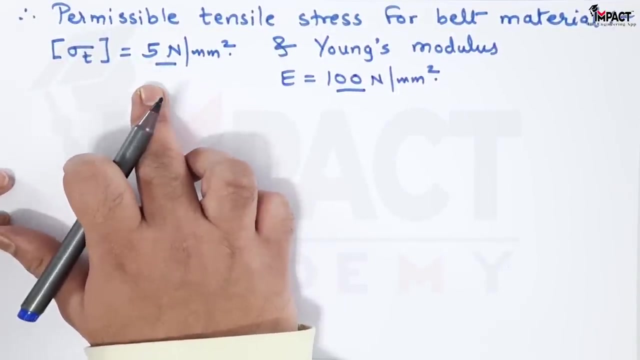 now we have to check the belt if it can resist the required stresses. so therefore I will write down the permissible now, these two values we have to remember. that is, the permissible tensile stress for the belt material is five Newton per mm square, whereas the young's modulus. 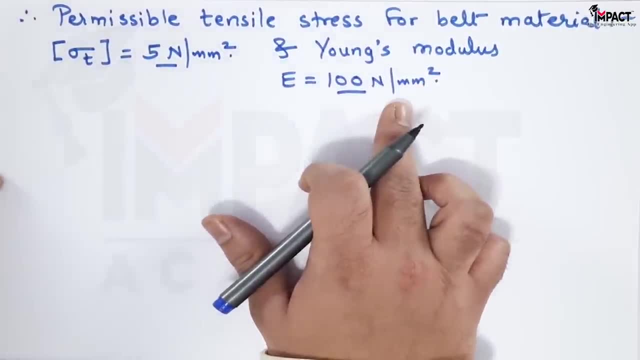 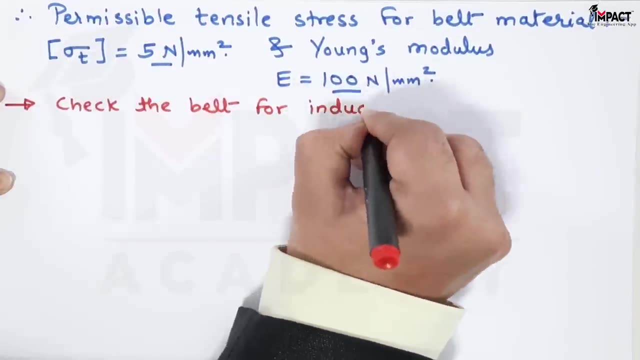 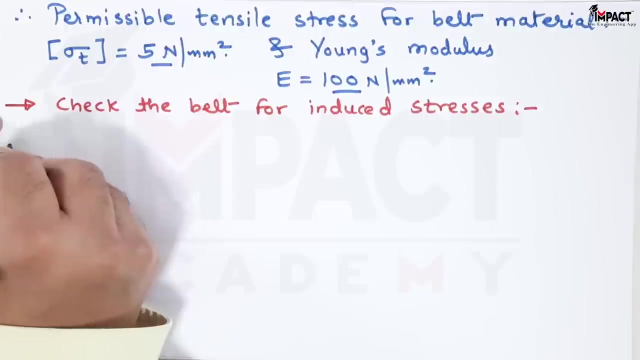 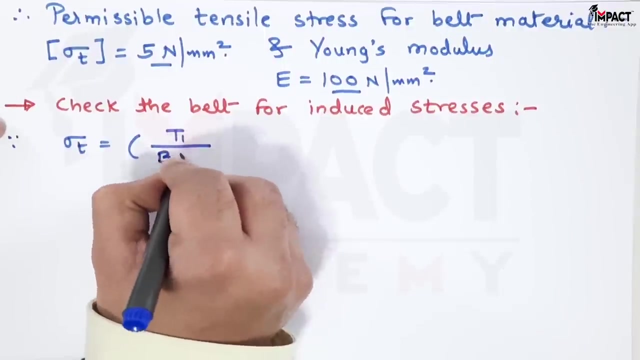 or the modulus of elasticity is hundred Newton per mm square. now we have to check the belt for the induced stresses, Hm, and for that first. the total tensile stress induced is given by T one, that is the maximum tension, or tension in the tight side upon the cross section that 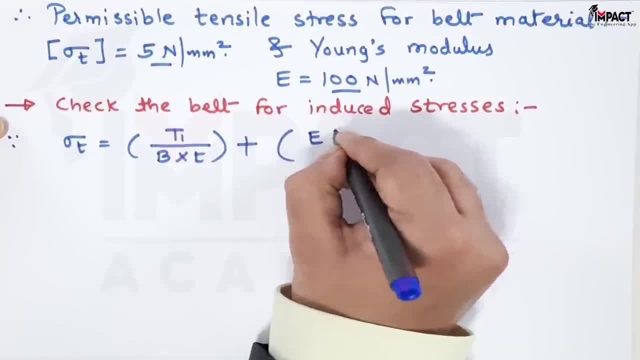 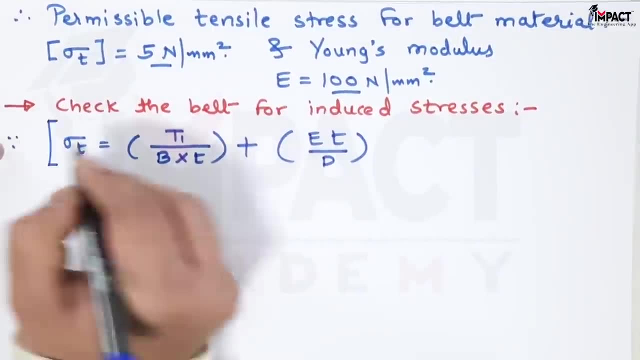 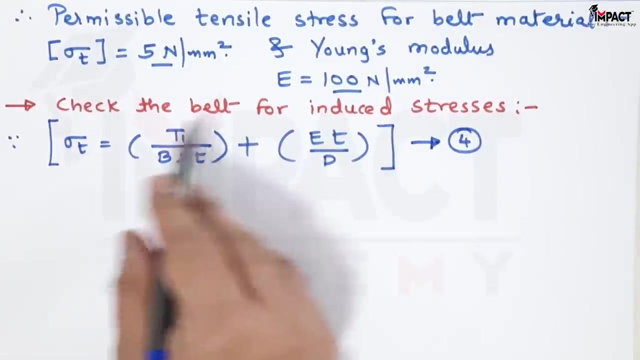 is V into T plus young's modulus into the thickness of the belt divided by the diameter of the pulley. So I'm keeping it as equation 4.. So first term. Now in equation 4 all the values are known, except D, which is the diameter of the driver. 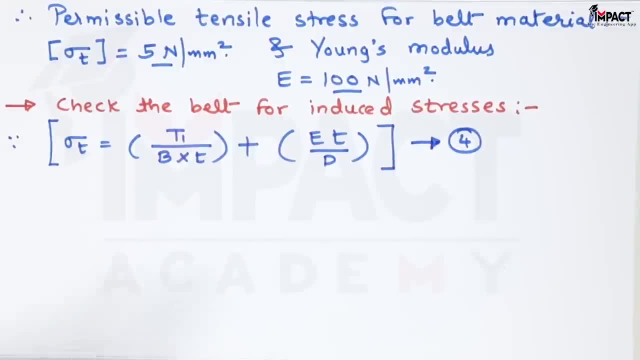 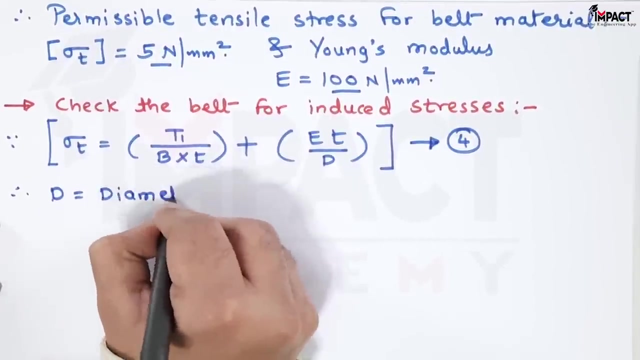 pulley and here driver and driven pulley. both are going to have the same dimensions because we don't want any kind of speed variation in the driver and driven pulley. So therefore D is the diameter of both driver and driven pulley in terms of mm. and for that 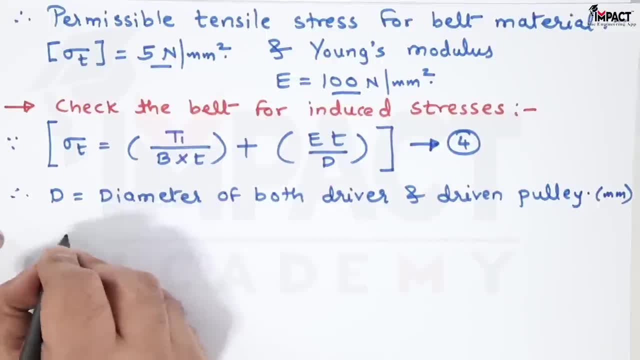 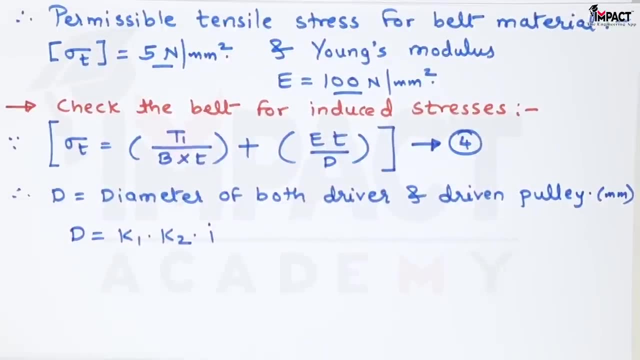 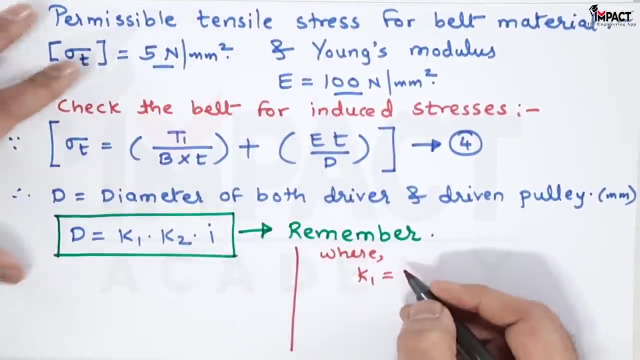 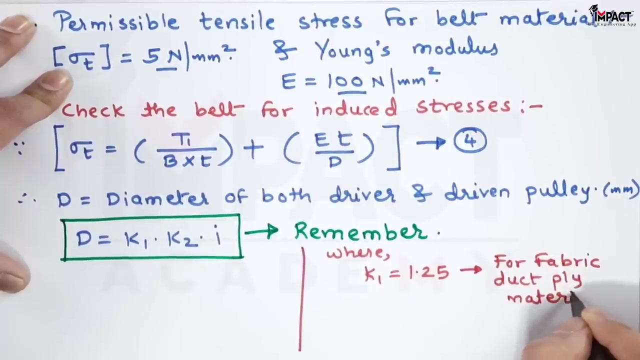 I am giving a quick formula of the diameter, which is K1, into K2 multiplied by I. This formula, we have to remember, where the value of K1 is equal to K2 multiplied by I, K2, 1.25. this is for the fabric, duct, ply, material of the belt. then K2 is equal to the value. 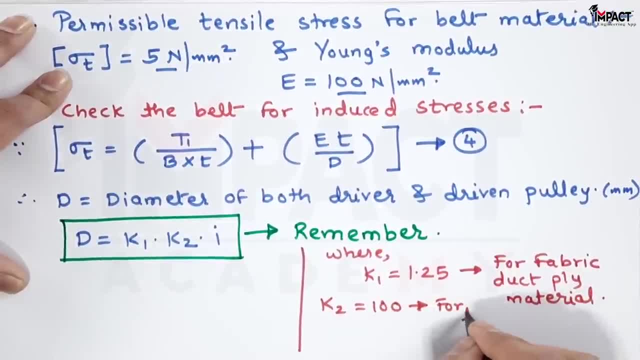 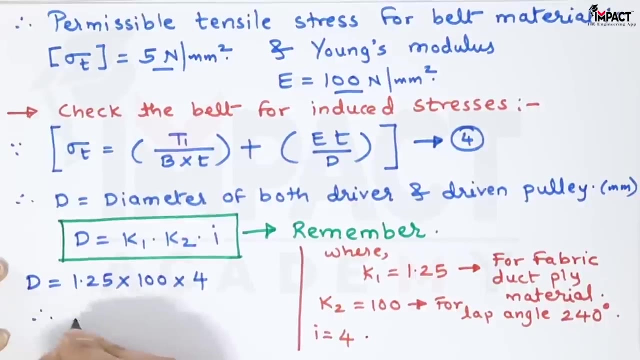 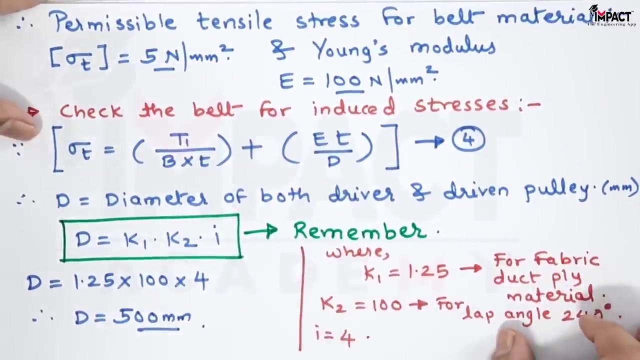 is 100 for lap angle: 240 degree, which is the snap pulley angle, and then I is the minimum number of plies, which is 4.. So putting these values to get the diameter, Then the answer is 500 mm. now, selecting the standard diameter for the driver and driven, 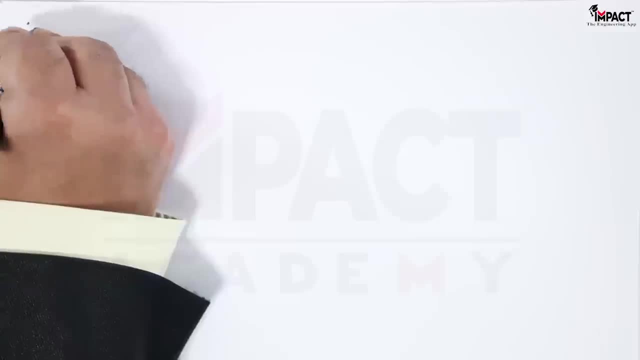 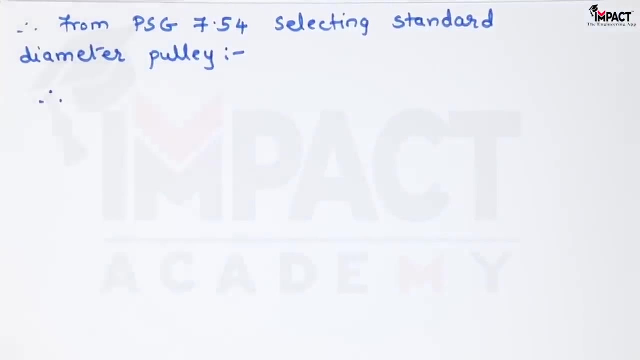 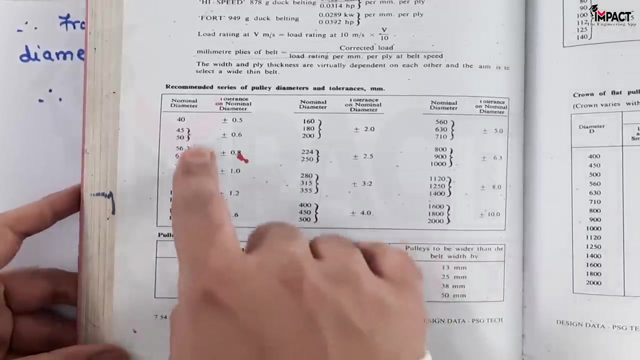 pulley. so therefore, using the reference, So from PSG 7.54, here on PSG 7.54, we have this table which gives us the value of standard pulley diameter. it is given as nominal diameter. The value which we have, It is 5.54.. 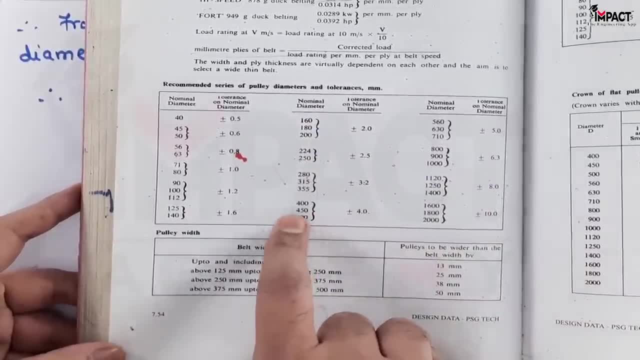 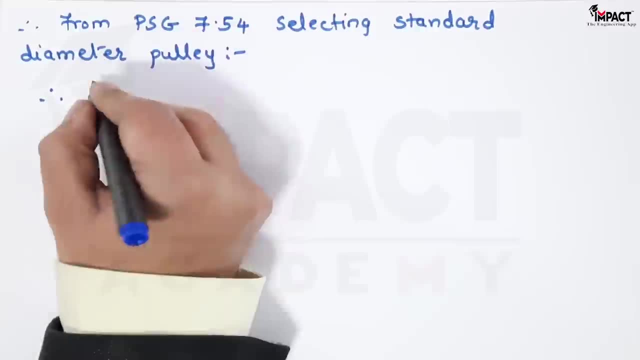 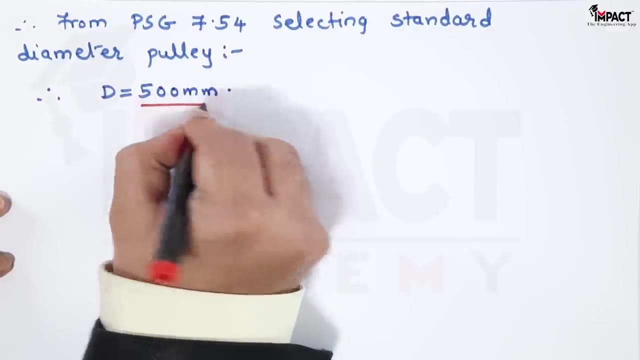 500, and here we can see exactly 500 mm diameter pulley is available, So the value is 500. I can write it as it is. So the D is finalized- the diameter of pulley. Now, once the diameter of pulley is known, I can put all values in equation 4.. 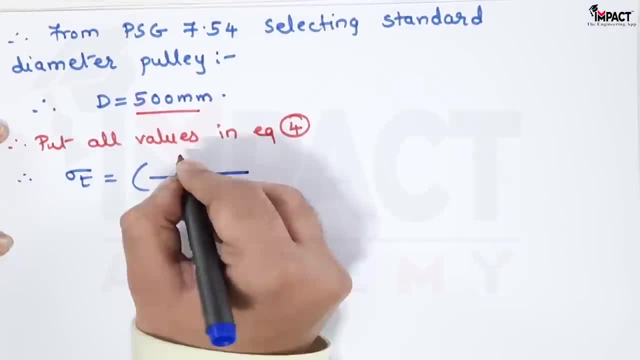 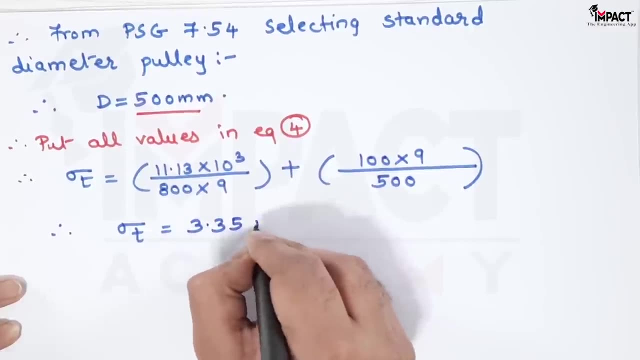 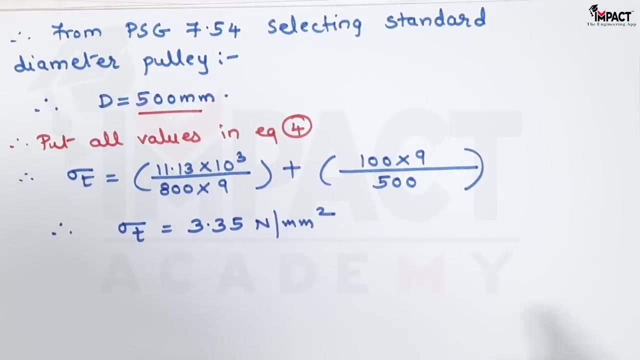 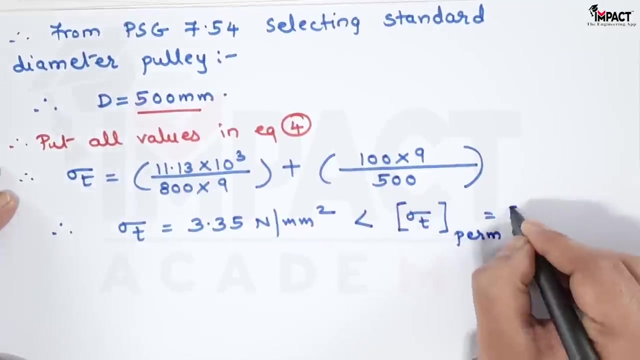 So therefore, The tensile stress value is 3.35 Newton per mm square, So comparing it with the permissible tensile stress, which is 5.. So this value is less than the permissible value, which is 5 Newton per mm square. So therefore, the belt is safe under tension. 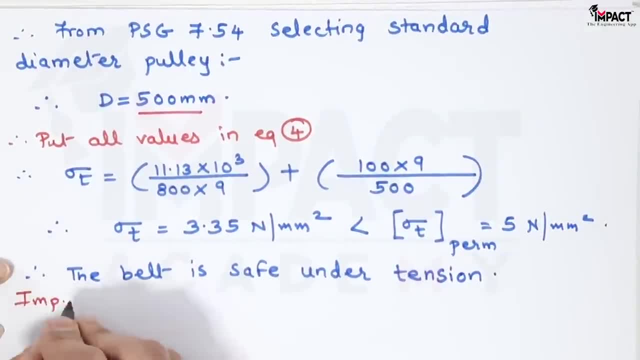 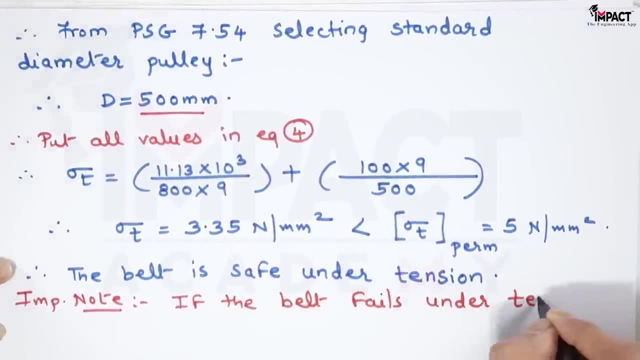 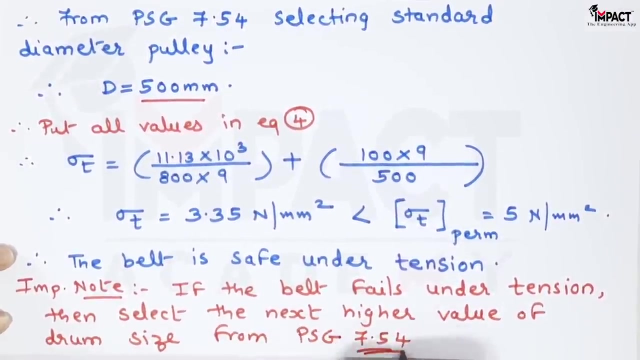 And here also I am giving an important note, that if Now, if the stress would have been greater than five, then what we have to do if the belt fails, Then Select. So here is this hint, that if the value of stress would have been greater than five, again, 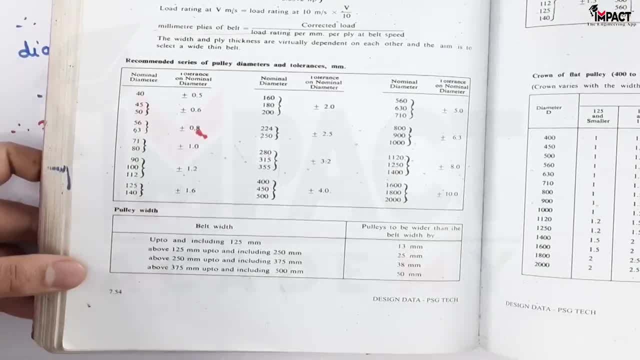 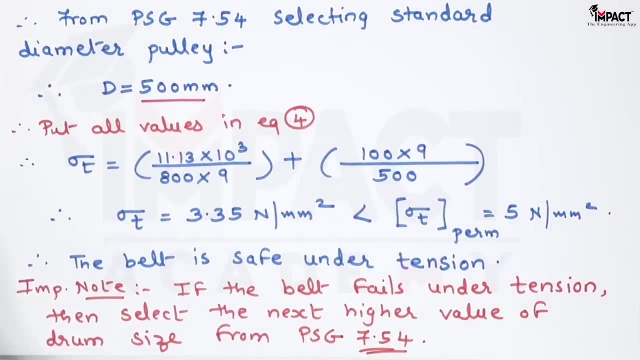 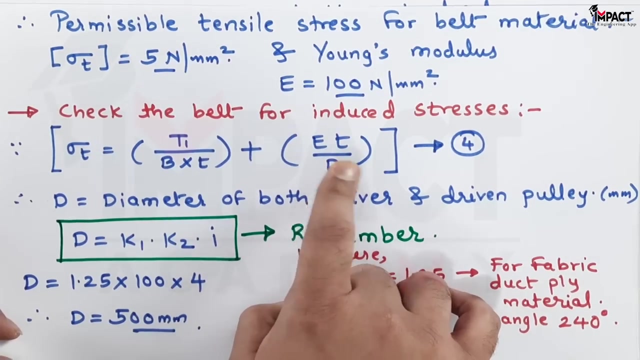 we have to go To PSG 7.54. And instead of 500 value, Select value, which is 560, and then check for the given stresses, because when we look at the stress formula, stress is inversely proportional to the diameter. so the moment we go on increasing. 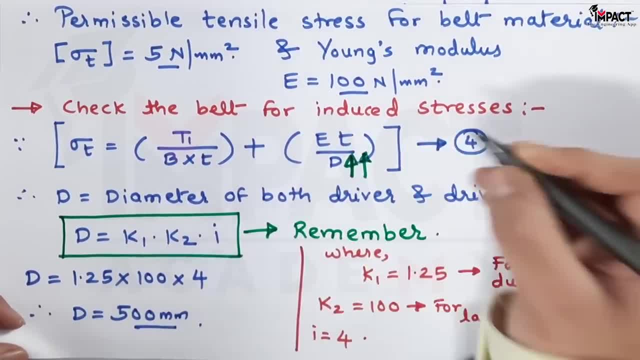 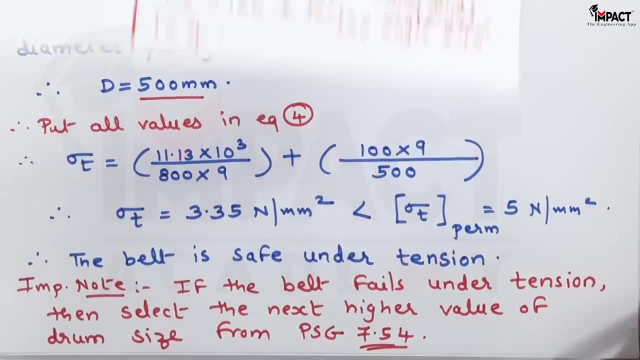 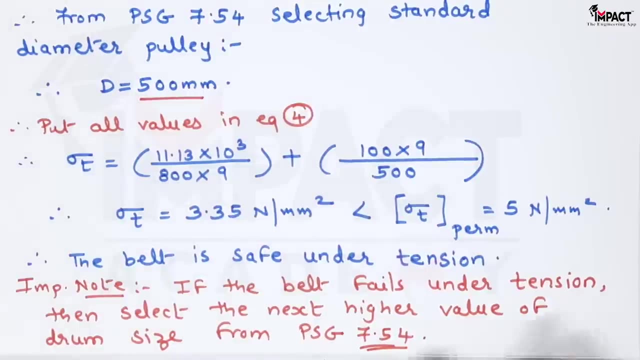 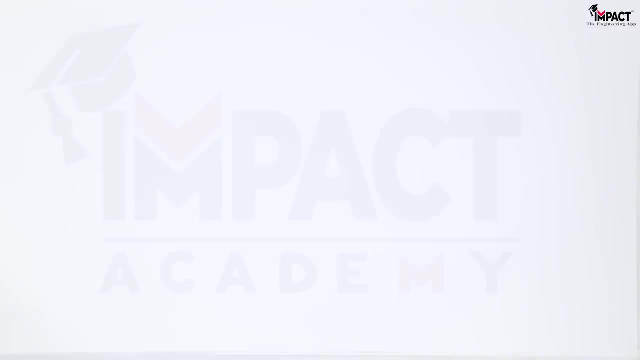 the diameter of the pulley, then the stress would be reduced considerably because they are in inverse proportion, and so now it is safe under tension. we have checked the belt. so that completes the step number three. now two steps are left. that is step number four, which is the design of drum, drum shaft and selection of bearing, and step number five. 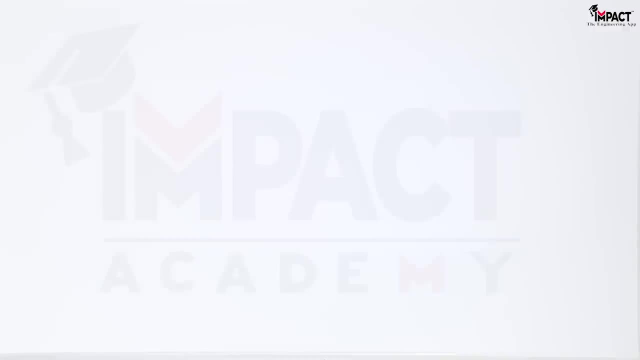 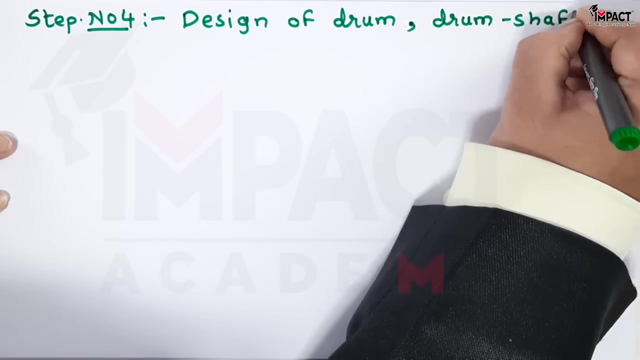 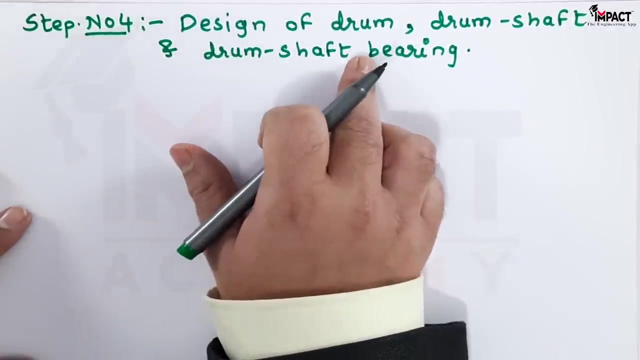 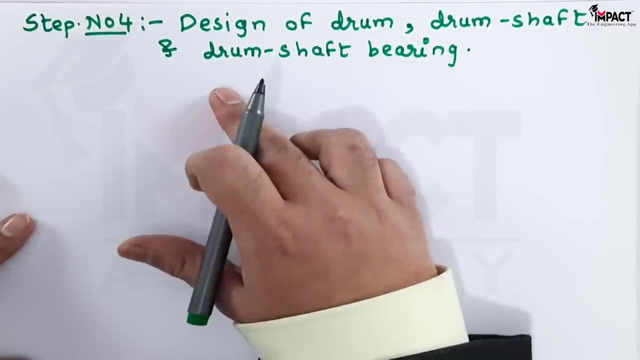 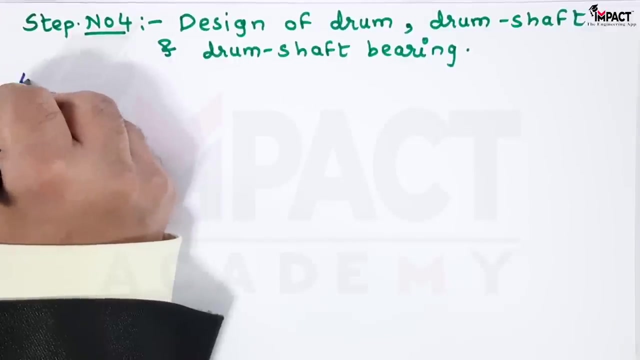 is the design of idlers. so starting with step number four. so here in step number four we have to design the drum already. the diameter of drum is there. with us we want the width of the drum, then drum shaft and the drum shaft bearing. so first is the cross section of the drum. 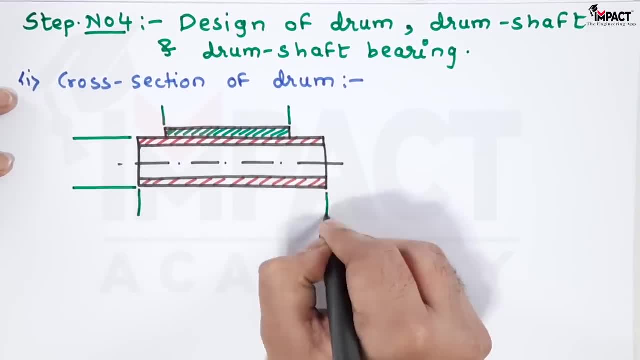 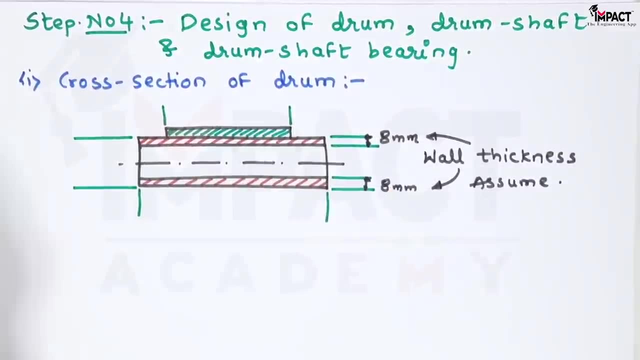 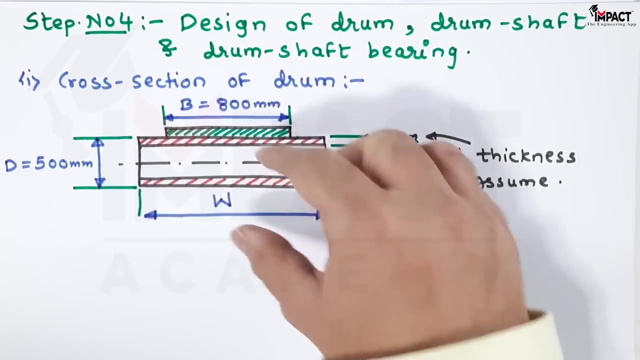 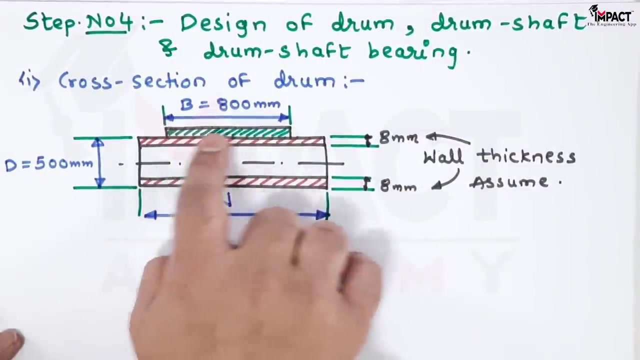 so here is the cross section of the drum. this is the driver pulley, or we can say even the driven pulley, because both are having the same dimensions over which the belt is mounted. belt is having a width of 800. that has been decided anymore. you can say in the differentalities you can see all three belts do not have the 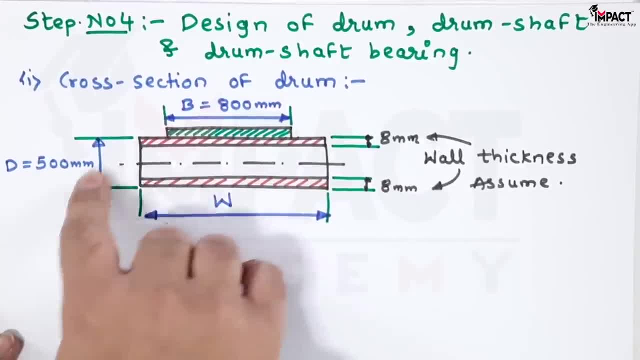 step number one. next, the drum is having a diameter of 500 mm. its thickness is assumed to be 8 mm, which is called as the wall thickness. now we have to find out how much is the width of the drum, leaving some amount of clearance. so therefore, 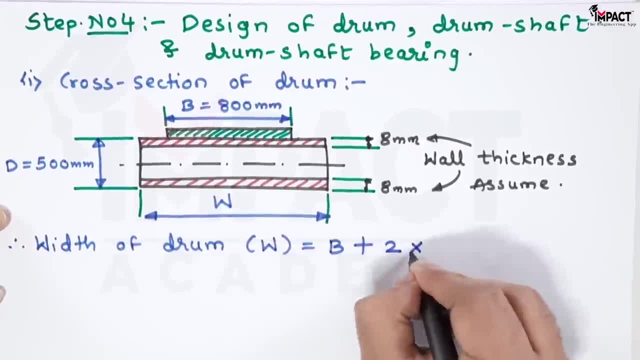 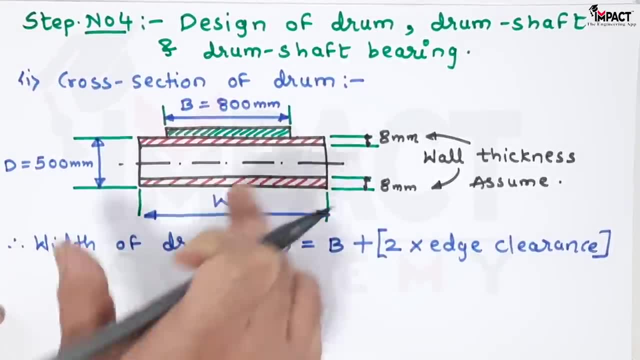 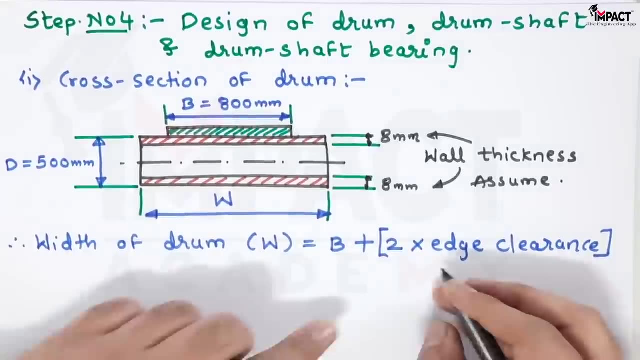 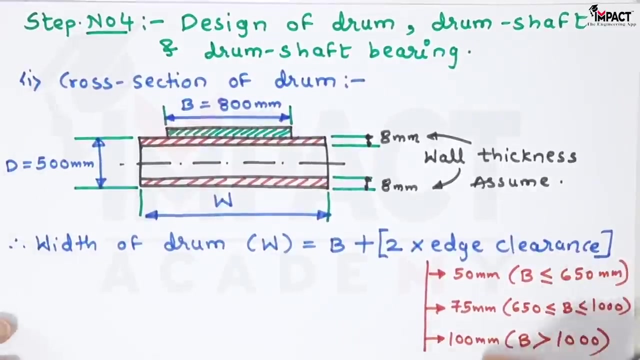 so the formula for the width of the belt is already we have. the width of the drum is already we have width of the belt plus 2 into edge clearance- how to get edge clearance. so these are the 3 values for the edge clearance, this depending. 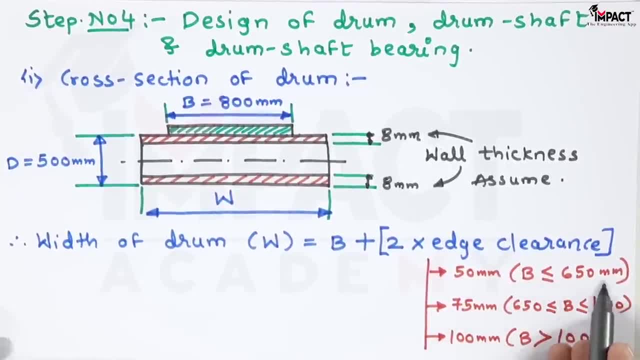 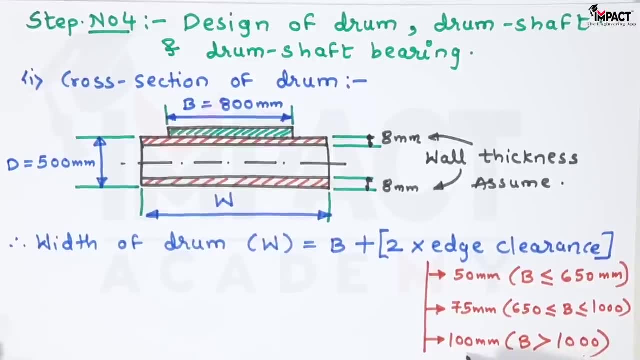 upon the width of the belt. if the width is less than equal to 650, we have to take edge clearance as 50. if the width is greater than 1000, to take a heat clearance of 100 mm. but since the width is 800 mm, it is in between this range, so therefore edge clearance has to be taken as 75 mm. 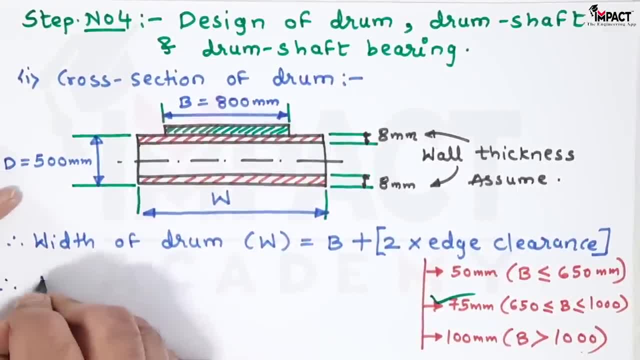 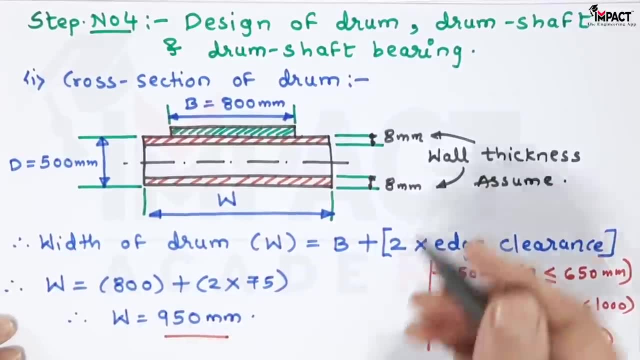 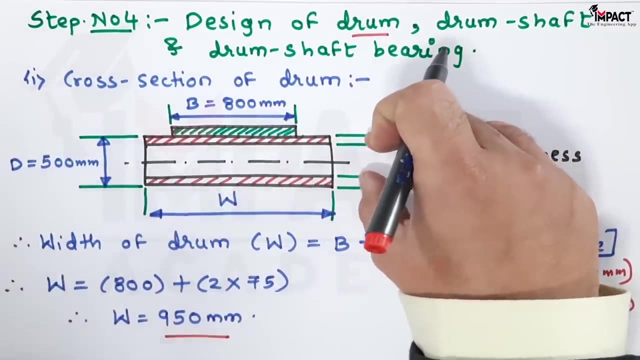 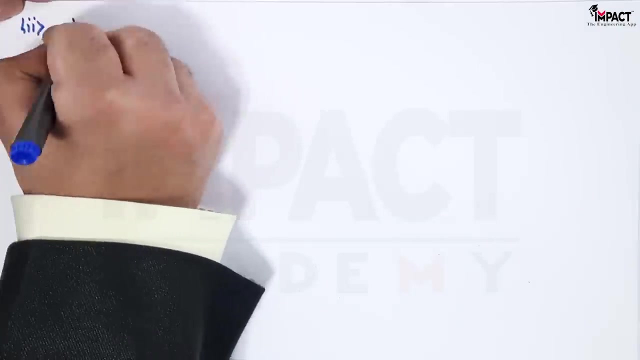 So, therefore, the width of the drum would become, which comes out to be 950 mm. So here the design of drum is completed. now going for the drum shaft, because this drum would be having a shaft in between. so, within this step, I will draw the diagram for the. 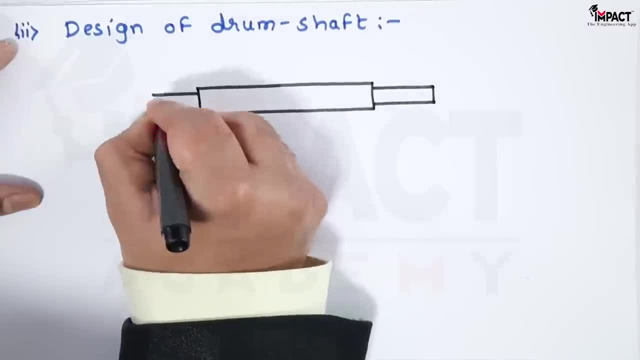 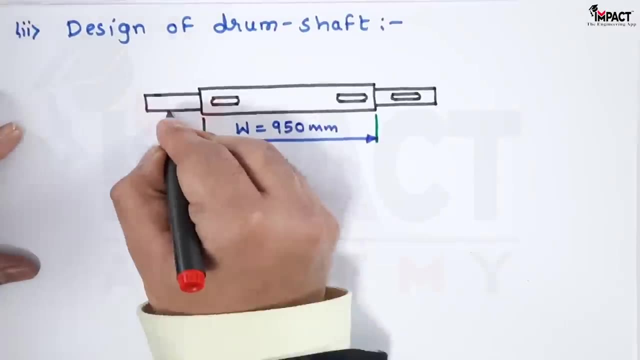 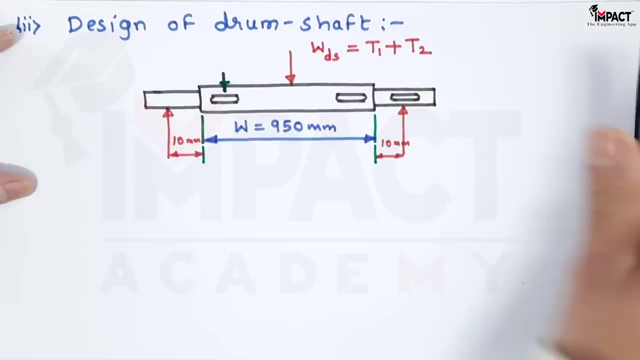 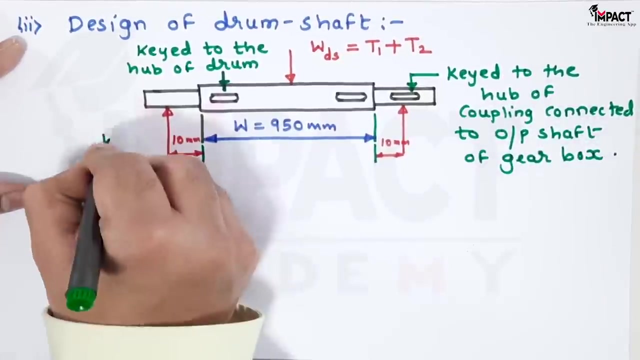 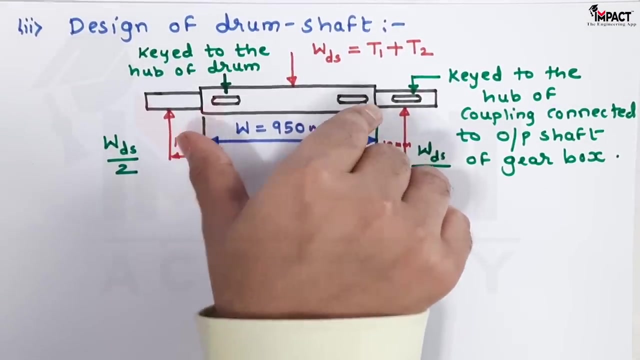 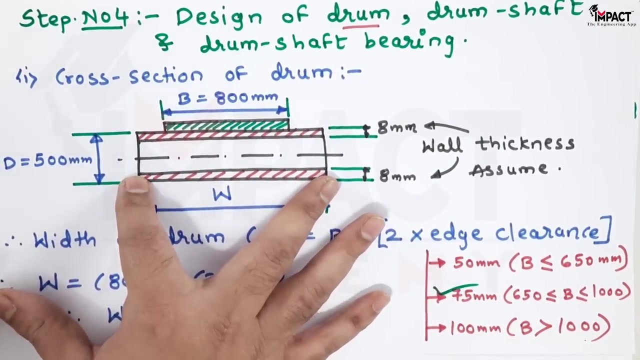 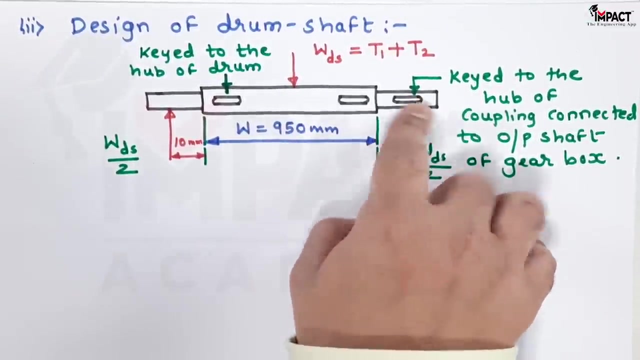 shaft. Now here is the diagram of the drum shaft. This drum shaft will fit into this drum because here, whatever is the width of this drum, exactly the same length of the shaft is there Now, extending 1010 mm on both sides, because here we have to extend the part. 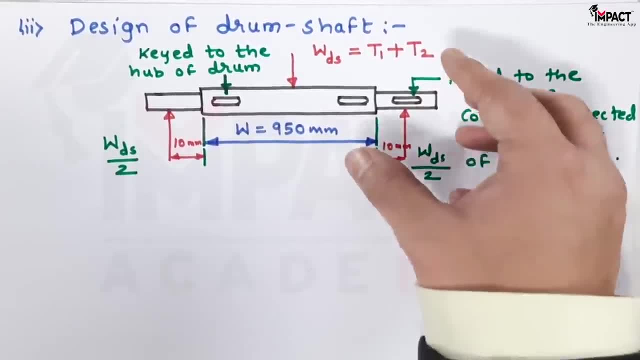 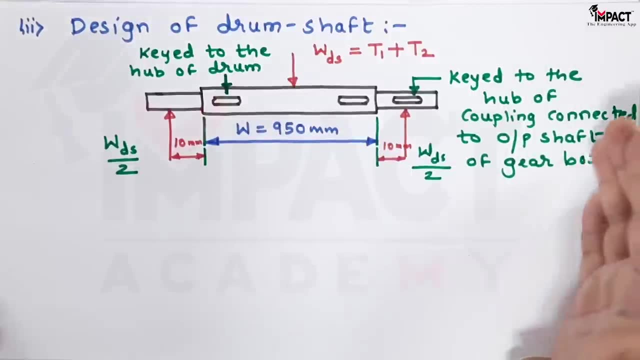 This end of the shaft is connected to or keyed to the coupling which is connected to the output shaft of the gearbox, because the arrangement is in such a way that we have a motor whose RPM is 1440 RPM already selected, So this RPM would be reduced by the help of the reduction gearbox to get the velocity. 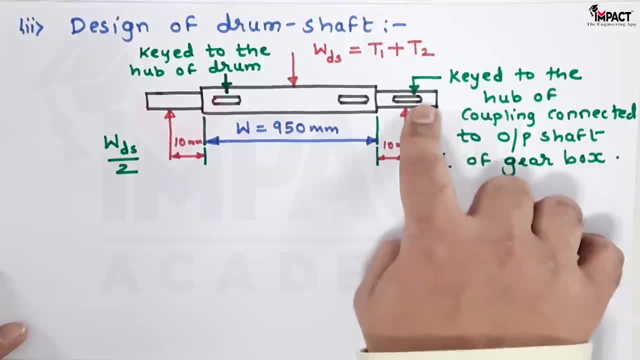 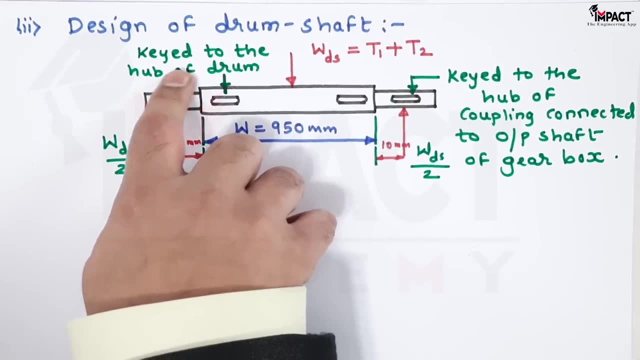 of belt as 1.35 meter per second. So output shaft of the gearbox would be connected over here. So the keyway is connected to the gearbox. Similarly, these keyways are, provided it would fit into the hub of the drum inside this drum. 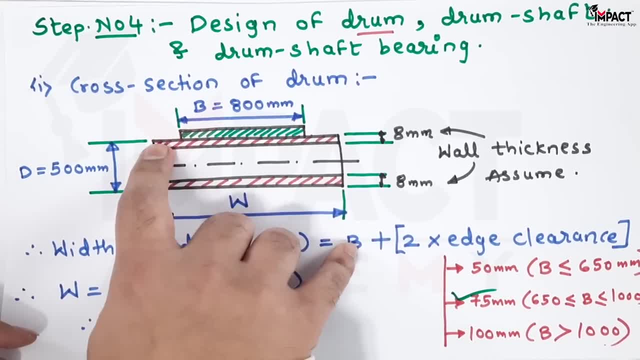 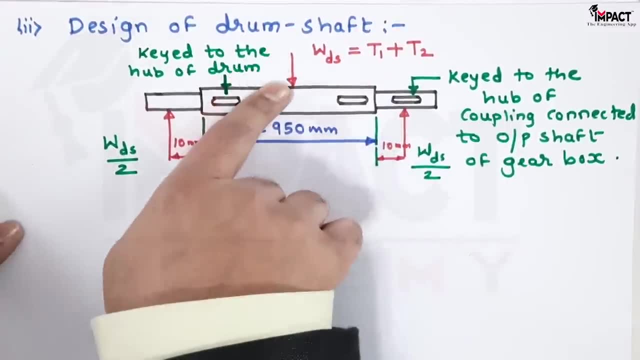 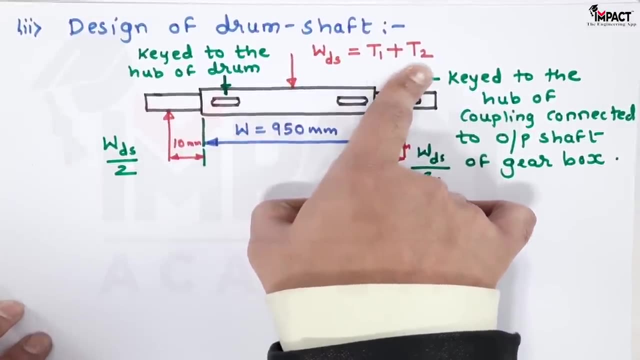 also, there would be keyway here. I have not shown in this diagram, but there would be keyway, so the shaft gets fit inside this drum and the load acting on the drum would be, or on the drum shaft is exactly at the center and that load is nothing but the tension on tight. 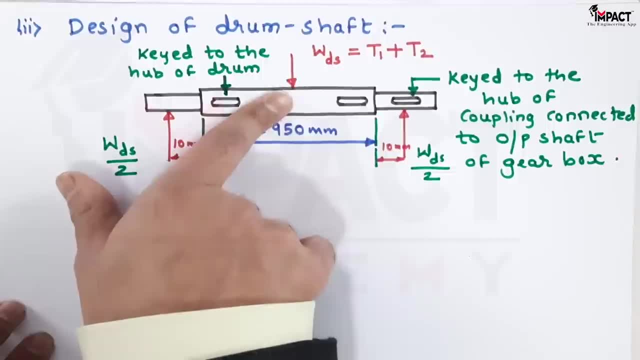 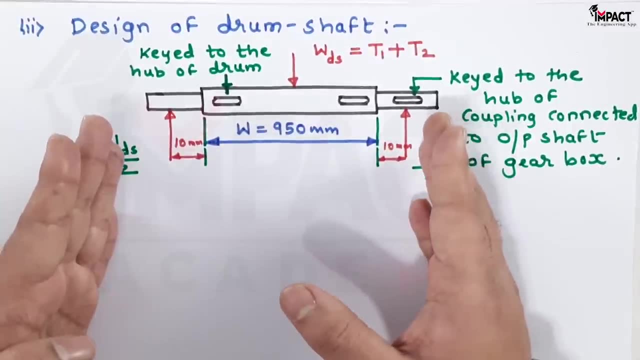 side and slack side, which is T1 plus T2.. So when this load is acting It gets divided on the shaft equally on both the parts, like it is acting as a support reaction. so when the load is acting on this beam we can say shaft as a beam. so when the load is 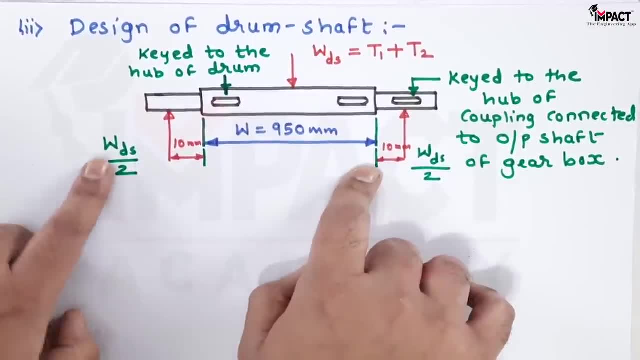 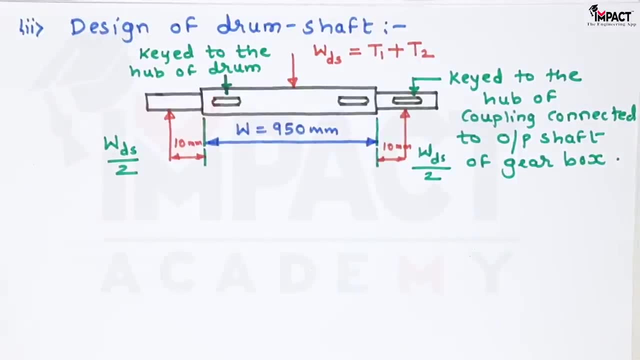 acting centrally, it gets divided equally on both the halves. so we have Wds by 2 on both side, which is the load acting on the drum shaft. now, therefore, the load acting on the drum shaft W suffix ds is T1 plus T2.. So this is the load acting on the drum shaft. 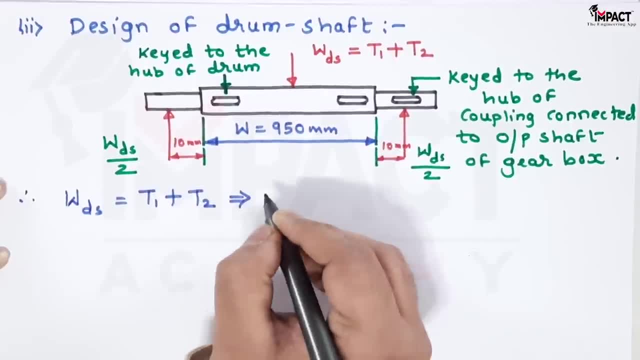 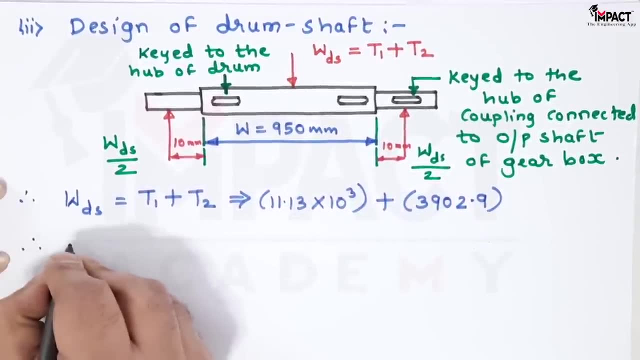 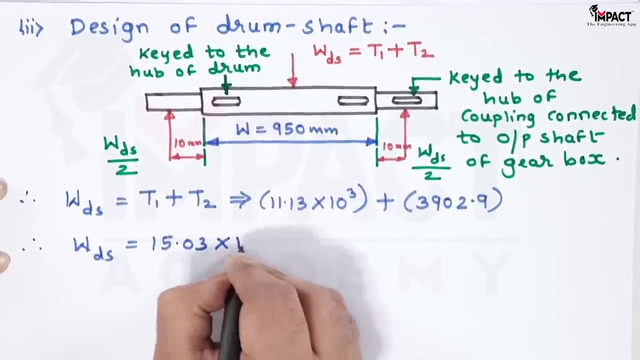 Now, therefore, Ws suffix ds is T1 plus T2. both the values are known to us. these values have been calculated before, so therefore W suffix ds. the load acting on the drum shaft is 15.03 into 10 raise to 3 Newton. it gets divided equally, so therefore Wds by 2 will be 7.52 into 10 raise to 3 Newton. 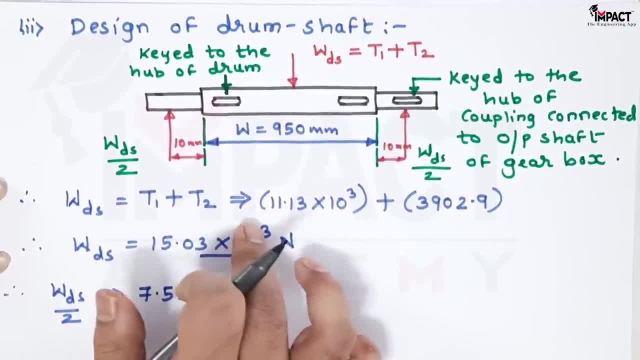 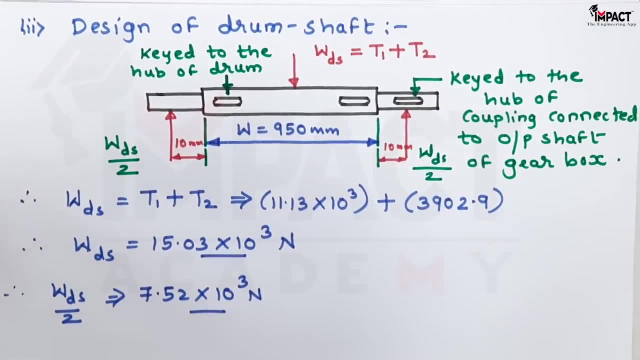 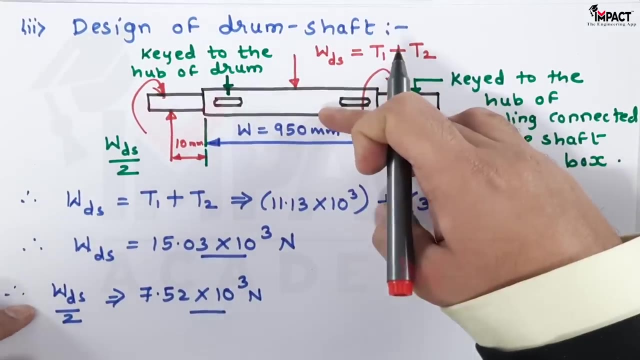 Taking the half of this value Now, the shaft would be subjected to combined twisting and bending, because the shaft is rotating. at the same time, the load is acting, because of which there are support reactions and there will be bending moment. so the same shaft will bend as well as well as rotate. 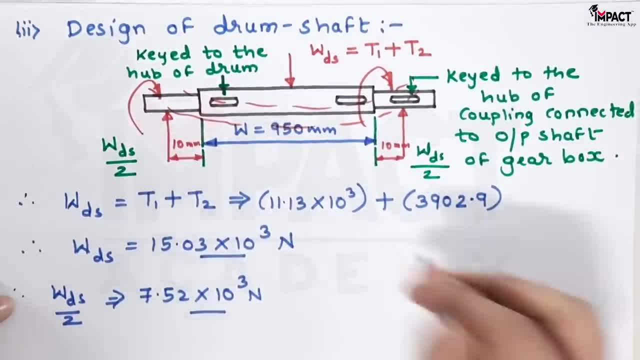 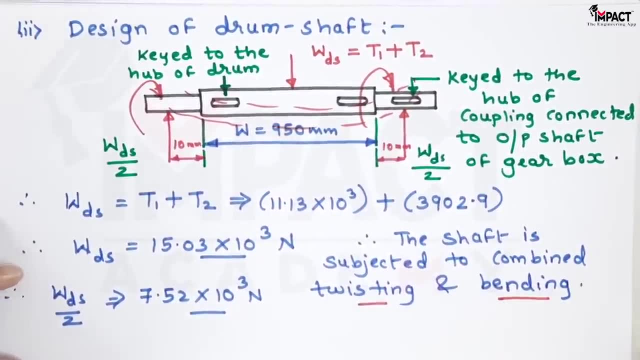 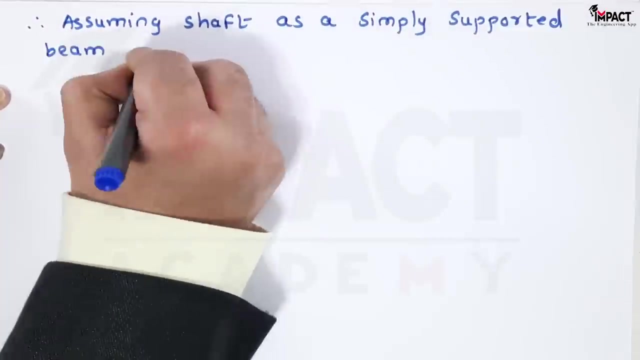 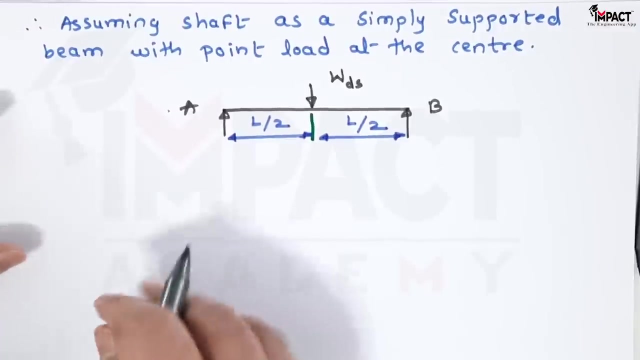 so it is subjected to combined twisting and bending. So therefore, Now, since it is subjected to combined twisting and bending, we are going to use the concept of equivalent torque, and for that first I will find out the maximum bending moment at the center. so therefore, assuming, 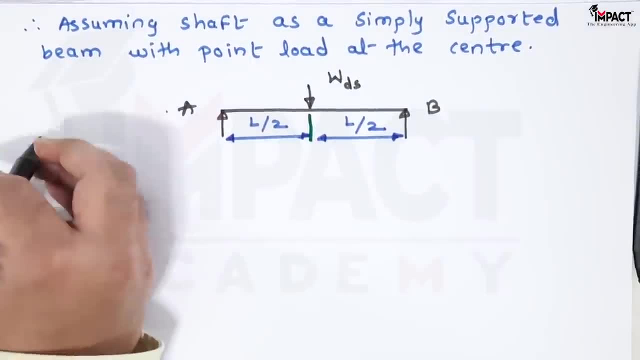 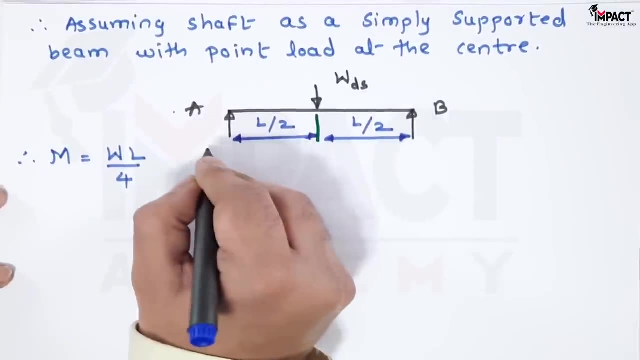 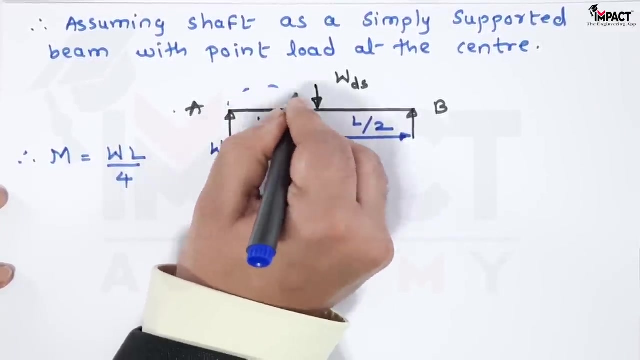 So for simply supported beam with point load at the center, the maximum bending moment is given by W, L by 4. and how to get that? it is very simple, since the support reaction here is W ds by 2, or we can simply say W by 2. so when I take the moment at the center, because at the center, 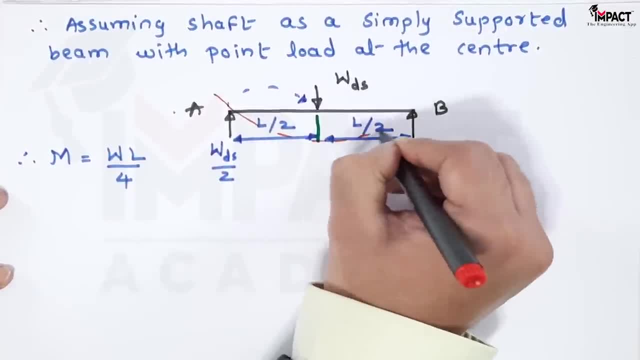 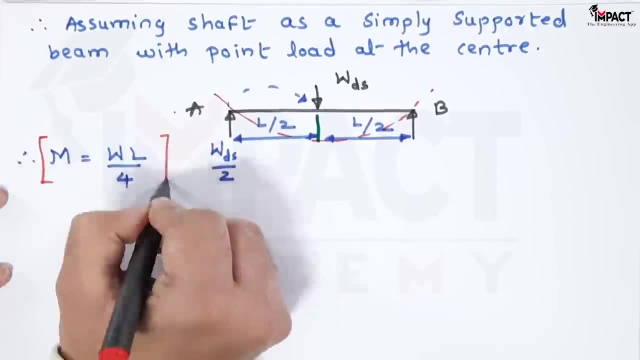 it will be maximum bending moment. shaft is bending in this fashion. so therefore it is W by 2 into L by 2, which gives me the answer as W, L by 4.. W value is 15.03 into 10. raise to 3.. So therefore it is W by 2 into L by 2 which gives me the answer as W, L by 4.. W value is 15.03 into 10, raise to 3.. W value is 15.03 into 10, raise to 3.. 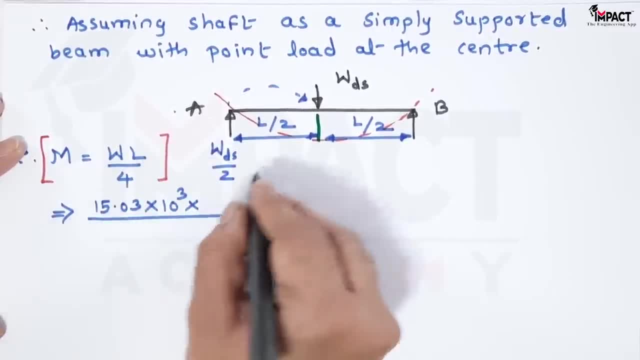 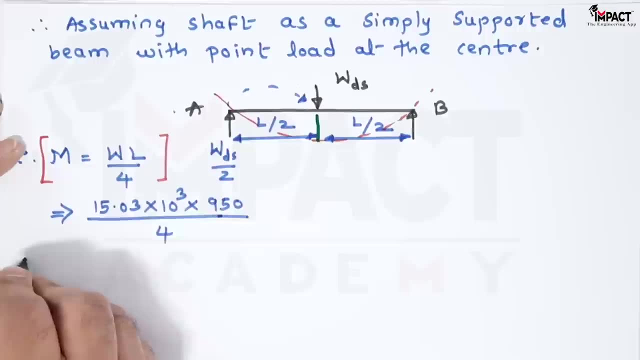 The length is 950 nm, already calculated, equal to the width of the drum divided by 4. so therefore, the maximum bending moment will come out to be 3.57 into 10 raise to 6 Newton nm. and now, once the bending moment is known, now I have to get the twisting moment, that is, the torque. 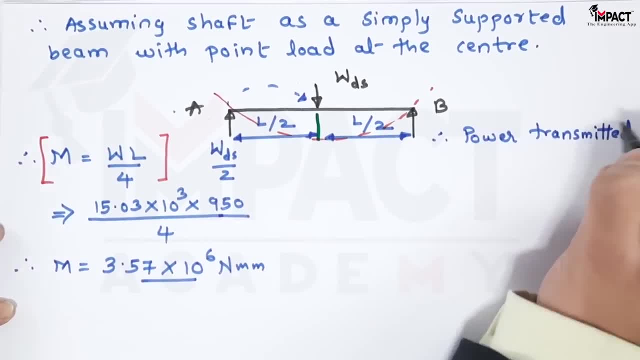 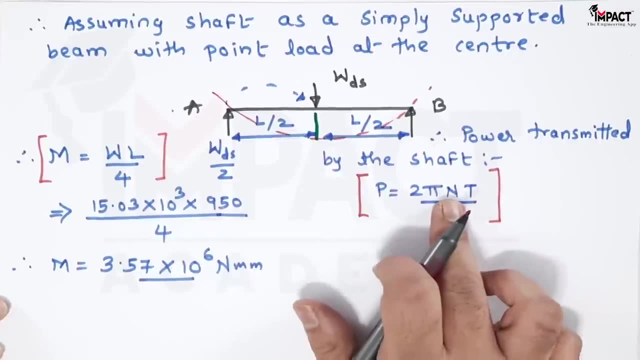 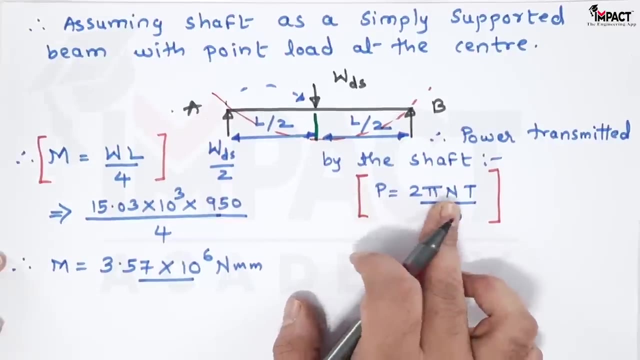 so therefore, power transmitted by the shaft, It is 2 pi NT upon 60. So N is the RPM. power is already known to us. it is 11 kilowatts, So 11 into 10, raised to 3. now how to get this N value for that? I am keeping this. 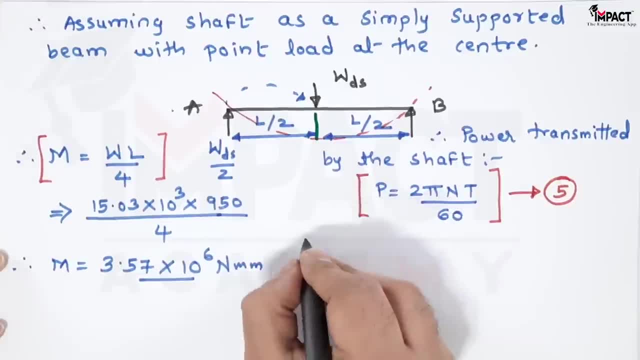 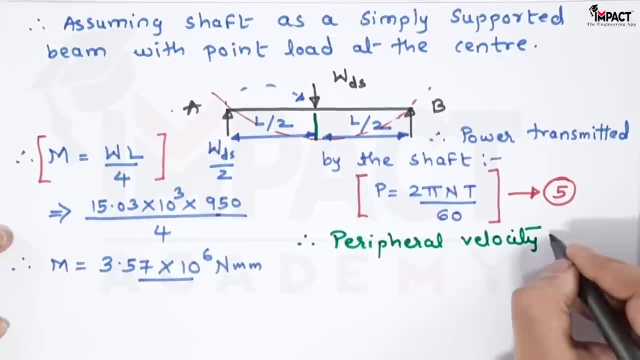 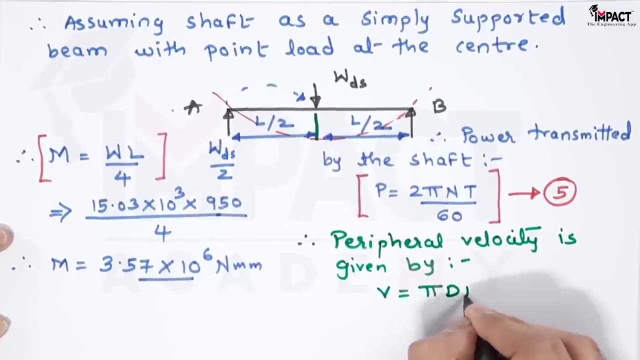 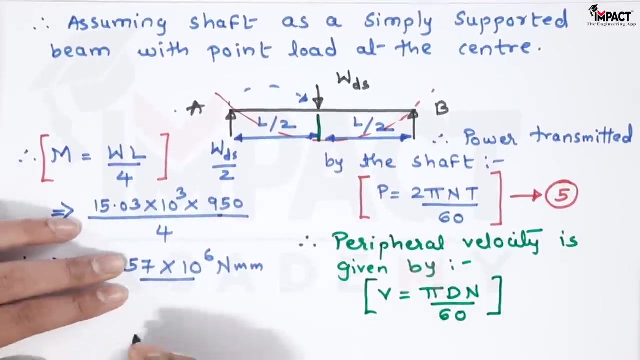 as equation number five, And therefore the peripheral velocity of the drum or the shaft is given by. also we can say the belt speed. it is pi into D, N upon 60.. So from this formula I can get the RPM and the velocity is 1.35 meter per second. pi diameter is 500 mm, So it is 0.5 meter. 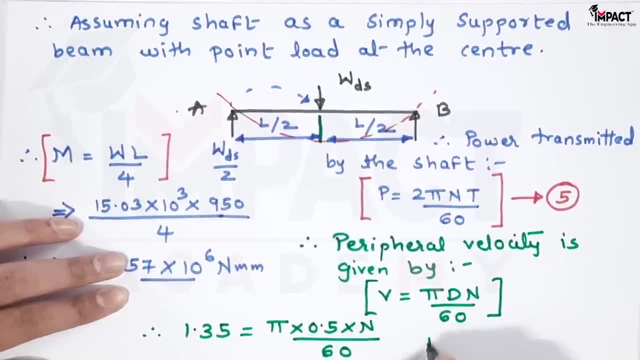 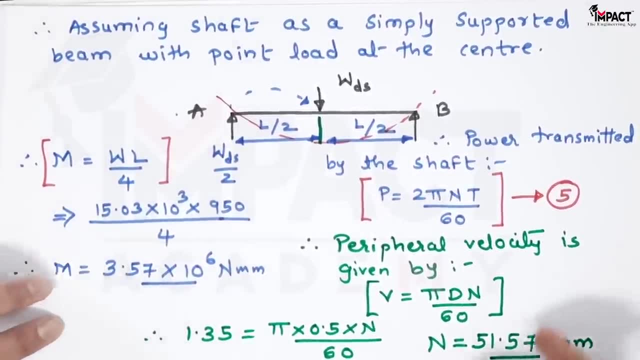 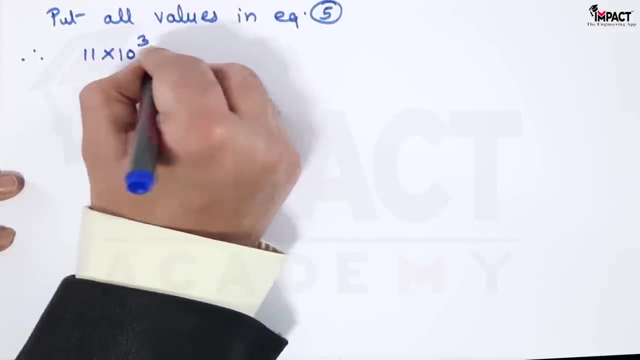 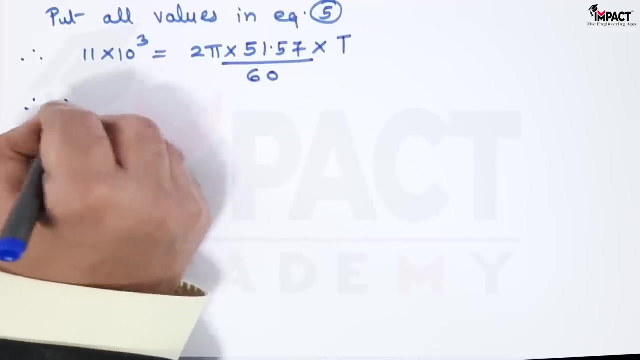 into N upon 60. On calculating this, I am getting the answer of N as 51.57 RPM. So, putting all values in equation, five power is 11 into 10, raised to 3 watts RPM, 51.57 divided by 60. So therefore torque comes out. 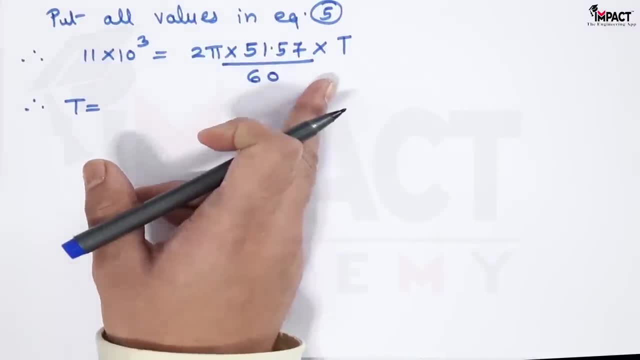 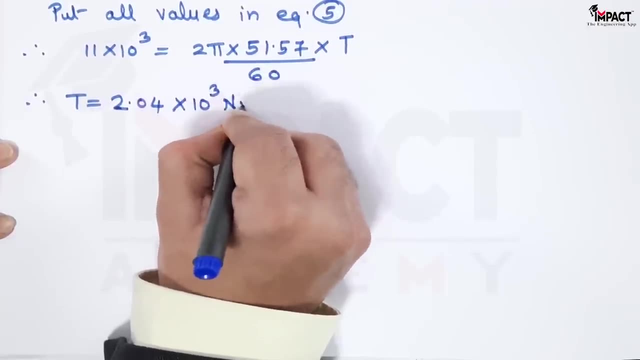 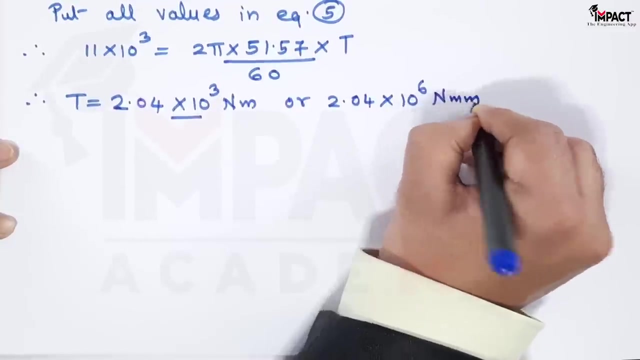 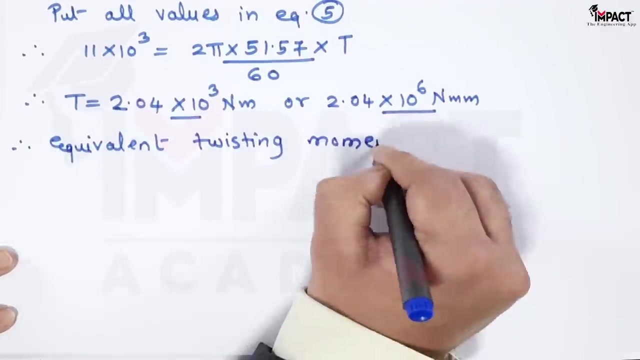 to be and remember when power is in watts. torque would be, in terms of Newton meter, 2.04 into 10 Newton meter, or multiplied with 10 raised to 3.. So it becomes 10 raised to 6 Newton mm. Now, therefore, equivalent twisting moment is given by: 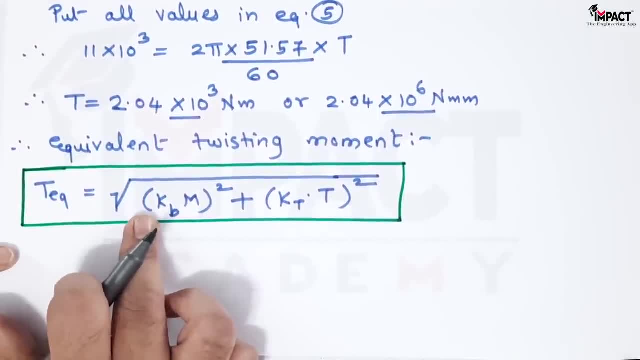 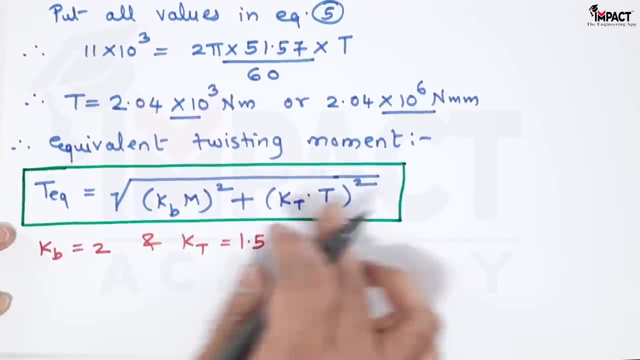 so this is the formula for equivalent twisting moment, where Kb is the shock and fatigue factor for bending, which is taken as 2 shock and fatigue factor for bending, and Kt is the shock and fatigue factor for twisting, taken as 1.5.. So putting the values over here, 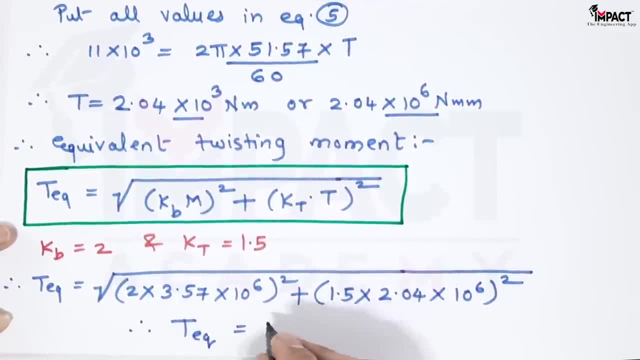 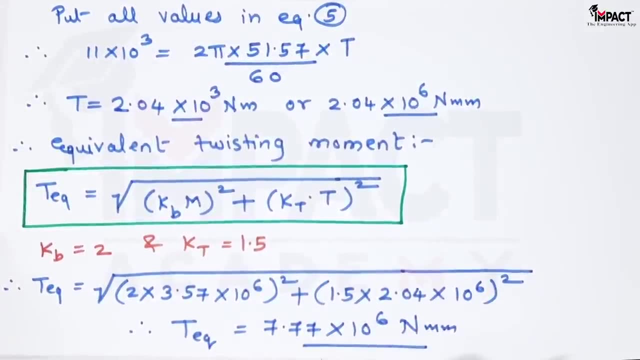 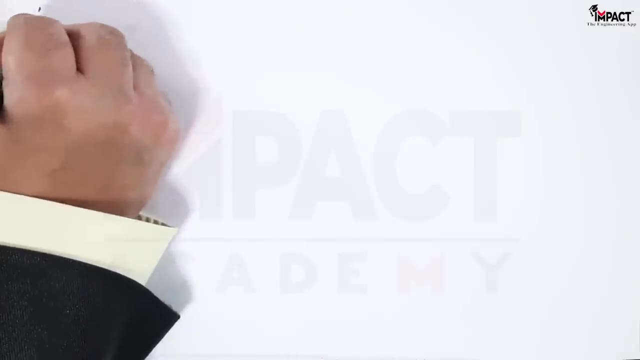 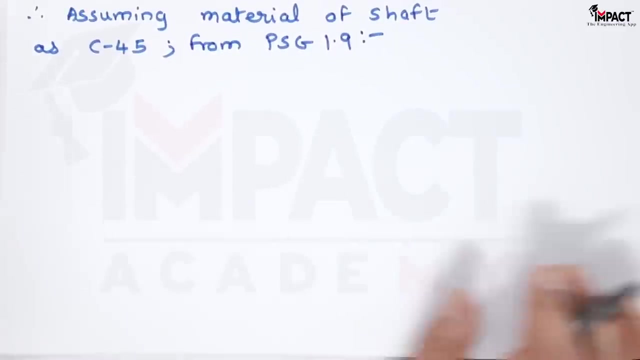 So, therefore, T equivalent will come out to be: it is 7.77 into 10, raised to 6 Newton mm. Now, in order to get the diameter of shaft, I am assuming the material of shaft. So therefore, so whenever the material is not specified for the shaft, we can take it as C45, because if 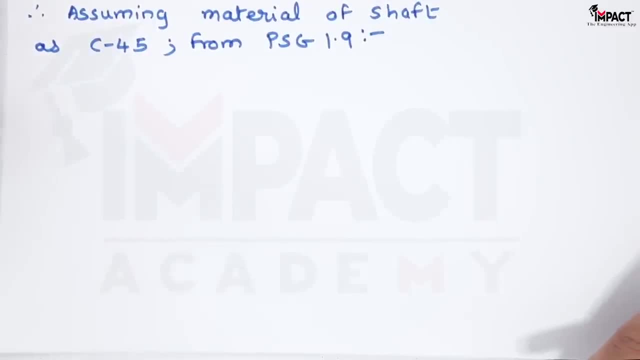 the carbon content would be reduced, like if, for example, we are taking C20 or C30 as the material for the shaft, then that shaft would be easily subjected to bending and twisting. it means the shape would change very quickly because of the list carbon content. So 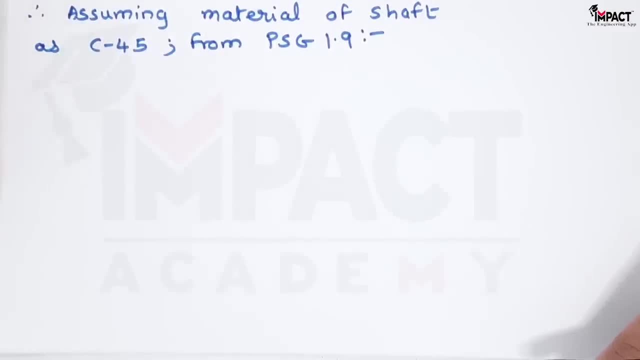 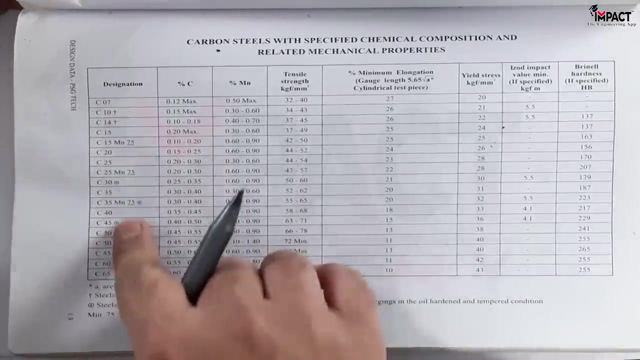 increase the carbon content and take it as c45 until and unless the other material if they have specified. so we have to take c45 and from psg 1.9- here we have psg 1.9 and in this column we have c45. 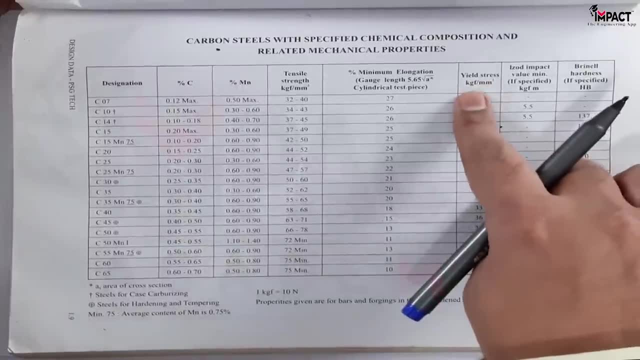 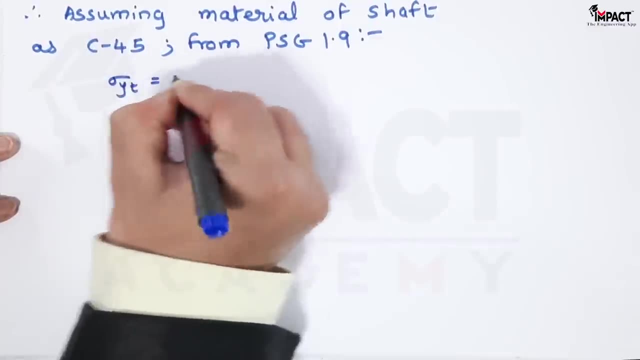 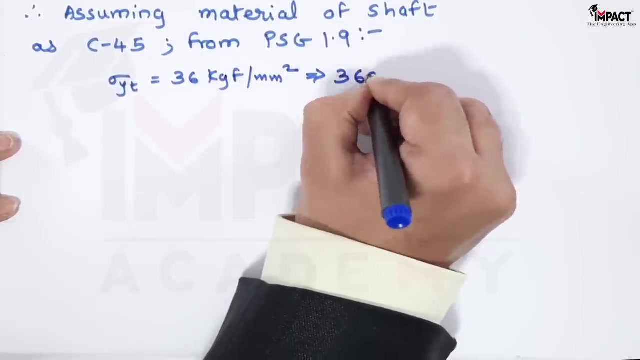 for that we have to select this value. here yield stress is given, but the unit is kgf per mm square, so it is 36. the yield tensile stress is 36 kgf per mm square multiplied by 10 and it becomes 360 newton per mm square. now stress value won't be this much high because it is. 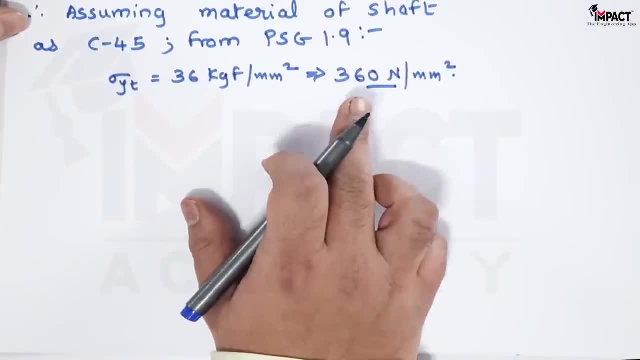 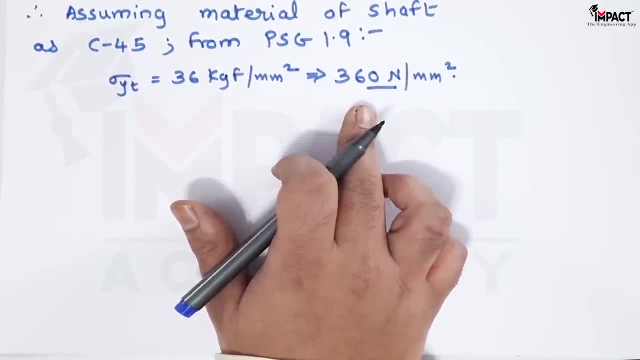 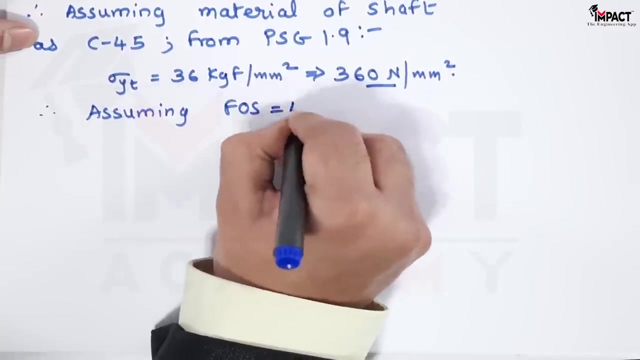 the yield value. so when the shaft is subjected to this much amount of stress then it can fail or it can break even though the load is removed. so we have to avoid so much stress in the shaft. so for that assuming factor of safety as 4, so therefore the permissible. 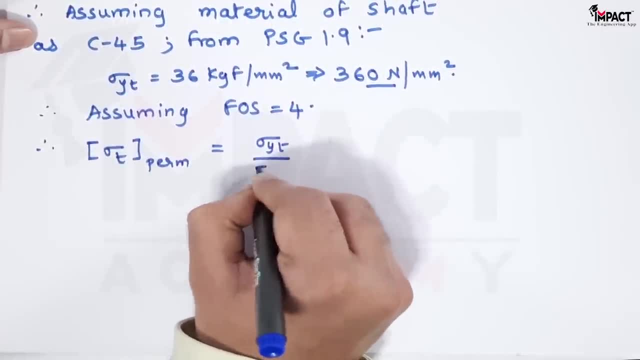 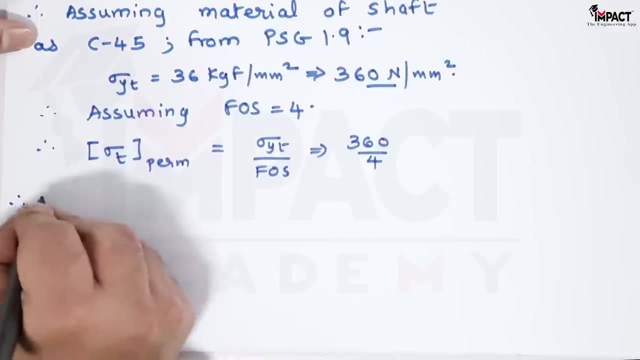 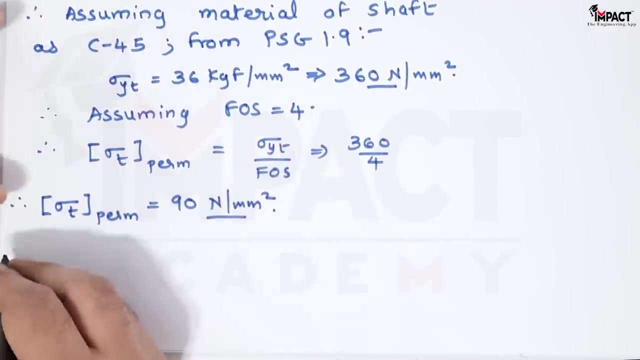 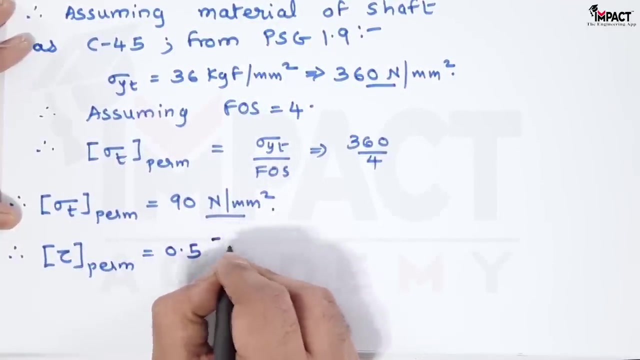 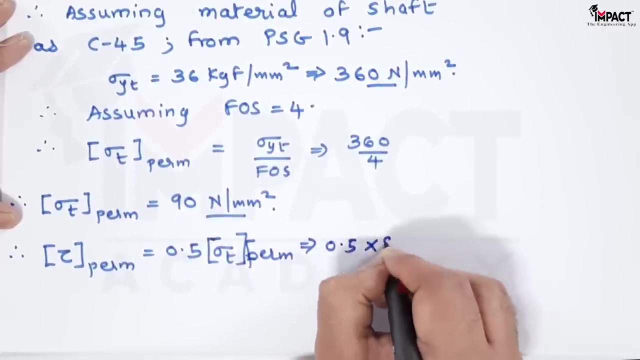 tensile stress would be sigma yt divided by fos, that is 360 by 4. so therefore permissible tensile stress is 90 newton per mm square and therefore the permissible shear stress which is required is half of 0.5 of sigma t permissible. so it is 0.5 into 90 and therefore tau permissible. 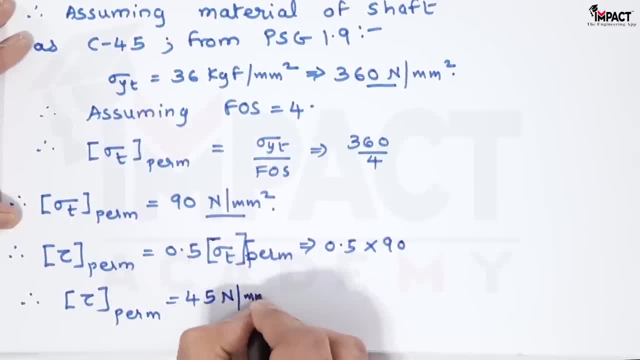 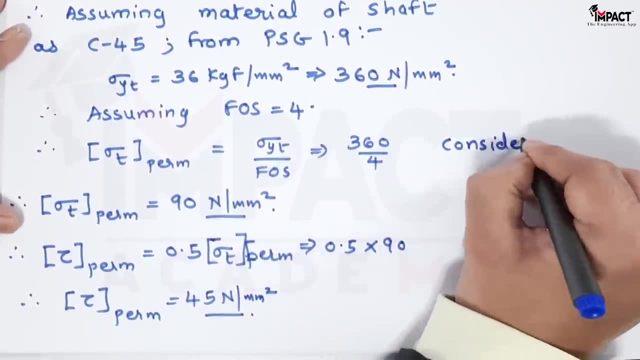 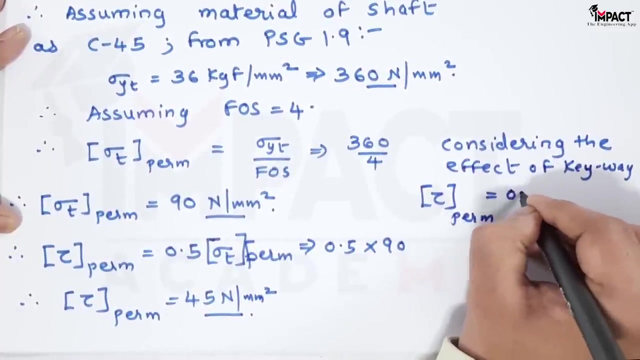 will be 45 newton per mm square now, therefore, since the shaft has keyway, so considering the effect of keyway, tau permissible would be again reducing it. so 0.75 into the tau permissible which has been calculated previously. so 0.75 into 45 and finally the tau permissible value would be: 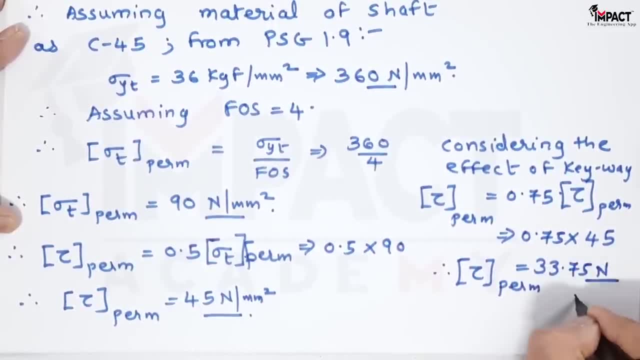 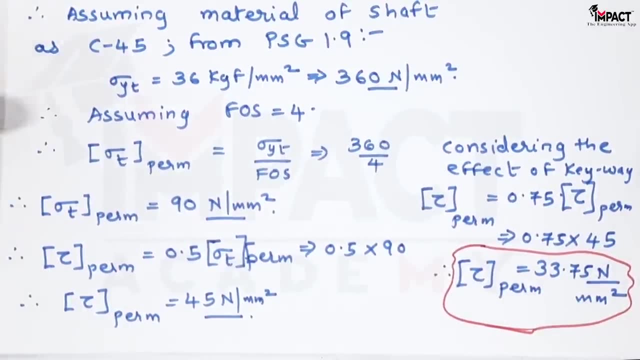 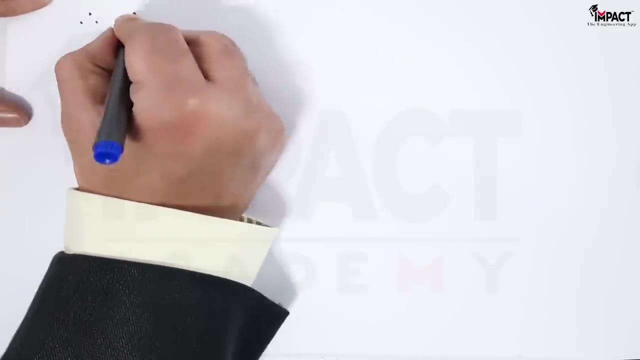 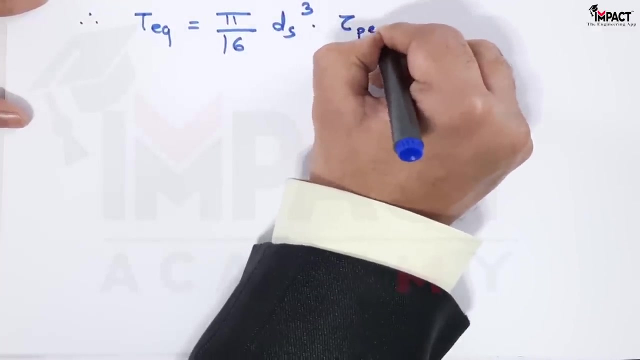 33.75 newton per mm square. now we have to use this value to get the excess value of the permissible shear stress for designing the shaft. so therefore i can write down t equivalent is given by 5 by 16 into ds cube, which is the diameter of shaft. 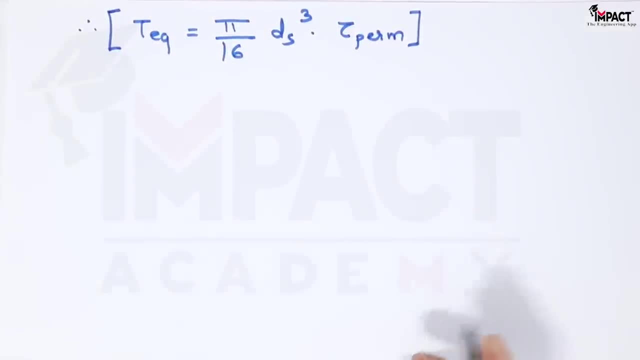 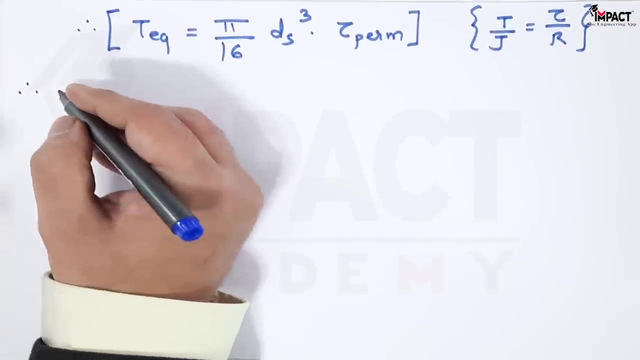 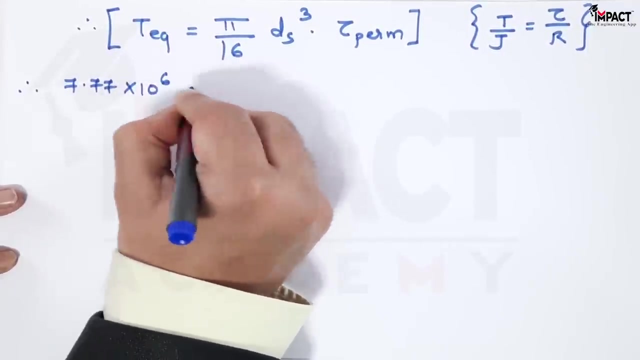 into tau permissible, and this formula comes from the strength criteria for shaft, that is, 3 by j is equal to tau by r. next, Therefore, putting the values, the equivalent is 7.77 into 10. raise to 6 is equal to 5 by. 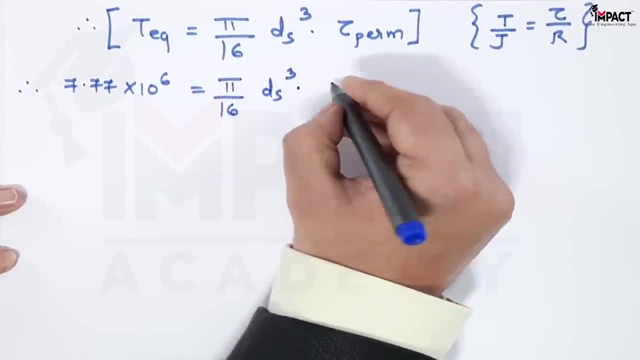 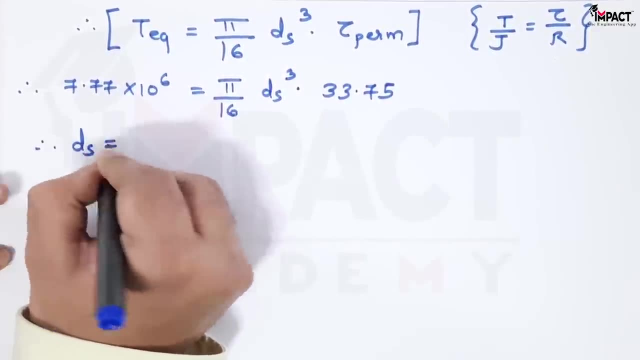 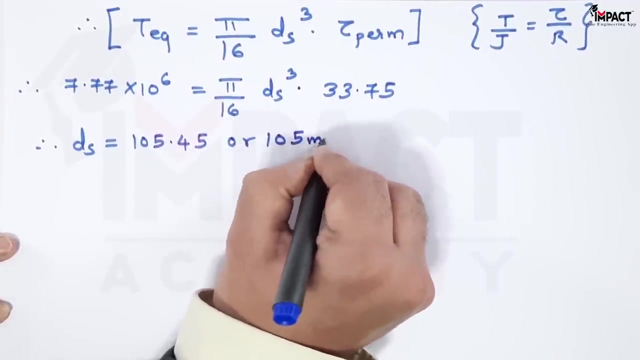 16 ds cube into the permissible tau, which is 33.75.. So on calculating this, I am getting the shaft diameter as 105.45, so closer to 105 mm. I am writing it as 105 mm. so that is the diameter of shaft. 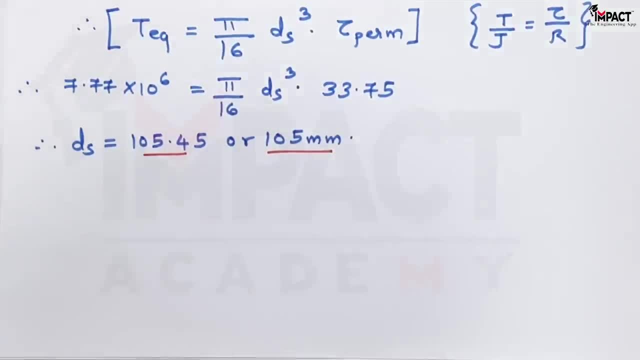 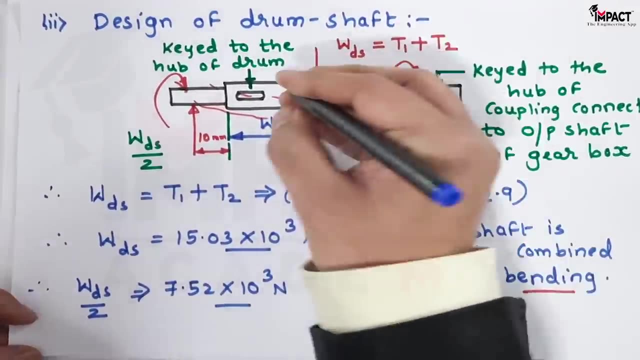 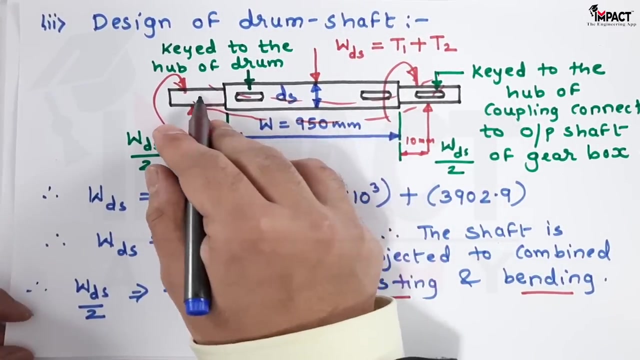 And at the same time we can see that we have found out the diameter of shaft, which is considering the maximum bending moment at the center. So this is the diameter of shaft. Here we are seeing a stepping. This stepping is given so that the bearing can be fixed over it. 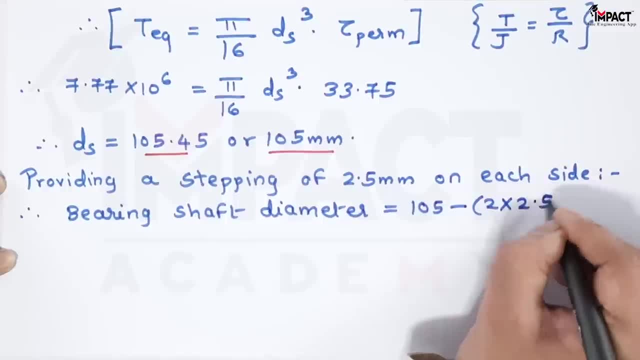 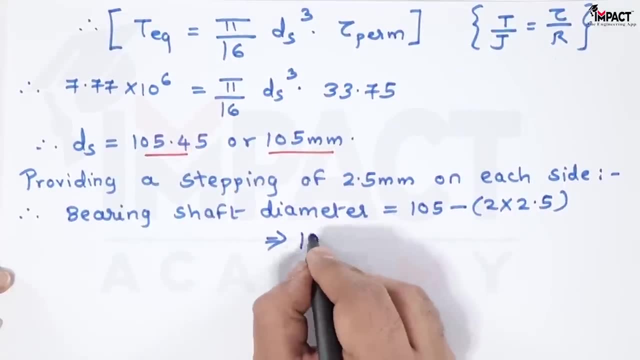 So, providing the stepping of 2.5 mm, therefore, the bearing shaft diameter, the diameter which goes into the bearing, will come out to be 100 mm. So here the shaft has also been designed. Now the step which is left in this step number 4, is the bearing selection for the drum. 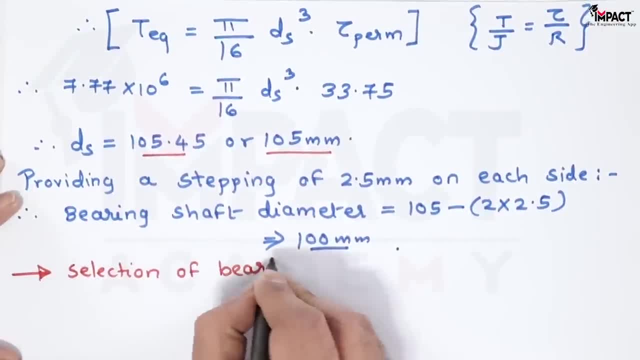 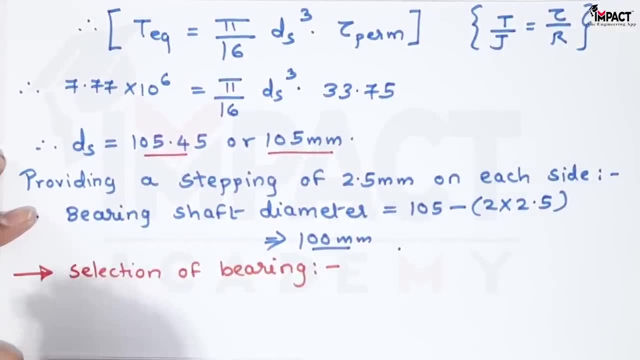 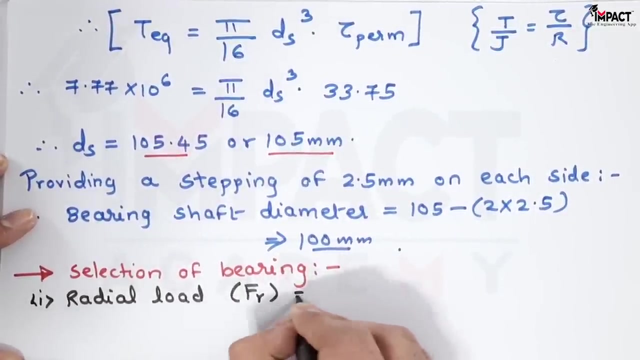 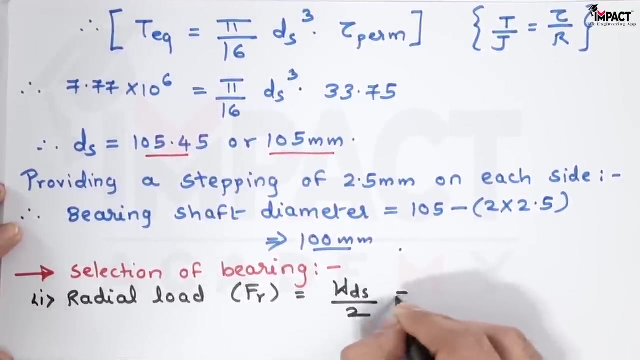 So, therefore, the selection of bearing, In that the first parameter which is required is the radial load, that is, F suffix R, and it is equal to half of the load on the drum shaft, which was 7.52 into 10, raise to 3 Newton. 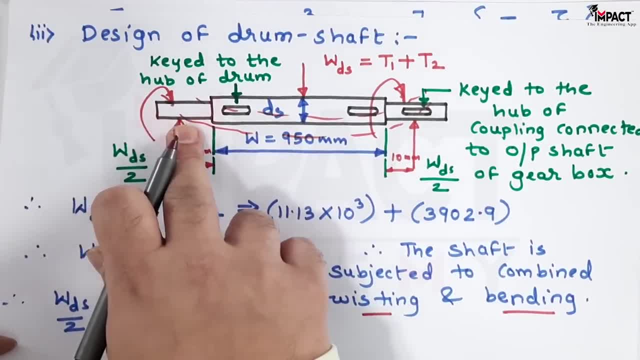 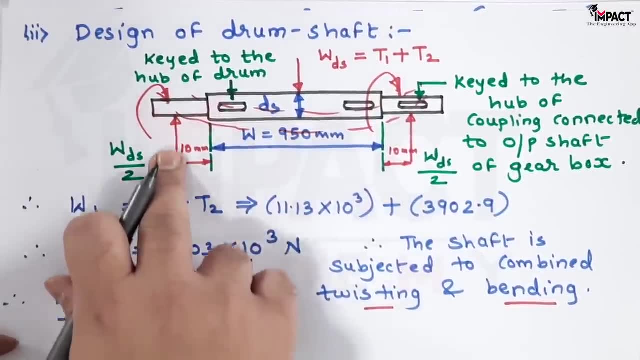 Because when we look into this diagram, the bearing would be connected to the drum shaft, So the bearing is connected over here. So when the bearing is connected on this diameter, which is of 100 mm, the load which is acting is radial. acting towards the center, it is the radial load. 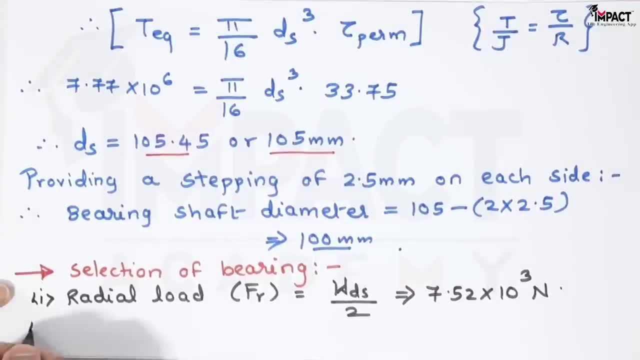 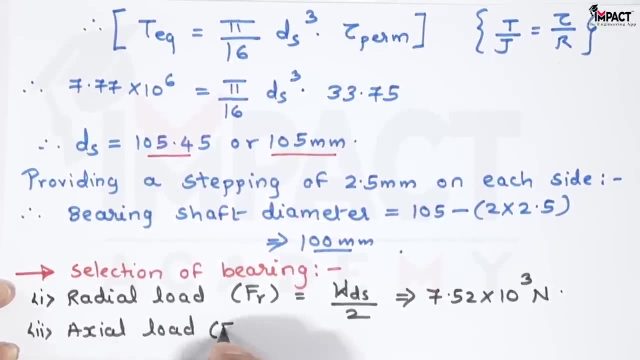 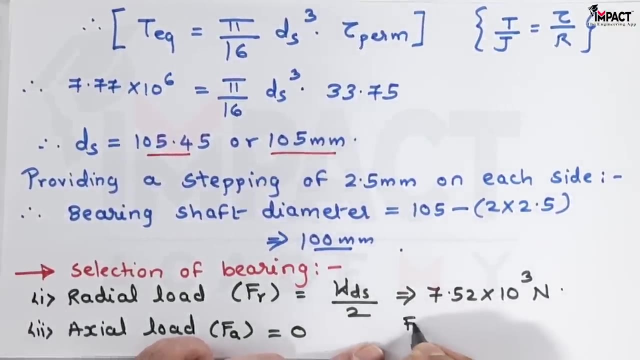 So that is Wds by 2 and axial load is not specified, it won't be acting, So the axial load is taken as 0. And since I can say that Fr is the radial load, the condition is it is less than 8 kilo Newton. 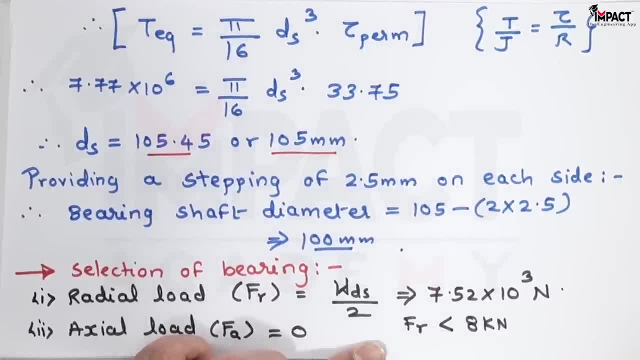 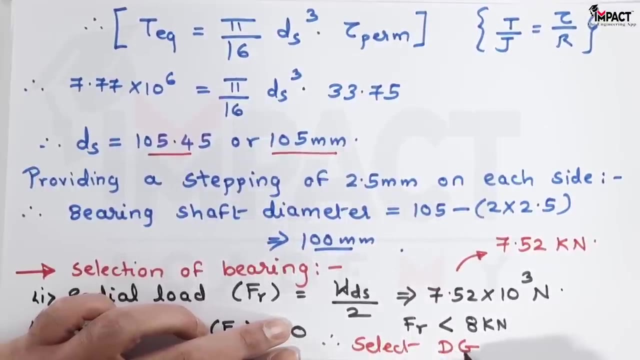 As we see here, it is 7.52 into 10 raise to 3 Newton means it is 7.52 kilo Newton. So therefore we have to select DGBB, that is, deep grove ball bearing, and for that I have to assume the life in hours for the bearing. 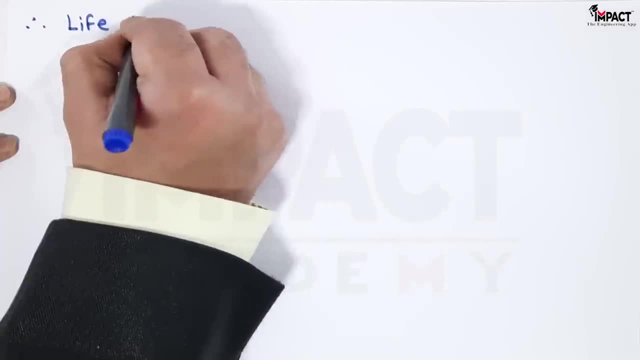 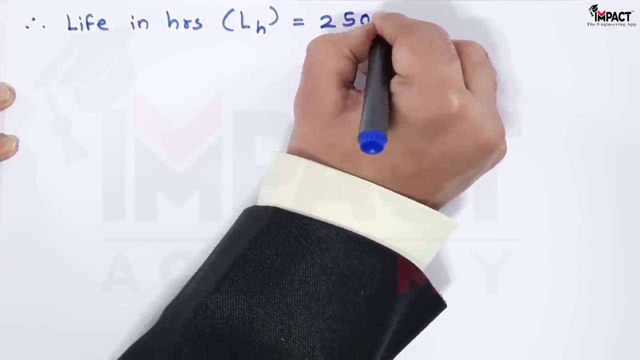 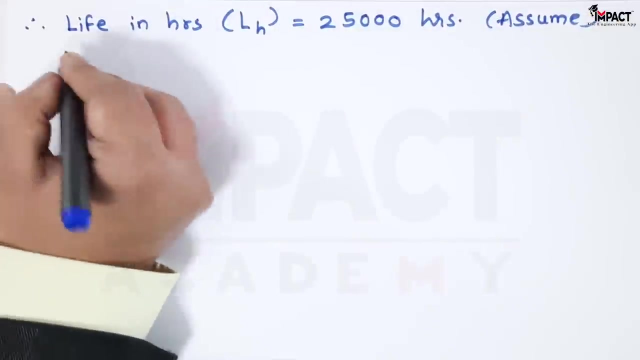 So that is the radial load. So therefore, life in hours for the bearing denoted as L suffix H, I am assuming it to be 25,000 hours. If nothing is mentioned, you have to assume this value: 25,000 hours. 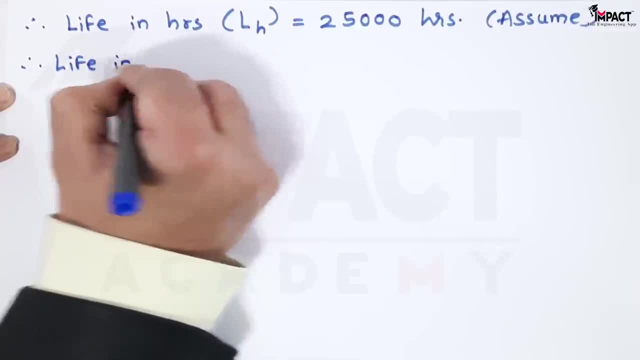 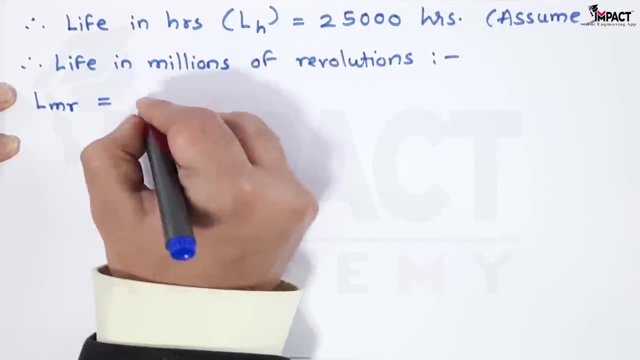 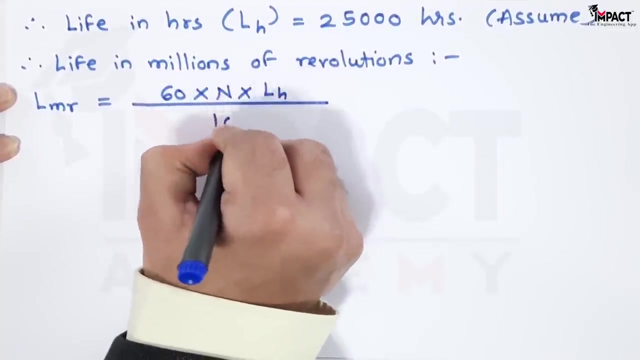 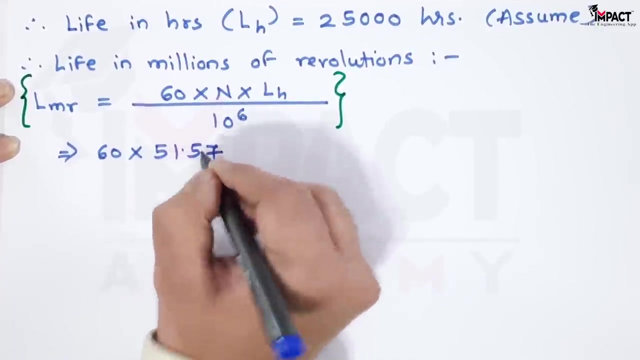 So, therefore, life in millions of revolutions is given by the formula. It is denoted as L suffix MR 60 into N, which is rpm. Okay, L suffix M into L suffix H, upon 10 raise to 6, rpm already calculated. 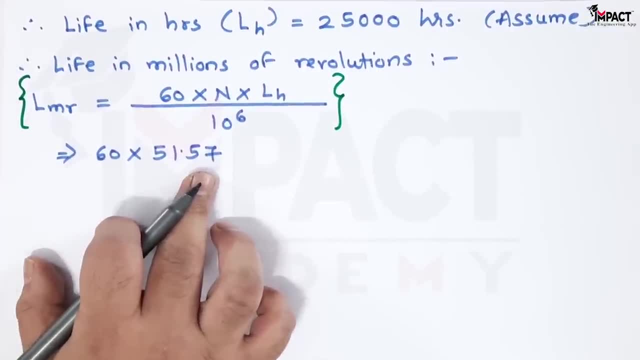 So the rpm is 51.57 of the shaft. It means the drum is also rotating with the same rpm. So the motor was giving an output of 1440 rpm. as we have selected the motor, we know the speed of the motor. 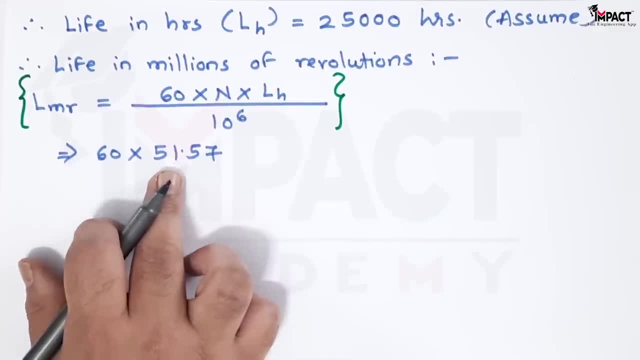 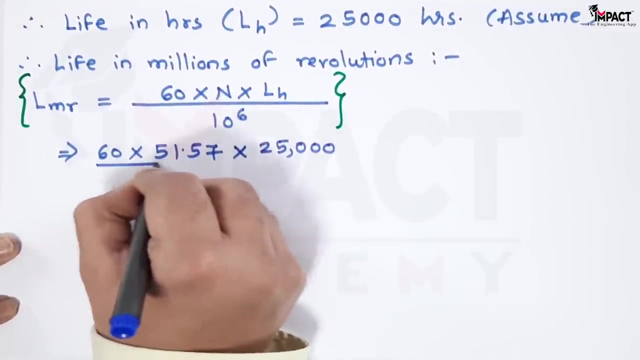 So from 1440, we have to reduce the value up to 51.57 rpm. That is possible with the help of the reduction gearbox. So that is the explanation regarding this rpm, and the life in terms of hours is 25,000.. 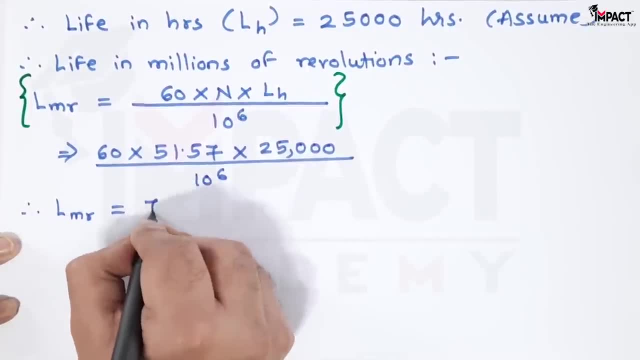 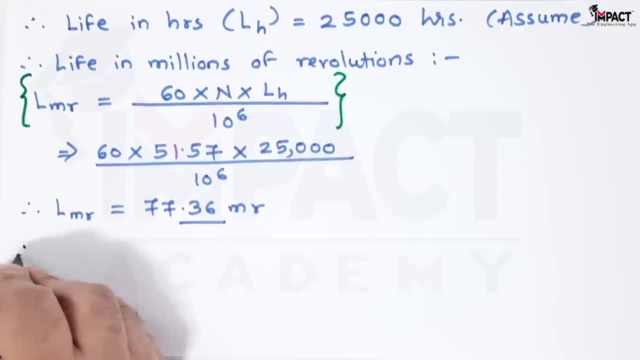 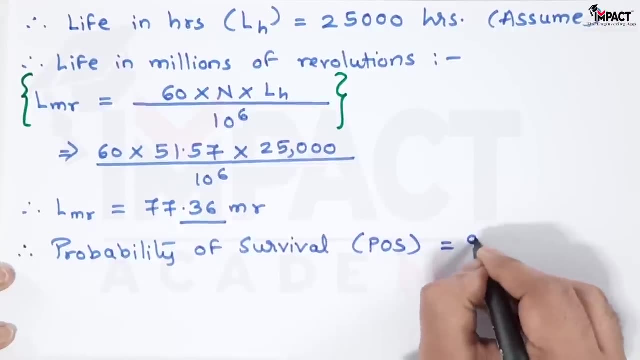 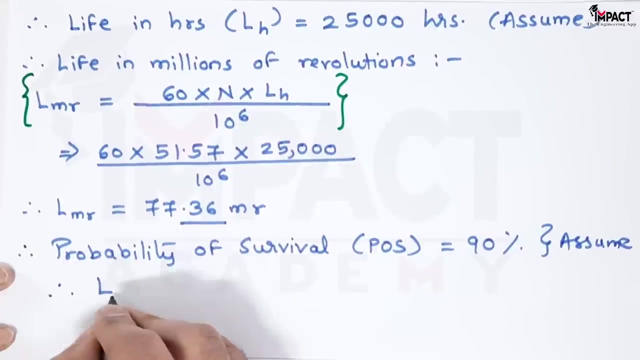 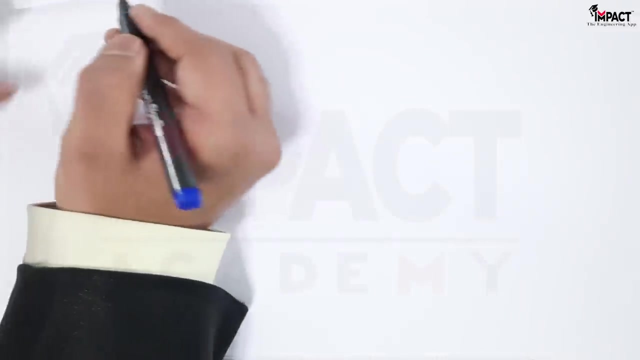 So that is the life of the bearing. And now the probability of survival POS is assumed to be 90%, unless specified, And therefore this LMR would be equal to L10.. Now from PSG, another formula, So therefore from PSG 4.2, we have a formula. 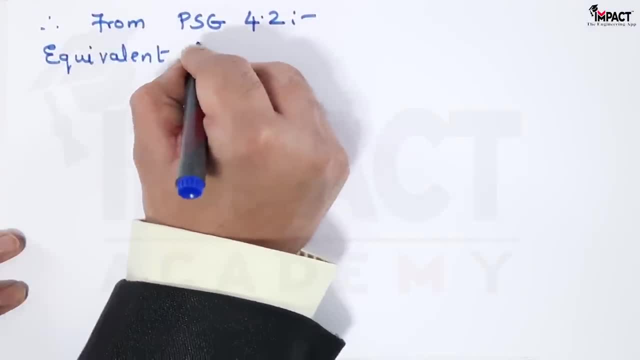 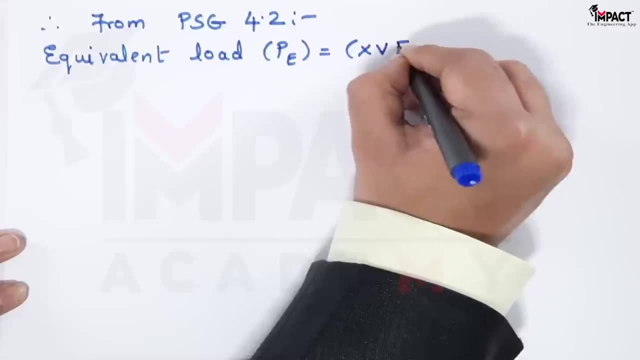 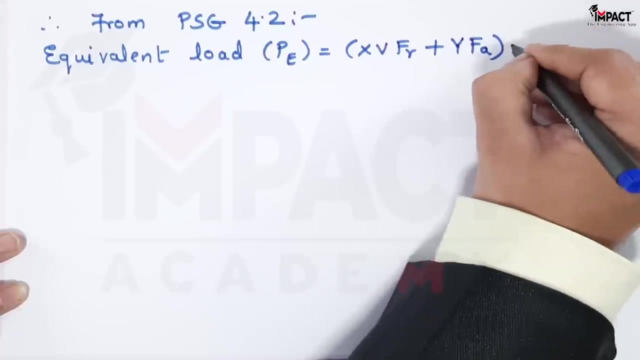 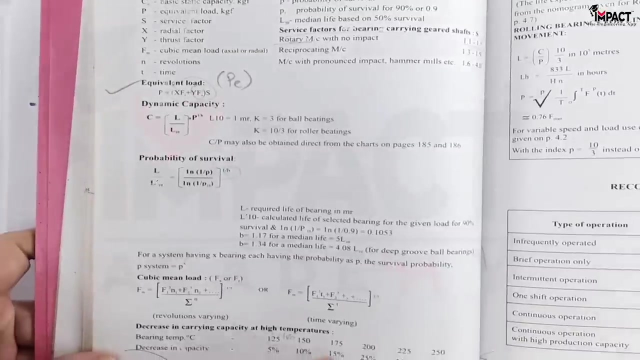 So from PSG 4.2, we have a formula of equivalent load, of equivalent load which is P suffix E, is equal to X, into V, FR plus Y, into FA, into S, into K suffix T. So from PSG 4.2, we have this formula of equivalent load wherein X is called as the relative. 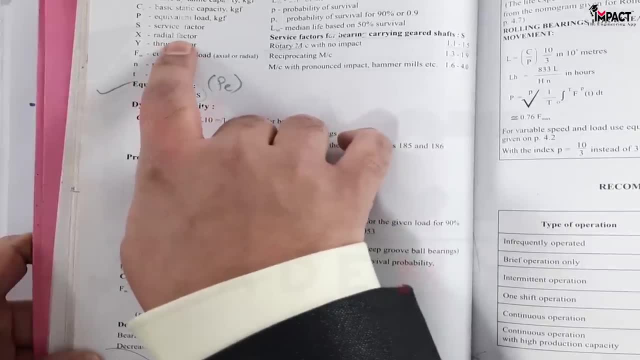 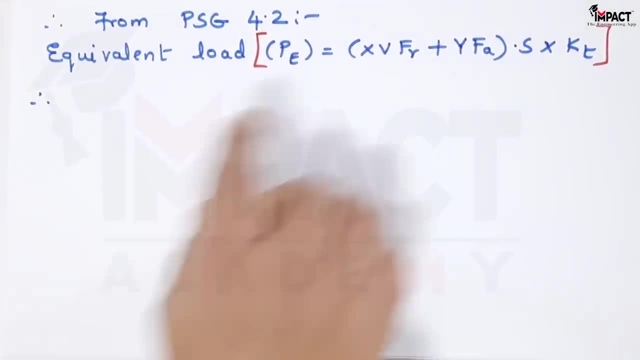 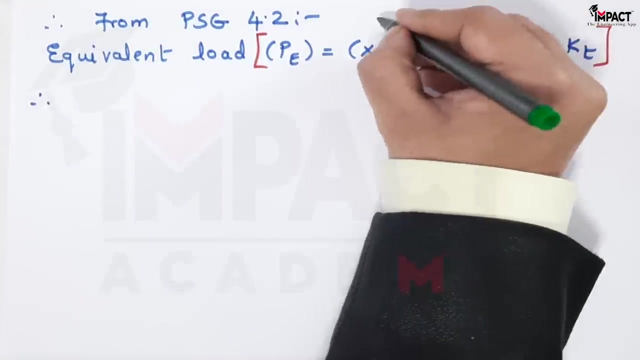 load. So from PSG 4.2, we have this formula of equivalent load, wherein X is called as the relative load, radial factor, and since the radial load is there, this factor has to be taken as 1.. Next here, v is for inner race rotation, and that is also taken as 1, so x value would 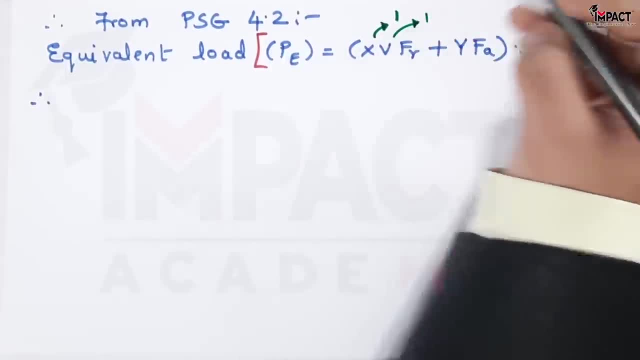 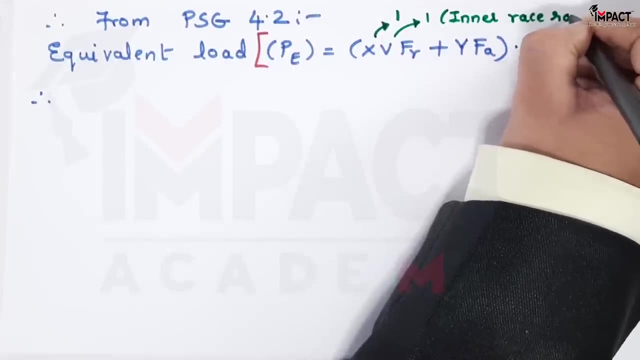 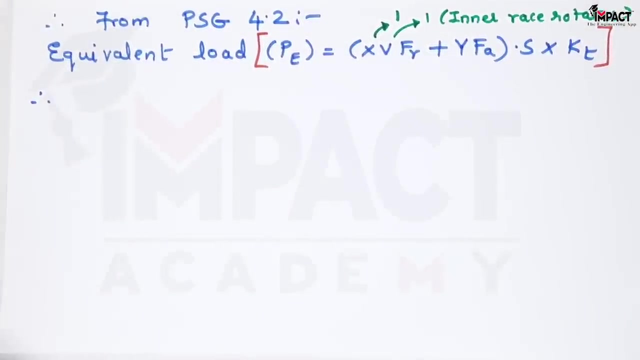 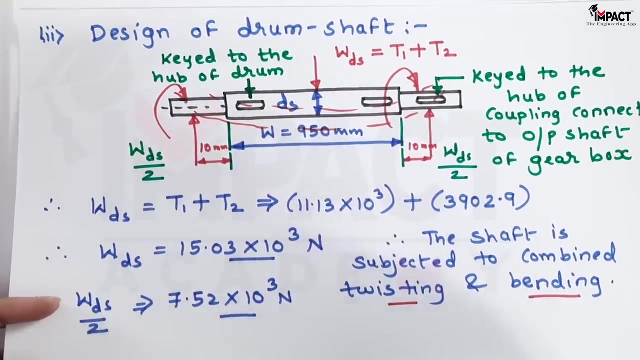 be 1 for radial factor v value would be 1 for as the inner race rotates, Because we do not have outer race rotation here. it means when the shaft is there inside the bearing, then bearing is fixed and the shaft is rotating. 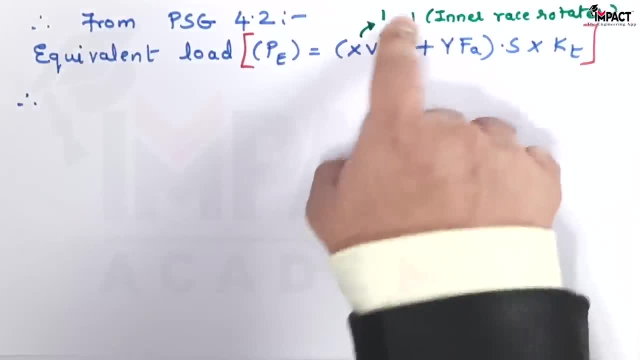 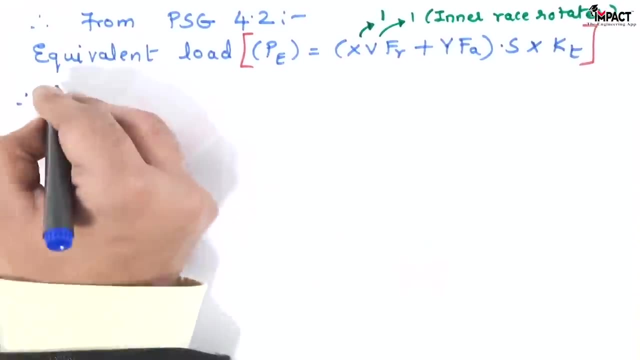 So there is inner race rotation. So therefore v is equal to 1.. Fr is the radial factor, Axial load. we already have the value, which is 7.52 kN, So I am just going on putting the values. 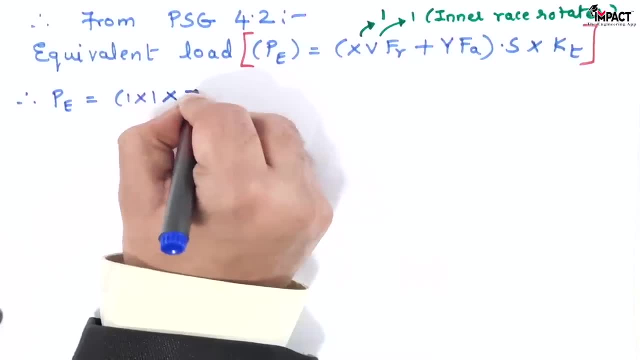 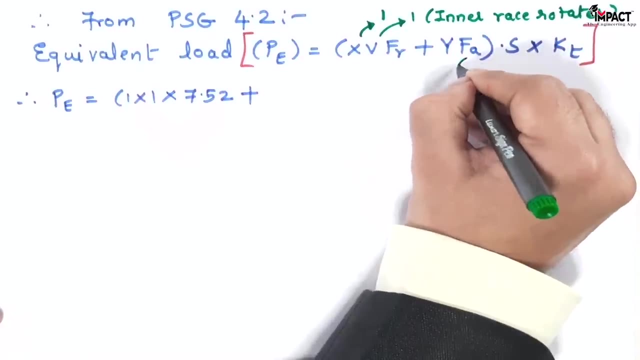 x is 1, v is for inner race rotation. radial factor: radial load is 7.52 kN plus y into fa. Now, since fa is 0 because axial load is not present, so y into fa becomes 0 where y is. 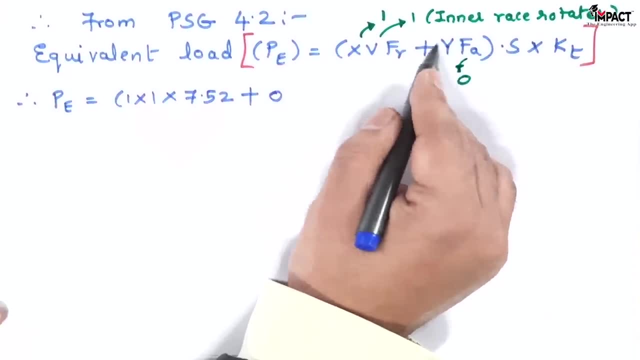 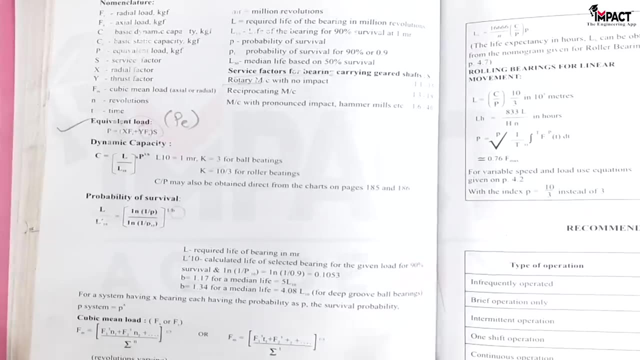 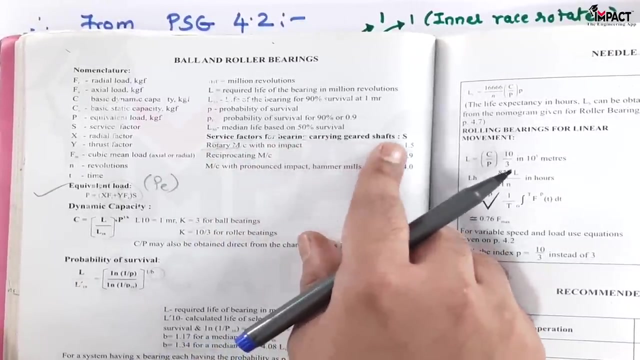 the thrust factor. Since axial load is not there, so thrust is also not there. Then s is the service factor. It has to be taken from PSG 4.2.. Here service factors for bearing carrying geared shafts are given Now for rotary machine with no impact. it is 1.1 to 1.5. 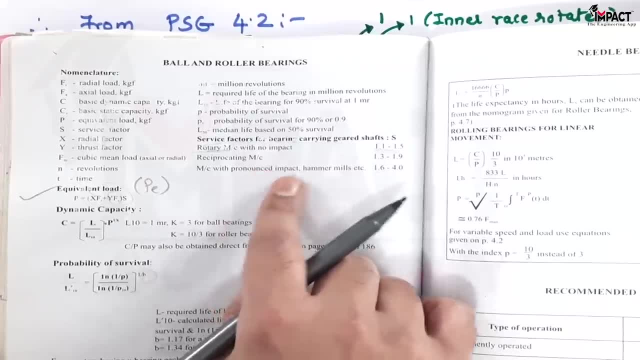 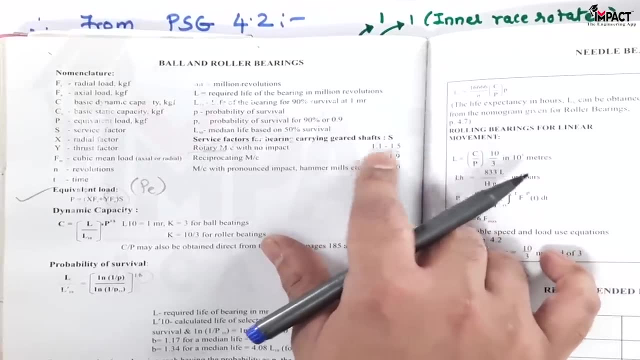 So, yes, it is a rotary machine. It is not a reciprocating machine And here we do not have hammer mills, so the value should be in the range of 1.1 to 1.5.. Better to take the average. 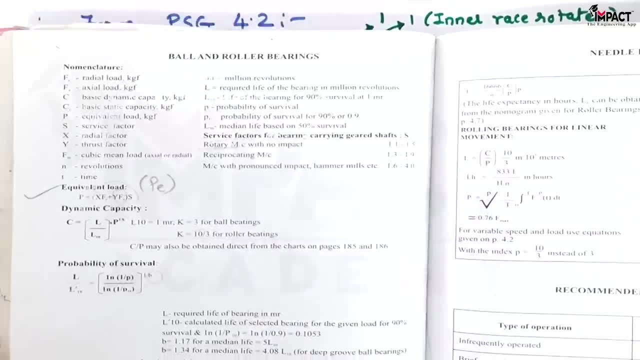 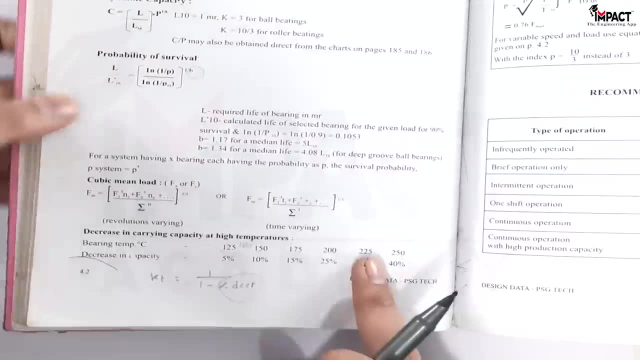 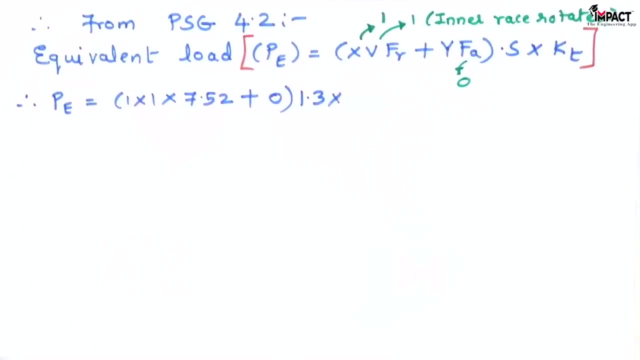 So the average comes out to be 1.3.. So service factor has to be taken as 1.3.. And K suffix. T is the temperature factor. It is the temperature factor, and since nothing is specified about the temperature, we can take that factor also as 1.. 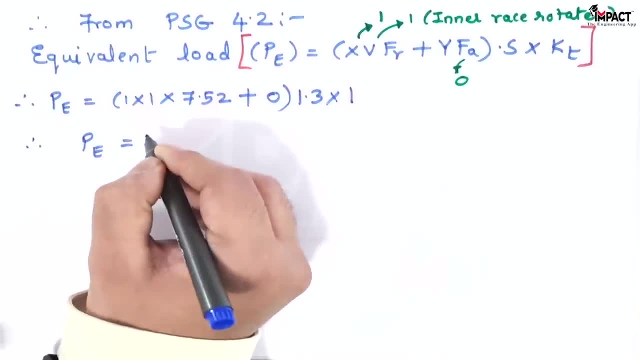 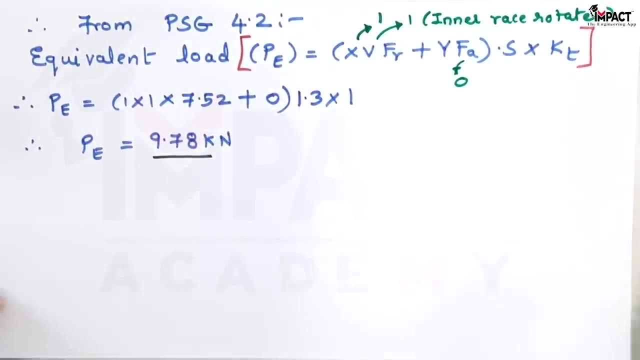 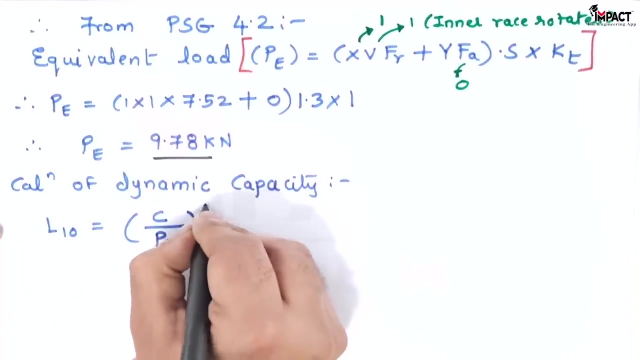 So therefore, on calculating this, I am getting the equivalent load and my answer is 9.78 kN And therefore, after reaching 1.5.. After reaching up till here, calculation of dynamic capacity of the bearing. the formula is: L10 is equal to it is C upon P suffix E raised to the power K. 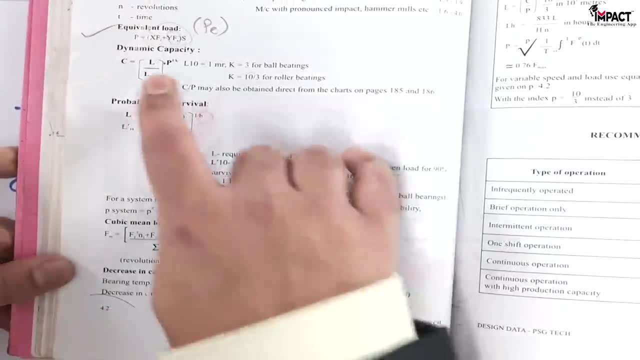 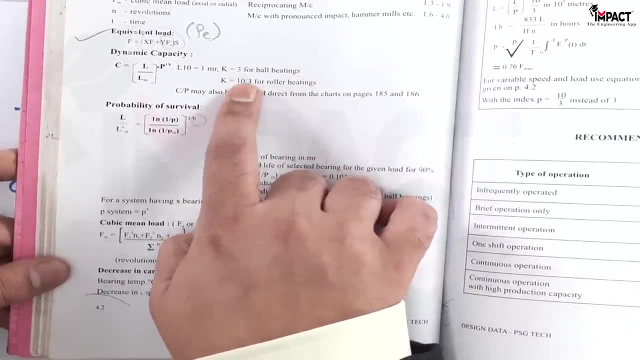 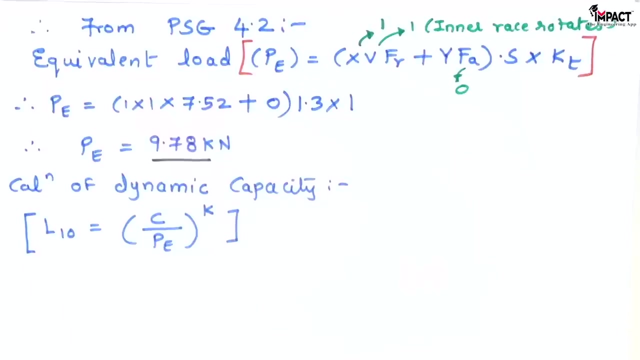 Now this formula is also there on PSG 4.2 over here, where we have to take K value equal to 3 for ball bearings and K equal to 10 by 3 for roller bearings. So since we are using ball bearings, K value would be equal to 3 and so therefore putting: 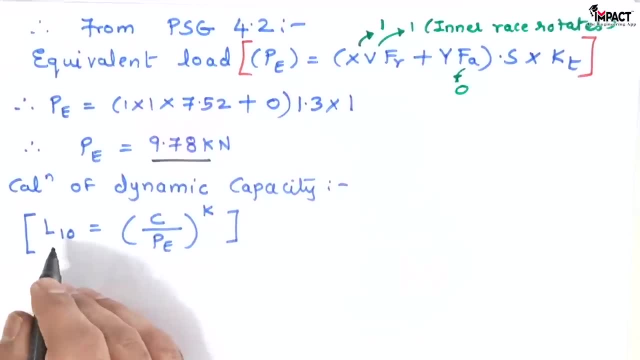 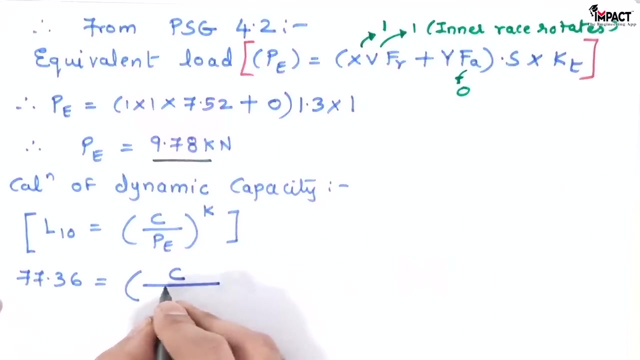 the values L10, we have got the millions of revolution, which was 77.36, is equal to C, is what we have to find out. that is the dynamic capacity, and equivalent load is 9.78 kN. So that is the dynamic capacity. 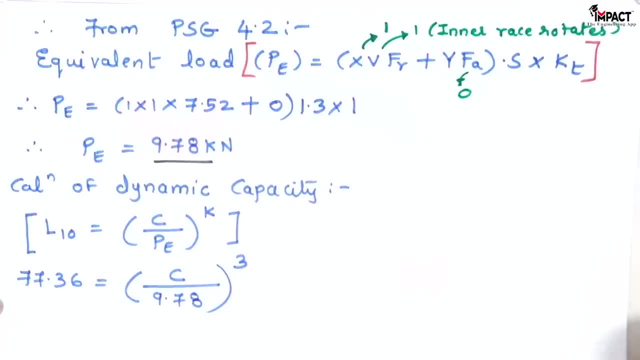 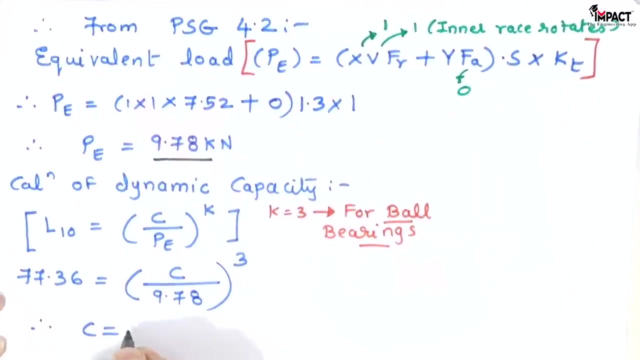 So that is the dynamic capacity. Or, if you haveRaise to power 3, because this K is equal to 3.. Ball bearings, And if it is roller bearing, the value is 10 by 3.. Now, from this C comes out to be: it is 41.68 kN. 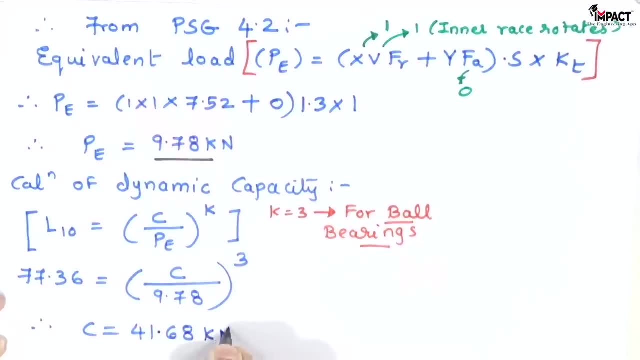 Now I want the value in terms of kGFC. first I will convert it into N x 10, raised to 3 N, And dividing it by 11.6, into a sin 9.4.. What is this? This is my depth. 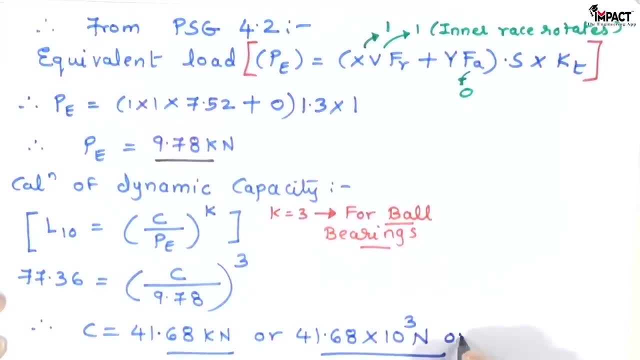 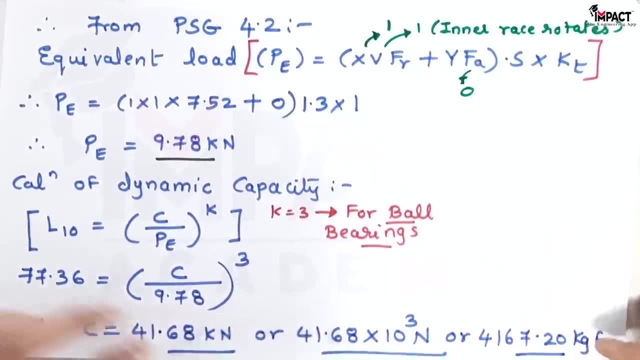 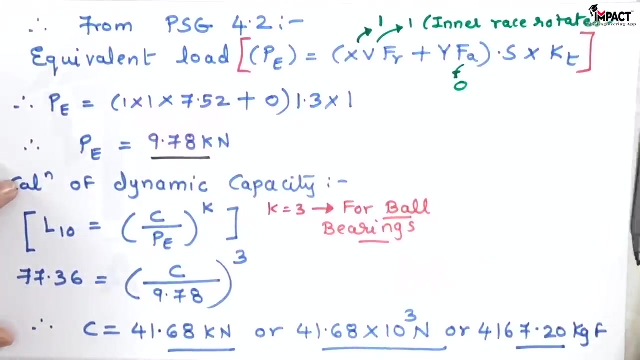 What is this? This is P Quando 1.3 registos al domestic mass growth 10.. So it is 4167.20 kgf. Now how to select the bearing for that. I am giving a short cut here. First, the bearing shaft diameter. the diameter which goes into the bearing is: 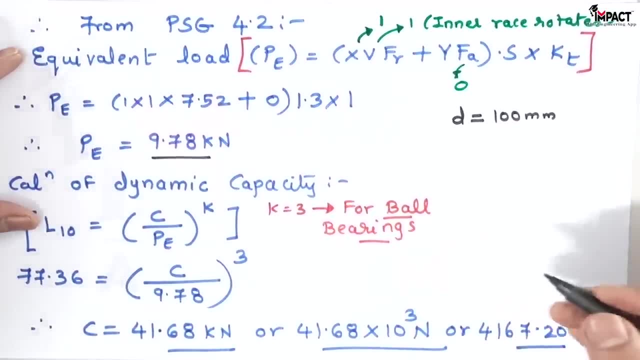 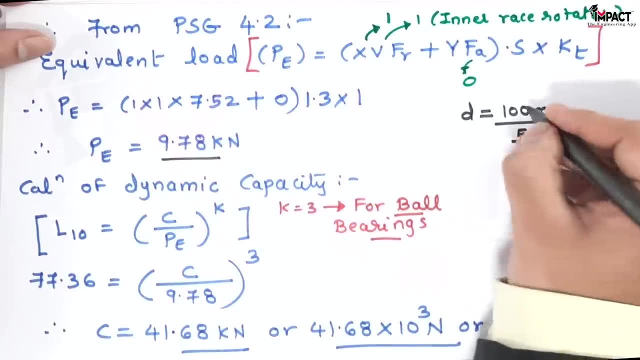 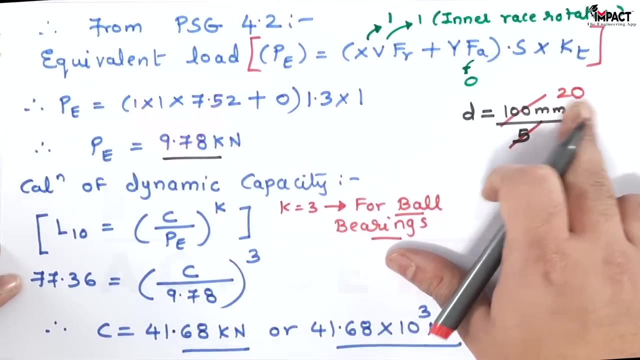 100 mm. So divide this by 5.. Simply divide this by 5.. So here it comes out to be 20.. So now we have to select those bearings whose last two digits are 20.. And for that, and 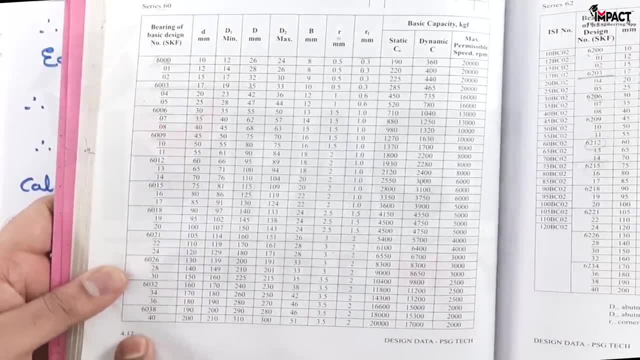 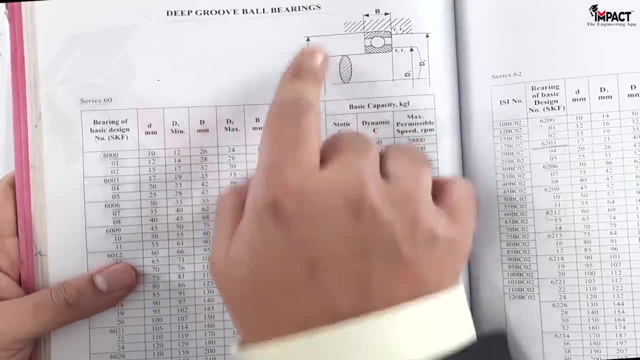 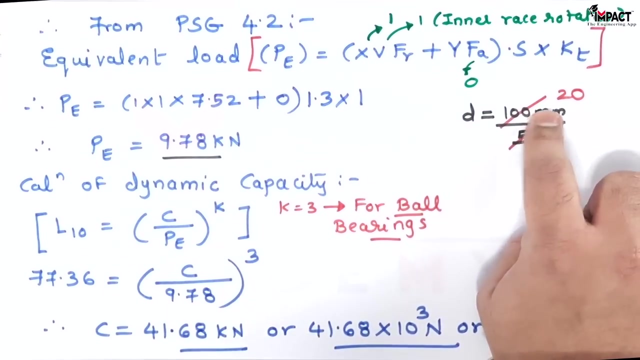 starting with PSG 4.12. as we can see here At the top it is written deep groove ball bearing, So it is DGBB. The diameter of the shaft is 100 mm And now, as I have explained, we have to check for the last two digits having. 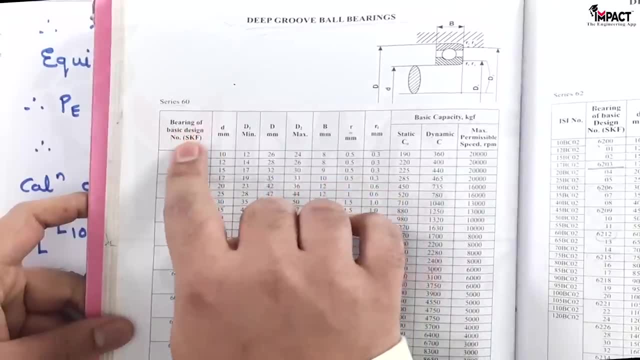 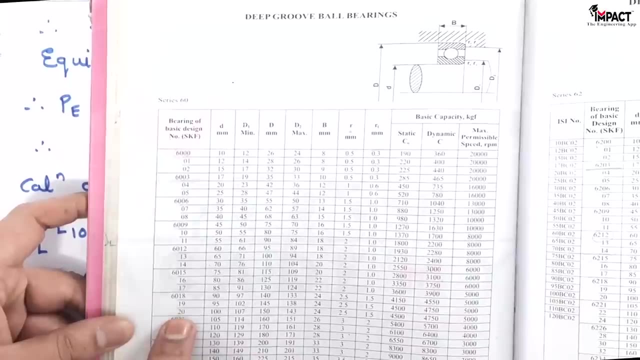 20.. So the bearing selection would be SKF series. Last two digits should be 20.. So here we have: it is 2.0.. So it is 6.020.. This is the bearing number And currently. 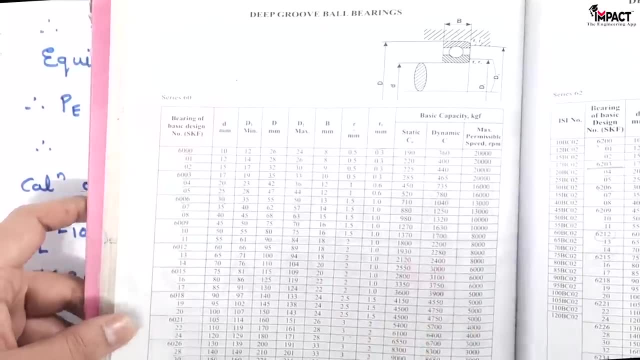 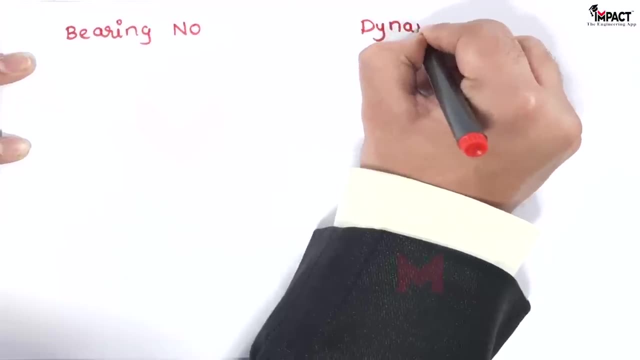 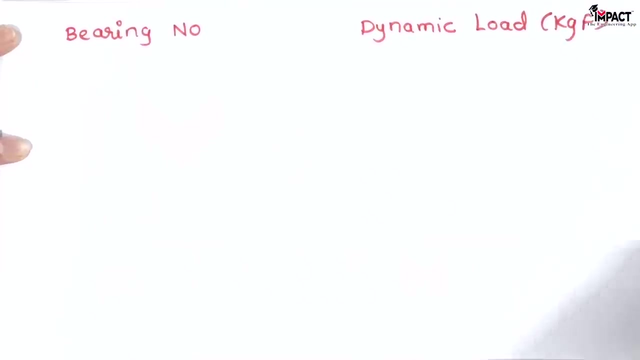 corresponding to it. we have to select the dynamic capacity. So I am writing it over here. I am writing the bearing number and the corresponding dynamic load, which would be in terms of kgf. Bearing number first, which is selected, is 6.020.. Corresponding to it. 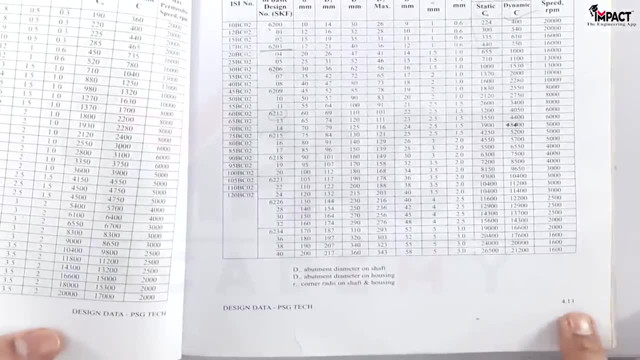 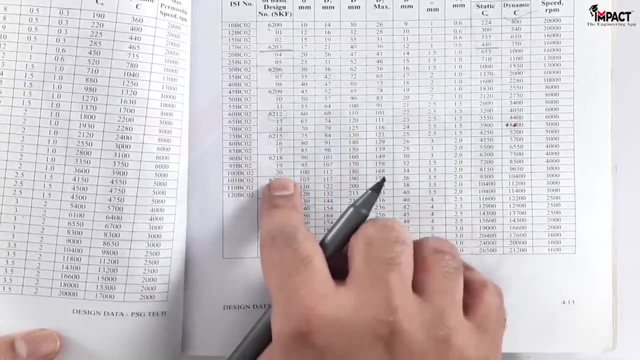 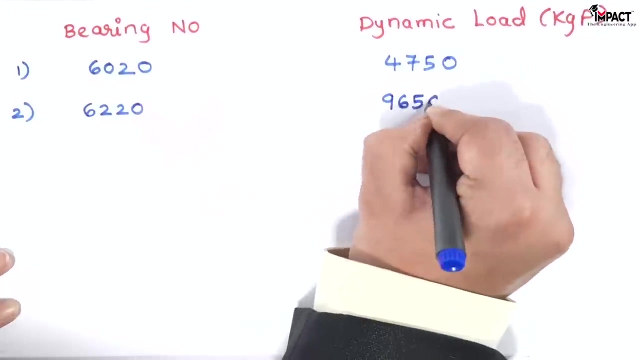 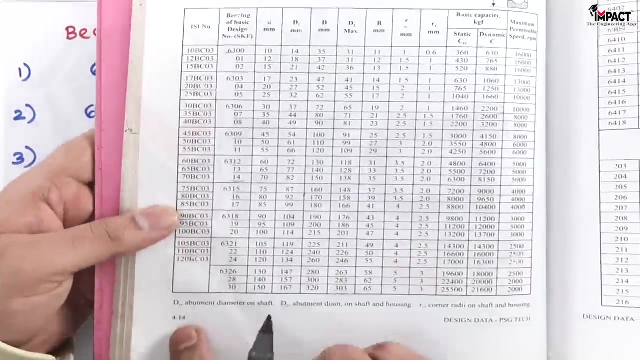 next, on PSG 4.13,, again, the last two digits should be 2.0.. So yes, it is 6.220.. And the dynamic load capacity is 9650 kgf. Third, on PSG 4.14, here we have 6.300.. So 6.320. 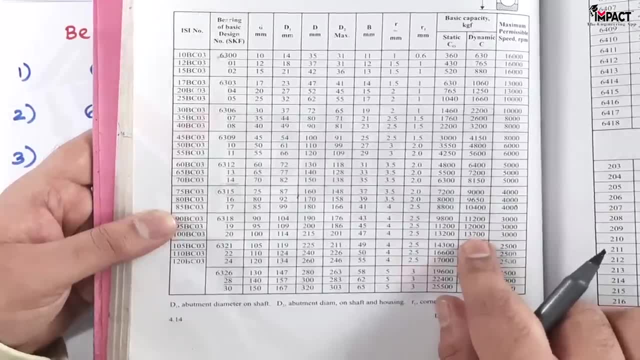 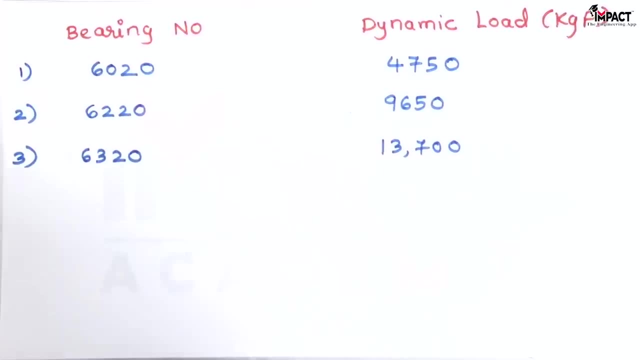 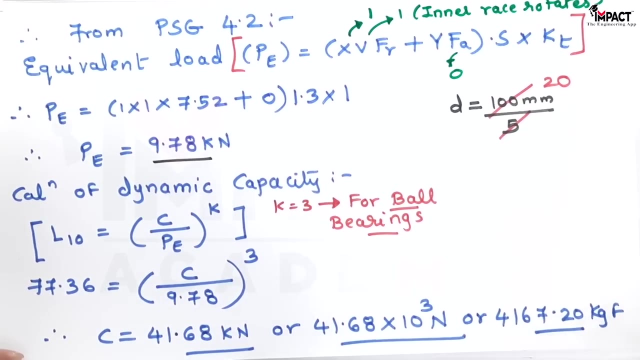 And the value is of dynamic load is 13700 kgf. Next, out of these loads, we have to see that the load which we have got, that is, the dynamic capacity, is closer to which one. So here the dynamic capacity is 4167, which is required And out of the bearing. 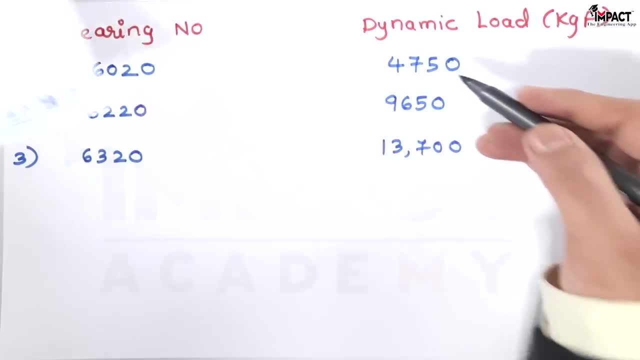 selected, we can see that the first bearing is closer to this load And the remaining bearings? they can resist more dynamic load. So if we go on increasing the dynamic load or the bearing number, then the cost may go on increasing. So, selecting a bearing of 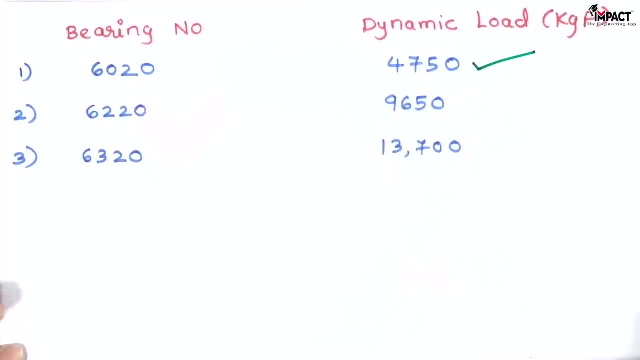 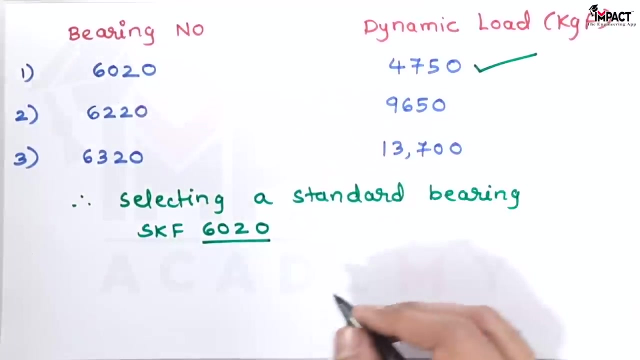 SKF 6.020.. So I am writing, therefore selecting a standard bearing SKF 6.020 which can resist the given kind of loading. Now, this is one of the reasons for which we are looking for the level of dynamic load. 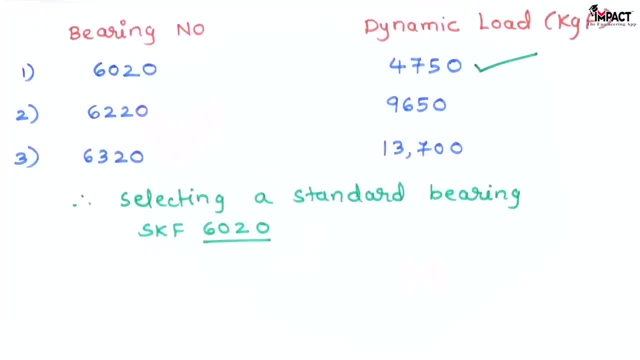 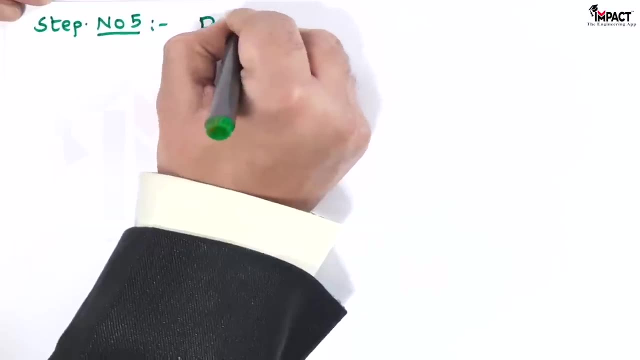 as we are seeing. So here, this is the bearing level and it will go up to the level of the dynamic load, as we are seeing here. So with the bearing selection we have reached up to Step number 4.. Now only step 5 is left. 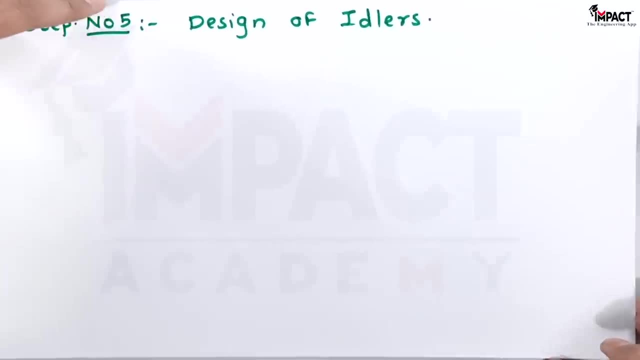 which is the design of the idlers. So here, Step number 5 is the design of idlers. and remember here idlers as well as the straight idlers. So for that now I am writing that idlers are tubes. 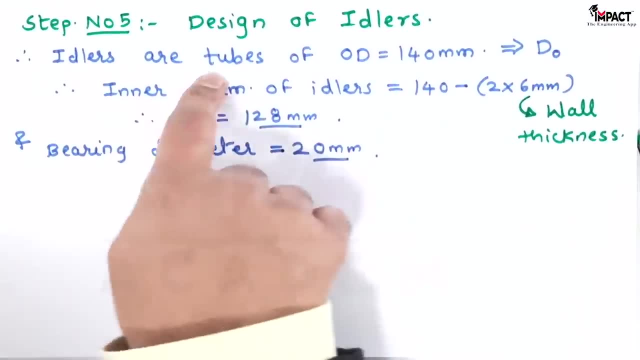 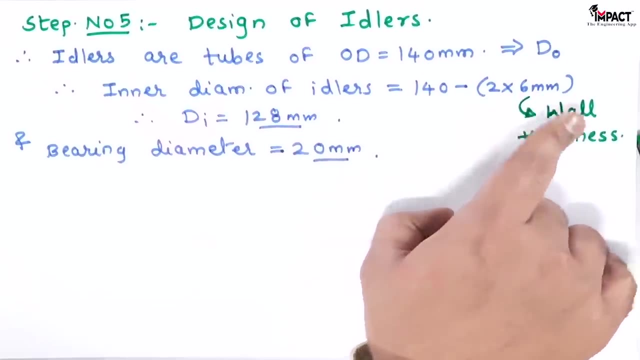 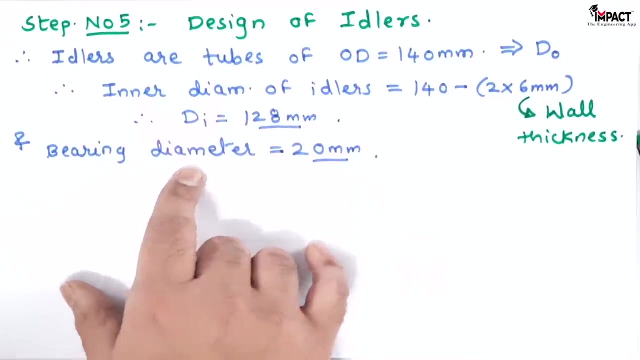 Now the idlers are tubes having outer diameter 140 mm and their inner diameters are taken as outer diameter minus 2 into wall thickness. So the thickness of the idlers are 6 mm, Inner diameter comes out to be 128 mm and the bearing which would be fitted inside that idler 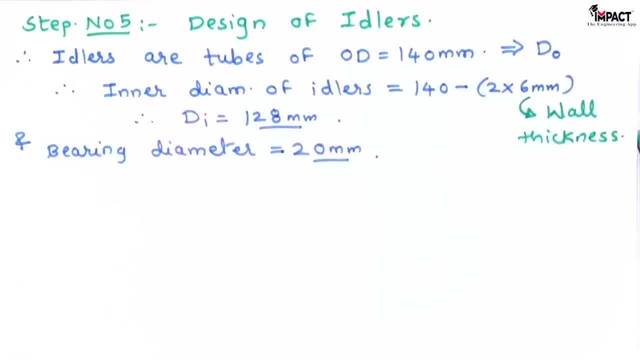 is having a diameter of 20 mm. And now, since the top idlers are carrying the material, so they are severely loaded compared to the bottom idlers. So we are going to design the top idlers, in this case the truffing idlers. So here I am going to mention the point. 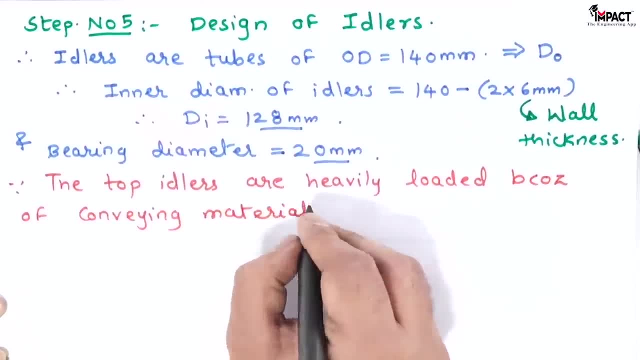 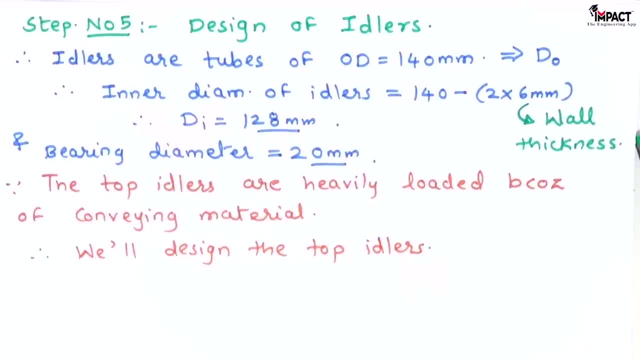 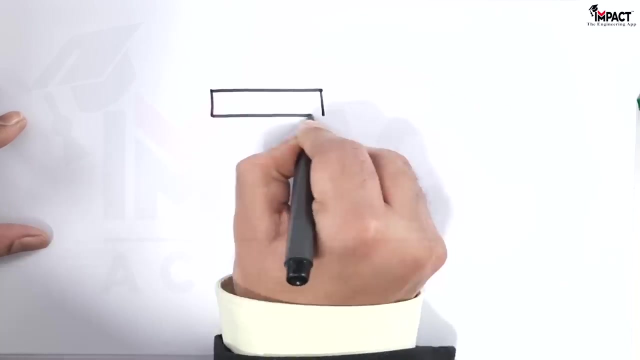 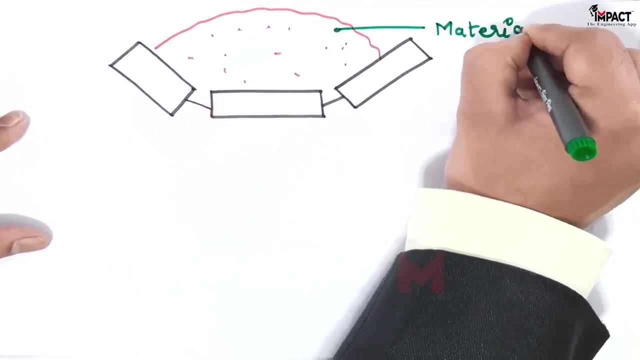 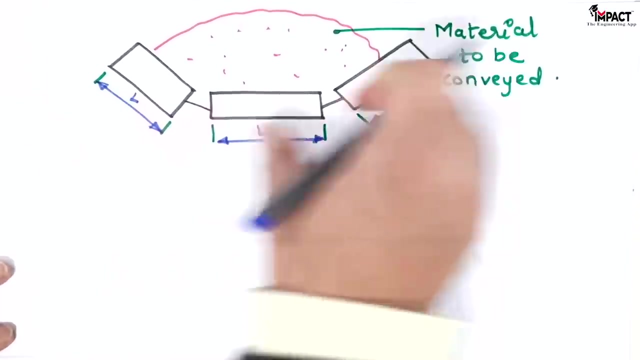 So, therefore, we are going to design the top idlers because they are being heavily loaded. I will quickly draw the diagram for the idler. for the top idler Now, the lengths would be kept same of these rollers At the same time, since we can see that the 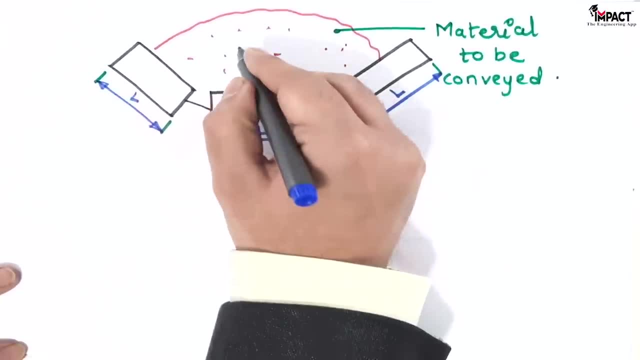 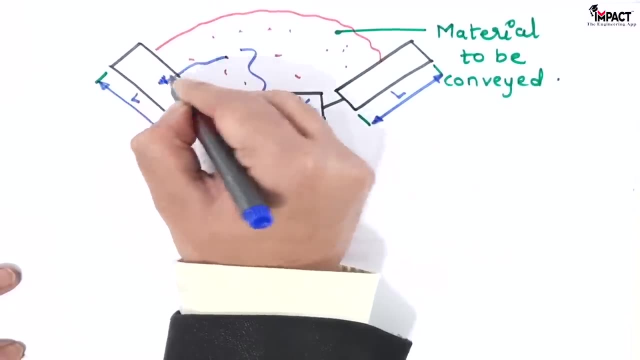 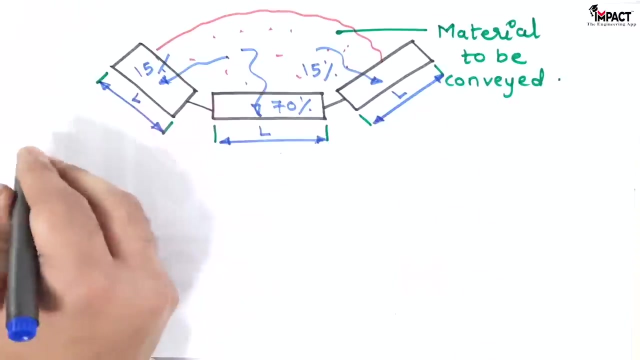 middle roller would carry the maximum weight of the conveyed material. So I can assume that 70 percent of the load is carried by the middle idler and remaining 30 is divided equally, 15-15 percent- on the remaining two idlers. Now, therefore, the total weight for one side of the ridler we have taken as our total idler, So we are nothing but 17 cbm. All contributions will be paid to the roll, which is approximately 18% of this dost Tyson running assimilator. So we can just write that end importance by having the total weight of. this idler with 1000 parts here. So the editors should have said: buy結果 from the middle roller Milan. once you have selected it over, you can taste as they have indicated to such a procedure by adding a clause here at the bottom in the title. So fairly disappointed by 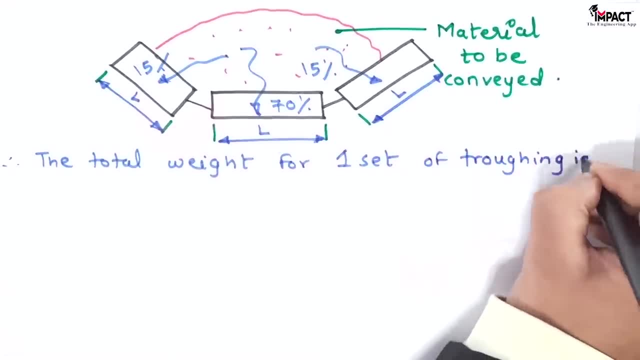 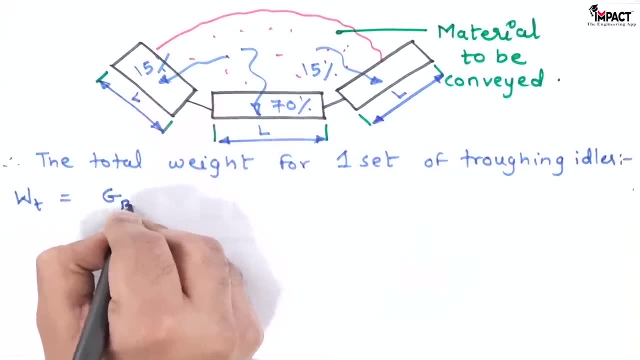 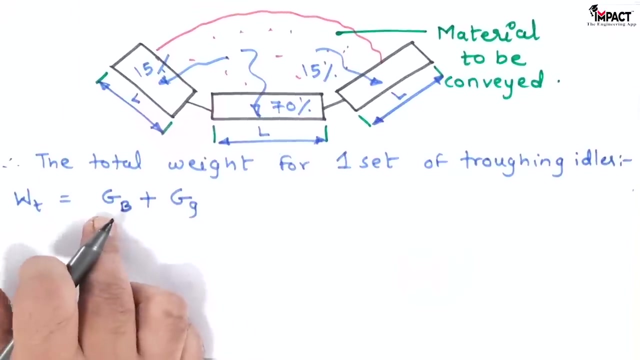 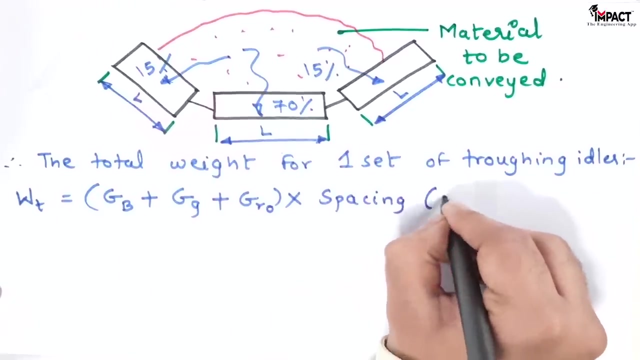 set of truffing idlers is W suffix T is equal to it. is G suffix B plus G suffix G. we have seen previously: G suffix B is for the conveyed material, G suffix G is for the belt plus GRO, that is for the truffing idlers into the spacing denoted as S. Now previously we have 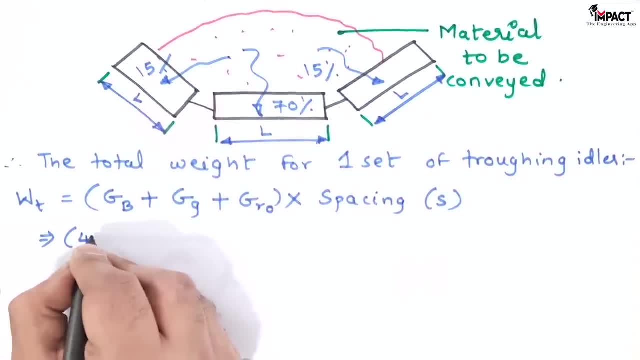 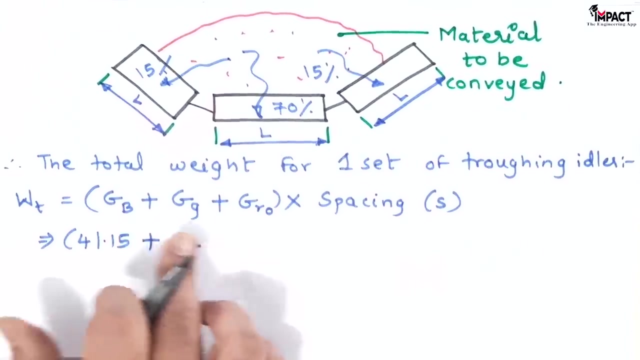 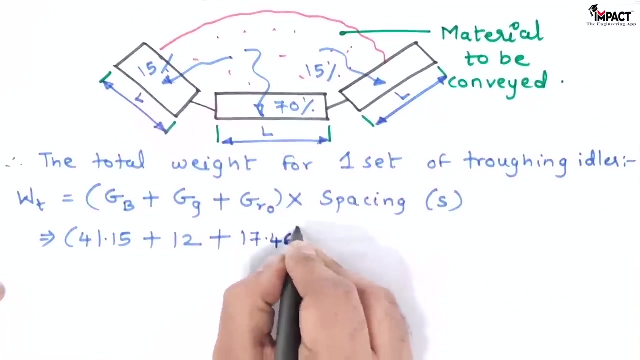 calculated for the top run, GB value was and even for the bottom run it was 41.15 plus G suffix G value for the belt was 12.. So you all can refer the video previously what in which way I calculated GB, G suffix G. it was there in step number. second, in the motor selection part, GRO 17.46 into.